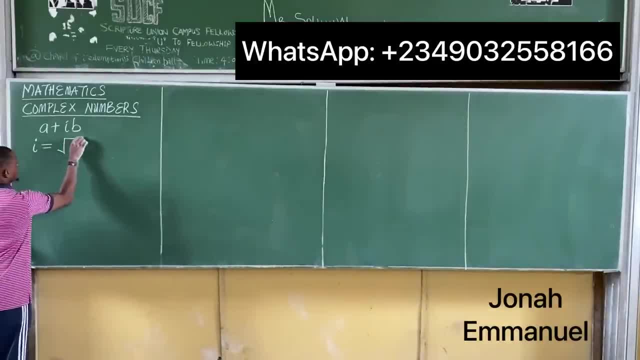 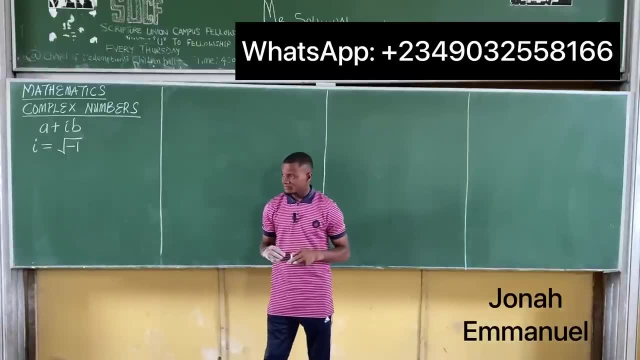 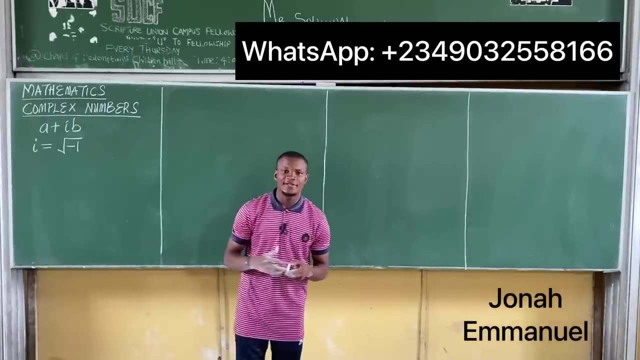 is equal to the square root of minus. Alright, so any number in the form a plus ib is called a complex number. Now, before the 16th century, it was difficult to find the square root of a negative 10.. Alright, for instance. 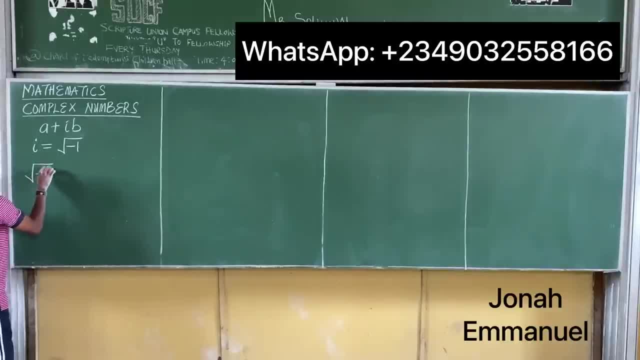 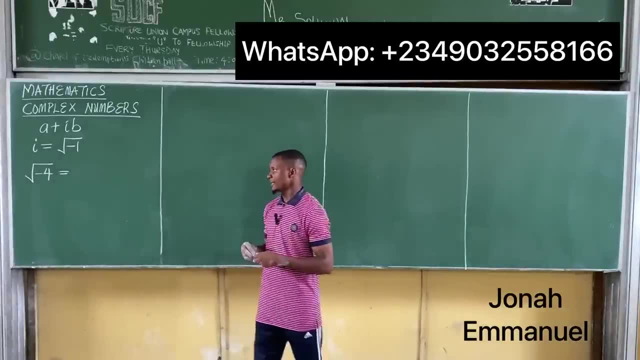 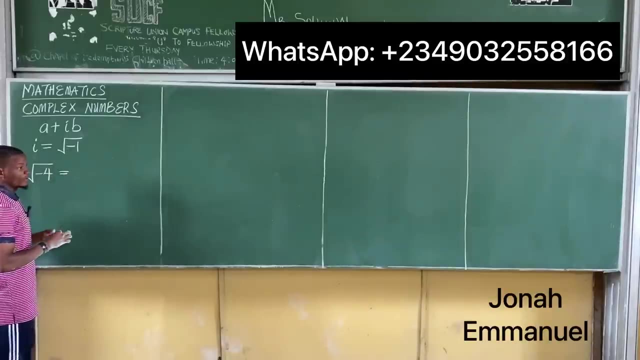 if I'm to get the square root of, let's say, minus 4, this would have been impossible not until the 16th century. It was in the 16th century that the idea that i should be equal to square root of minus 1 was formed, and hence it gave us the edge. 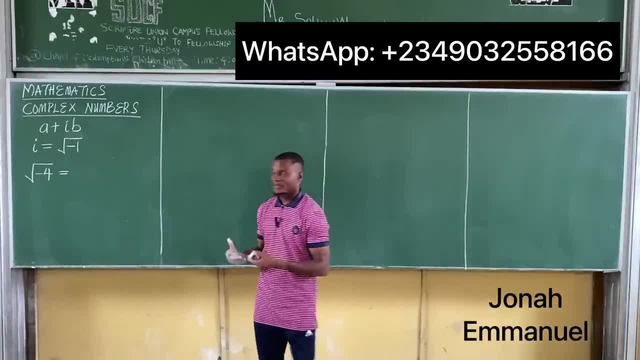 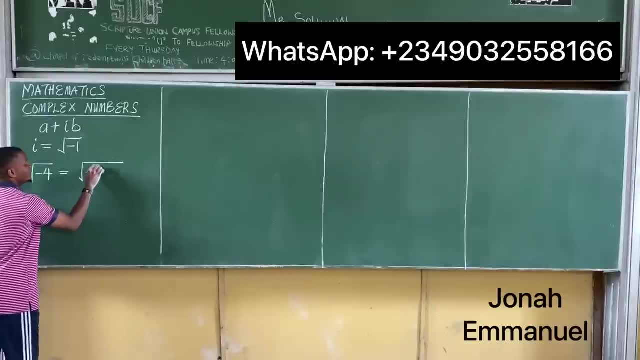 or the ability to find the square root of a negative 10.. How, From here, if I'm to solve this using the idea of sod, this would be equal to the square root of minus 4, sorry, the square root of this becomes equal to the square root of 4 times minus 1.. 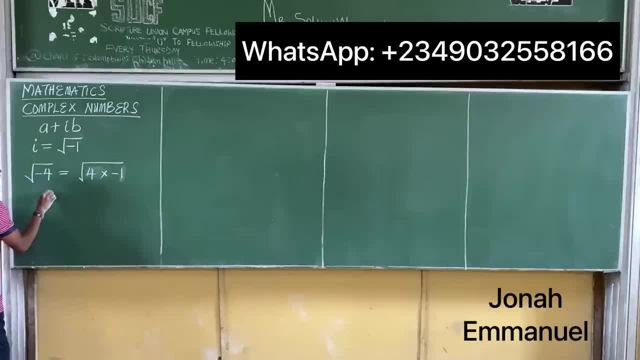 So I have this. of course, 4 times minus 1 gives you minus 4.. So this is equal to: we can separate this: 2, square root of 4 times square root of minus 1.. From the idea of sod, this is correct. 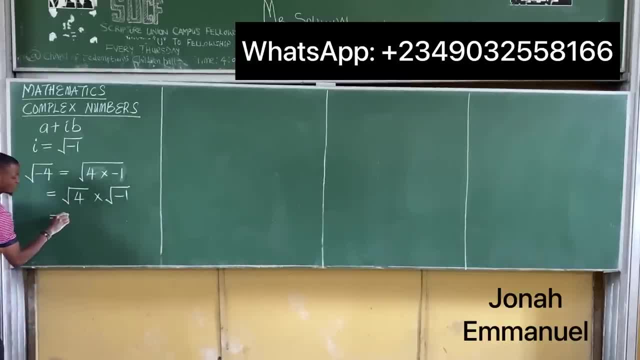 Okay, this is equal to square root of 2 of 4 is, of course, 2 times root minus 1.. Now we said root minus 1 is equal to i, So this is equal to 2i. Alright, so hence the square root of a. 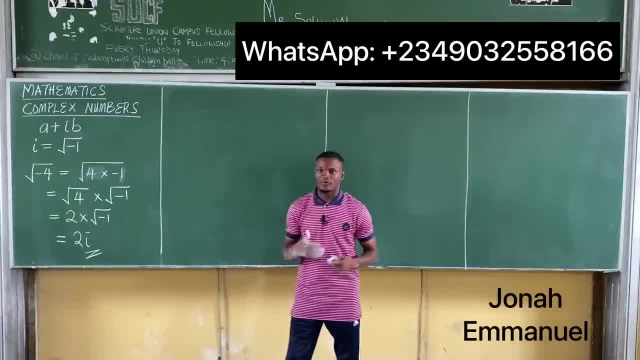 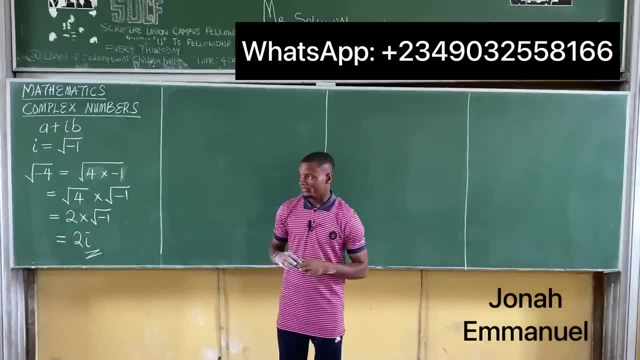 negative 10 can now be found. Example: the square root of minus 4 is equal to 2i, and this is a complex number. Say i is equal to the square root of minus 1.. Alright, so that's what a complex number is. 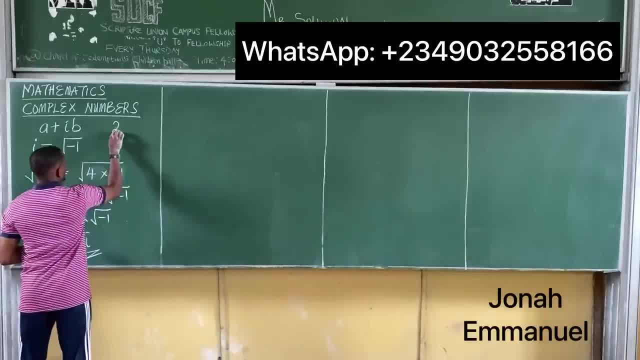 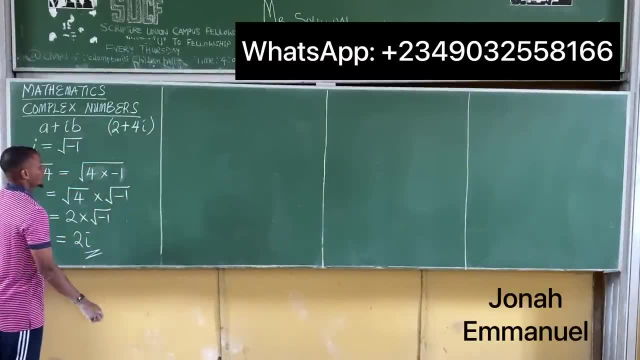 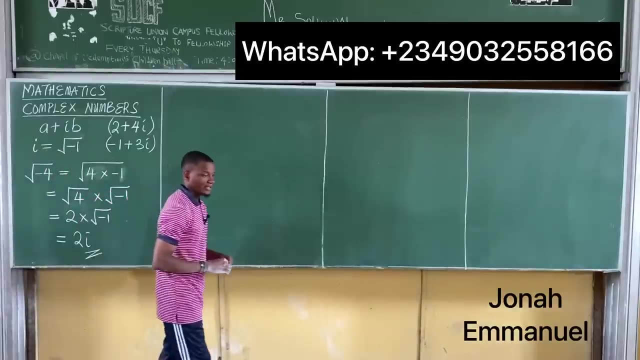 Examples of complex numbers include 2 plus, let's say, 4i. This is a complex number, right? So observe, I'm placing the i after the number, Is it okay? Minus 1 plus 3i is a complex number, etc. Alright, next up, let's look at the representation of complex numbers. 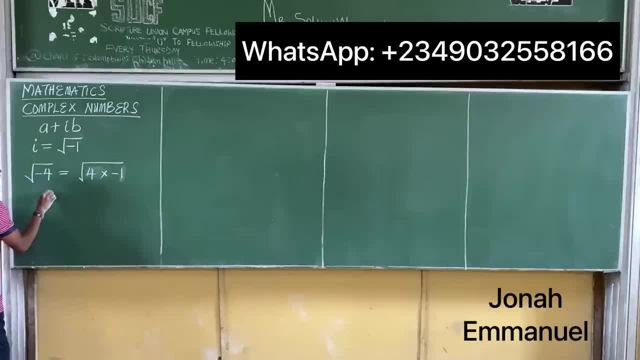 So I have this. of course, 4 times minus 1 gives you minus 4.. So this is equal to: we can separate this: 2, square root of 4 times square root of minus 1.. From the idea of sod, this is correct. 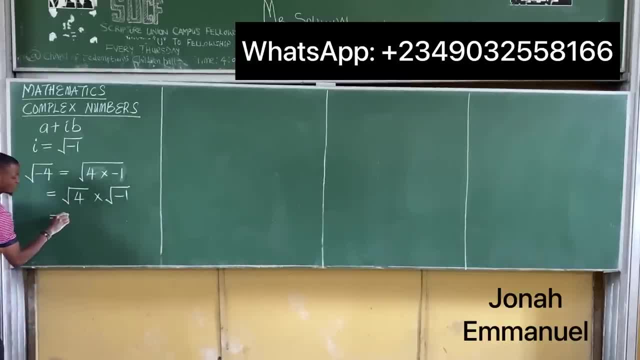 Okay, this is equal to square root of 2 of 4 is, of course, 2 times root minus 1.. Now we said root minus 1 is equal to i, So this is equal to 2i. Alright, so hence the square root of a. 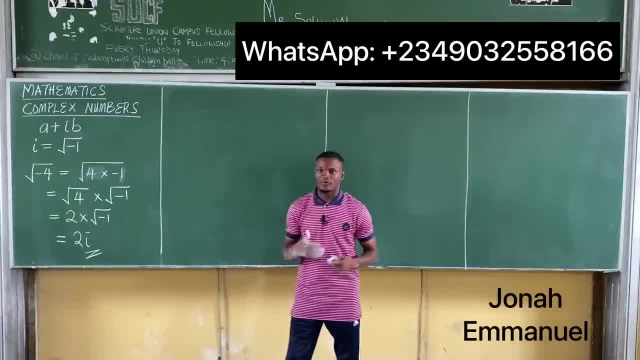 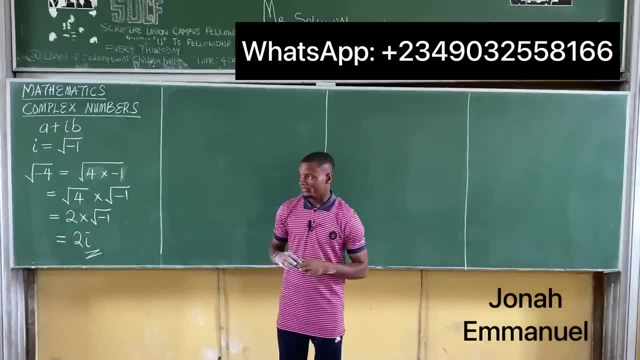 negative 10 can now be found. Example: the square root of minus 4 is equal to 2i, and this is a complex number. Say i is equal to the square root of minus 1.. Alright, so that's what a complex number is. 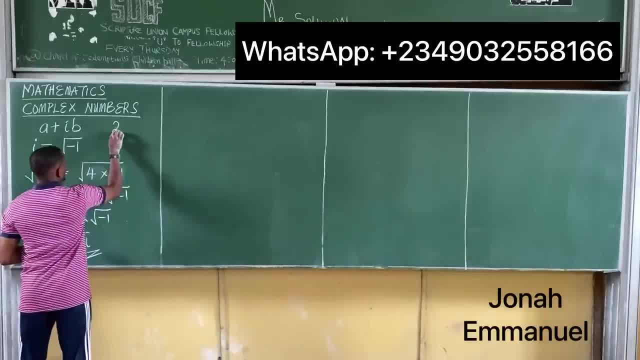 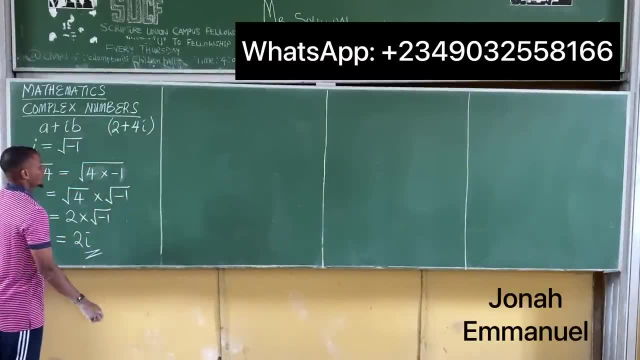 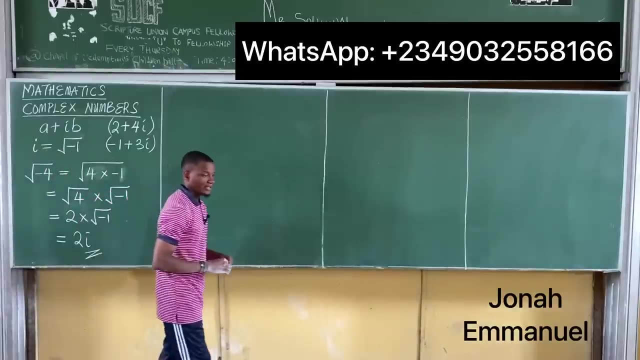 Examples of complex numbers include 2 plus, let's say, 4i. This is a complex number, Alright, so observe, I'm placing the i after the number. Is this okay? Minus 1 plus 3i is a complex number, etc. Alright, next up, let's look at the representation of complex numbers. 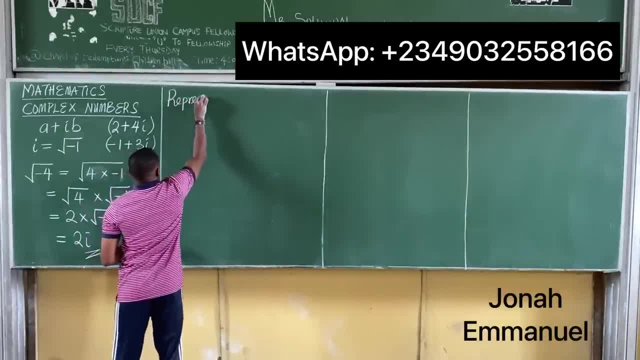 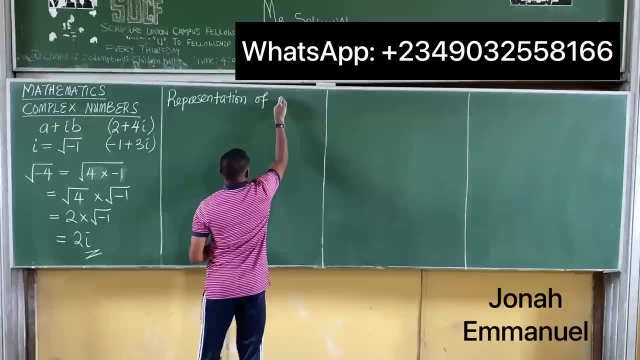 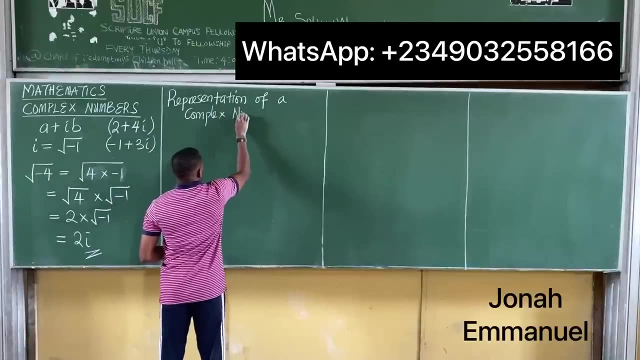 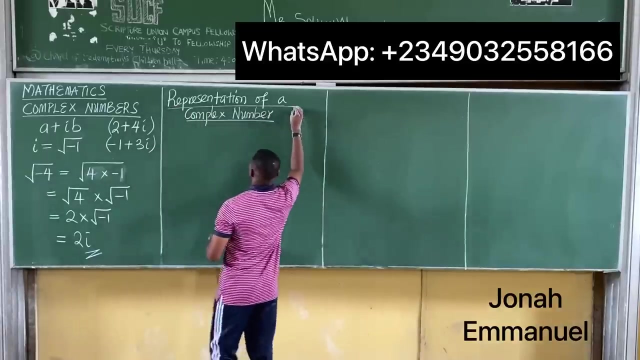 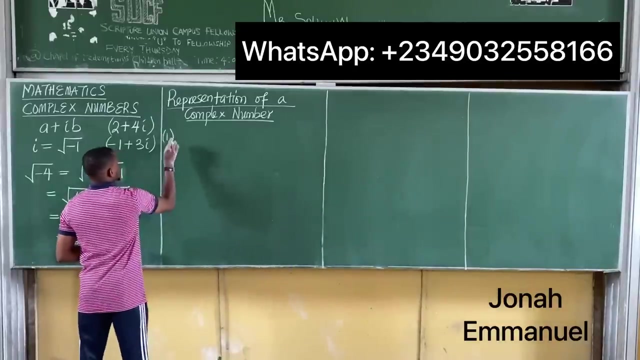 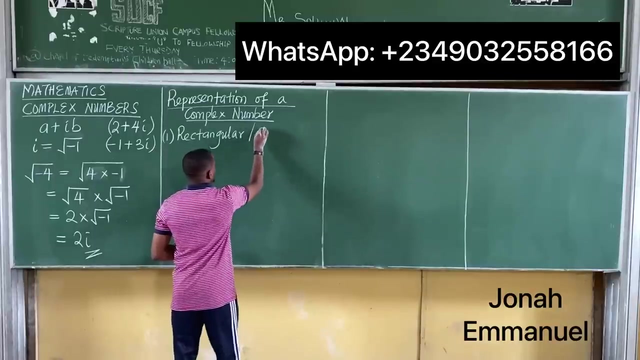 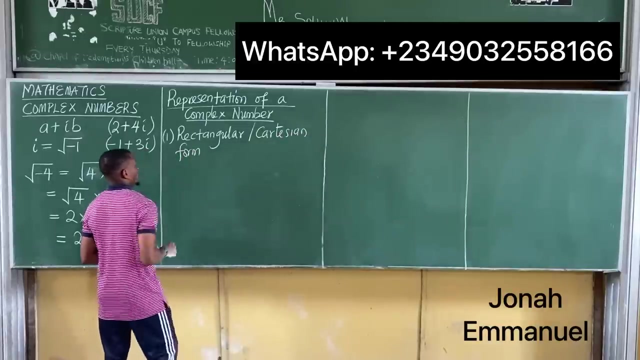 We represent. look at representation of a complex number. Alright, we represent complex numbers in different forms. The first one is called the rectangular. The rectangular also called the Cartesian, The Cartesian form. That's the first form of representing complex number. In this form, a complex number takes the shape a plus. 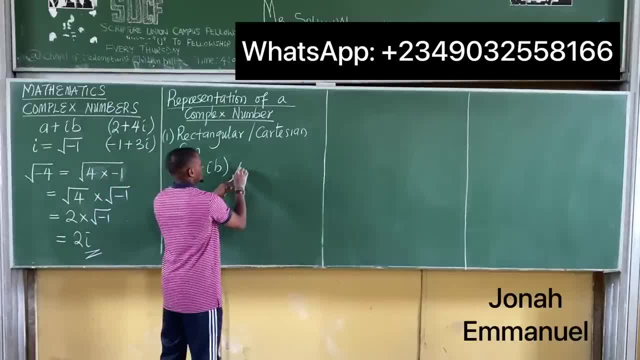 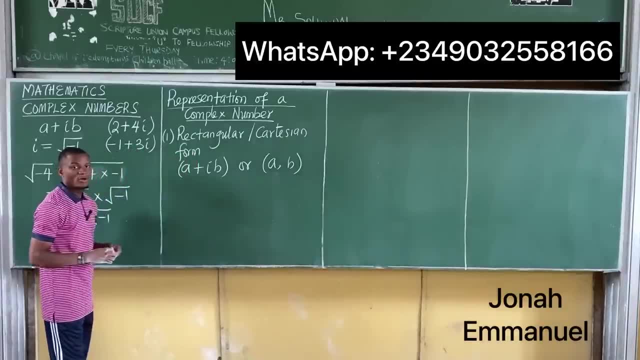 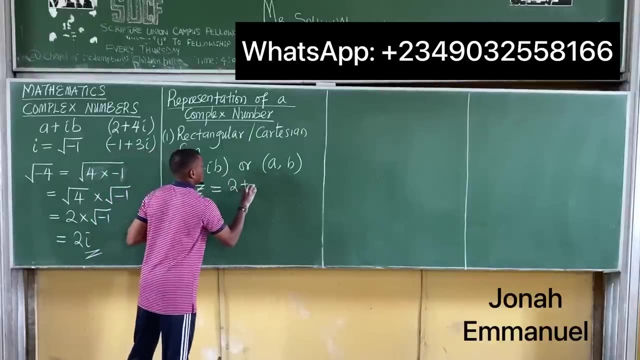 i, b, as we said earlier here, or perhaps in brackets a, b. Alright, so this is the Cartesian or the rectangular form of representing complex numbers. Example: let's say: complex number z is equal to 2 plus 3i. This is a rectangular or a Cartesian form representation of this complex. 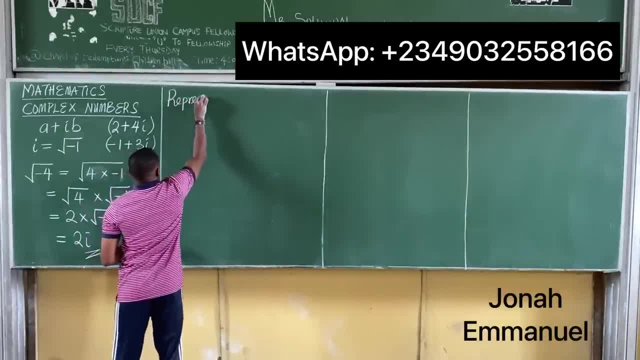 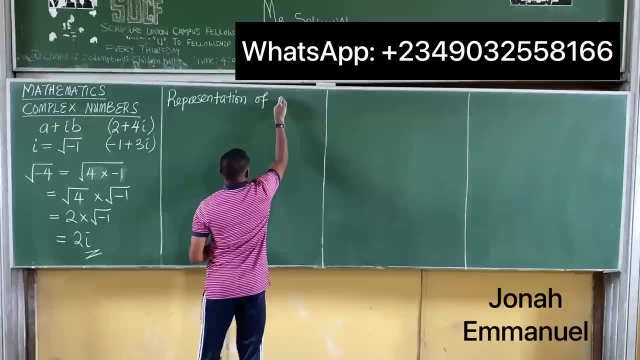 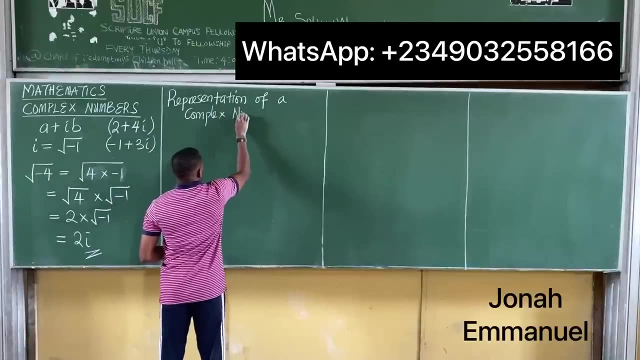 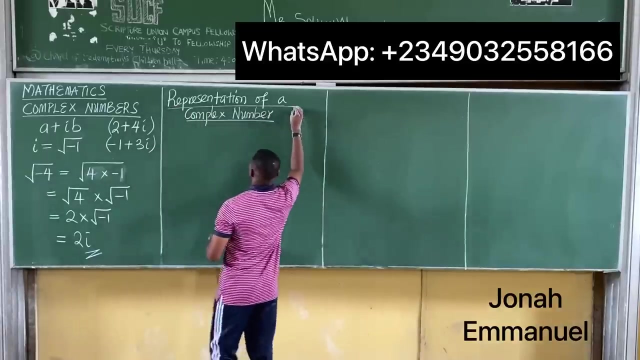 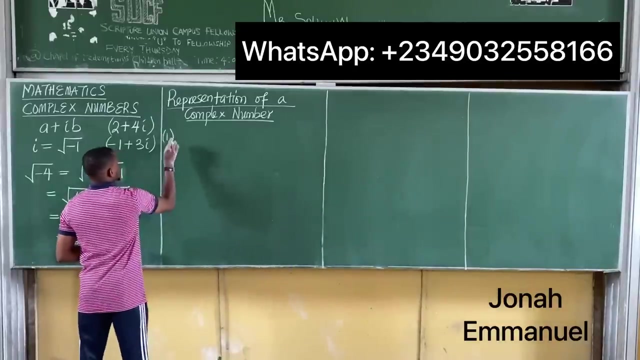 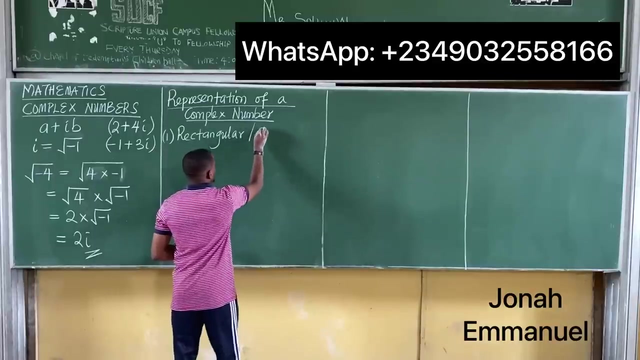 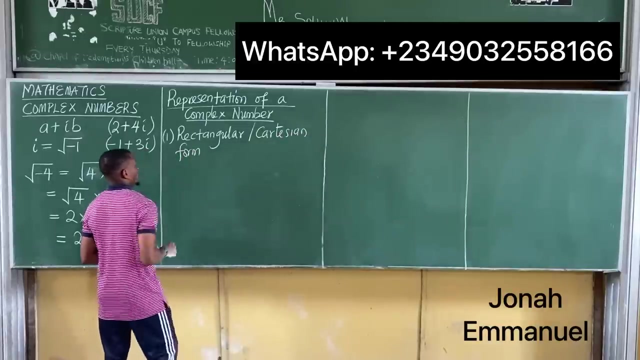 We represent. look at representation of a complex number. Alright, we represent complex numbers in different forms. The first one is called the rectangular. The rectangular also called the Cartesian, The Cartesian form. That's the first form of representing complex number. In this form, a complex number takes the shape a plus. 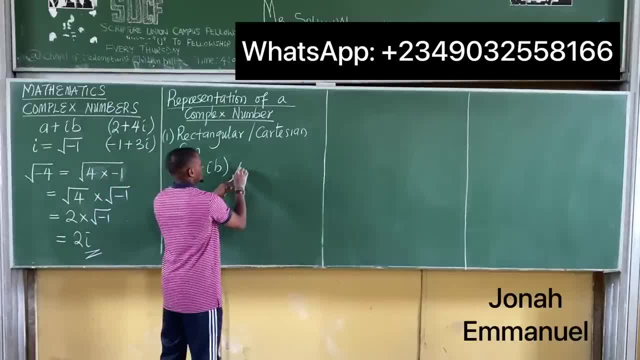 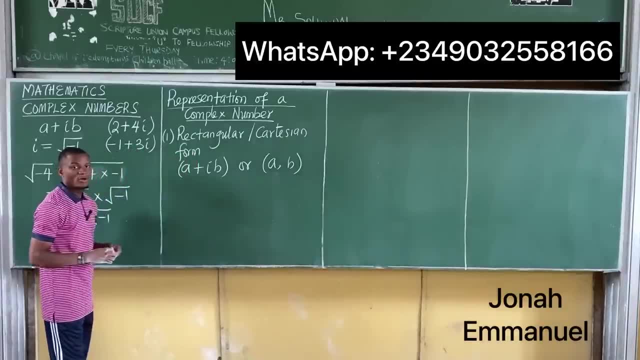 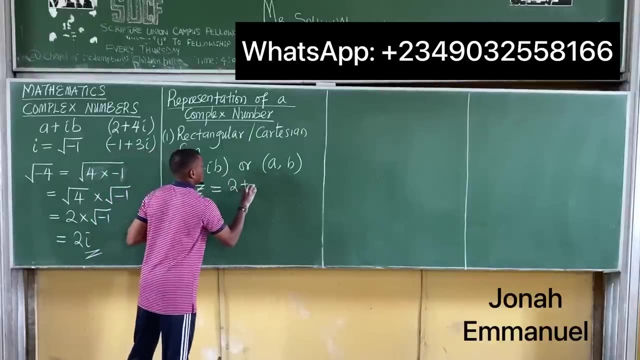 i, b, as we said earlier here, or perhaps in brackets a, b. Alright, so this is the Cartesian or the rectangular form of representing complex numbers. Example: let's say: complex number z is equal to 2 plus 3i. This is a rectangular or a Cartesian form representation of this complex. 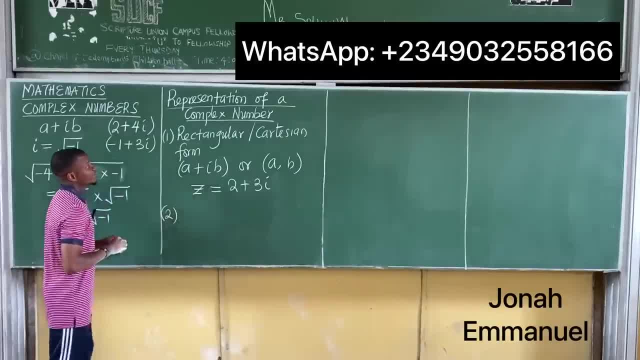 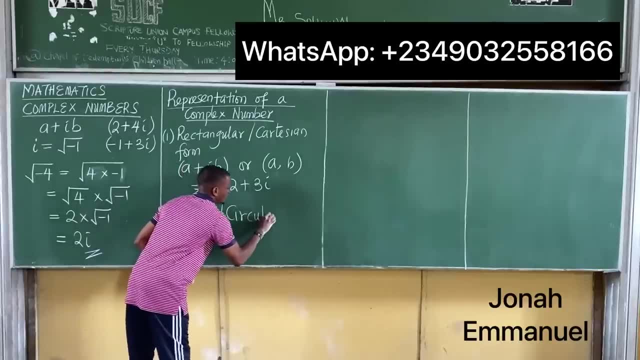 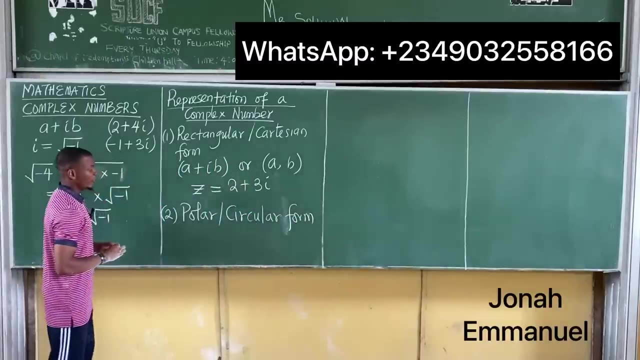 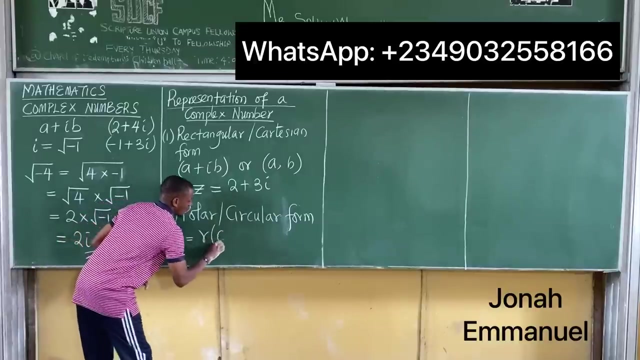 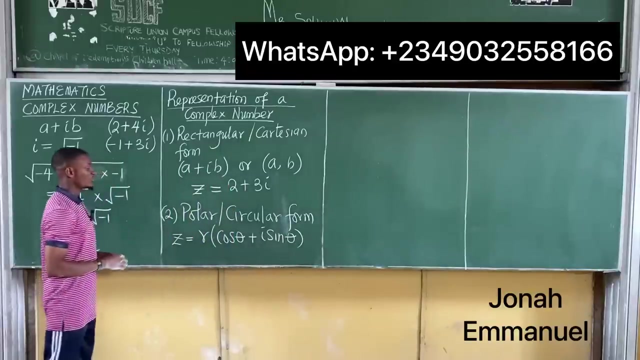 number. The second form of representing complex number is called the polar or the circular form, Or the circular form. For the polar form, a complex number is represented as z being equal to r into cos theta plus i sine theta. This is called the polar form or circular form, representation of a complex number. So let's look at the. 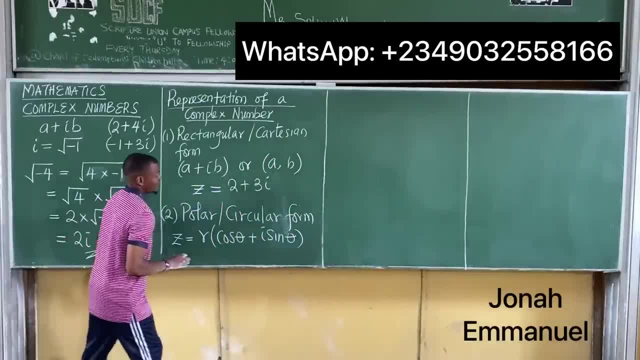 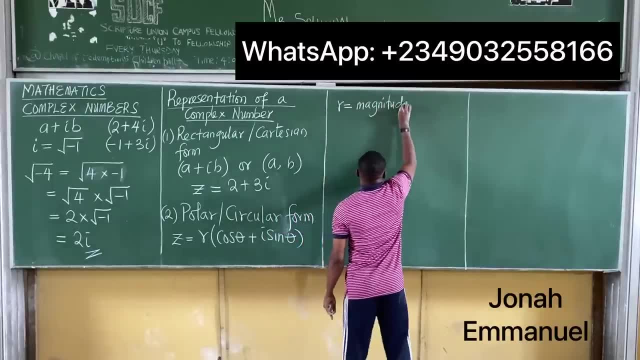 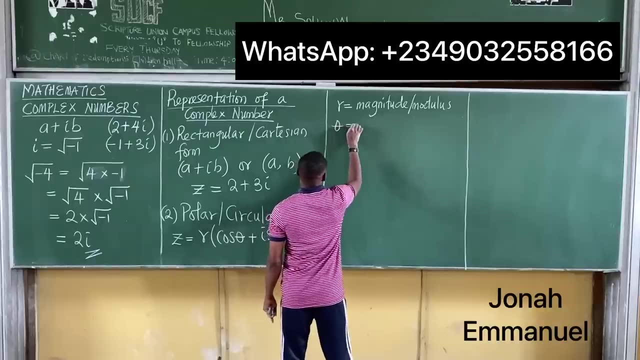 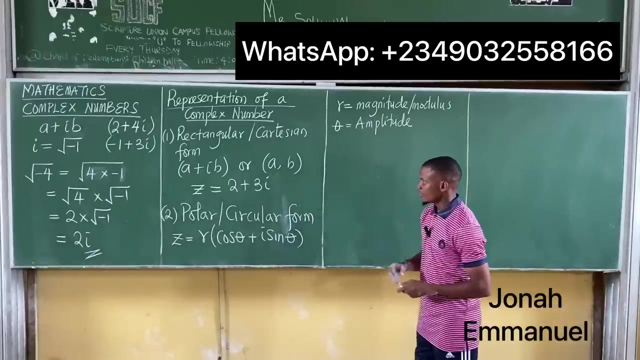 second form of representing complex number, where r is called the magnitude or the modulus of the complex number and theta is called the amplitude or the angle of the complex number. So this is the second form of representing complex numbers. The third form is called the. 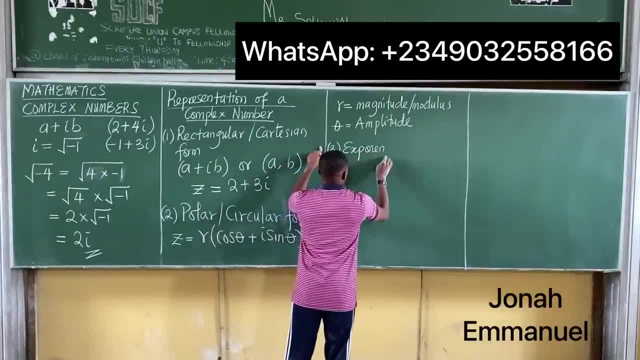 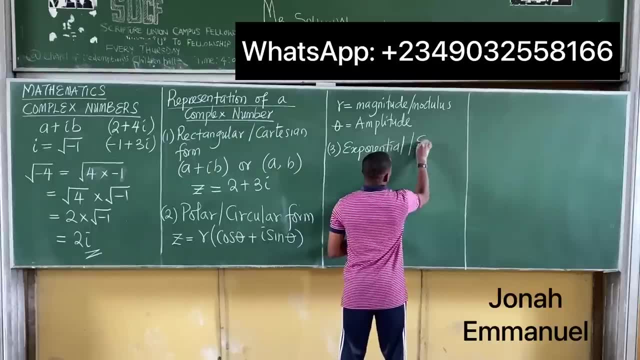 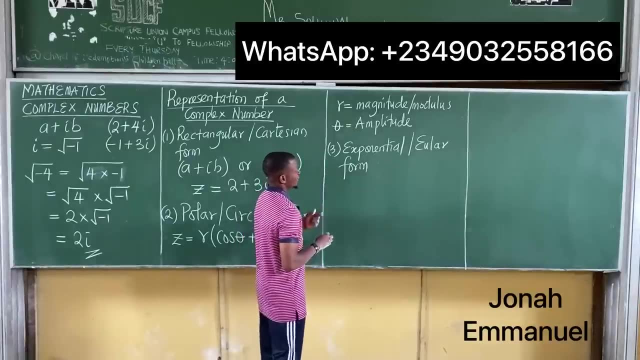 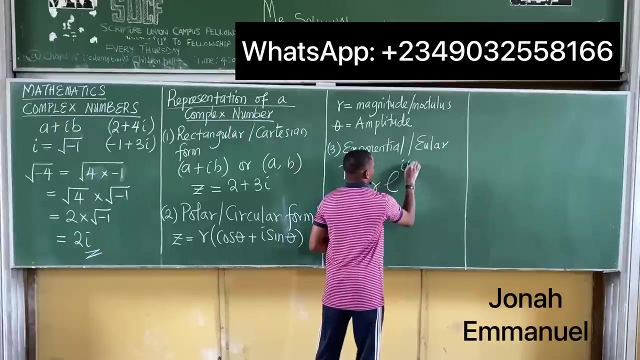 exponential. We'll give examples of this much more later. The third form is called the exponential or the Euler's form. Alright, or the Euler's form of representing complex number, We said, for here we have something of nature: z equal to r. exponential i times. 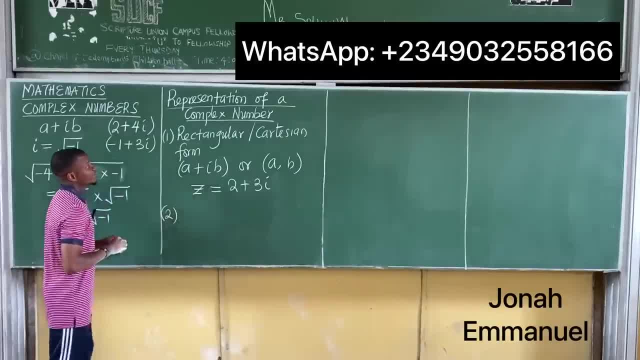 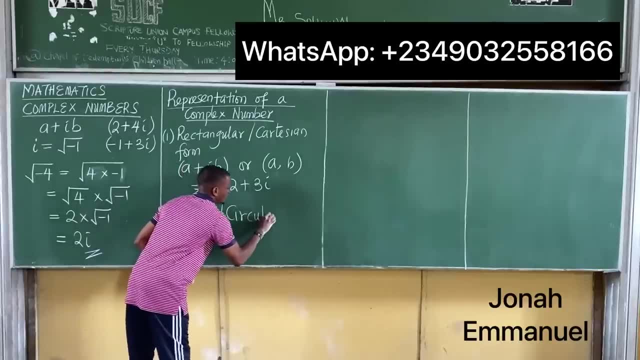 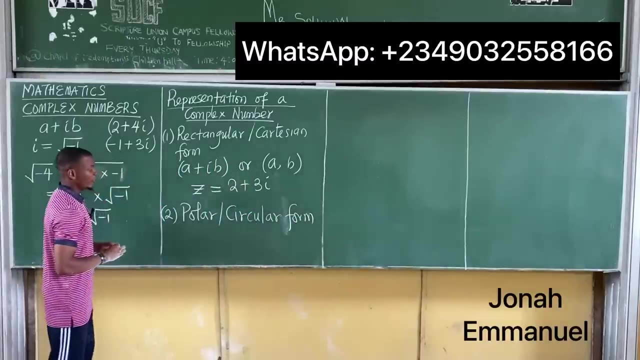 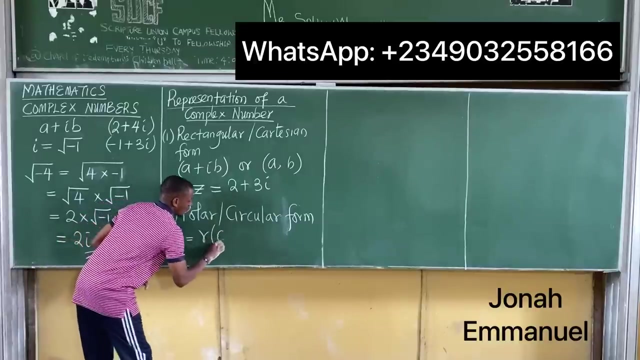 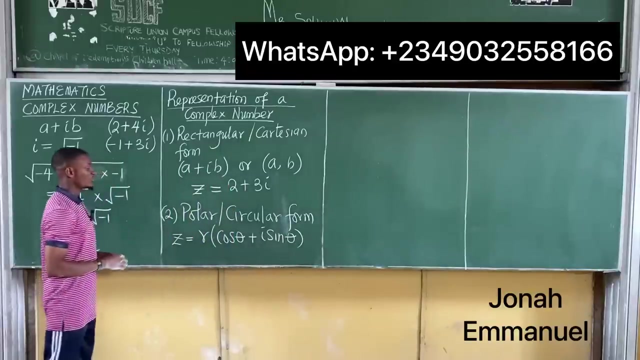 number. The second form of representing complex number is called the polar or the circular form, Or the circular form. For the polar form, a complex number is represented as z being equal to r into cos theta plus i sine theta. This is called the polar form or circular form, representation of a complex number. Alright, so this is a. 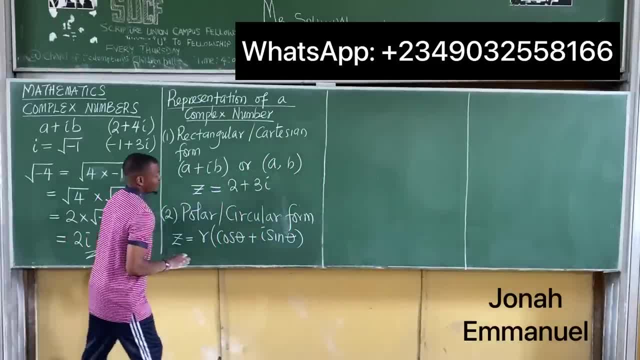 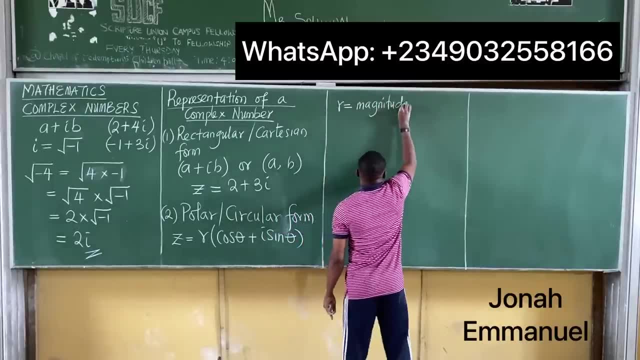 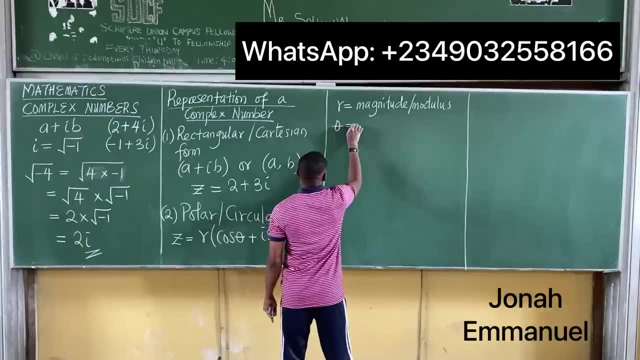 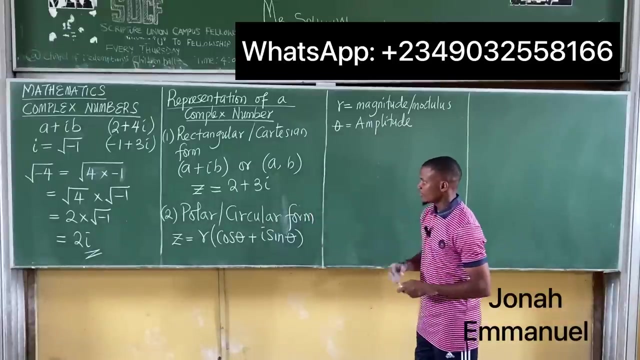 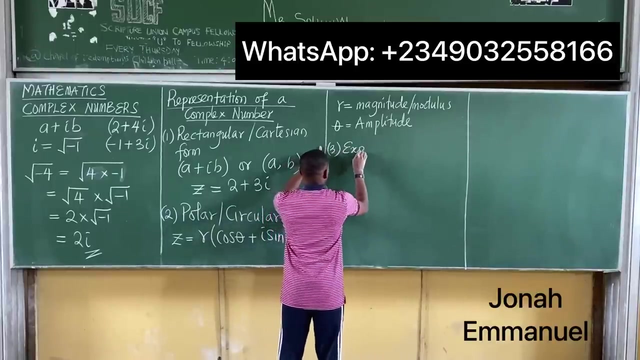 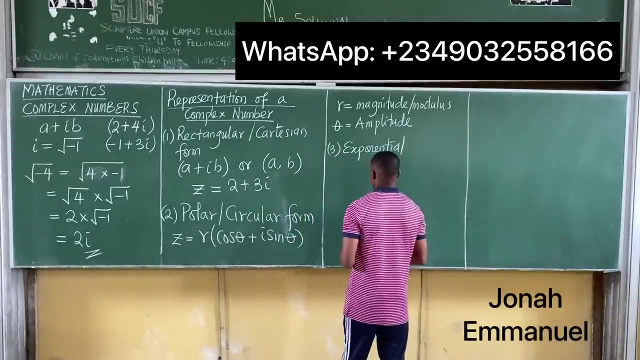 complex number, Where r is called the magnitude or the modulus of the complex number and theta is called the amplitude or the angle of the complex number. So this is the second form of representing complex numbers. The third form is called the exponential. We'll give examples of this much more later. The third form is called: 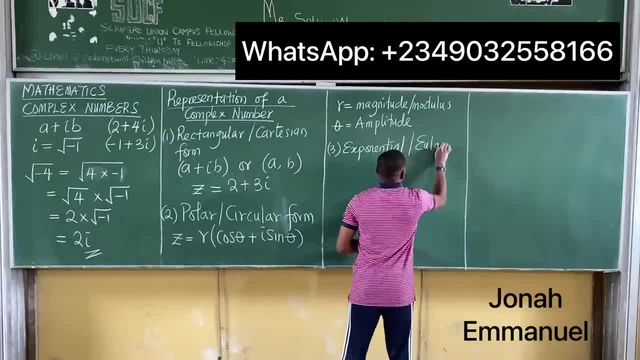 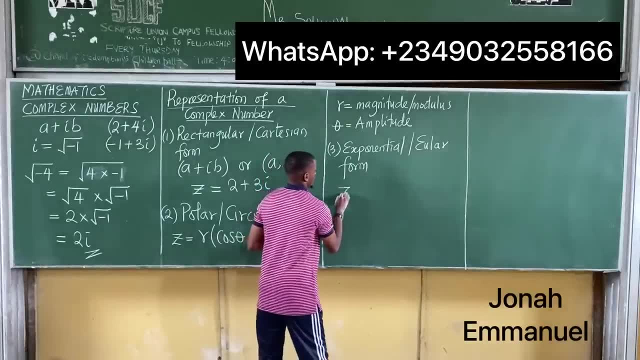 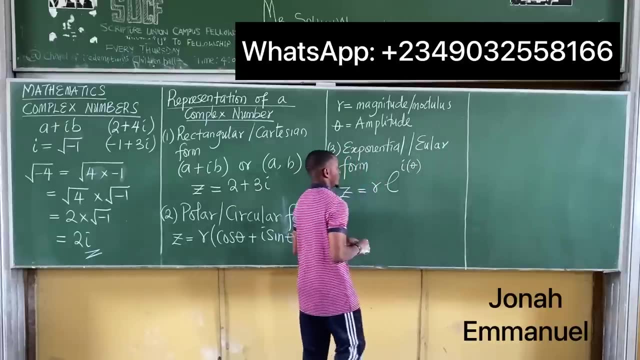 the exponential or the Euler's form, Alright, or the Euler's form of representing complex number. We said, for here we have something of nature, z equal to r exponential i times theta, Alright, so this is the Euler's form of representing complex numbers, Alright. 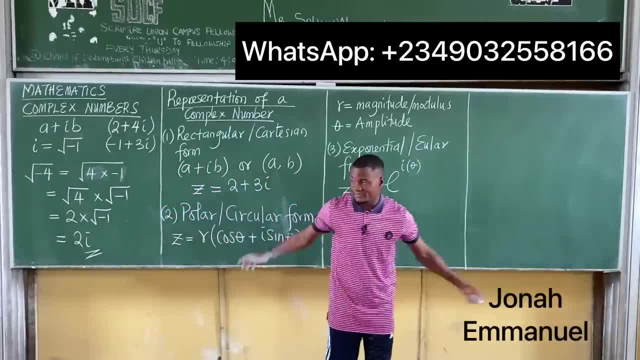 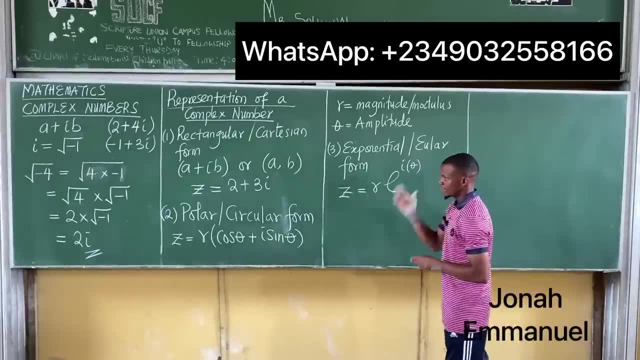 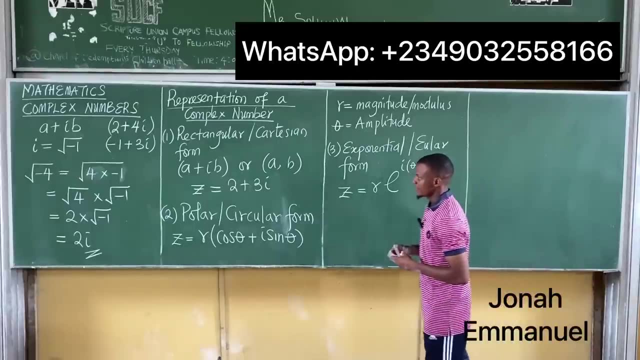 so we have our forms or pattern of representing complex numbers: Rectangular form or Cartesian, polar form or circular, then exponential form or Euler's form. Next up, let's look at the algebra of complex numbers. How do we add complex numbers? How do we subtract them? 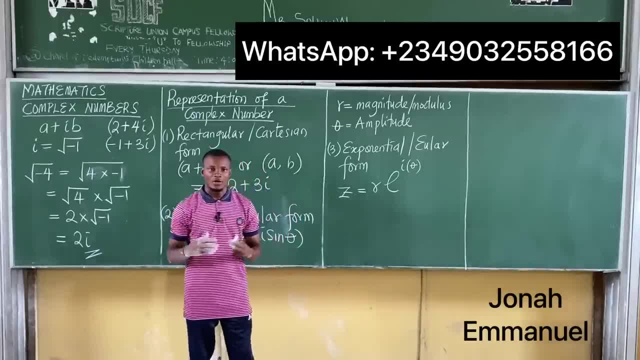 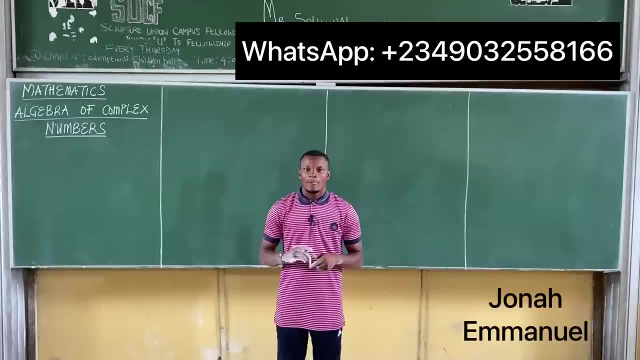 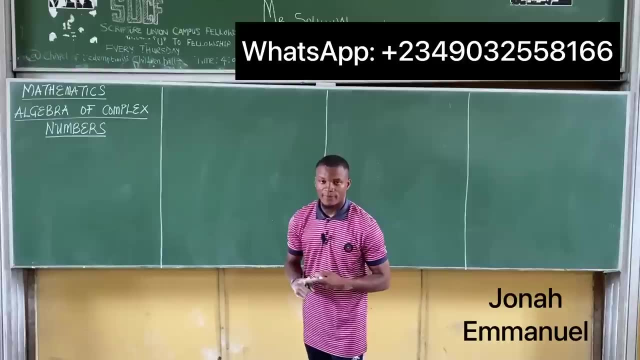 How do we multiply and how do we even divide complex numbers? Let's look at them in the algebra of complex numbers. Alright, so let's look at the algebra of complex numbers. For the algebra of complex numbers, we'll be considering the addition of complex numbers, the subtraction. 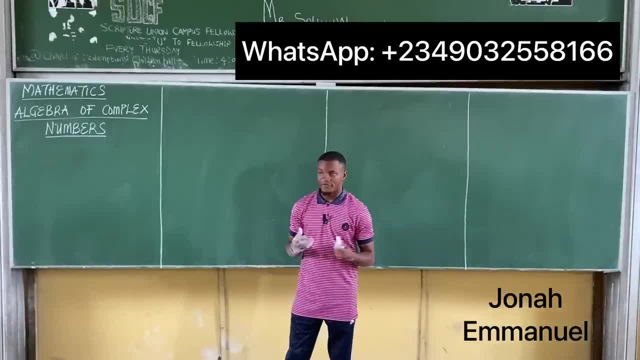 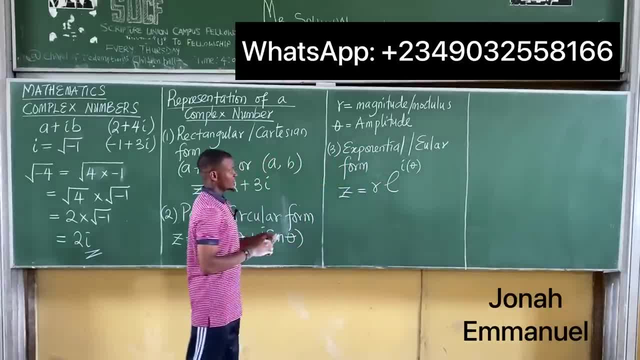 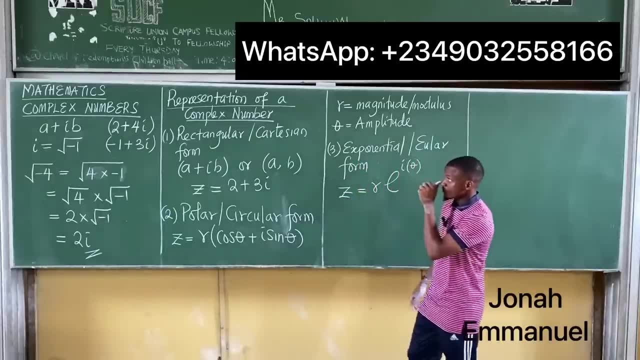 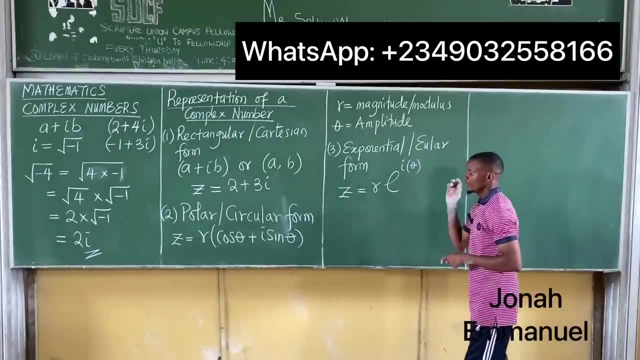 theta. Alright, so this is the Euler's form of representing complex numbers. So let's look at the second form of representing complex numbers. Alright, so we have a forms or pattern of representing complex numbers: Rectangular form or Cartesian, polar form or circular. 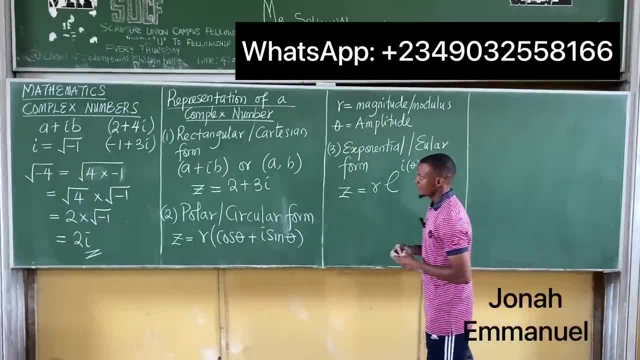 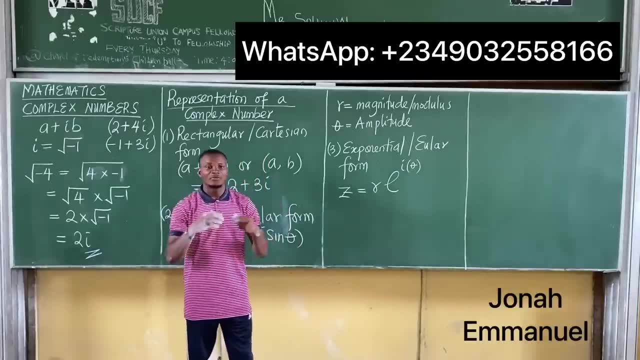 then exponential form or Euler's form. Next up, let's look at the algebra of complex numbers. How do we add complex numbers, How do we subtract them, How do we multiply and how do we even divide complex numbers? Let's look at them in detail. 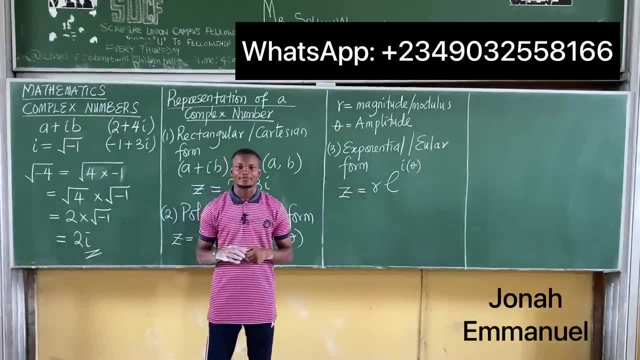 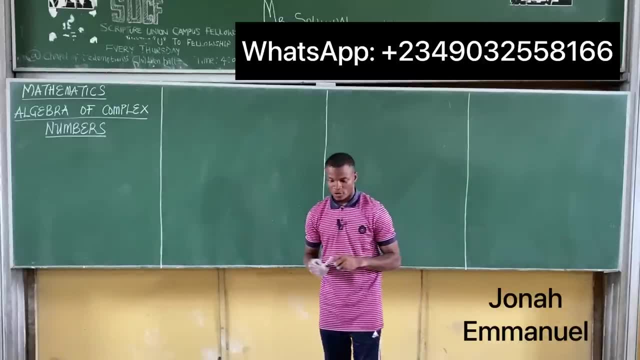 Let's look at the algebra of complex numbers. Alright, so let's look at the algebra of complex numbers. For the algebra of complex numbers, we'll be considering the addition of complex numbers, the subtraction of complex numbers, the multiplication of complex numbers and. 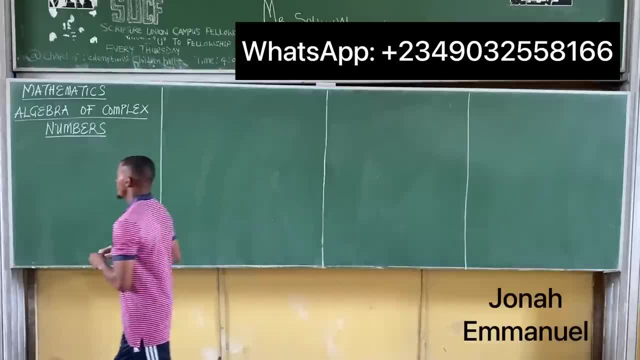 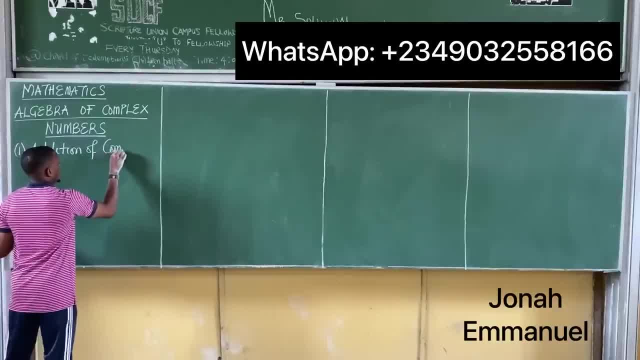 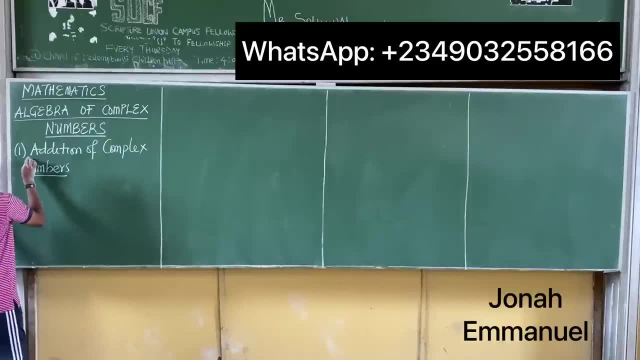 numbers. Let's start with addition of complex numbers. Let's start with addition of complex numbers, complex numbers. all right, let's look at how to add complex numbers. given a complex number, let's give him two complex numbers. let's say: Z 1 has been equal to a 1 plus IB 1. 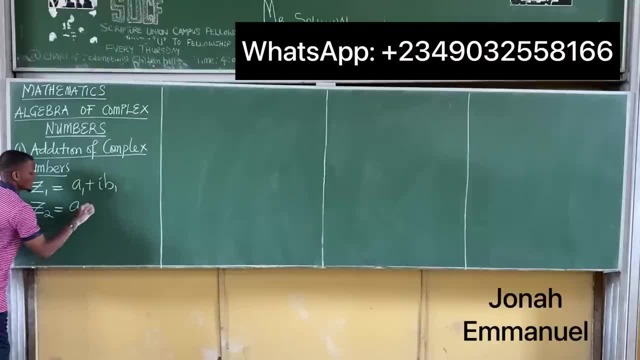 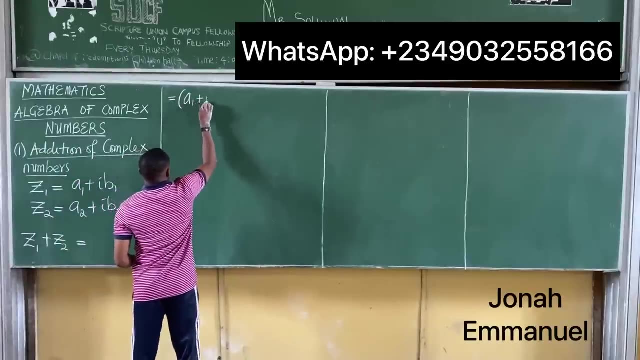 and Z 2 has been equal to a 2 plus IB 2. if a max will add them, that's find their sum. Z 1 plus Z 2 will be equal to. that will be equal to Z 1 is a 1 plus IB 1. 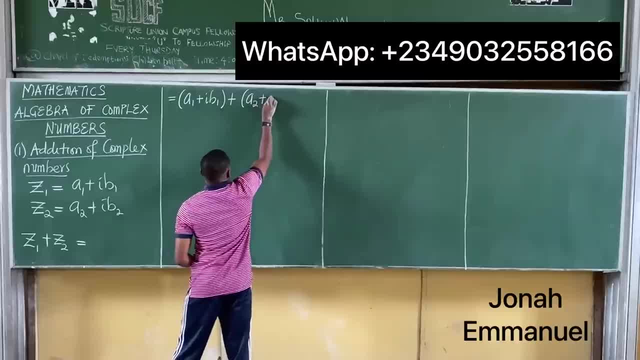 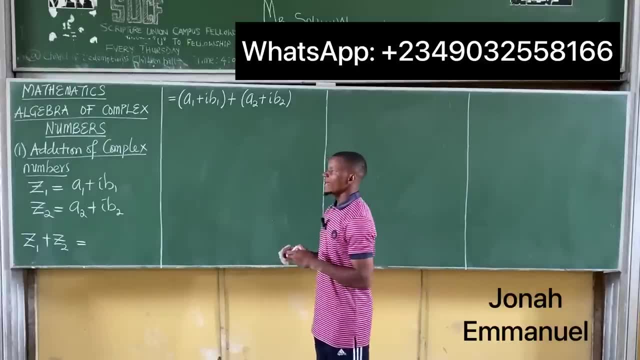 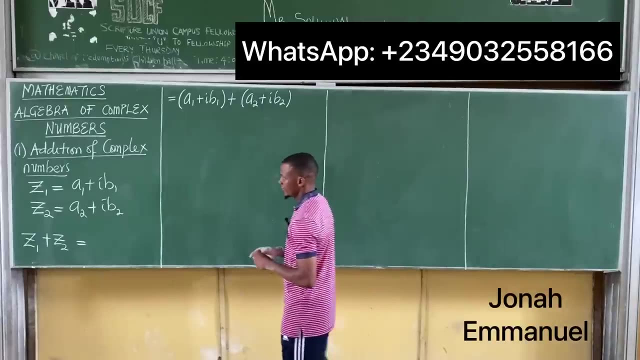 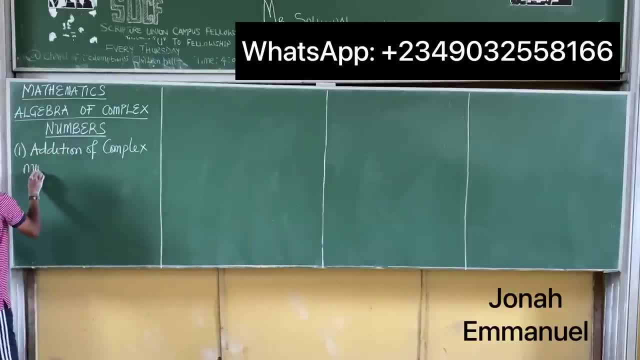 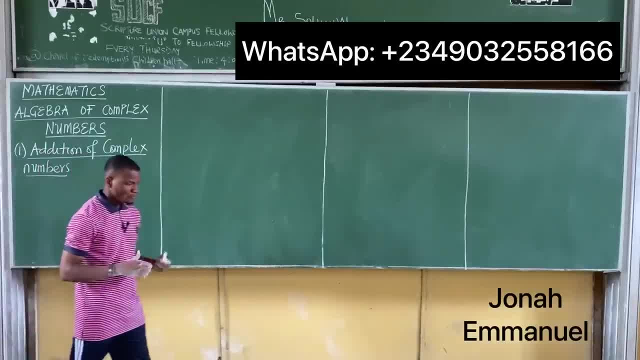 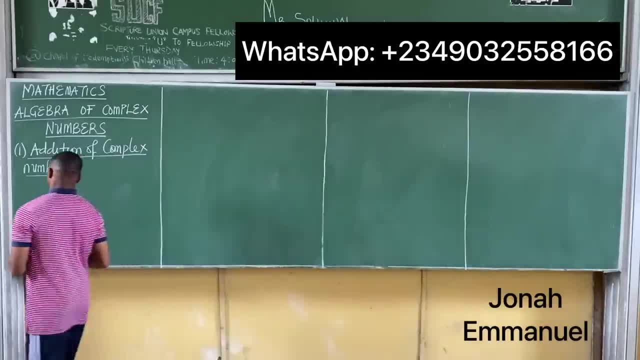 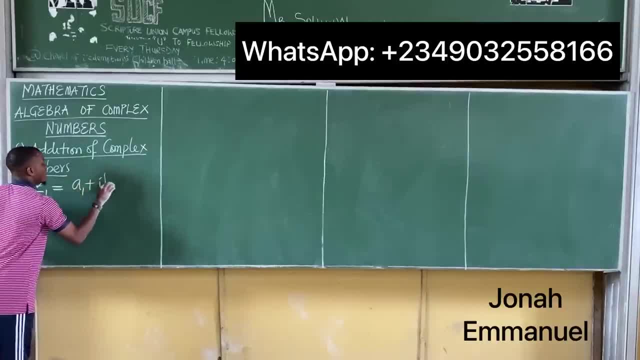 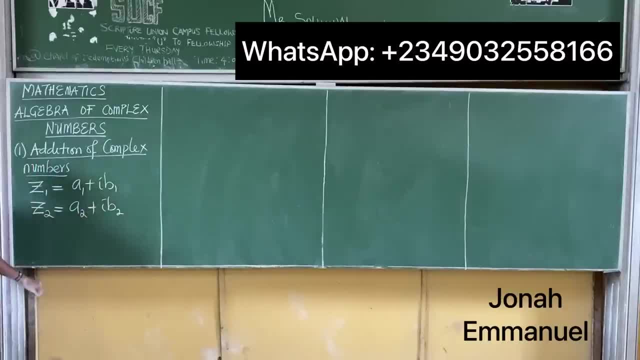 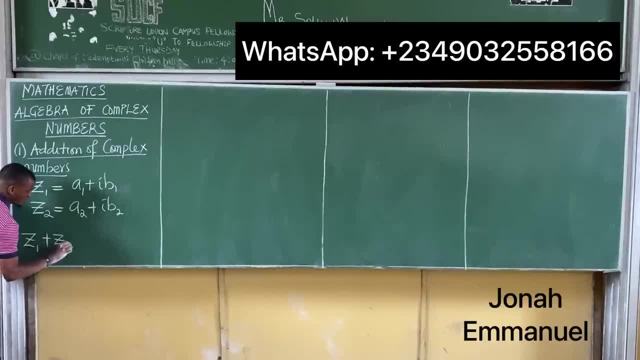 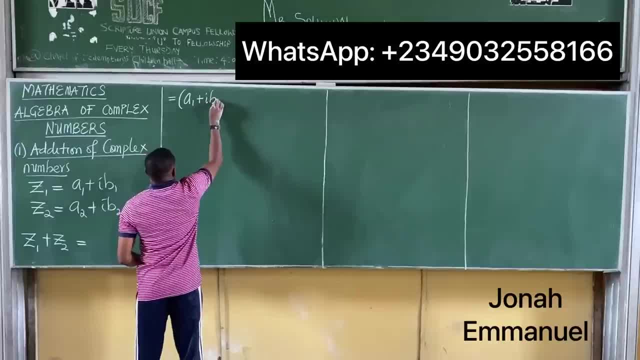 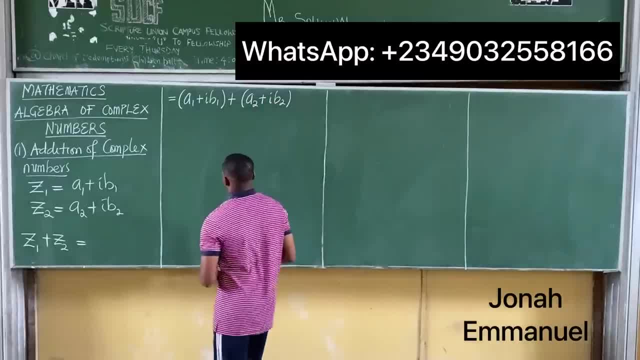 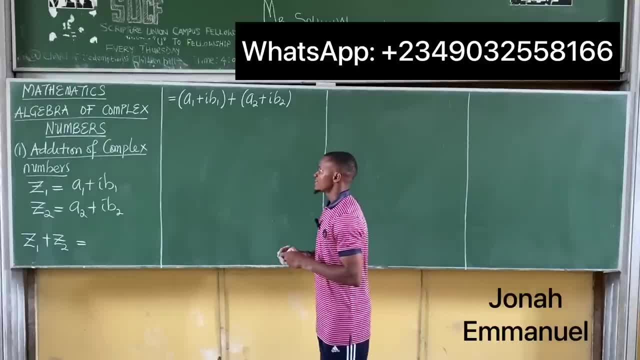 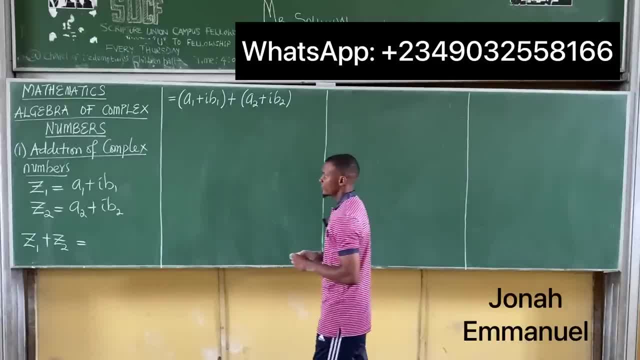 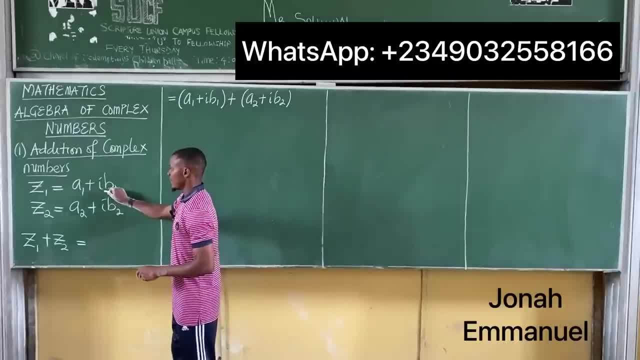 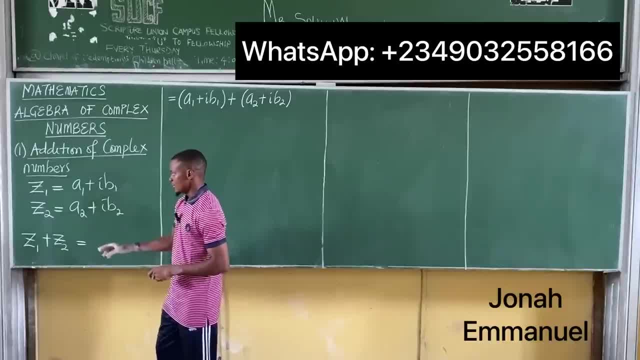 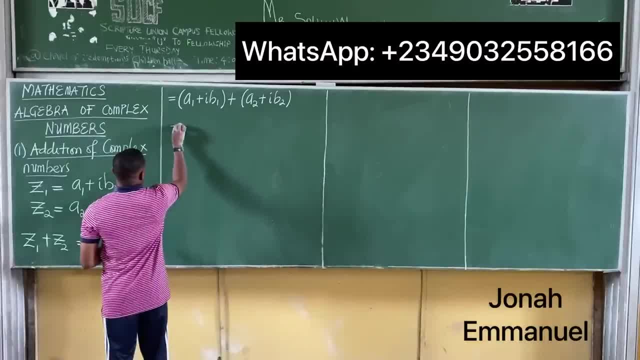 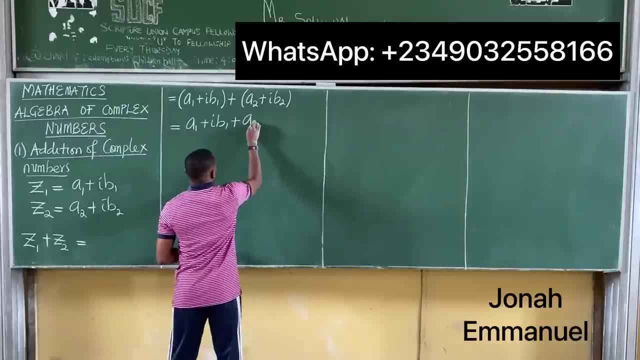 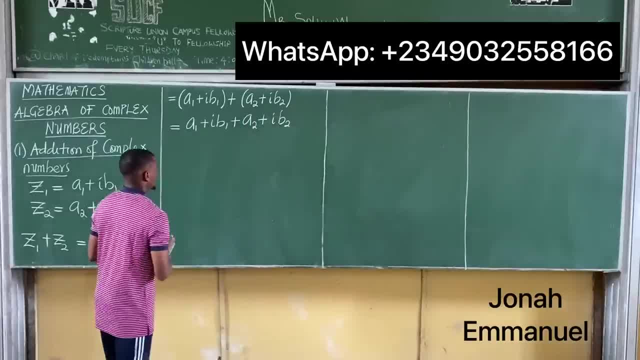 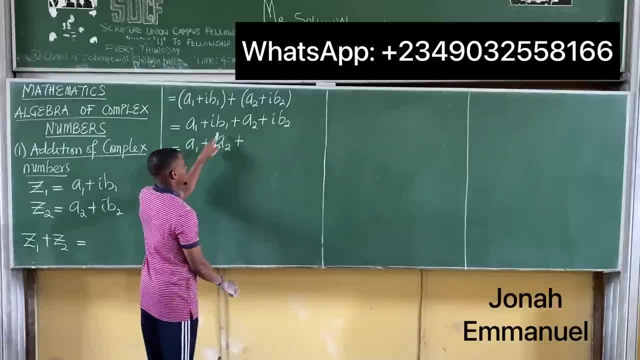 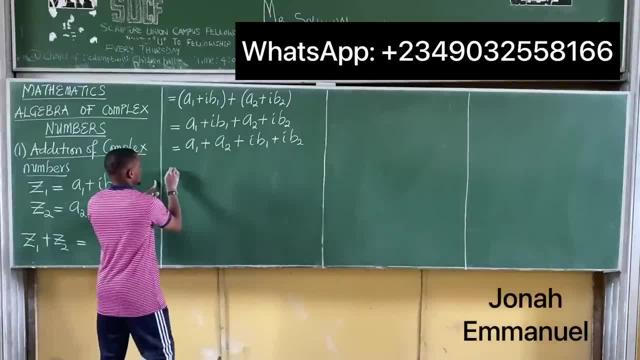 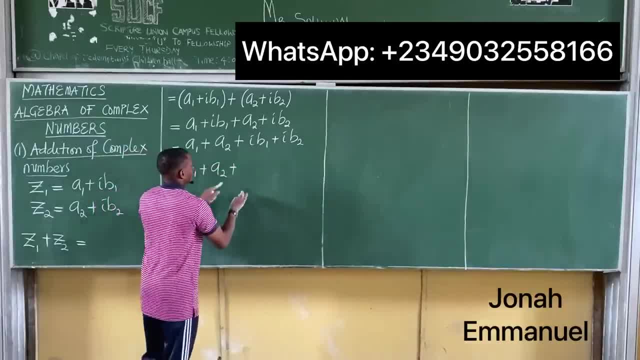 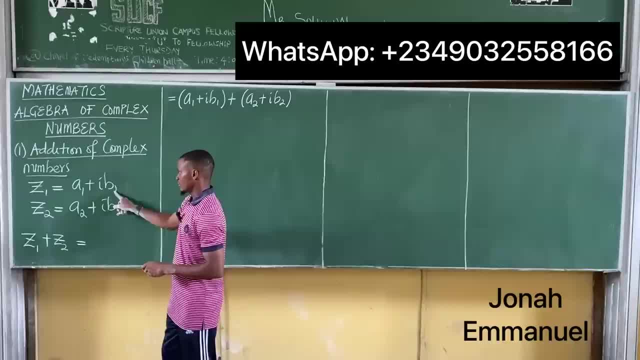 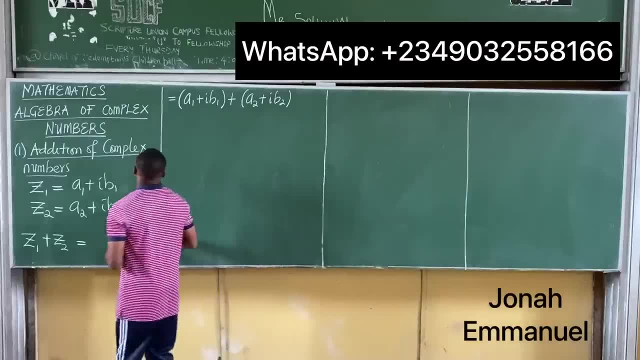 now the part with the I, that's IB, IB 1. that's it in Z 2. the real part is a 2, while the imaginary part is IB 2. so this will be equal to: if I take off brackets, becomes a 1 plus IB 1. 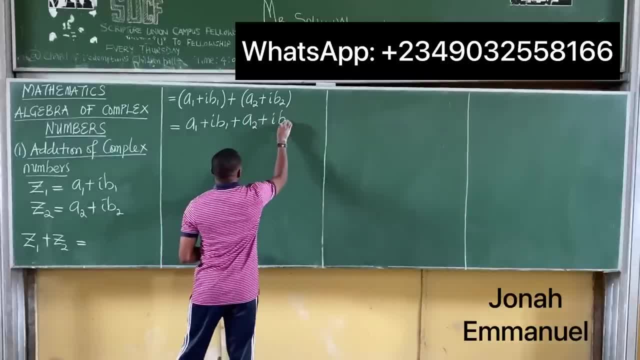 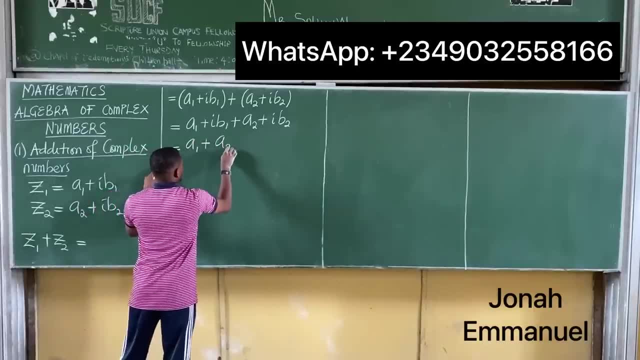 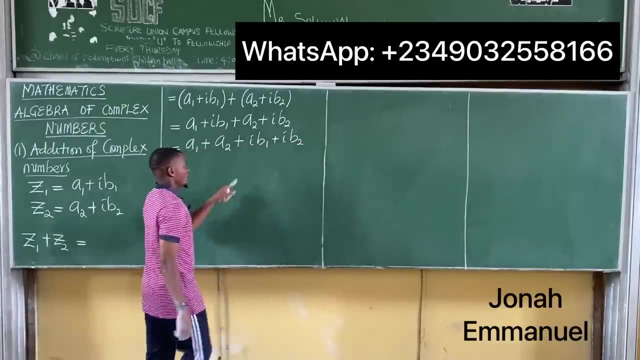 plus a 2 plus IB 2. take the real part, that's equal to a 1 plus this one here, a 2 plus. take the imaginary part, IB 1 plus IB 2. let's factorize the I's, this will be equal to a 1 plus a 2 plus. if I factorize, I am left with B 1 plus B 2. I. 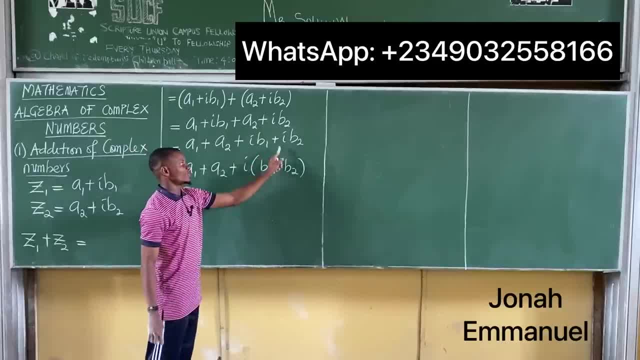 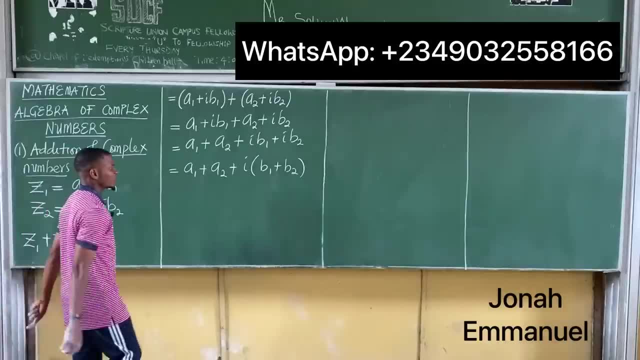 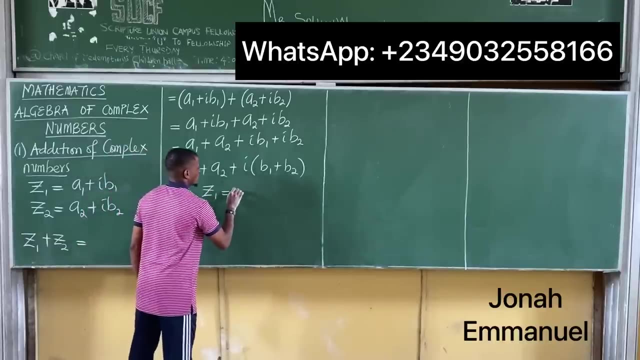 times b1 i b1. i times b2 i b2. all right, so this is how we add or this is how we take the sum of complex numbers. let's take a quick example. so let's say a simple example. let's say z1 is equal to minus 3 plus 2i and z2 is equal to minus 1 minus i. we'll have that z1 plus z2. 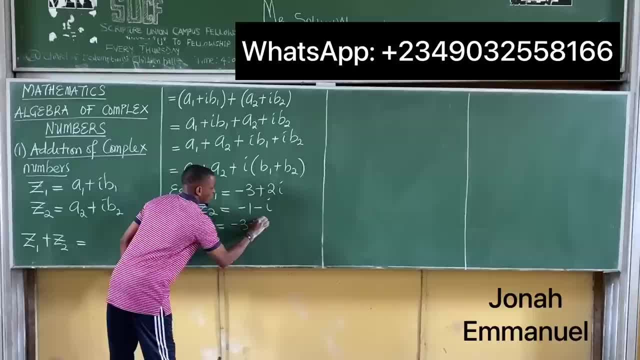 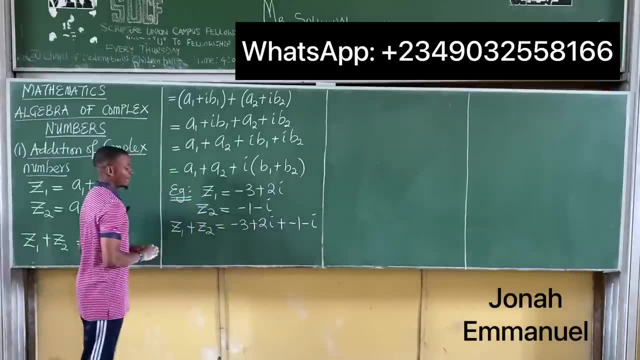 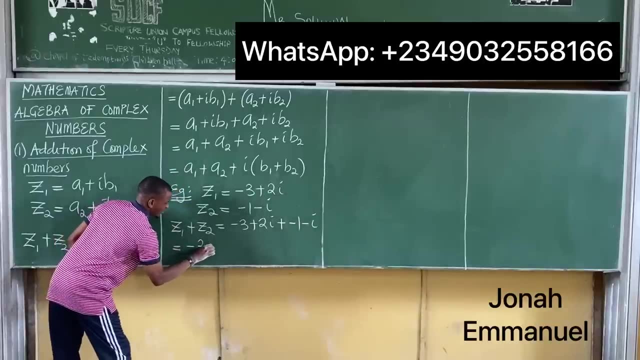 is equal to this: z1 is minus 3 plus 2i plus z2 is minus 1 minus i. if i take out my real parts, i'm having minus 3 plus minus is minus. so minus 3 minus 1. if i take out imaginary parts, i'm having 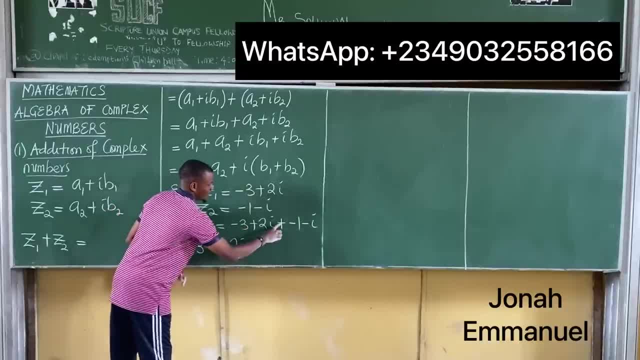 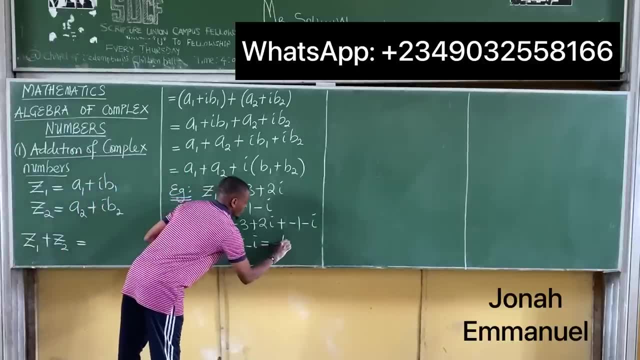 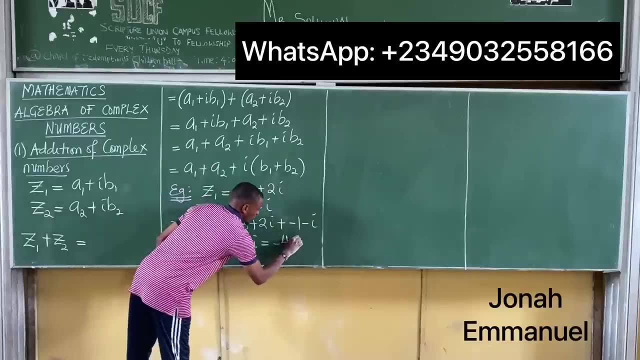 plus 2i. that's plus 2i. plus minus is minus i. if i work on this, minus 3 minus 1 is minus 4, plus 2 minus 1. so 2 minus 1 is 1. that's a positive 1. so plus i. so my answer: 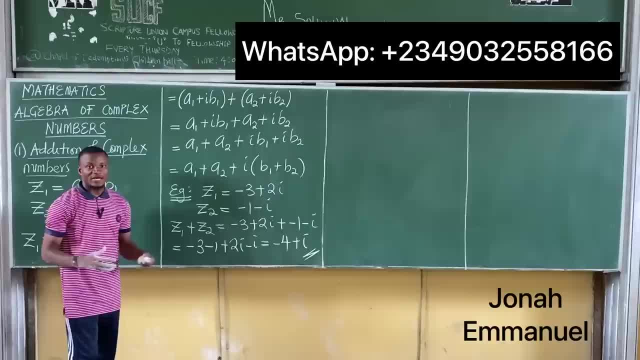 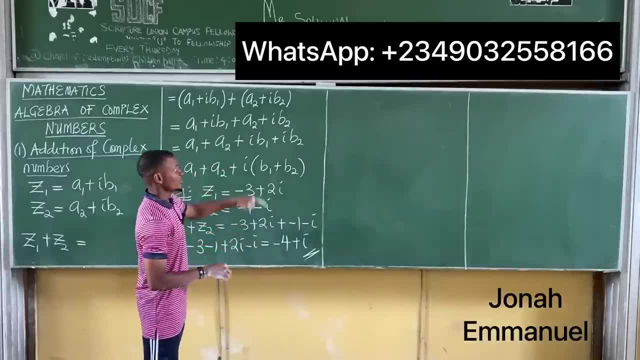 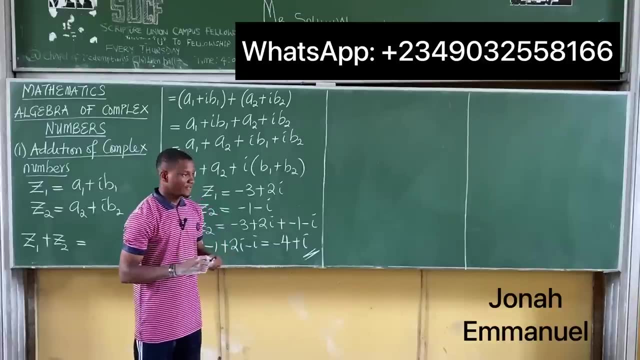 becomes minus 4 plus i. so this is how we add up complex numbers. at the end of this class i'll leave a link to show you how you can do the algebra of complex numbers using just your calculator. all right, we'll provide the link in the description of this video, but for now let's 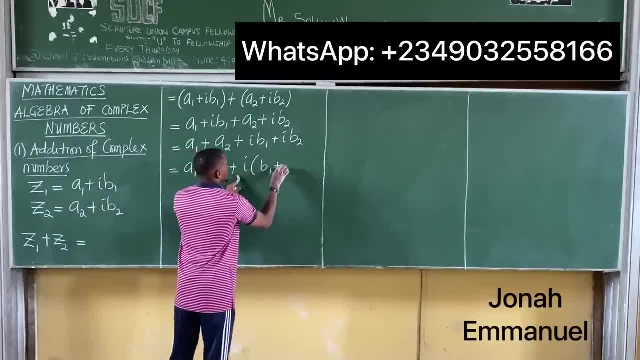 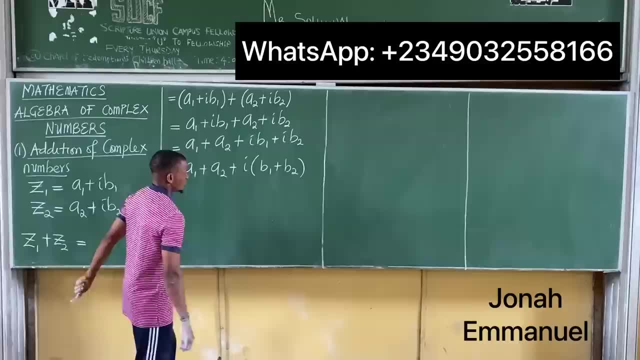 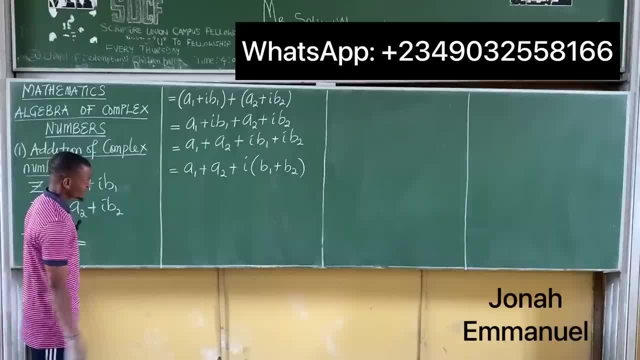 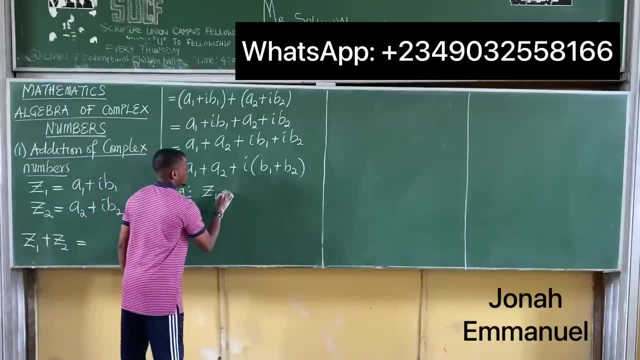 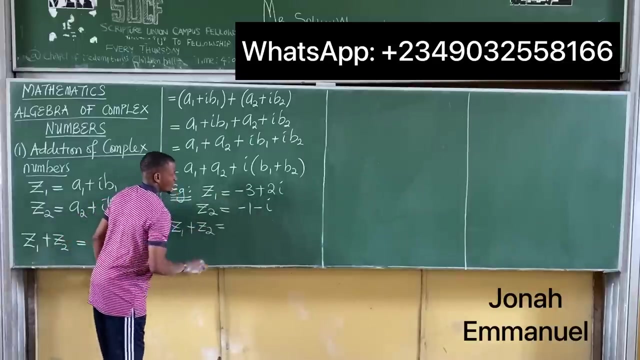 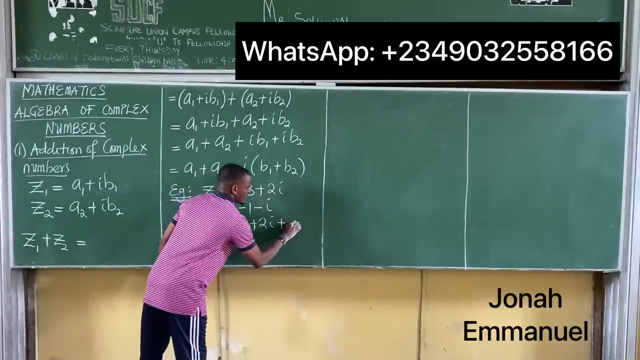 or this is how we take the sum of complex numbers. Let's take a quick example. So let's say a simple example. Let's say z1 is equal to minus 3 plus 2i and z2 is equal to minus 1 minus i. We have that z1 plus z2 is equal to this. z1 is minus 3 plus 2i plus z2 is 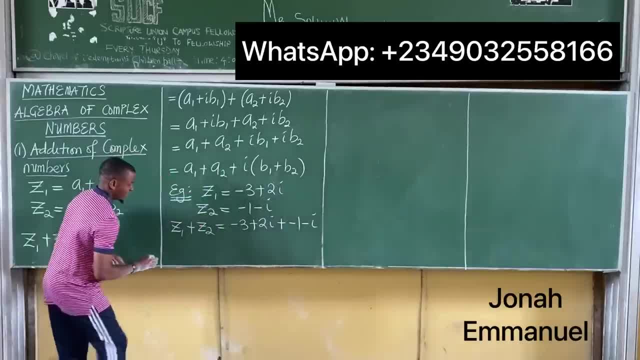 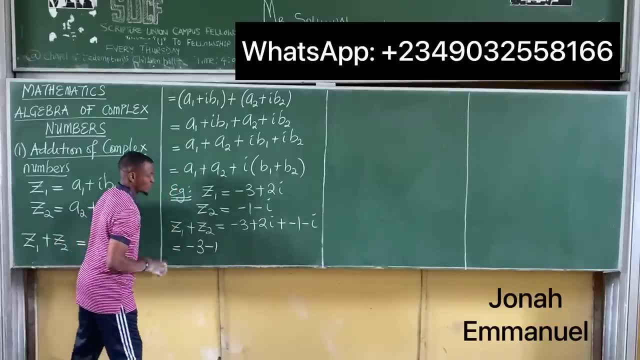 minus 1 minus i. If I take out my real parts, I'm having minus 3 plus minus is minus, so minus 3 minus 1.. If I take out imaginary parts, I'm having plus 2i, that's plus 2i. 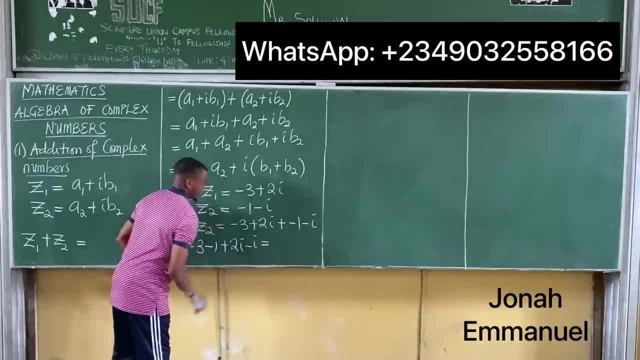 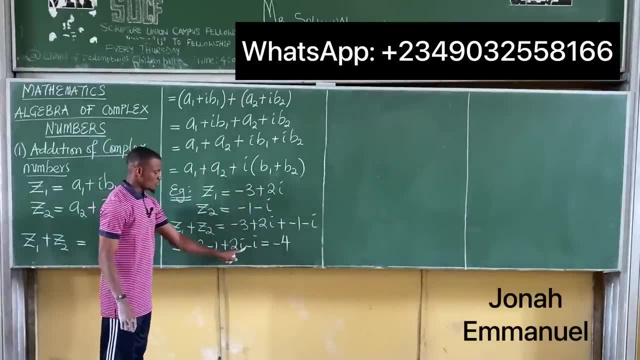 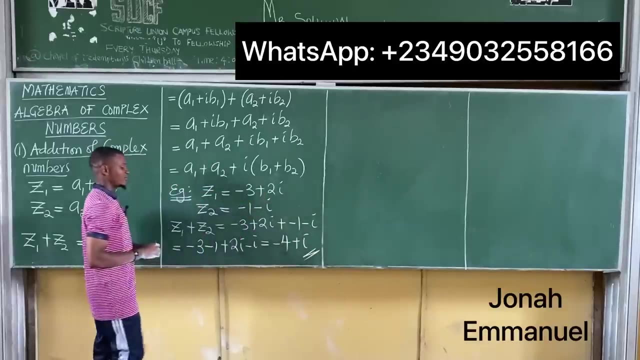 plus minus is minus i. If I work on this, minus 3 minus 1 is minus 4, plus 2 minus 1, so 2 minus 1 is 1, that's a positive 1, so plus i. So my answer becomes minus 4, plus. 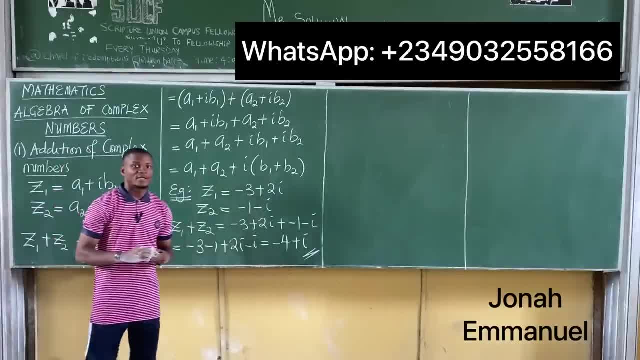 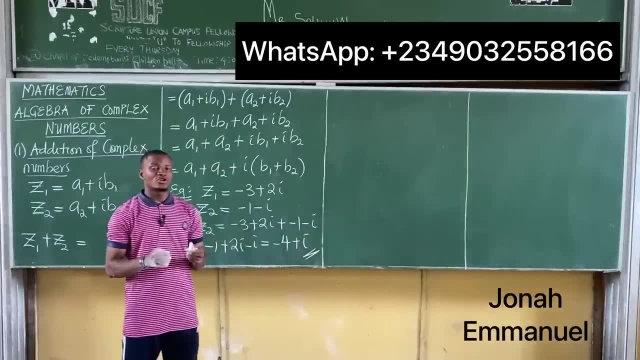 i, So this is how we add up complex numbers. At the end of this class, I'll leave a link to show you how you can do the algebra of complex numbers using just your complex numbers calculator. alright, We'll provide the link in the description of this video, But for 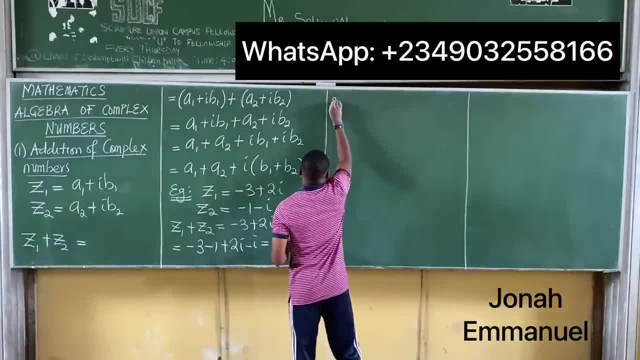 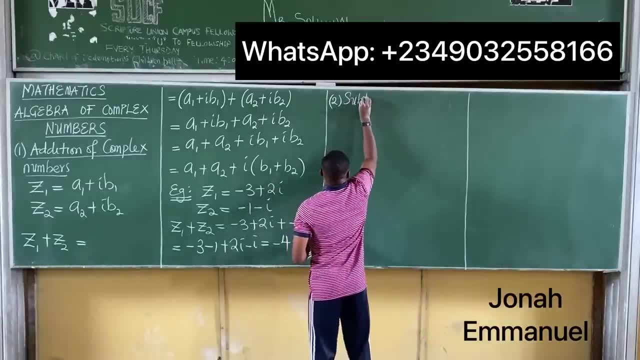 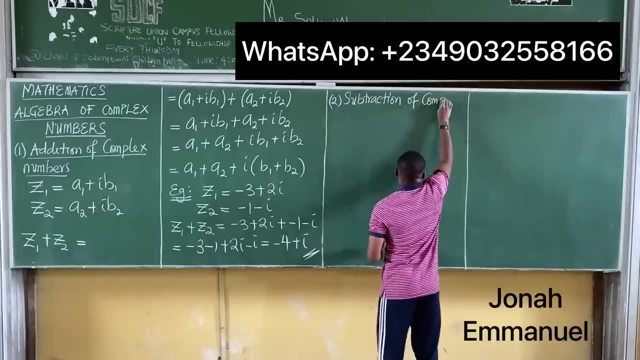 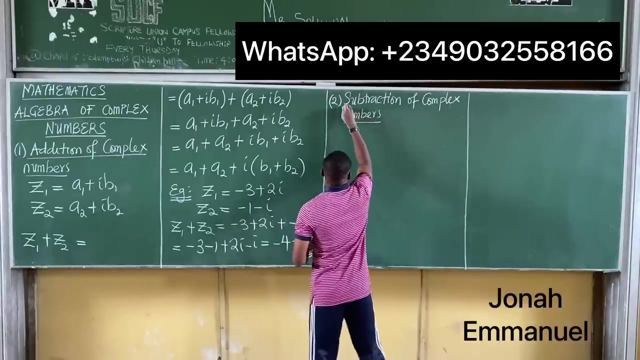 now let's proceed with this. Let's look at the second algebra of complex numbers, which is the subtraction. Let's look at subtraction: Subtraction of complex numbers. Let's look at the second algebra of complex numbers: Subtraction of complex numbers. Alright, 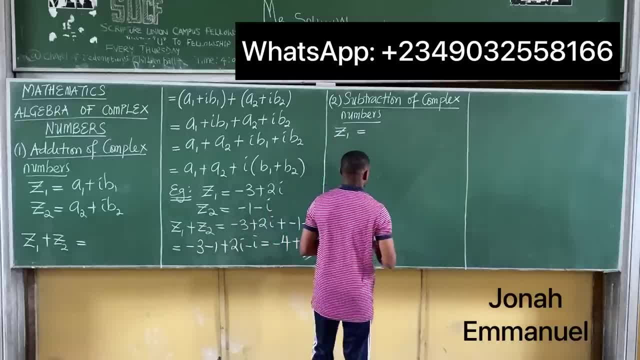 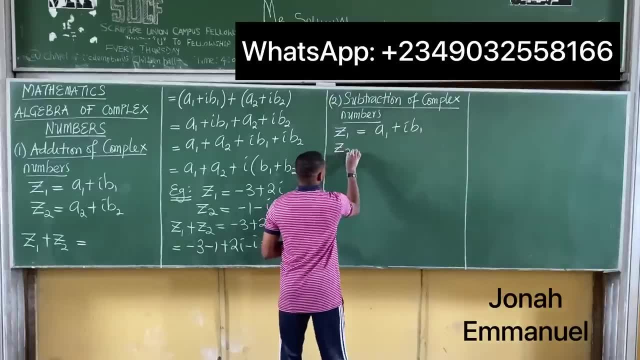 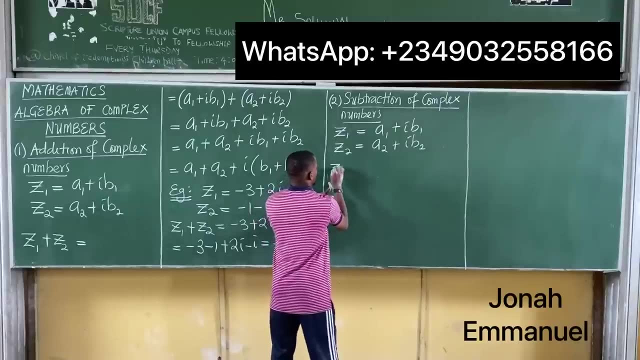 let's have z1 as being equal to a1 plus ib1, and z2, same thing as being a2 plus ib2.. To subtract them it's as easy as z1 minus z2, which will be equal to um. that will be equal. 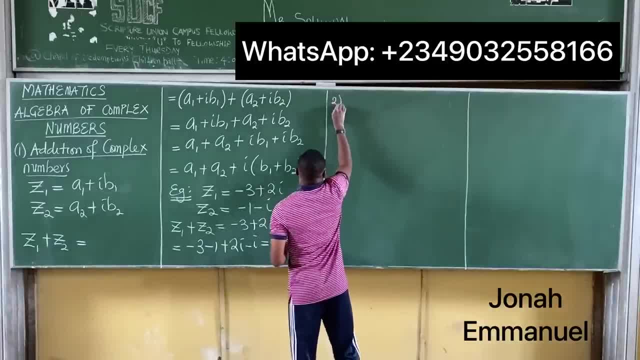 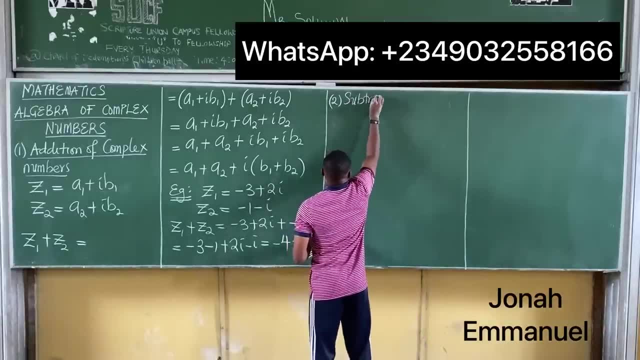 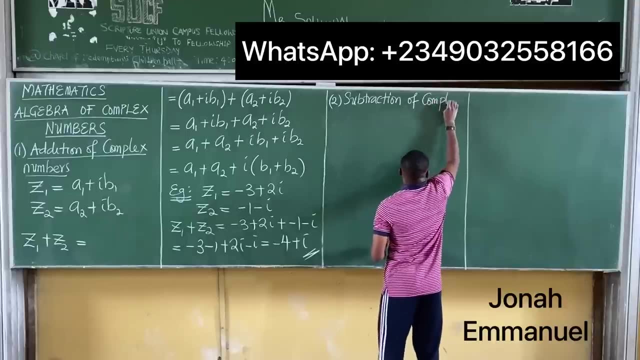 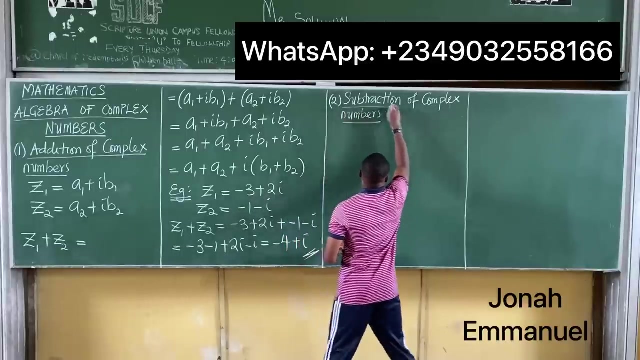 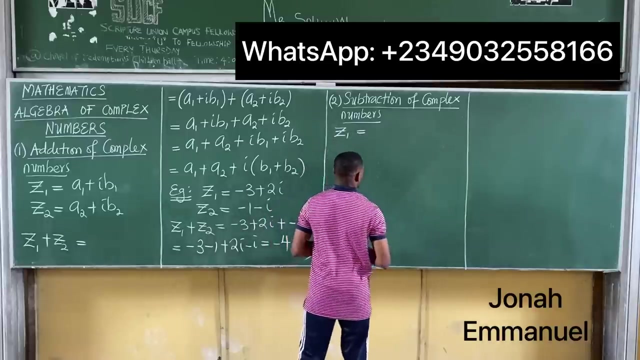 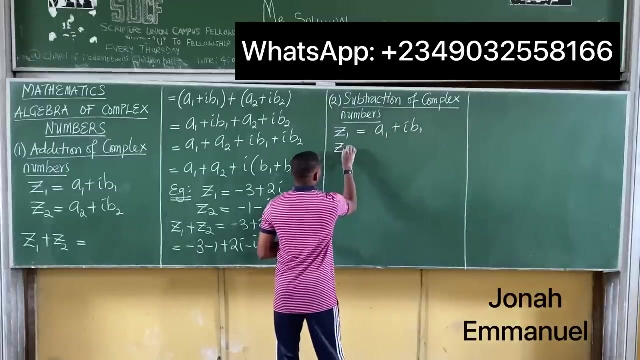 proceed with this. let's look at the second algebra of complex numbers, which is a subtraction. let's look at subtraction, subtraction of complex numbers, subtraction of complex numbers. all right, let's have z1 as being equal to a1 plus i, b1 and z2 same thing as being a2 plus i- b2. to subtract them, it's as: 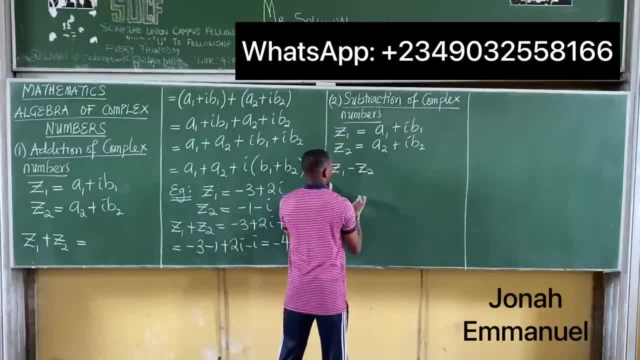 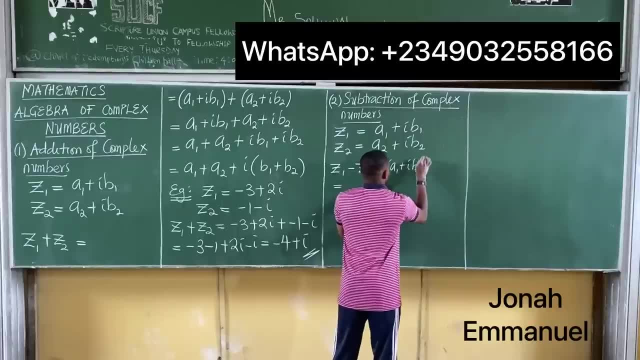 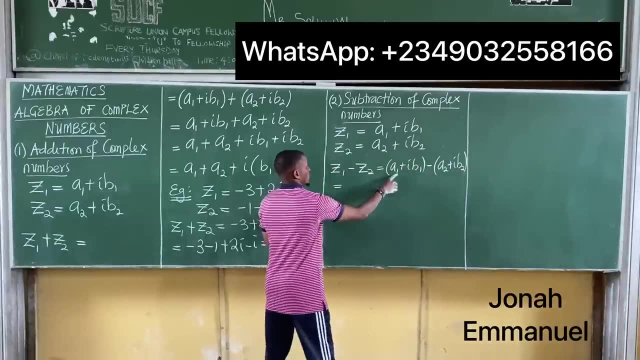 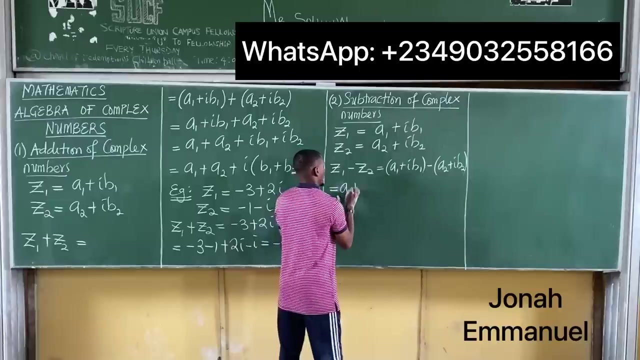 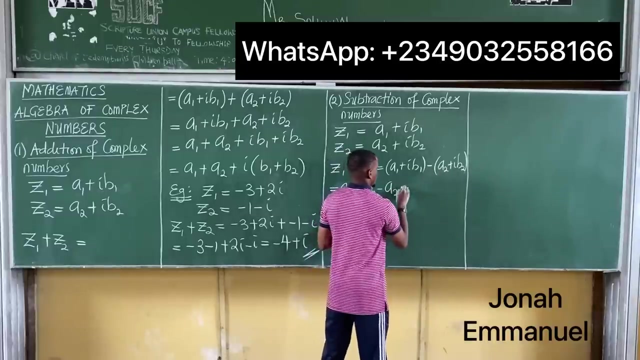 easy as z1 minus z2, which will be equal to um. that'll be equal to z1 a1 plus i b1 minus a2 plus i b2. all right, that's z1 minus z2. if i expand brackets, i have here as a1 plus i b1 minus. this is minus a2 minus plus minus i b2. so we have this. 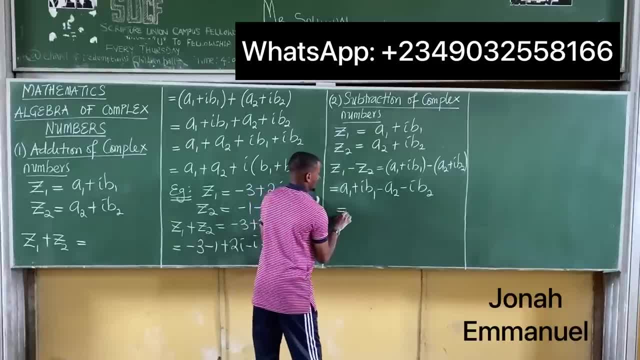 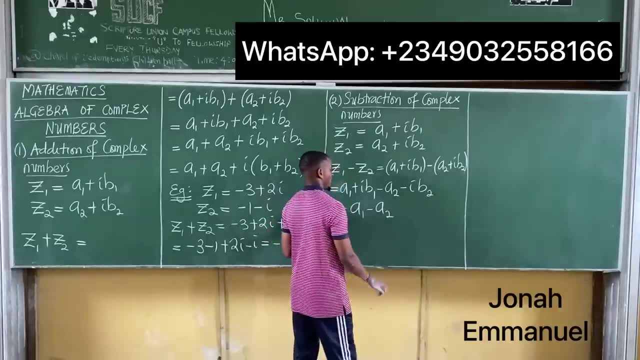 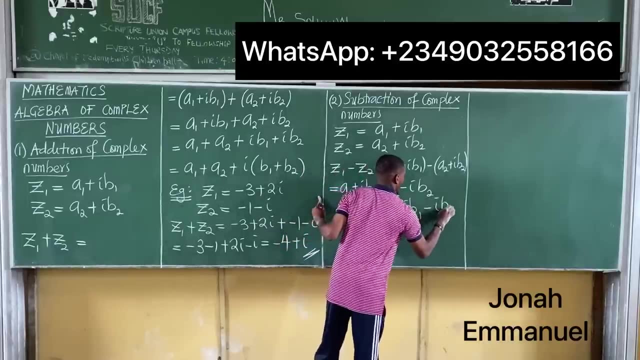 all right, let's collect the real parts, which is a1 and minus a2, so i'm having a1 minus a2. take the imaginary part which is plus i b1, so plus i b1, then this one here, minus i b2. finally, let's 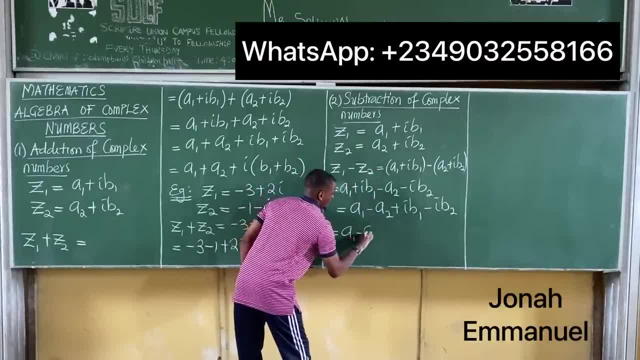 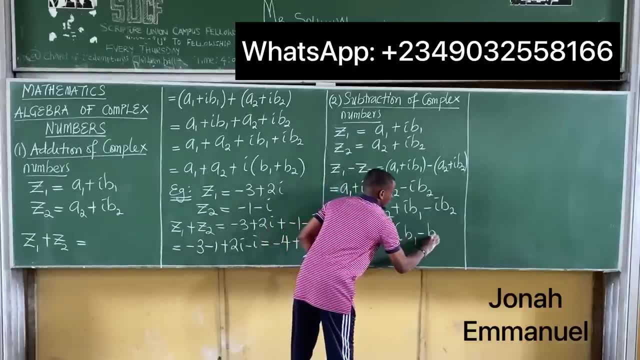 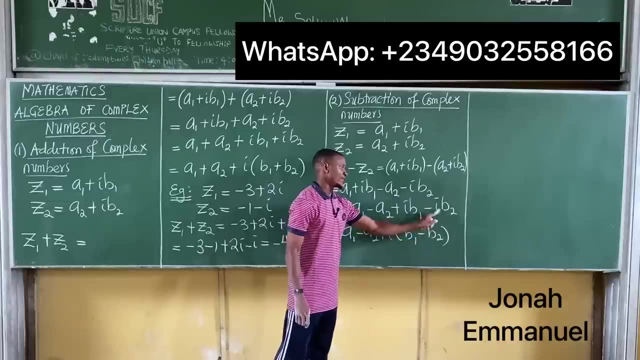 factorize that's equal to a1 minus a2, plus take out the i's plus i, i have b1 minus b2. i times b1, i b1, i times minus b2 minus i b2. so i have this: um, let's go ahead and go ahead and do this. 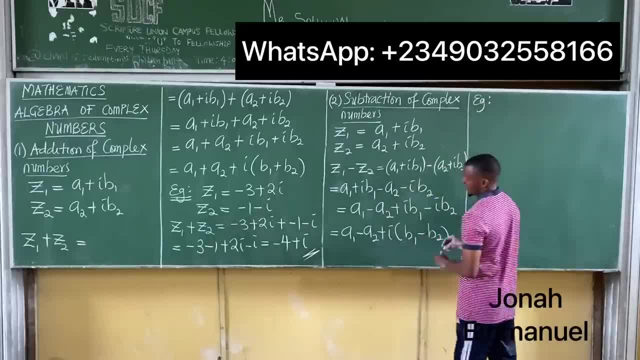 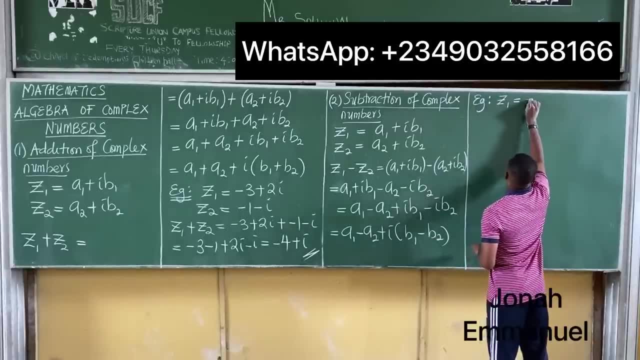 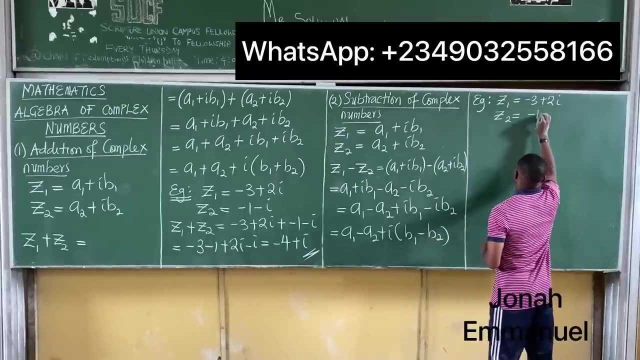 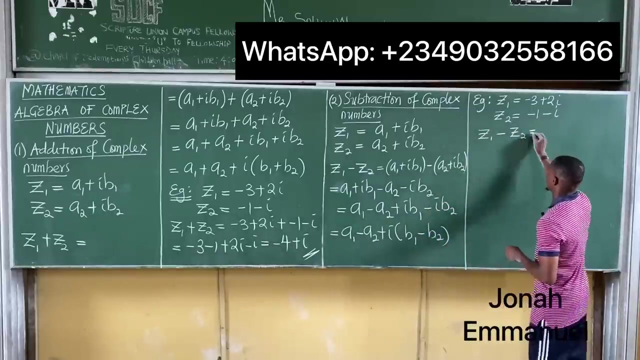 example, example um. perhaps let's take the same example. the same example as saying z1 should be equal to minus 3 plus 2i and z2 should be equal to minus 1 minus i. let's find z1 minus z2. that's equal to z1 is minus 3 plus 2i. 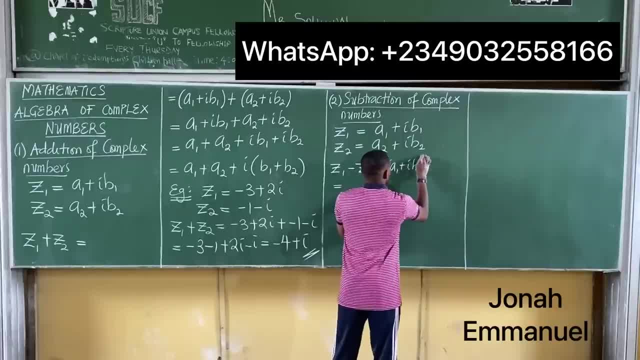 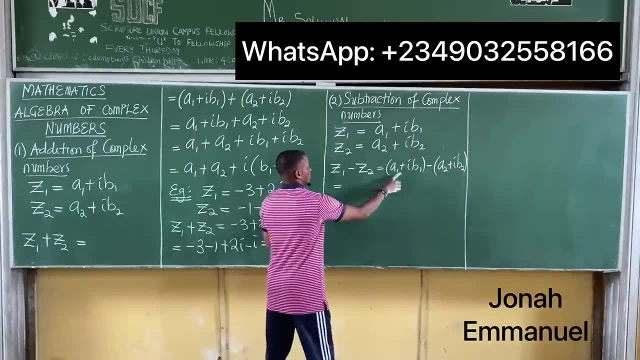 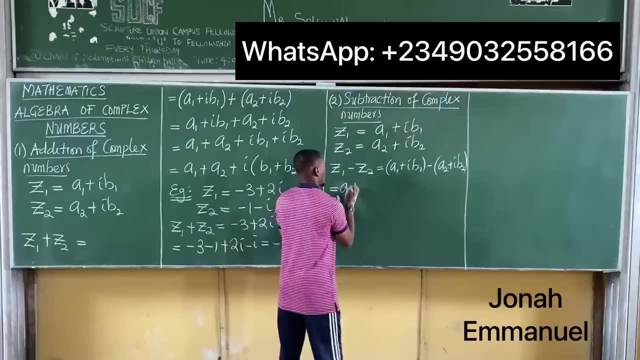 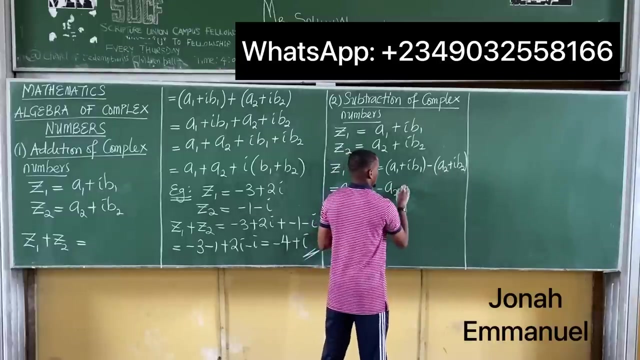 to z1, a1 plus ib2.. i b1 minus a2 plus i b2. all right, that's z1 minus z2. if i expand brackets, i have here as a1 plus i b1 minus, this is minus a2 minus plus minus i b2. so we have this. 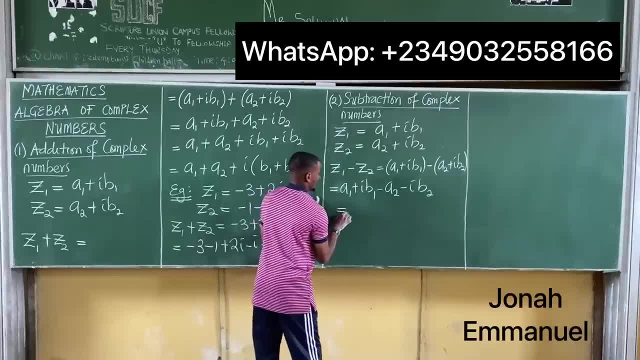 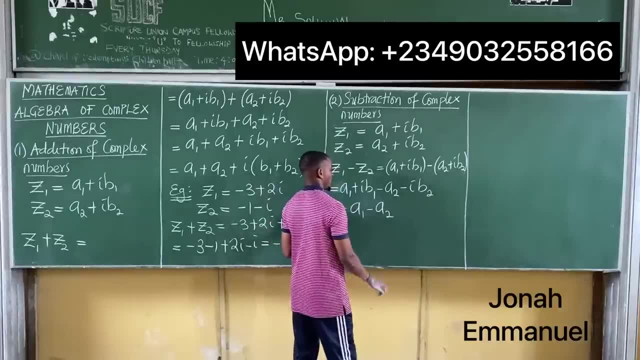 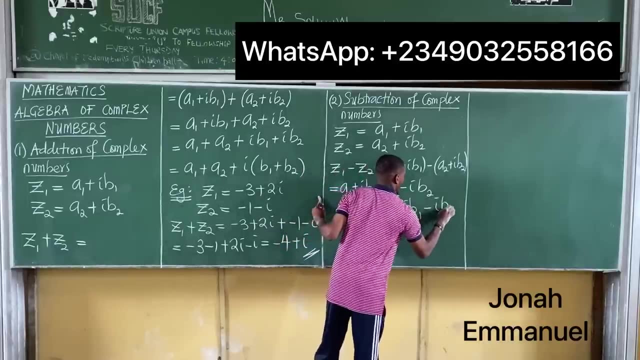 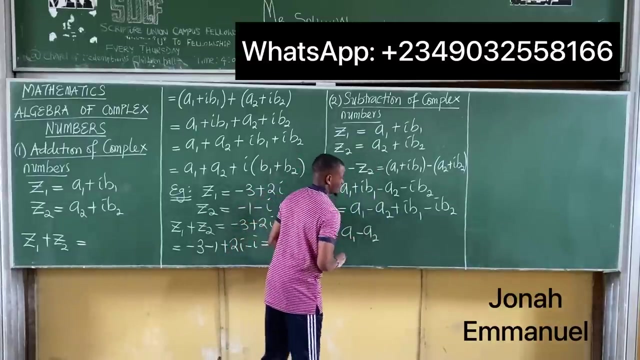 all right, let's collect the real parts, which is a1 and minus a2, so i'm having a1 minus a2. take the imaginary part which is plus i b1, so plus i b1, then this one here, minus i b2. finally, let's factorize that's equal to a1 minus a2, plus take out the i's plus i. i have. 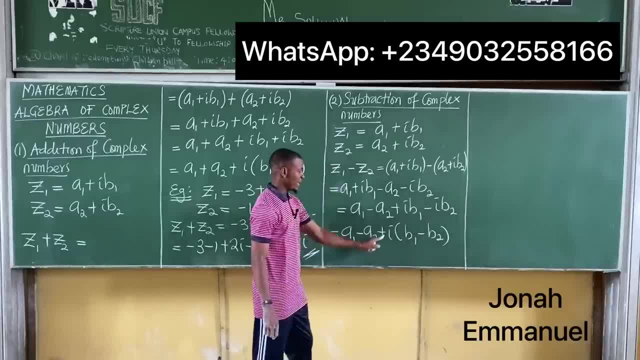 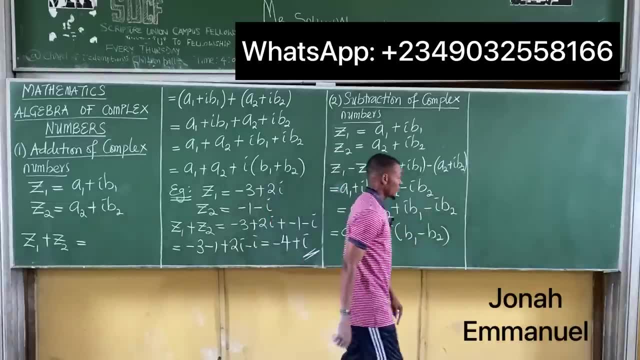 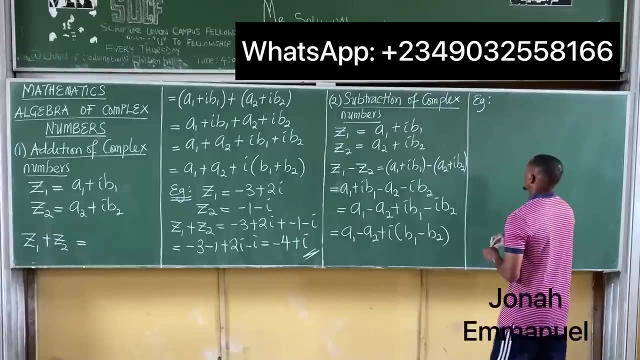 b1 minus b2. i times b1 i b1. i times minus b2 minus i b2. so i have this: um, let's take an example example, or perhaps let's take the same example, the same example as saying: z1 should be equal to. 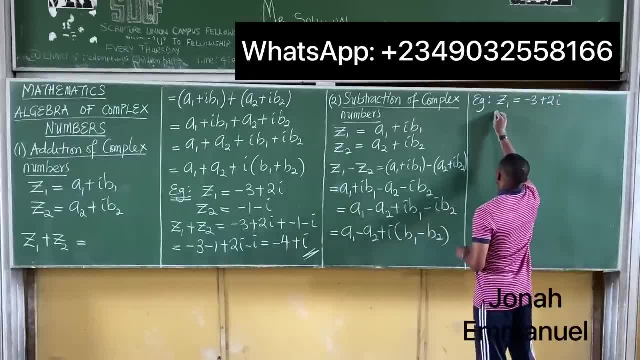 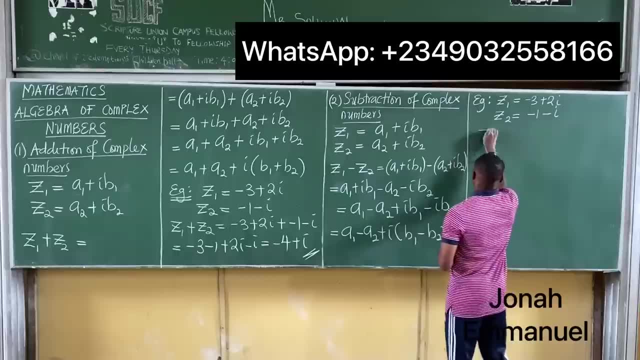 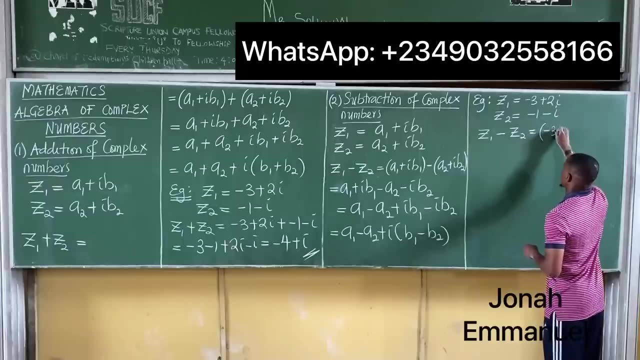 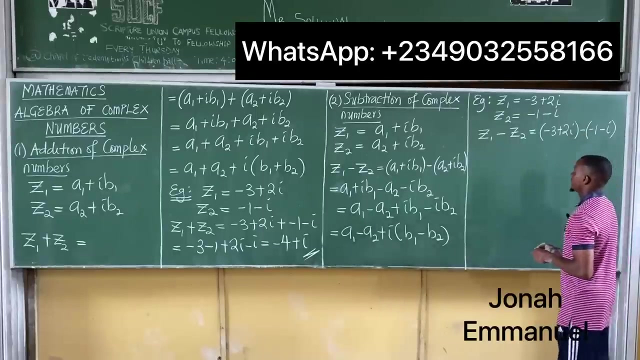 minus 3 plus 2 i, and z2 should be equal to minus 1 minus i. so let's find: z1 minus z2. that's equal to. z1 is minus 3 plus 2 i minus z2 is minus 1 minus i, so that's equal to: if i subtract this, this gives: 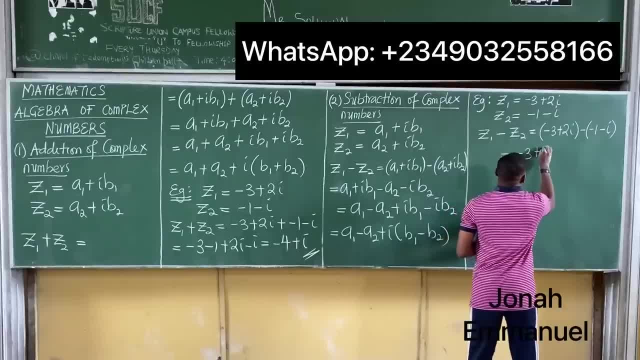 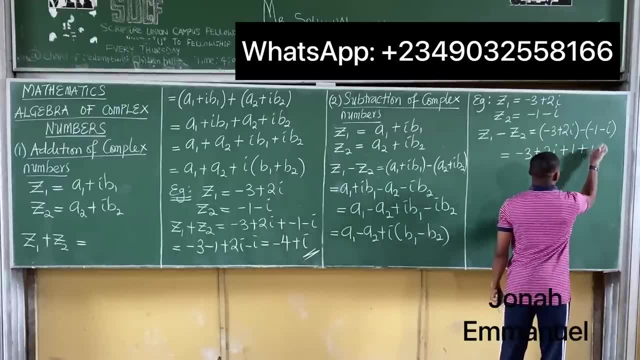 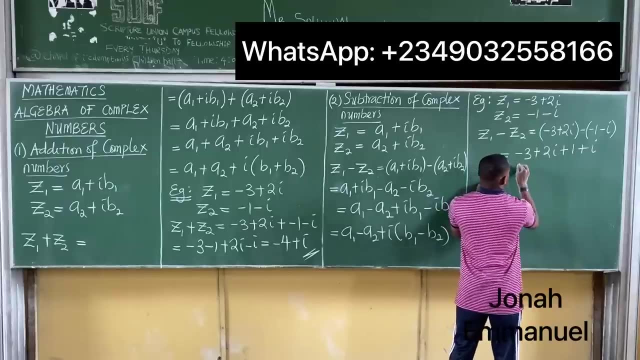 you. or if i expand the bracket gives you إ is equal to minus 3 plus 2 i. minus minus is plus 1, minus minus is plus i. next up, take the real parts and the imaginary parts. this is equal. for real parts, i have minus 3 and plus 1. for the imaginary part, i have plus 2 i. 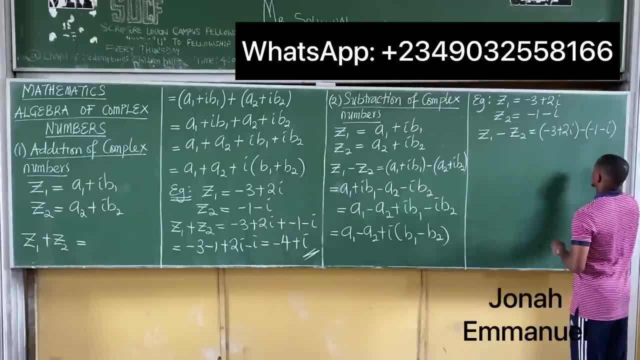 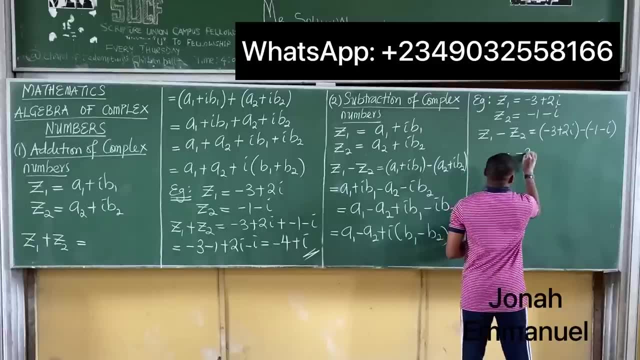 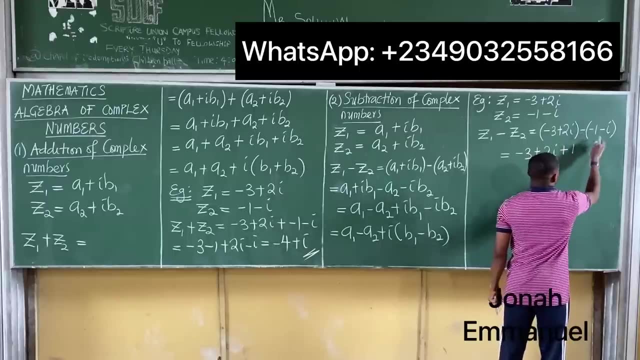 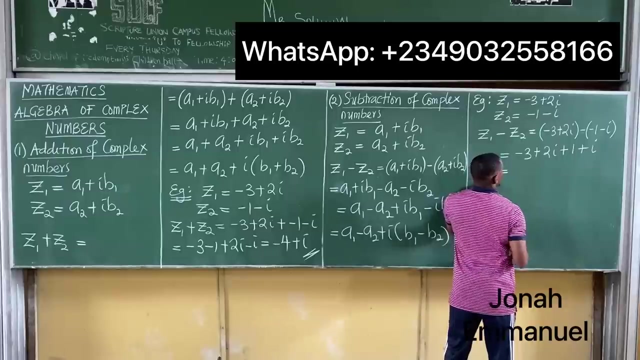 minus z2 is minus 1 minus i. so that's equal to: if i subtract this, this gives you, or if i expand bracket gives you minus 3 plus 2i. minus minus is plus 1, minus minus is plus i. next up, take the real parts and imaginary parts. this is equal. for real parts, i have minus 3 and plus 1. for the, 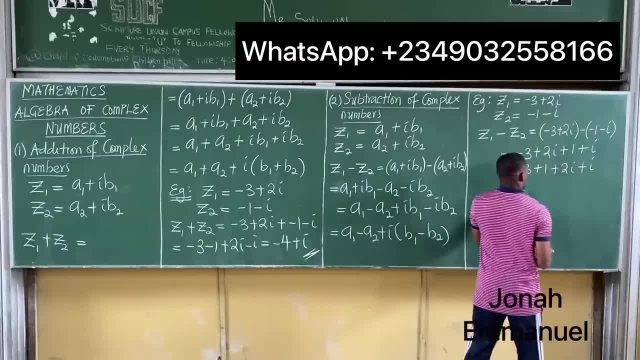 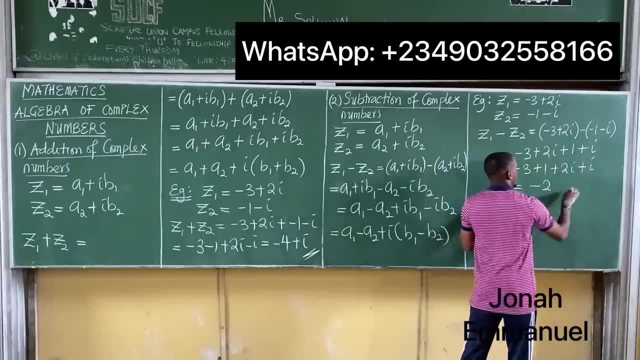 imaginary part. i have minus 3 and plus 1. minus minus is plus 1, minus minus is plus i minus minus. i have plus 2i plus i. this is equal to minus 3 plus 1 is minus 2, 2 plus 1 plus 3i. so that's your. 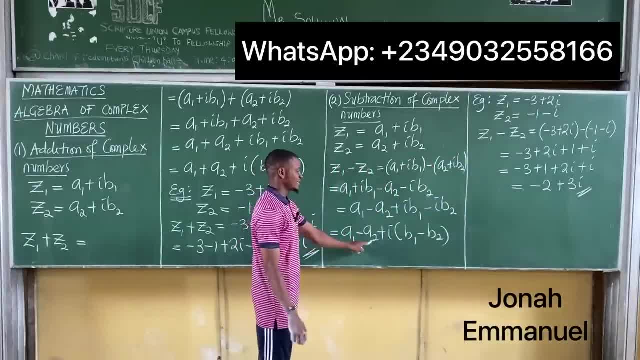 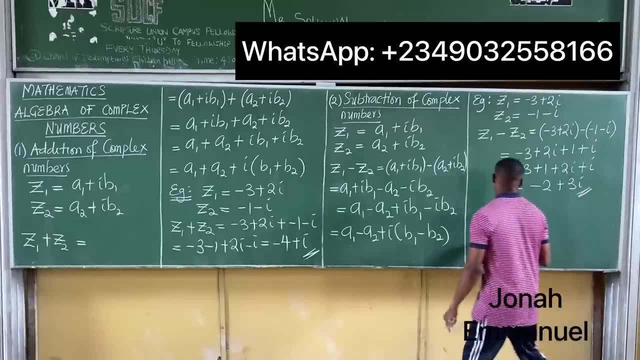 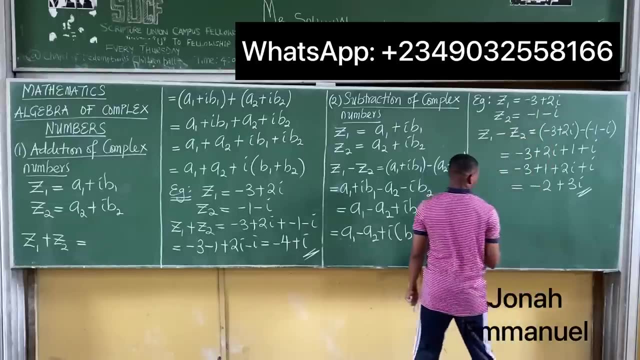 answer. we can still use the formula to get an answer if we want to. if we use the formula, this is equal. from the formula there we'll say that a1. compared to the formula here, this becomes a1, b1, b2. so if i use the formula- so, taking this one off a bit, let's try using the formula. so a1 will be. 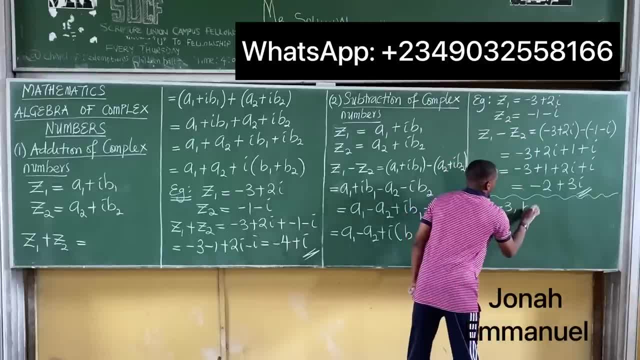 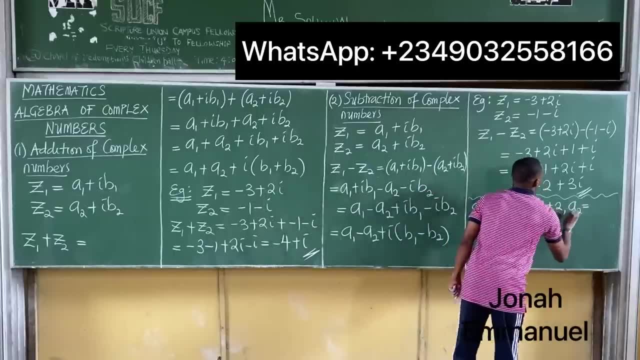 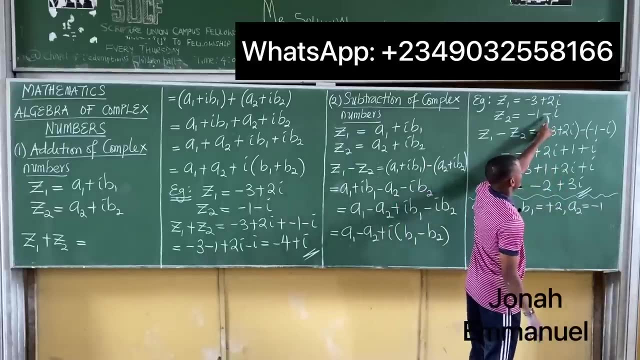 equal to this minus 3. b1 will be equal to this plus 2. a2 will be equal to this minus 1. also, b2 will be equal to coefficient of i here minus 1, that's minus 1. let's fix them to this formula. 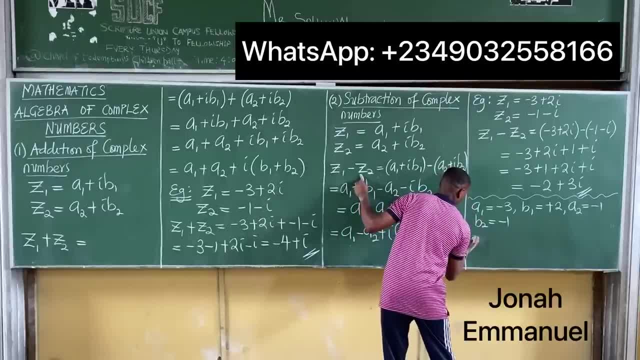 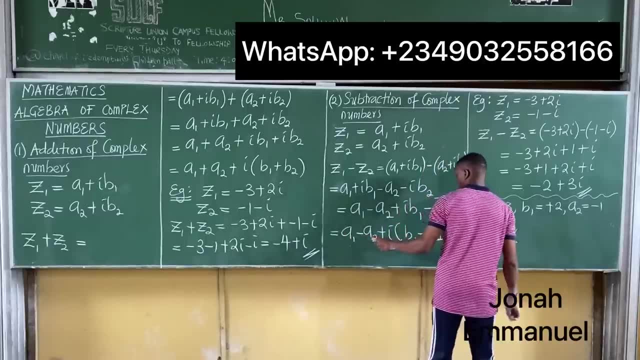 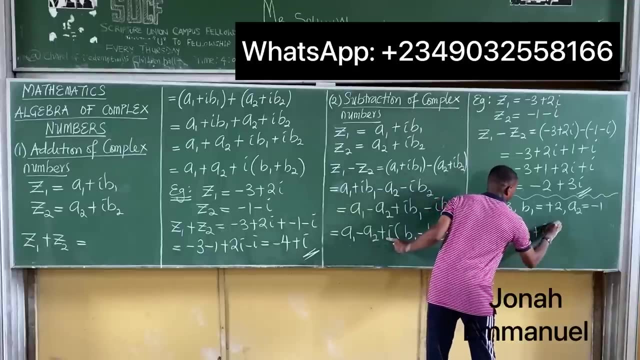 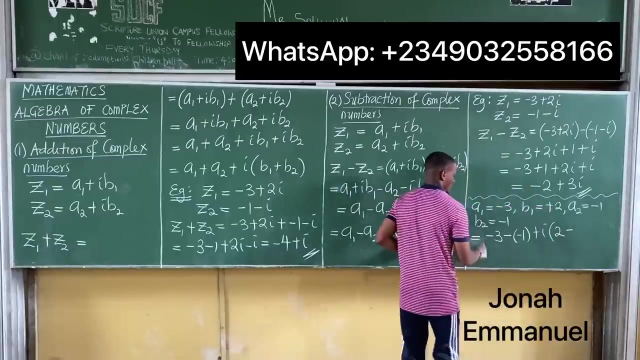 b1 minus, it will be equal to. will be equal to. we said a1, that's minus 3 minus a2. a2 is minus 1. okay, plus i into b1. b1 is plus 2 minus, so, minus b2, b2 is minus 1. if i work on this, this is equal to. 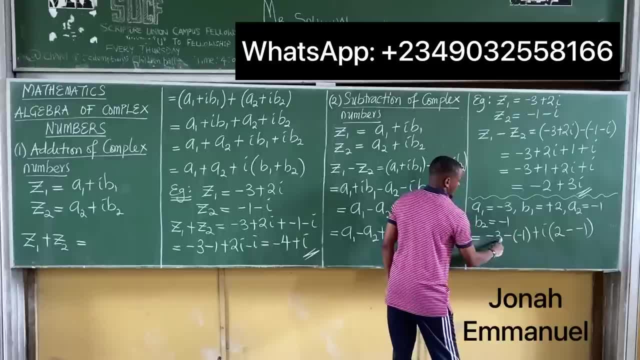 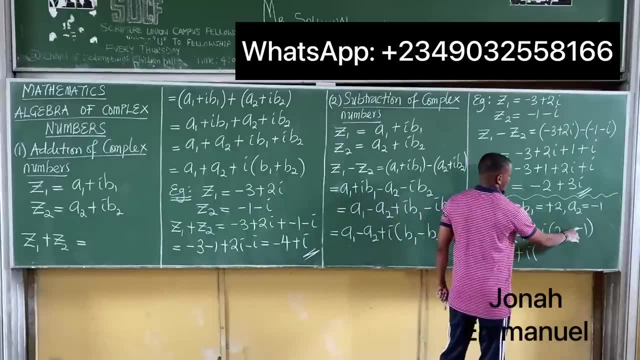 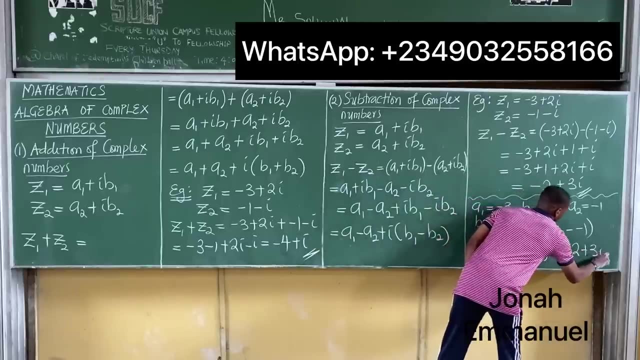 having minus 3 minus minus is plus minus 3 plus 1 is minus 2 plus i into 2 minus minus is plus 2 plus 1 is 3. so this will be equal to minus 2 plus 3i the same value, so you can choose to use. 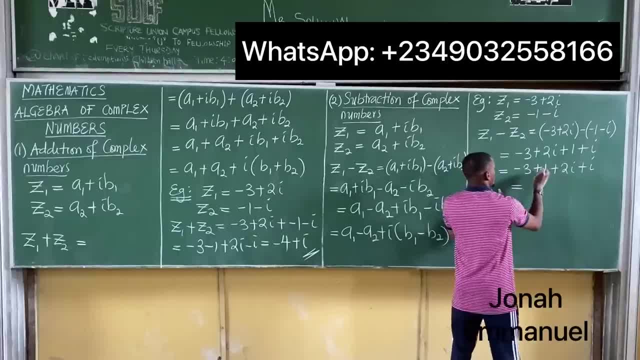 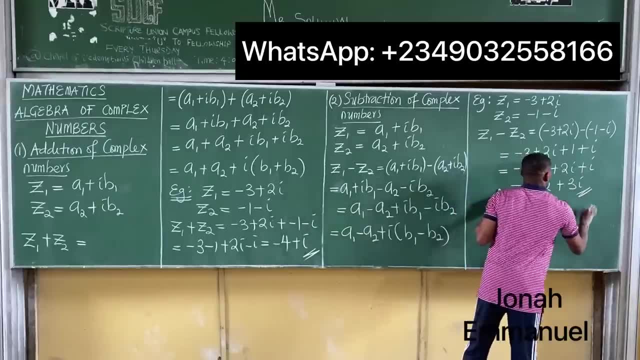 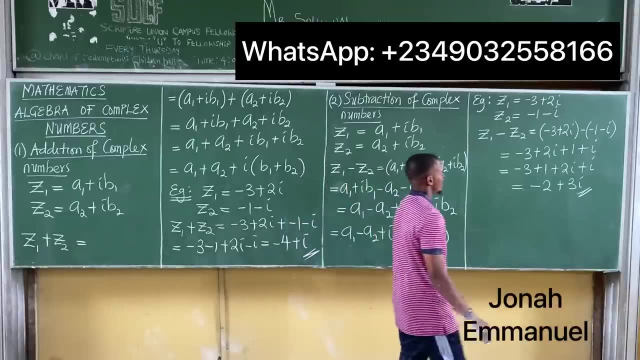 plus i. this is equal to minus 3 plus 1, is minus 2, 2 plus 1 i. we Intro plus 3i, so that's your answer. we can still use the formula to get an answer if we want to. if we use the formula, this is equal from the formula there. 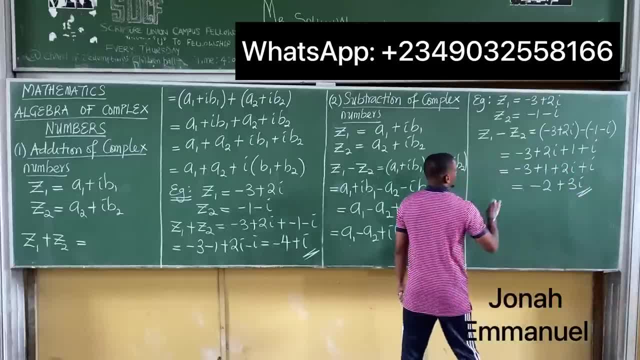 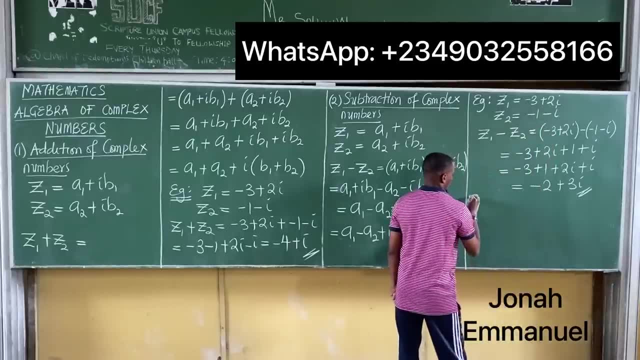 we'll say that a1,. compare this to the formula here. this becomes a1, b1, a2, b2. so if I use the formula- so taking this one off a bit, let's try using the formula. so a1 will be equal to this. 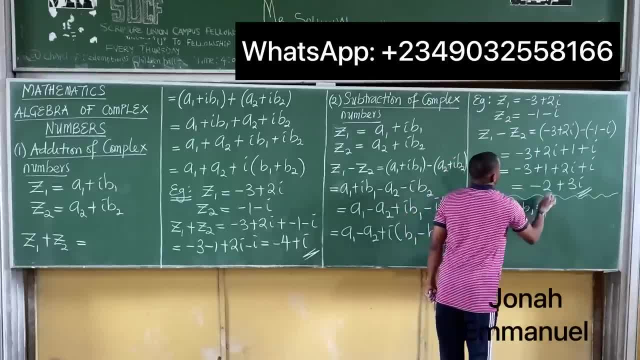 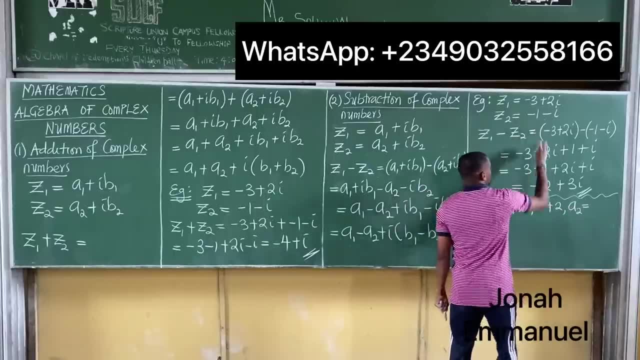 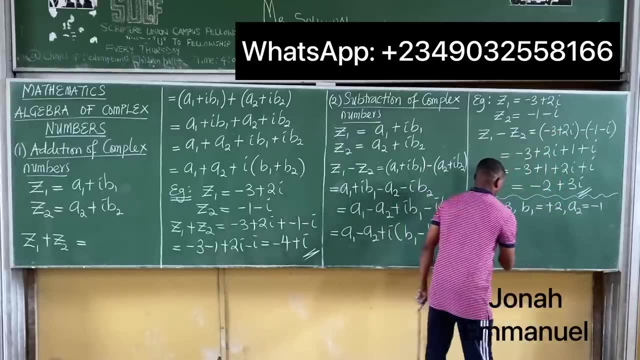 minus 3, b1 will be equal to this plus 2, a2 will be equal to this minus 1. also, b2 will be equal to coefficient of i here minus 1, that's minus 1, let's fix them. 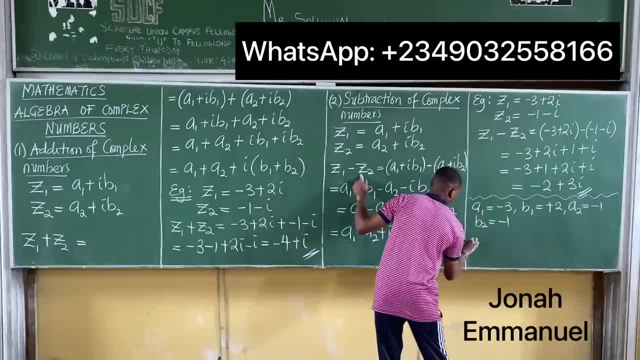 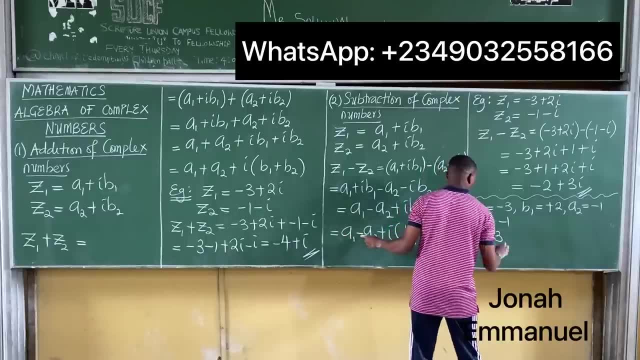 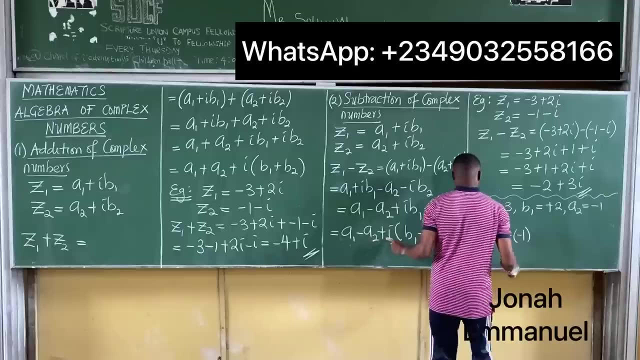 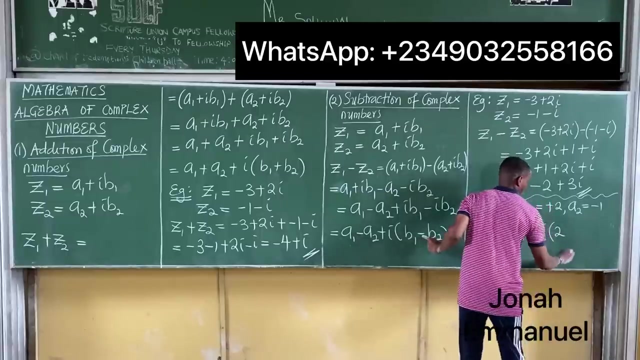 into this formula. so z1 minus z2 will be equal to, will be equal to. we said a1, that's minus 3 minus a2, a2 is minus 1, okay, plus i into b1, b1 is plus 2, minus, so minus. 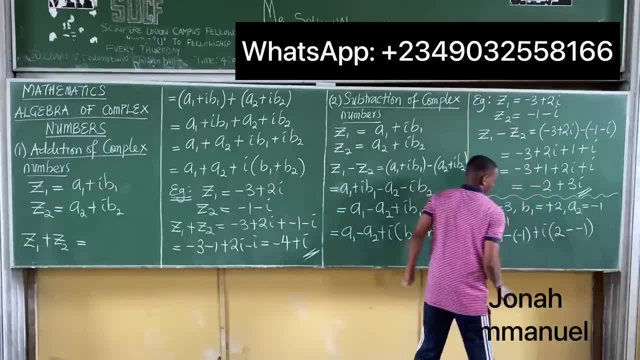 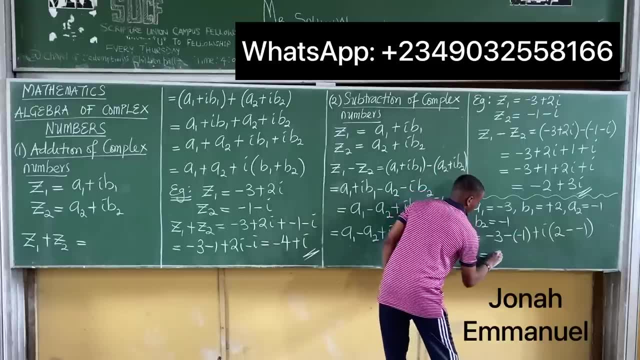 b2, b2 is minus 1, if I work on this, this is equal to I'm having minus 3, minus minus is plus. minus 3 plus 1 is minus 2. plus i into 2, minus minus is plus. 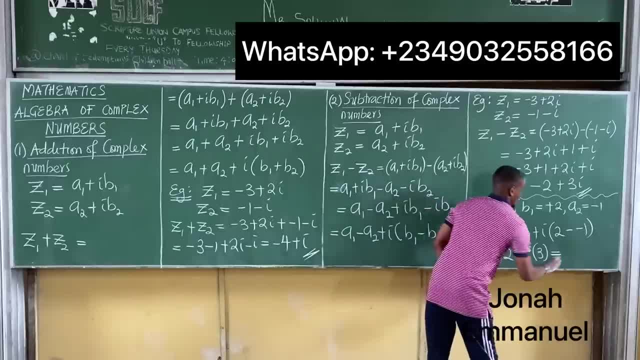 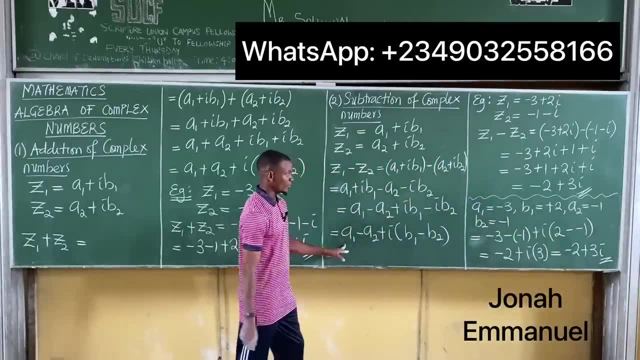 2 plus 1 is 3, so this will be equal to minus 2 plus 3i the same value. so you can choose to use this formula if you want, to any of the formula, or you can subtract directly. so this is a simple idea of how you. 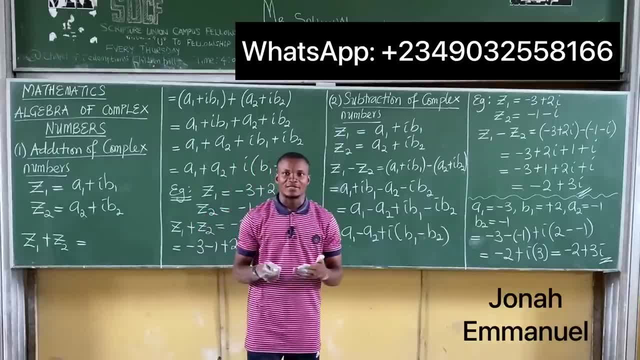 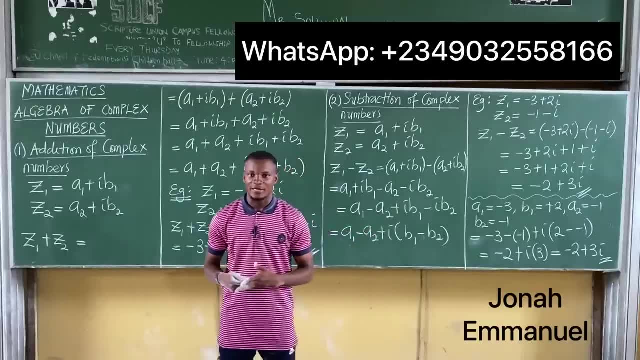 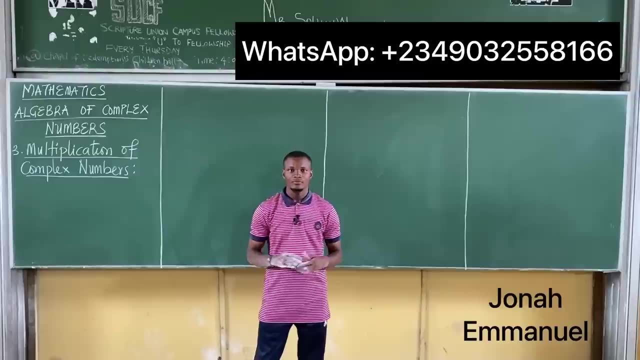 add and subtract complex numbers. simply add their real parts together and perhaps add and subtract their imaginary parts together. alright, let's look at the next concept, which is the multiplication of complex numbers. alright, so let's look at the multiplication of complex numbers. 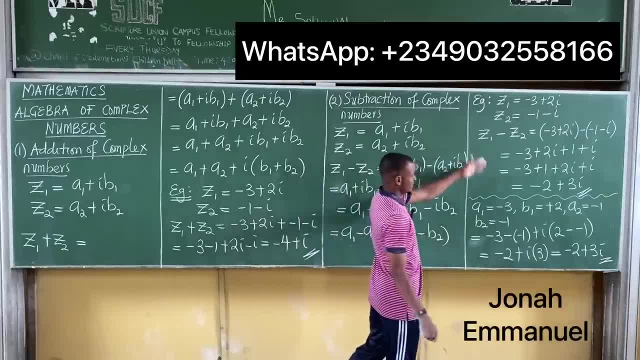 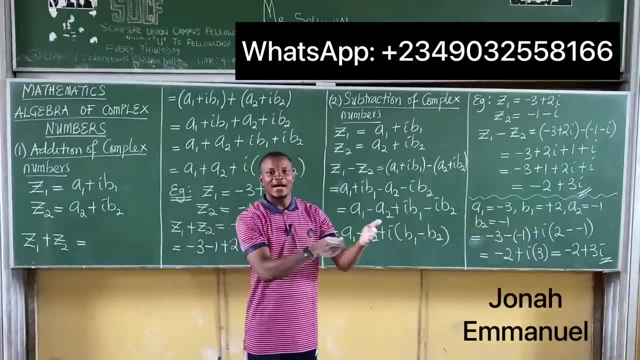 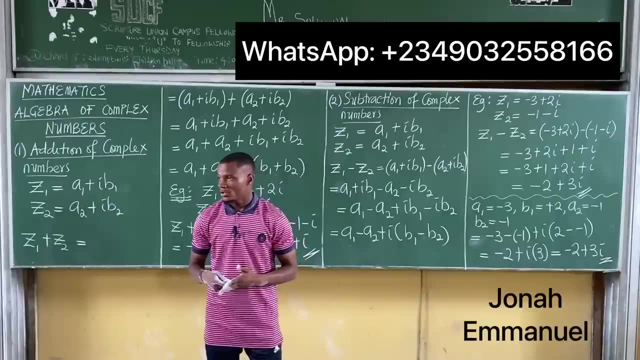 this formula, if you want to any of the formula or you can subtract directly. so this is a simple idea of how you add and subtract complex numbers. simply add their real parts together and perhaps add and subtract their imaginary parts together. all right, let's go to the next concept, which is the multiplication of 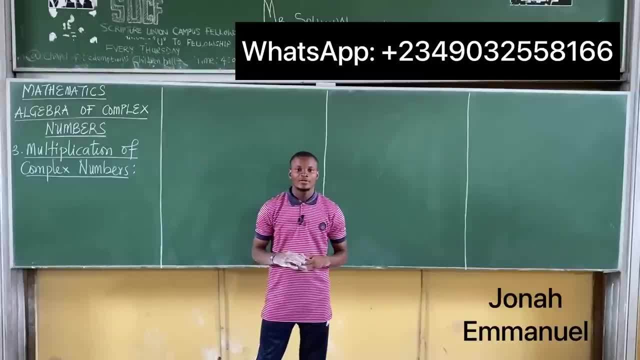 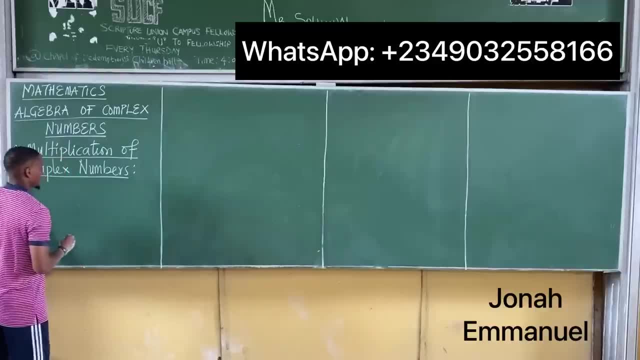 complex numbers. all right, so let's look at the multiplication of complex numbers. before we look at multiplication of complex numbers, let's note something we said: i is equal to square root of 2, so if i take, i squared, that will be equal to the square root of minus 1, all squared. where this 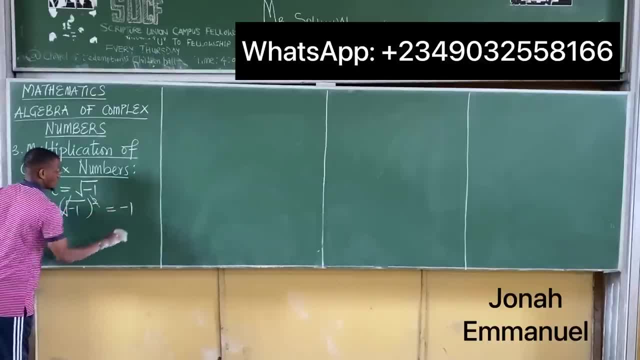 square will cancel square root and that's equal to minus 1. okay, i cubed will be equal to um. root minus 1 cube, which is equal to root minus 1 squared times root minus 1. of course, this 2 will give 6. give you root minus 1 cube, the square of it. 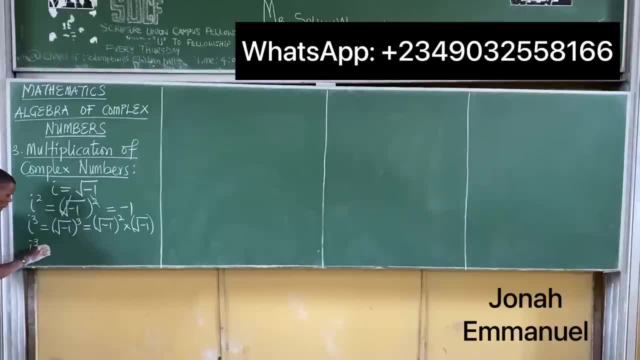 and then itself. That means that i cubed is equal to root minus 1. squared, as we've gotten here, is equal to minus 1. multiplying root minus 1, we said, is equal to i. That's i. This is equal to minus i. Finally, i. 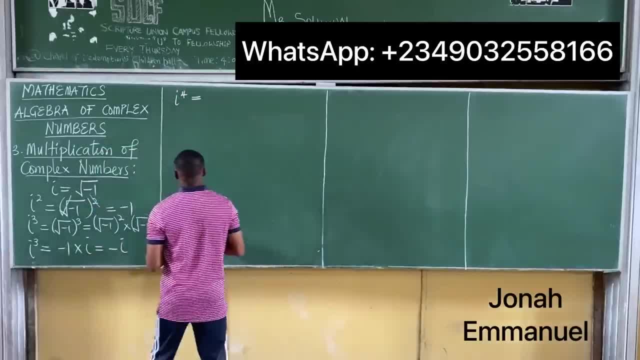 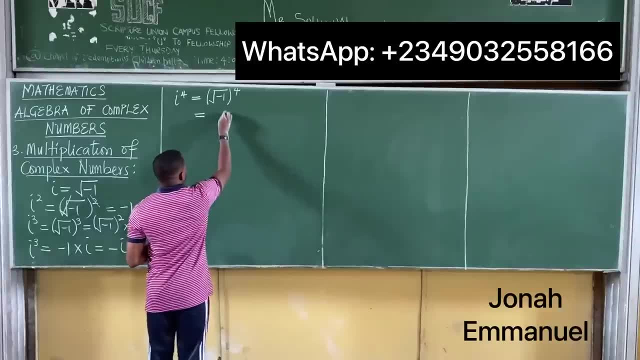 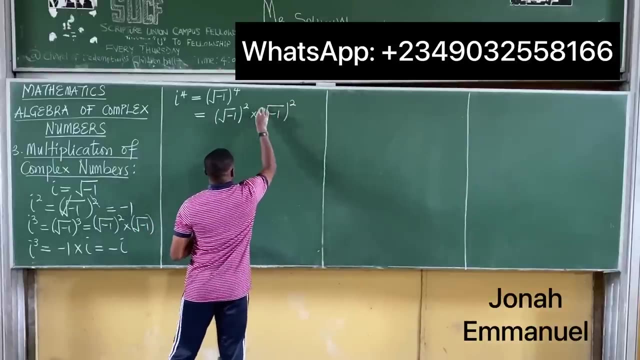 to the power 4 is equal to root minus 1. all to the power 4. this can be broken down as root minus 1, all squared, multiplying root minus 1, all squared, And that's equal to root minus 1. all squared is equal to minus 1. 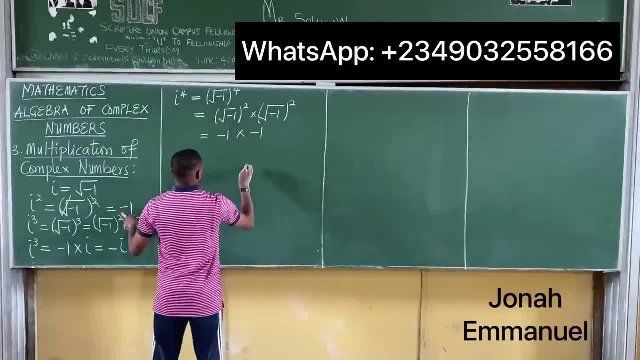 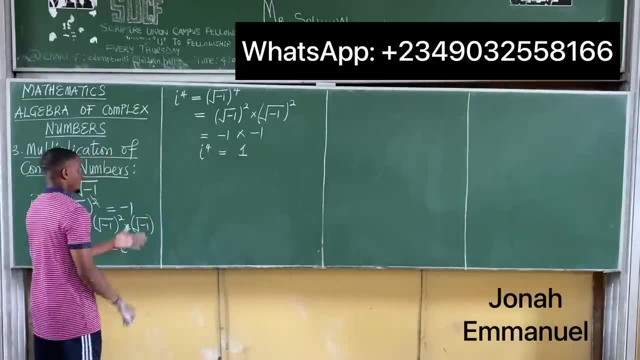 multiplying root minus 1, all squared is equal to minus 1 minus 1. times minus 1 is 1.. So i to the power 4 is equal to 1.. So note these four things. Note that i is equal to root minus 1. 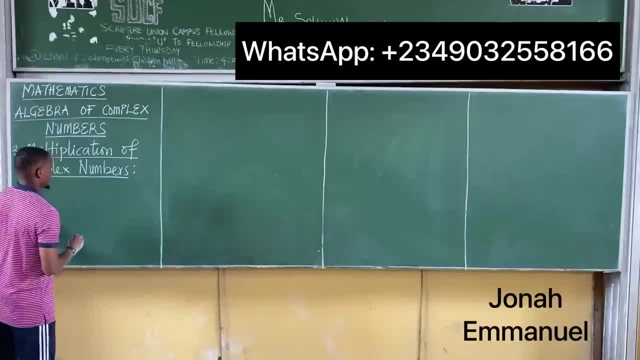 before we look at multiplication of complex numbers, let's note something we said: i is equal to square root of minus 1, so if I take, i squared, that will be equal to the square root of minus 1, all squared where this square will cancel square root, and that's equal to. 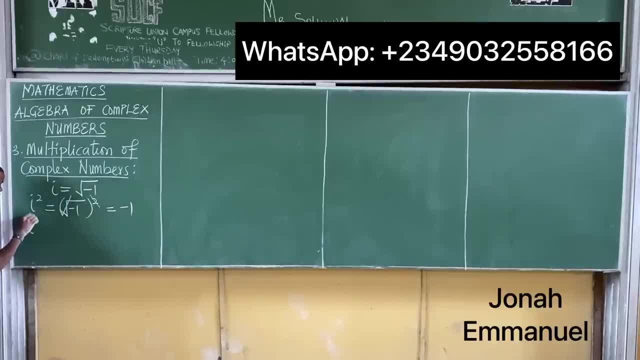 minus 1, okay, i cubed will be equal to root minus 1 cubed, which is equal to root minus 1 squared times root minus 1. of course, these two will give you root minus 1 cubed, the square of it and then itself. 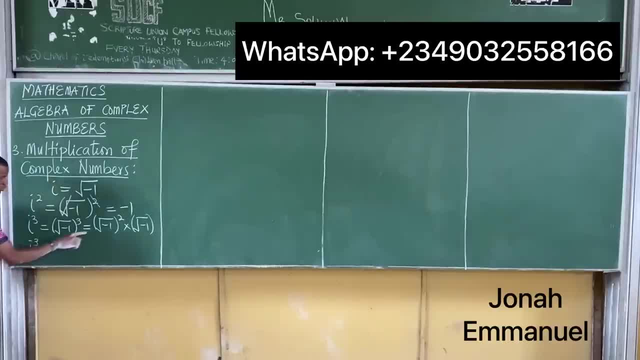 that means that i cubed is equal to root minus 1. squared as we've gotten here, is equal to minus 1, multiplying root minus 1, we said, is equal to i. that's i. this is equal to minus i. finally, i to power 4. 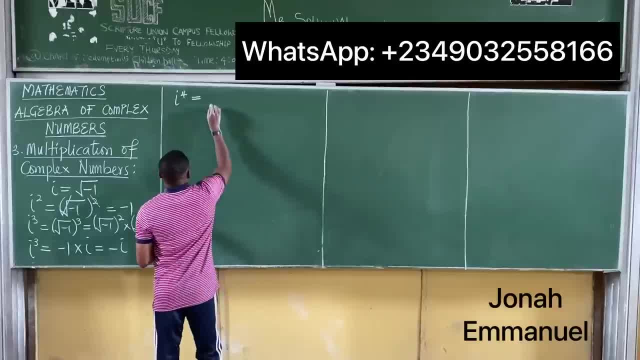 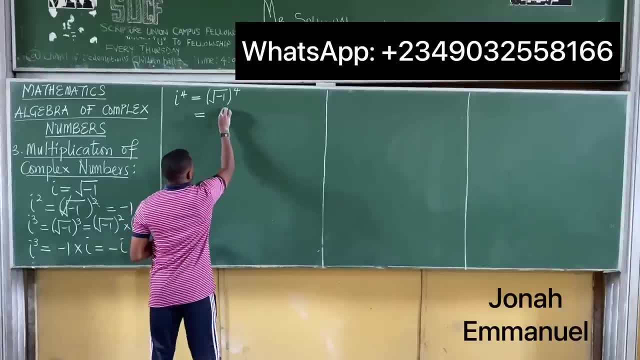 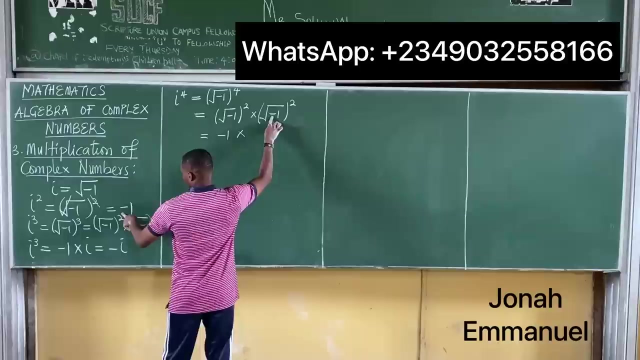 is equal to root minus 1, all to power 4. this can be broken down as: root minus 1, all squared. multiplying root minus 1, all squared, and that's equal to root minus 1, all squared is equal to minus 1, multiplying root minus 1, all squared. 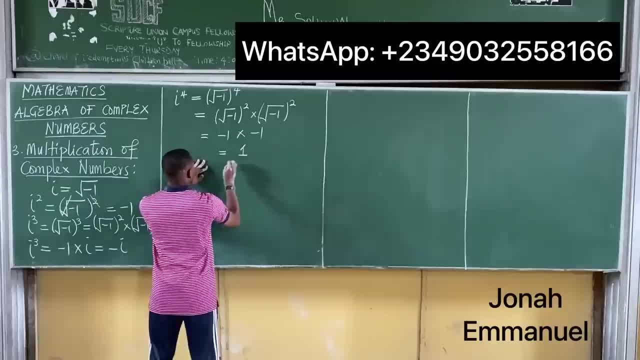 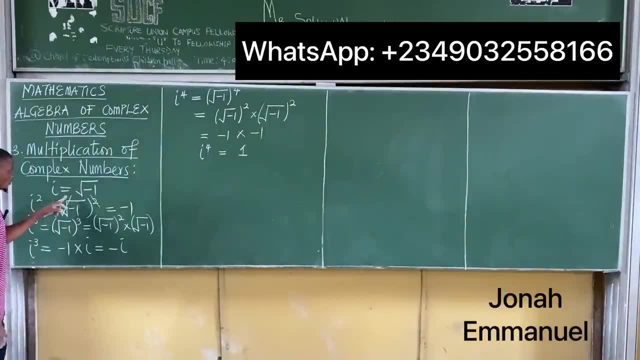 is equal to minus 1, minus 1 times minus 1 is 1. so i to power 4 is equal to 1. so note these four things. note that i is equal to root minus 1. i squared is equal to minus 1. 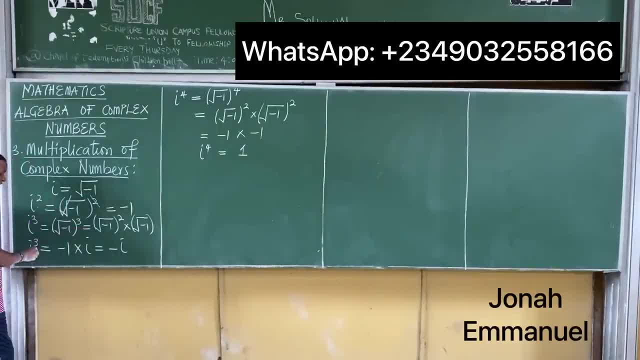 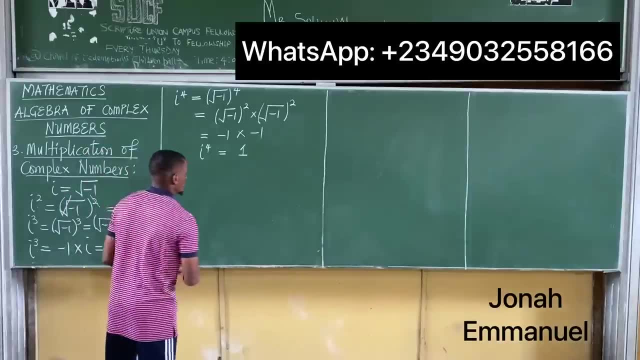 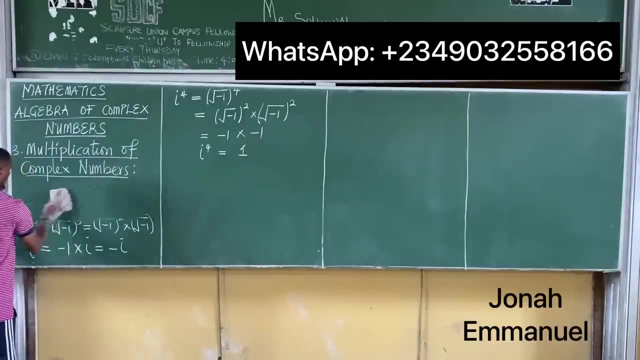 i squared is minus 1.. i cubed is minus i. i to the power 4 is 1.. So get this down and we use them in our solving table. 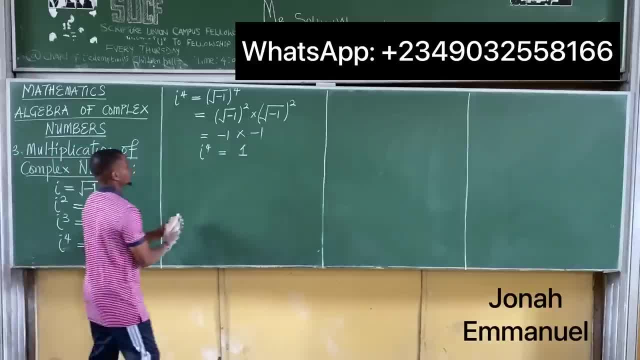 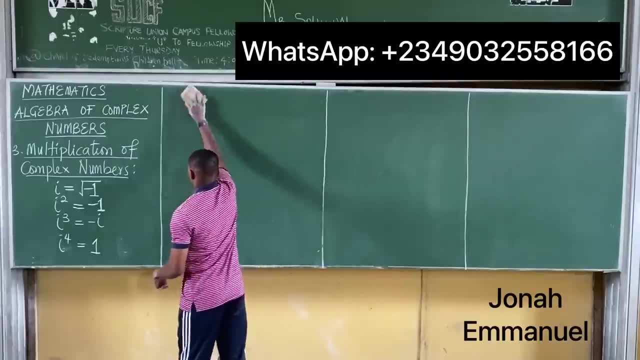 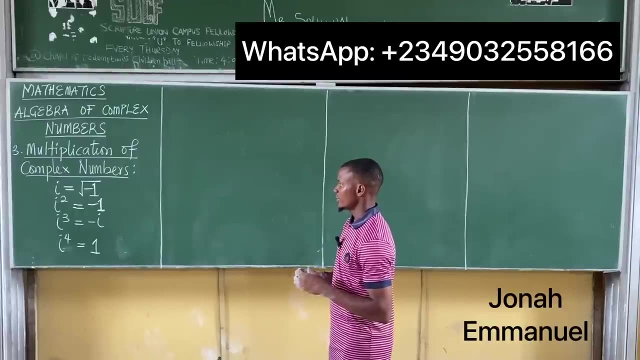 All right, I think this is good. All right. so we said: i is equal to root minus 1, i squared is minus 1, i cubed is minus i and i to the power of 4 is 1.. Let's see how we can use this in solving. 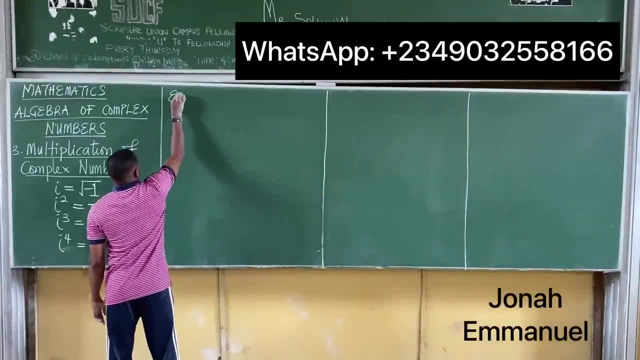 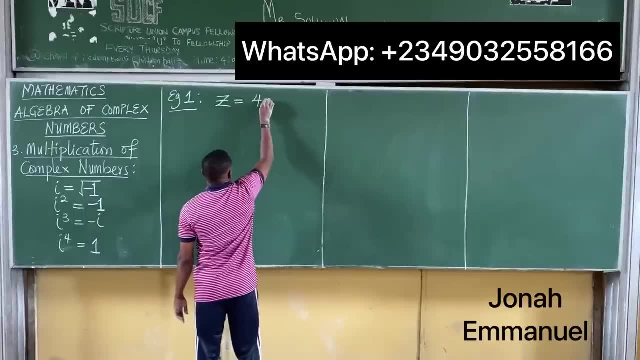 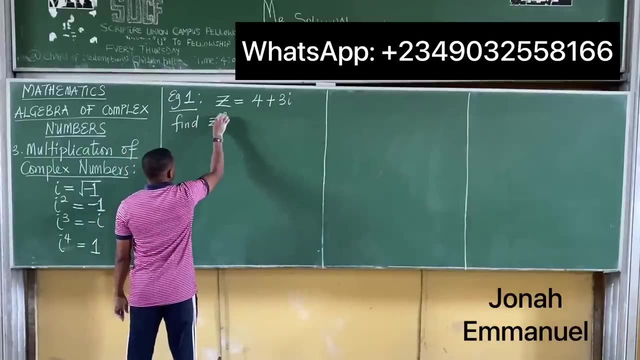 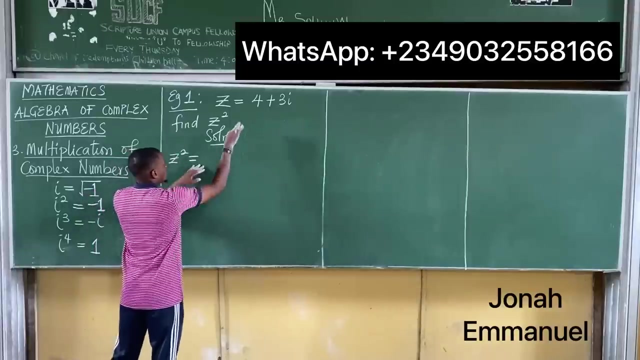 So let's say example 1.. Example 1, let's say z is equal to 4 plus 3i, find z squared. Let's say: find z squared, Solution: z squared will be equal to what I have here: 4 plus 3i, all squared. 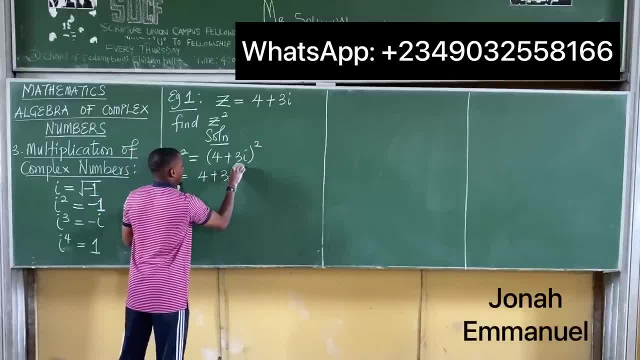 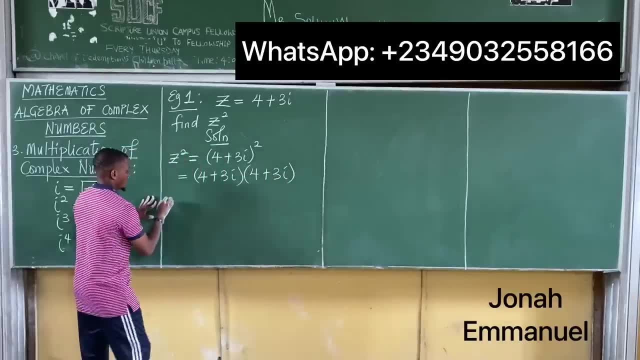 which is equal to 4 plus 3i. 4 plus 3i, all squared, Multiplying 4 plus 3i, Multiplying itself, that's equal to: we said for multiplication, use the first term in the first bracket, 4,. 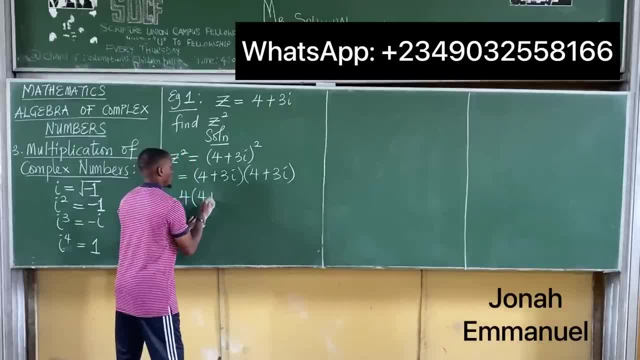 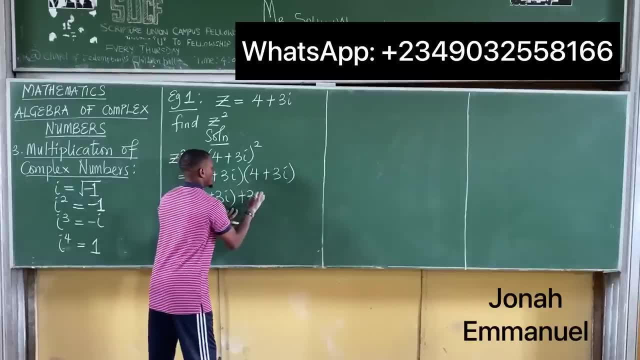 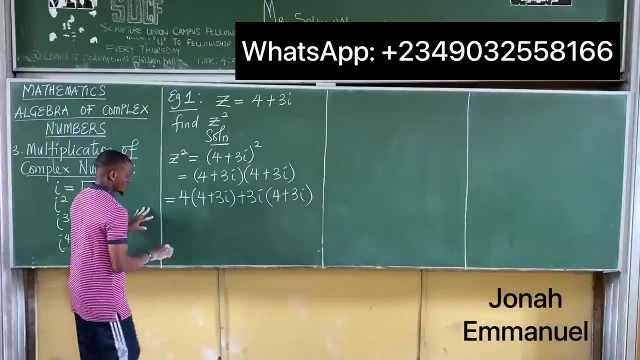 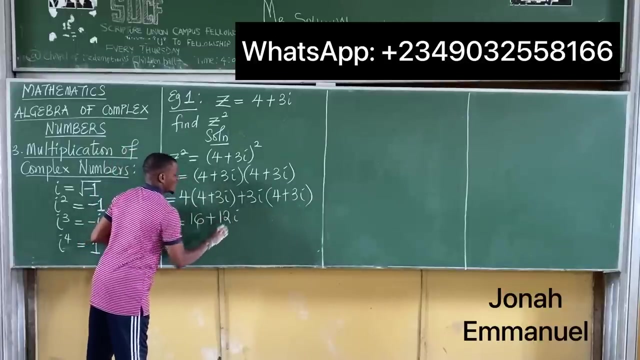 multiply everything in second bracket 4 plus 3i- Second bracket- use the second term in first bracket- plus 3i. multiply everything in second bracket 4 plus 3i. All right, that's equal to 4 times 4, 16, plus 4 times 3i is 12i. 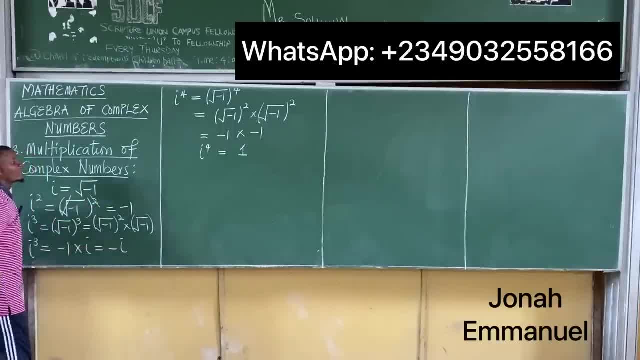 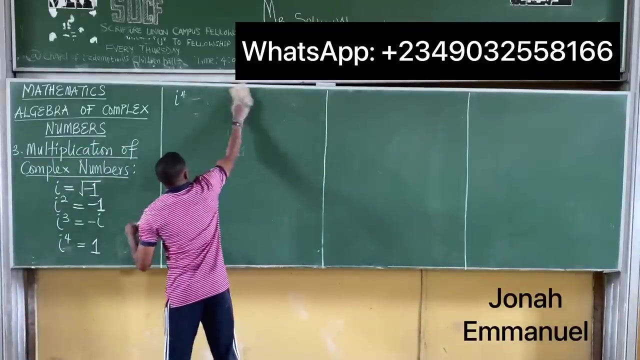 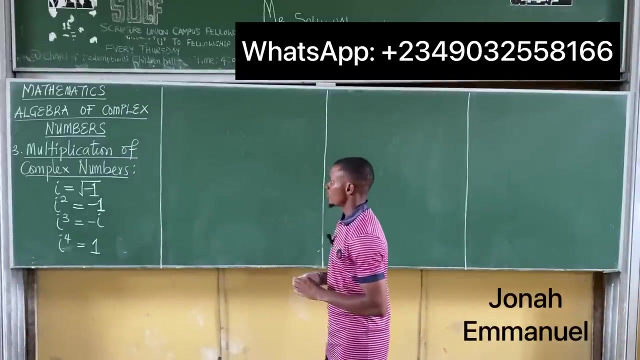 i cubed is equal to minus i. i to power 4 is equal to 1. so we get these down and we use them in our solving. all right, i think this is good. all right, i think this is good, all right. so we said i is equal to root minus 1. 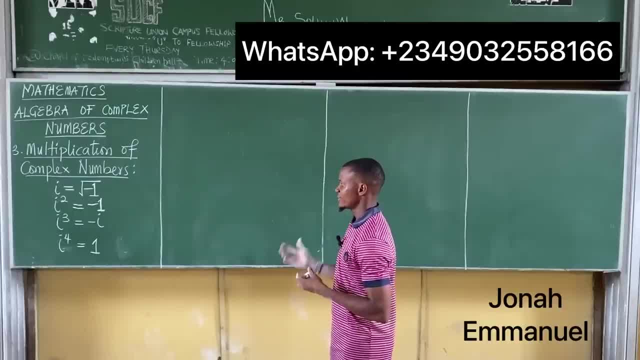 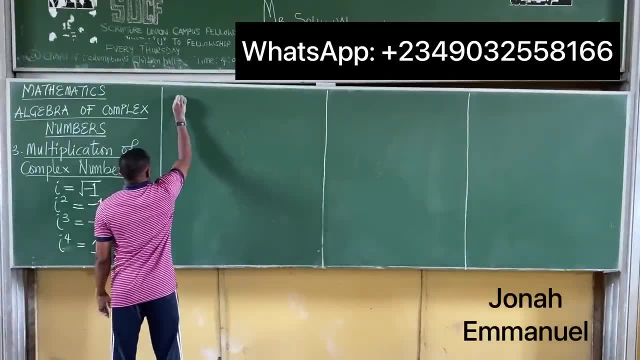 i squared is minus 1, i cubed is minus i and i to power 4 is 1, let's see how we can use this in solving. so let's say example 1, example 1, let's say z is equal to. 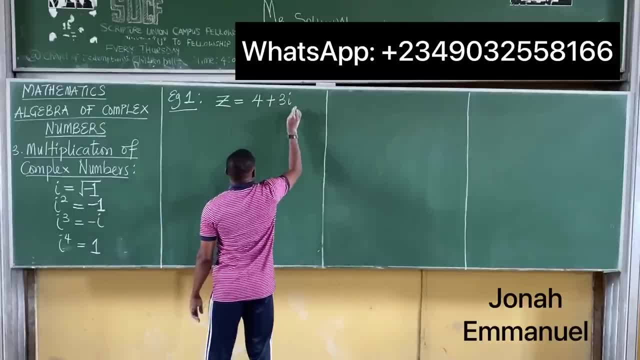 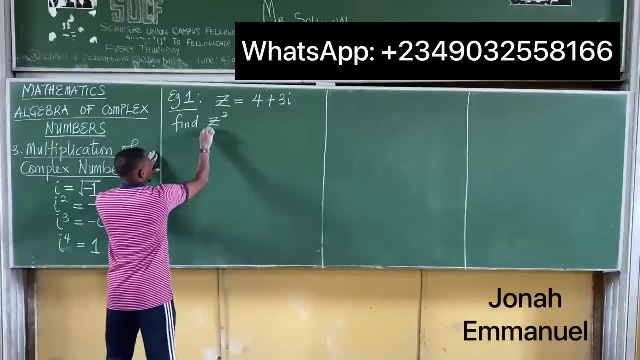 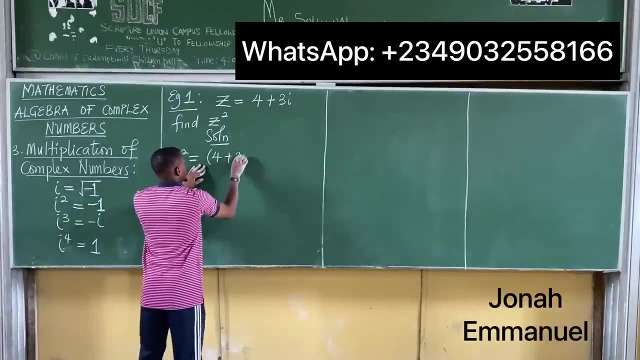 4 plus i squared is equal to minus 1. this in the square root of z squared. find z squared and the solution z squared will be equal to what i have here: 4 plus 3 i all squared, which is equal to 4 plus 3 i. 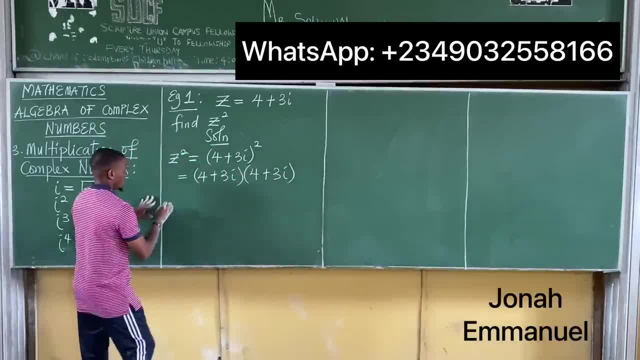 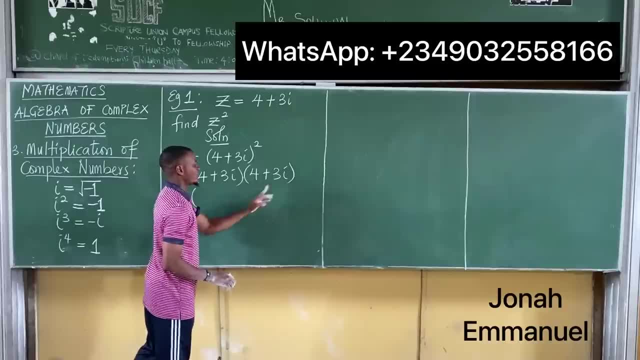 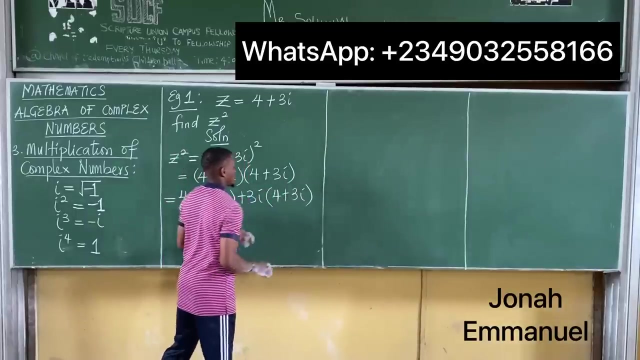 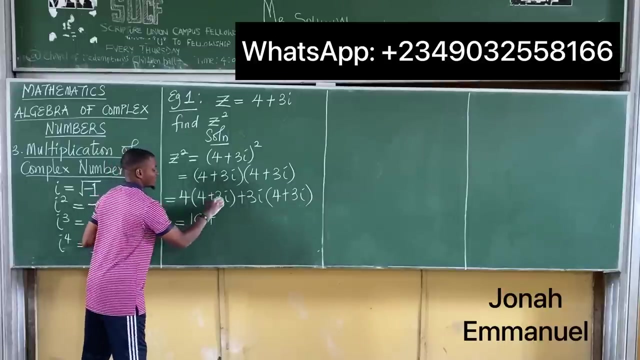 multiplying 4 plus 3: i. multiplying itself, which is equal to the central multiplication in the式的性3má основản了. use the first term in the first bracket, 4,. multiply everything in second bracket, 4 plus 3i. second bracket: use the second term in first bracket plus 3i. multiply everything in second bracket, 4 plus 3i. all right, that's equal to 4 times 4, 16, plus 4 times 3i is 12i. 4 times 3 is 12,. 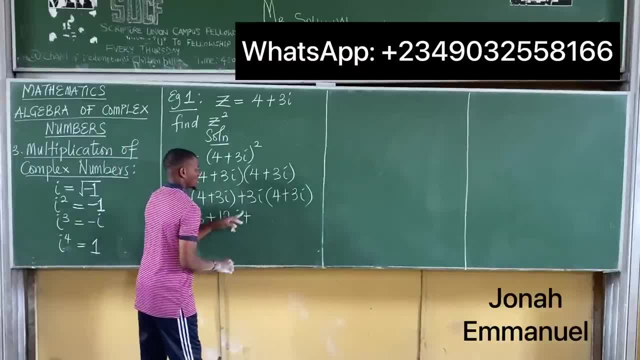 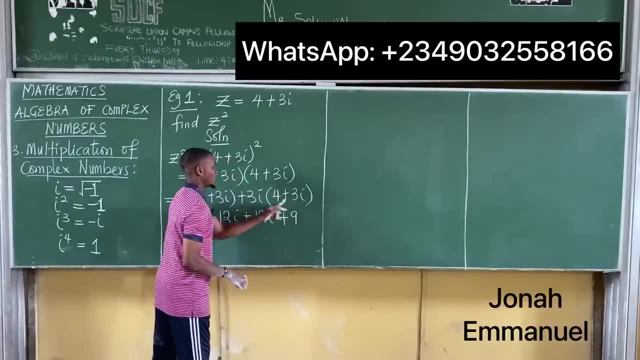 4 times 3 is 12,. bring down the i plus 3 times 4 is 12i plus 3 times 3 is 9,. i times i is i squared. All right, this is equal to 16,. 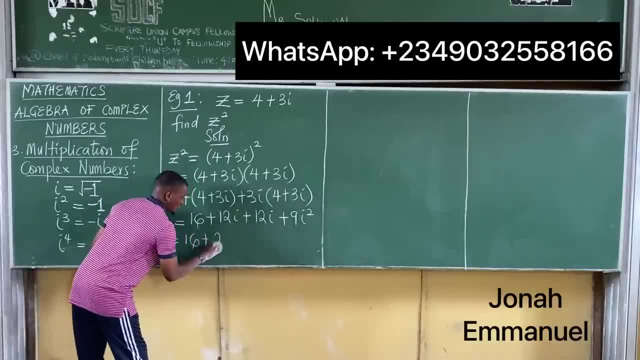 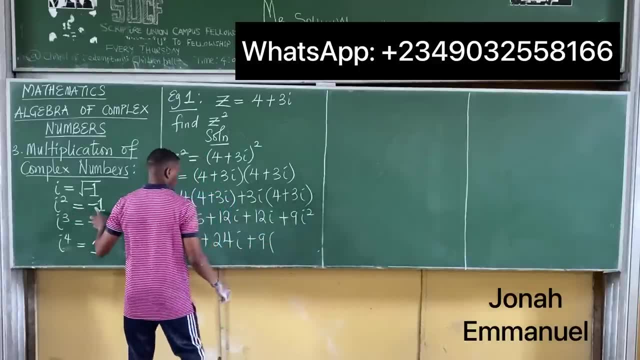 plus 12i plus 12i gives you 24i plus 12i plus 12i gives you 24i plus 9 into i squared. We said i squared is equal to minus 1, but that's minus 1.. 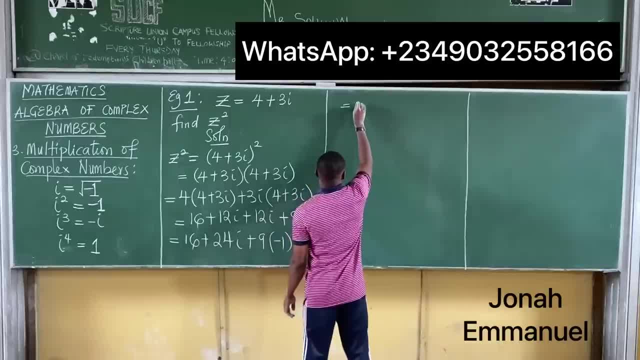 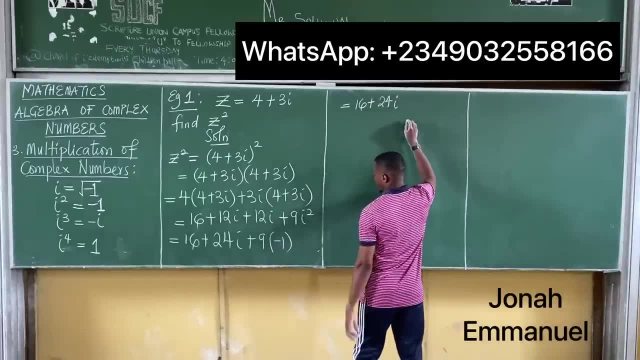 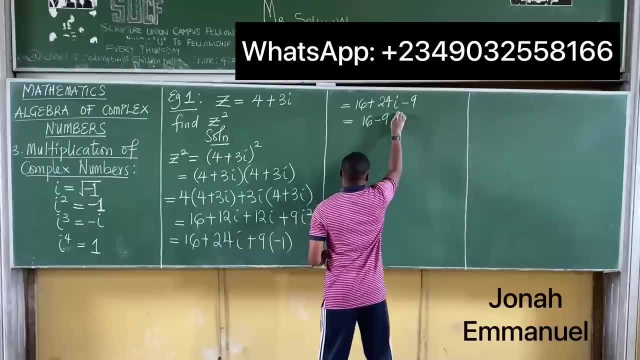 So this is now equal to I'm having here 16, plus 24i, and then plus 9 times minus 1 is minus 9.. If I take out the real parts: 16 minus 9 plus 24i. 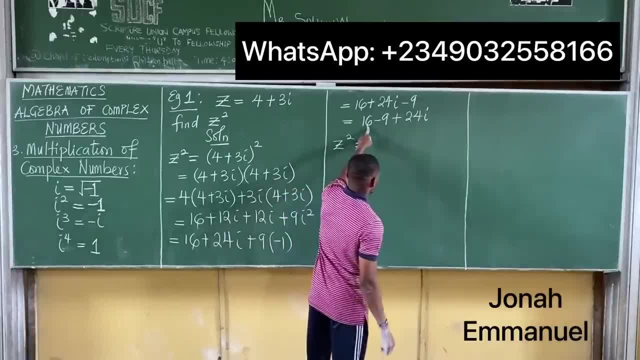 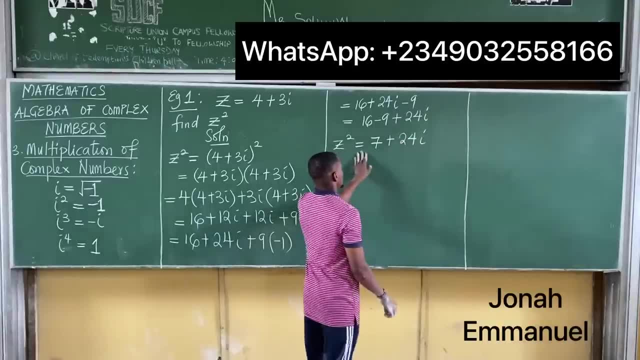 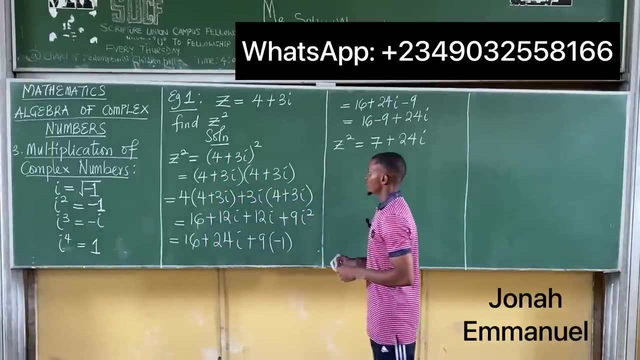 So hence z squared is equal to 16 minus 9,, that's about 7 plus 24i. My answer is 7 plus 24i. So this is how we work, or this is how we solve multiplication of complex numbers. 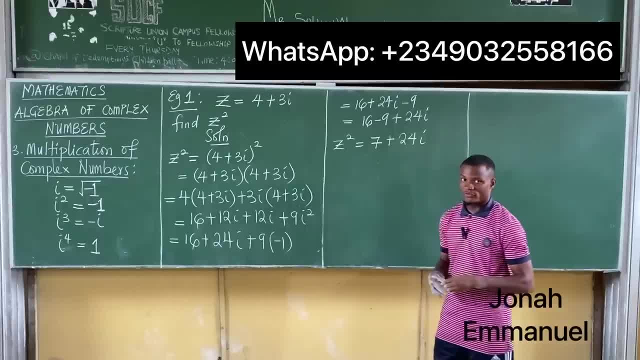 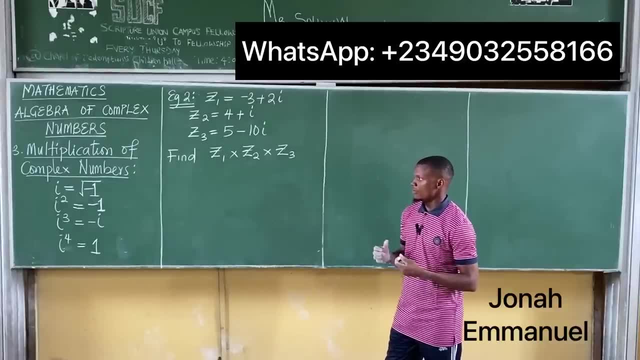 We'll take a second example on this and then we'll move on. So let's take a question, another question on multiplication of complex numbers. We are given z1 has been equal to minus 3 plus 2i, z2 has been equal to 4 plus i. 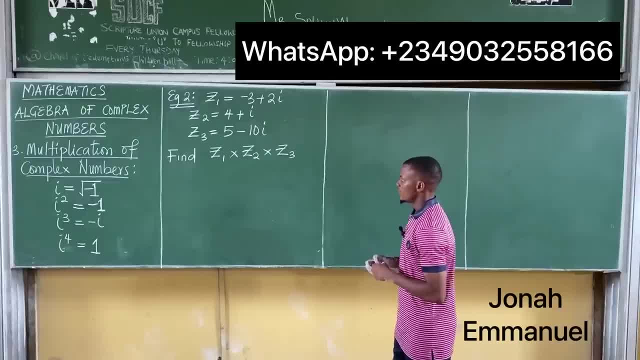 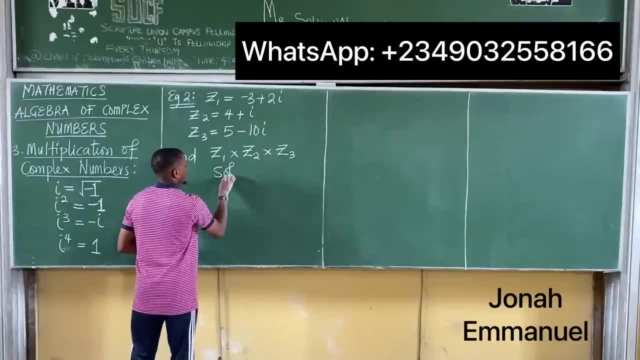 and z3 has been equal to 5 minus 10i, In order to find the value of z1 times z2 times z3.. How do you solve that Solution? of course, your first task is to multiply 2 first. 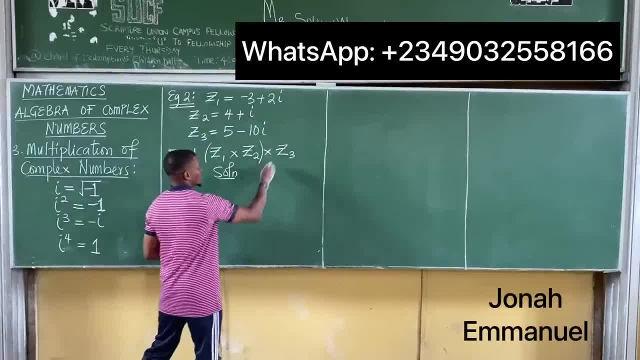 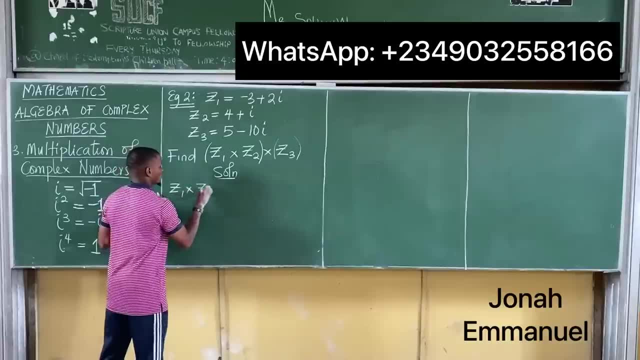 I can choose to work on these two first, Then, with my result, I will now multiply it with z3.. So I'll keep z3 pending work with just z1 and z2.. So z1 times z2 would be equal to. 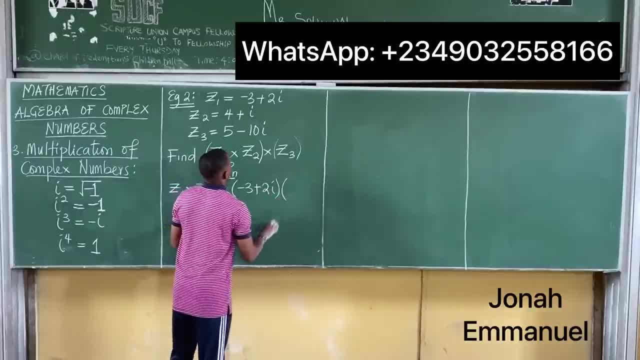 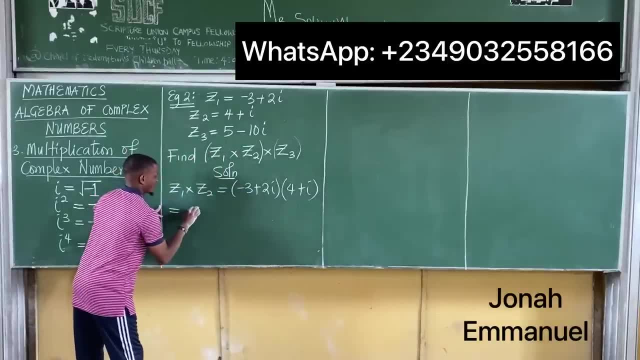 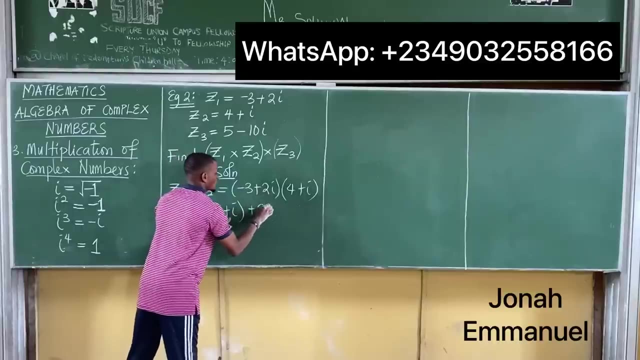 minus 3 plus 2i into z2, 4 plus i. So this will now be equal to the first term in the first bracket minus 3, multiply everything here: 4 plus i. Second term here, plus 2i. 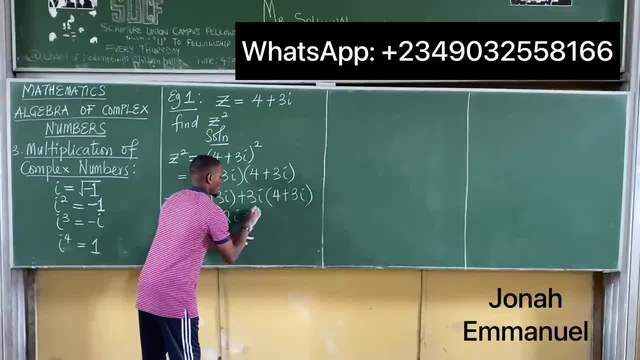 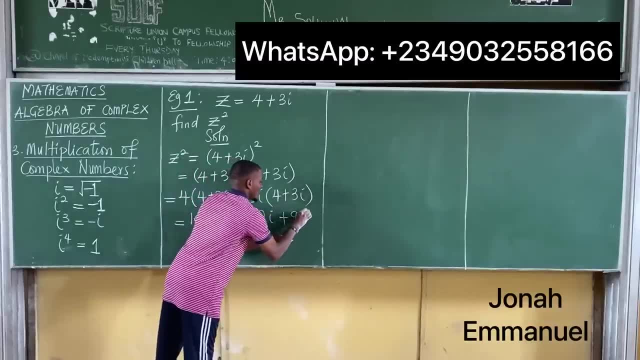 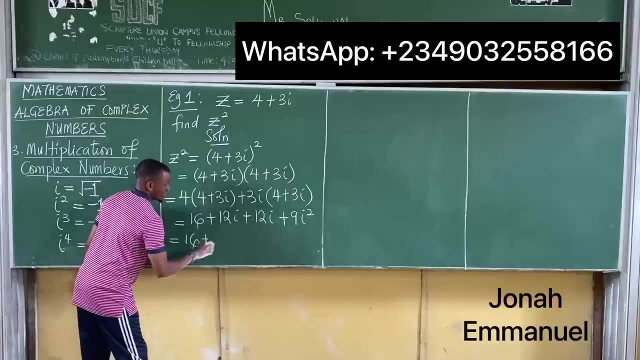 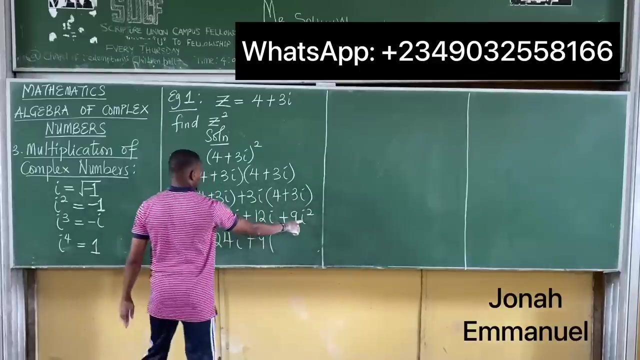 bring down the i plus 3 times 4 is 12i plus 3 times 3 is 9,. i times i is i squared. all right, this is equal to 16, plus 12i plus 12i gives you 24i plus 9 into i squared. we said i squared is equal to minus 1, so that's minus 1,. 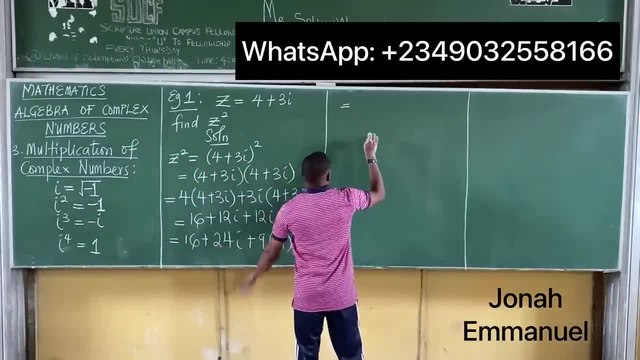 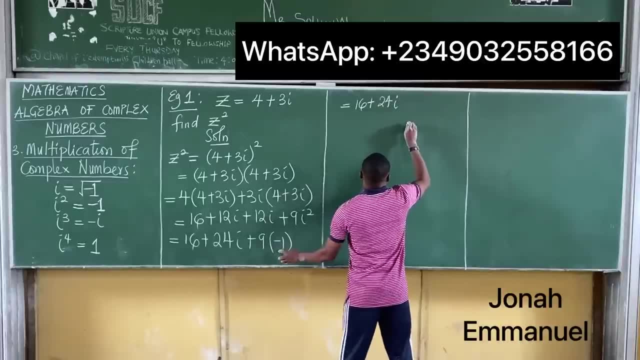 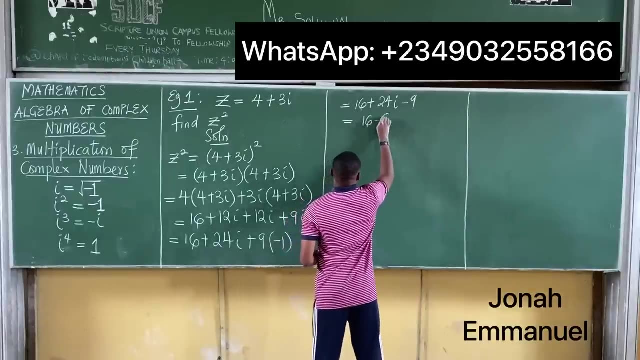 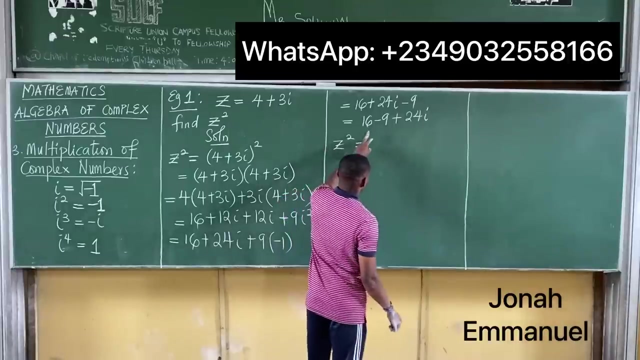 so this is now equal to- i'm having here 16, plus 24i, and then plus 9 times minus 1 is minus 9, if i take out the real parts, 16 minus 9 plus 24i. so hence z squared is equal to 16 minus 9, that's about 7,. 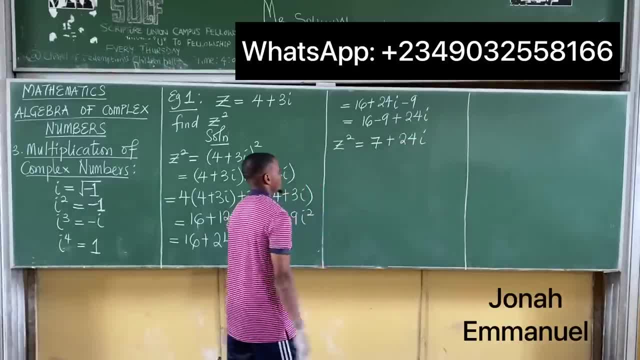 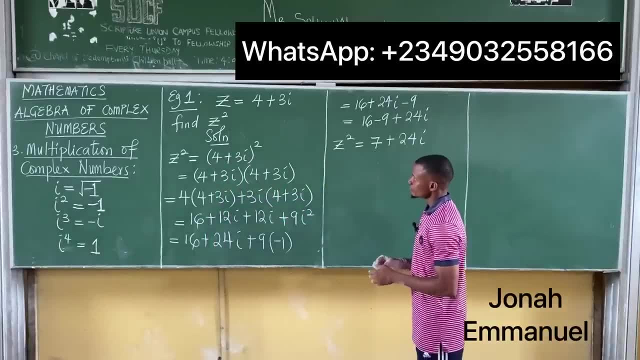 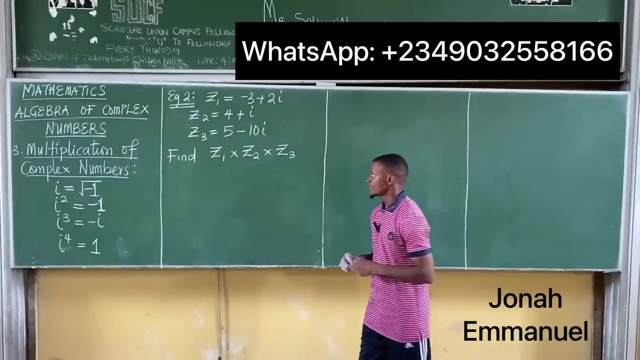 24i. so my answer is 7 plus 24i. so this is how we work, or this is how we solve multiplication of complex numbers. we'll take a second example on this and then we'll move on. so let's take a question. another question on multiplication of complex numbers: we are given z1 has been equal to minus 3 plus 2i. 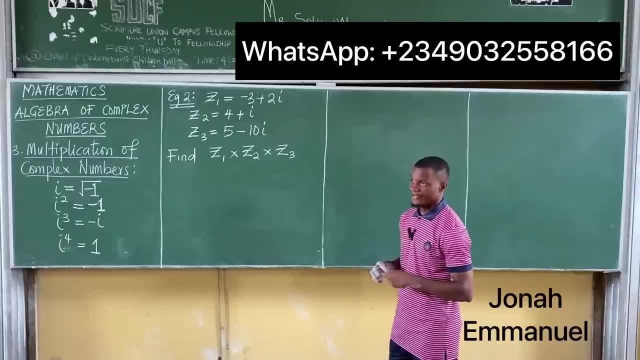 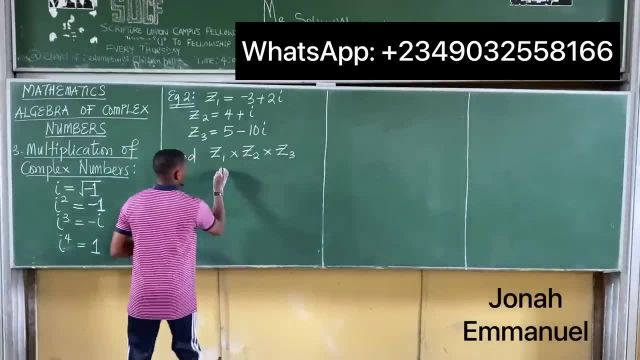 and z3 has been equal to 5 minus 10i, in order to find the value of z1 times z2 times z3, how do you solve that solution? of course, your first task is to multiply 2 first. 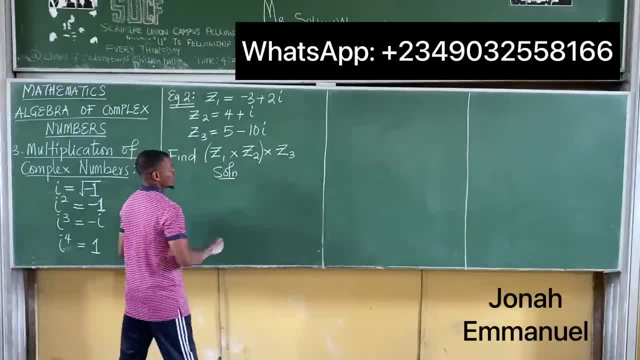 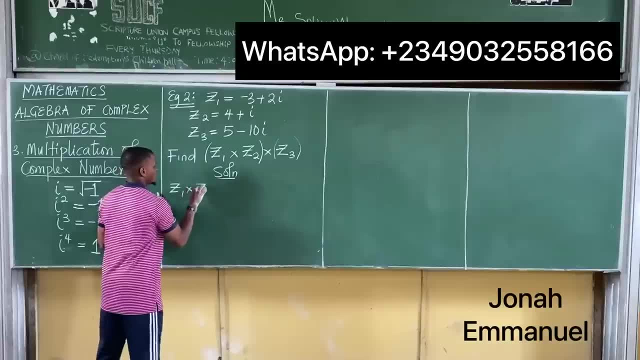 i can choose to work on these 2 first, then with my result. i will now multiply it with z3, so i'll keep z3 pending, work with just z1 and z2, so z1 times z2 would be equal to minus 3 plus. 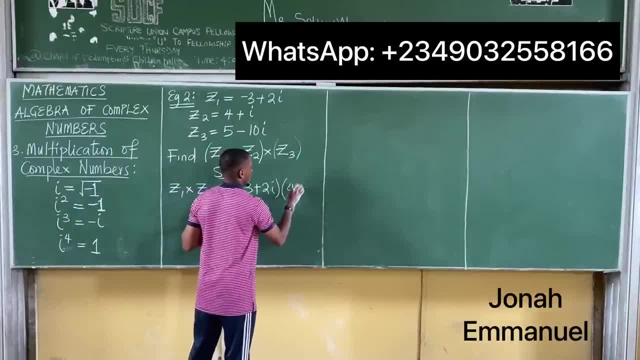 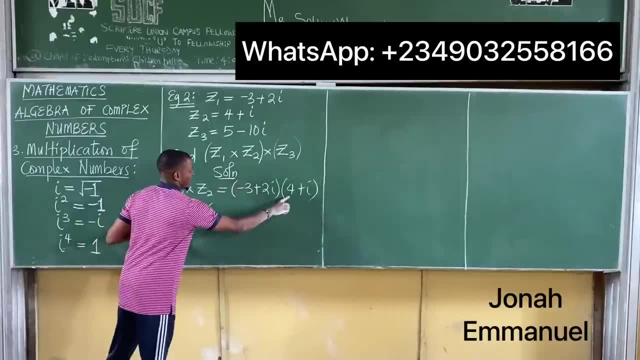 2i into z2, 4 plus i. so this would now be equal to the first term in the first bracket minus 3, multiply everything here: 4 plus i. second term here plus 2i. 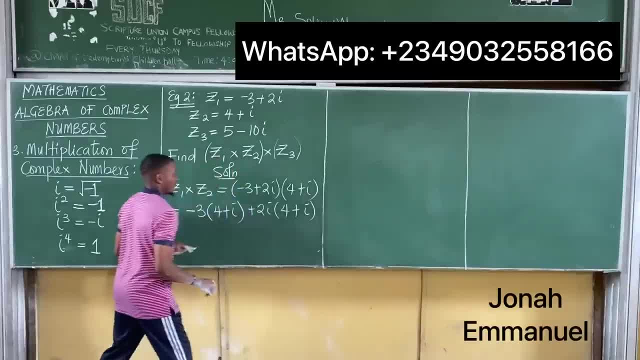 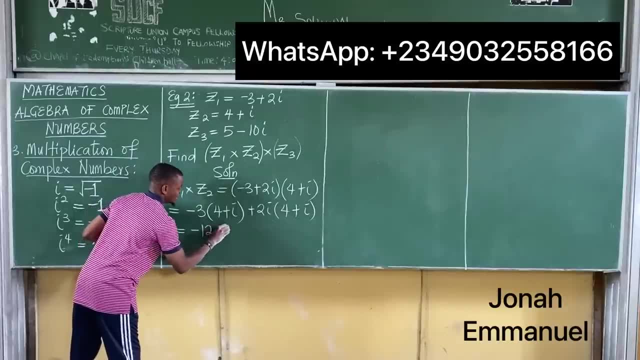 multiplies everything here: 4 plus i. So multiply this: minus 3 times 4 is minus 12,. minus 3 times i is minus 3i. plus 2i times 4 is plus 2 times 4 is 8,. 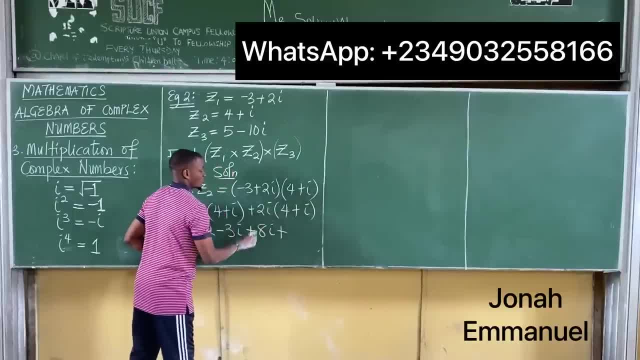 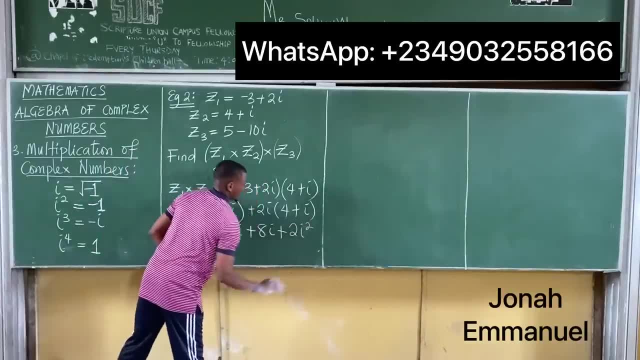 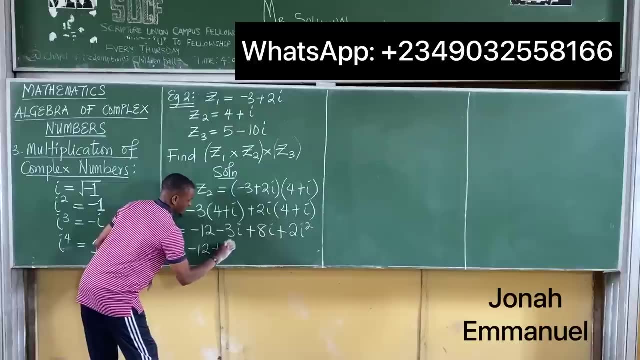 bring down the i plus plus is plus 2i times i is 2i squared. This is i squared, please, Alright, so that's equal to minus 12, minus 3, minus 3 plus 8 is plus 5i. 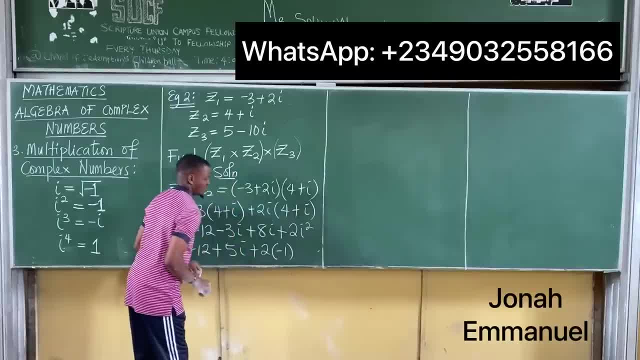 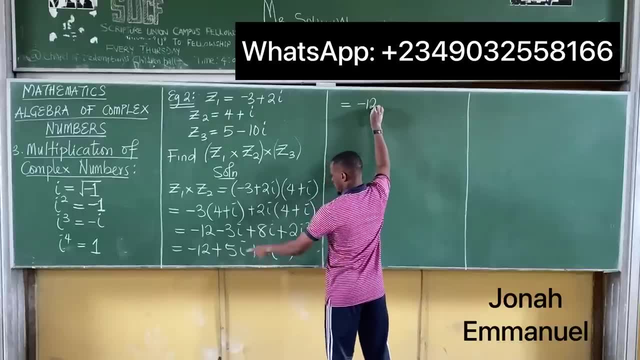 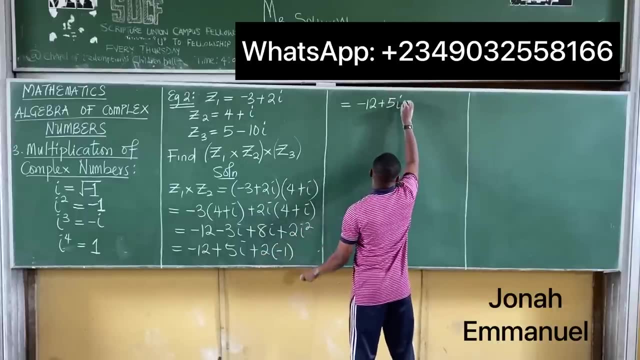 then plus 2, i squared, we said is minus 1.. So that will be equal. to take the okay. simplify this first: minus 12 plus 5i plus 2 times minus 1 is minus 2.. So if I take the real part, 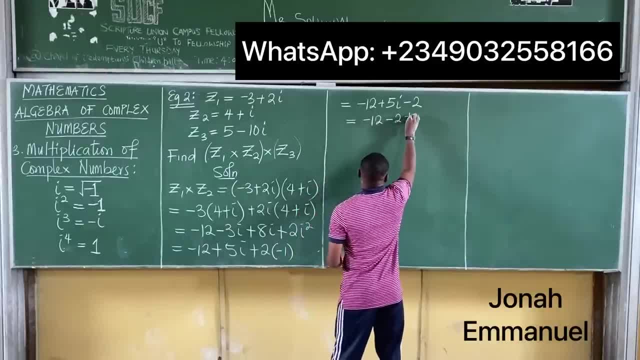 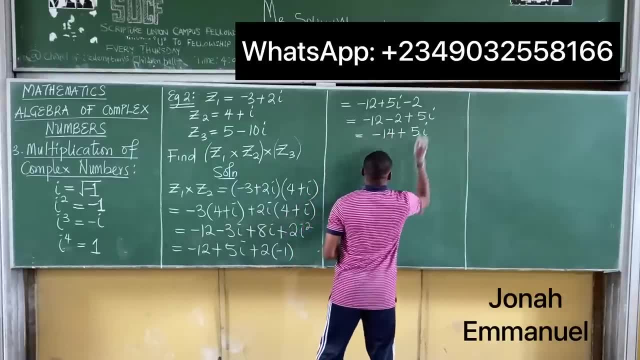 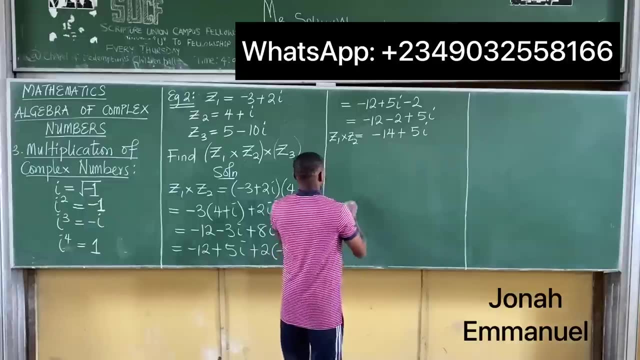 minus 12 minus 2, the imaginary part plus 5i, Minus 12 minus 2 is minus 14 plus 5i. This is the value of z1 times z2.. Finally, let's now add z1 times z2 times z3.. 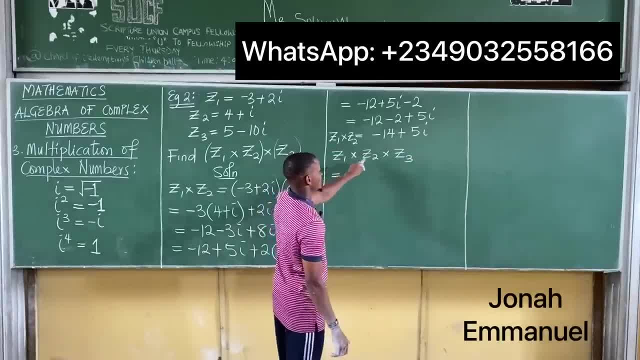 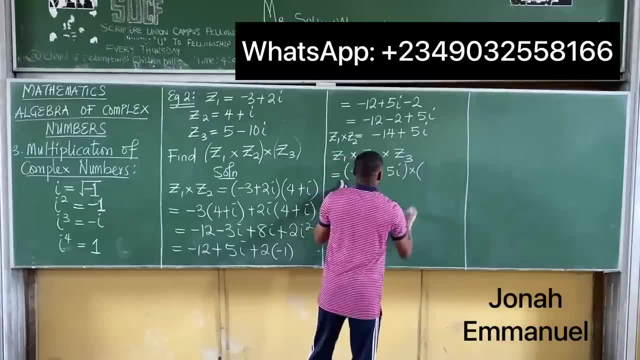 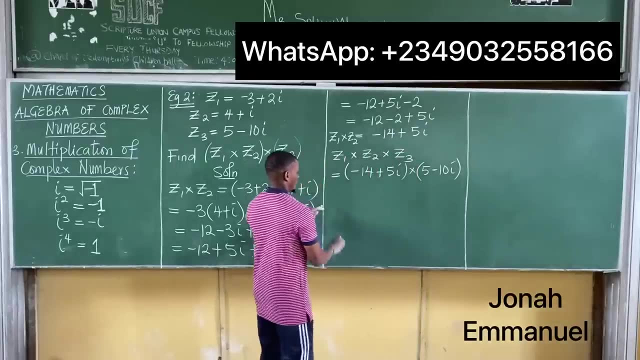 So that will be equal to the result of z1 and z2, we have it as minus 14 plus 5i, multiplied by the result of z3, that's 5 minus 10i. Alright, so we go again. 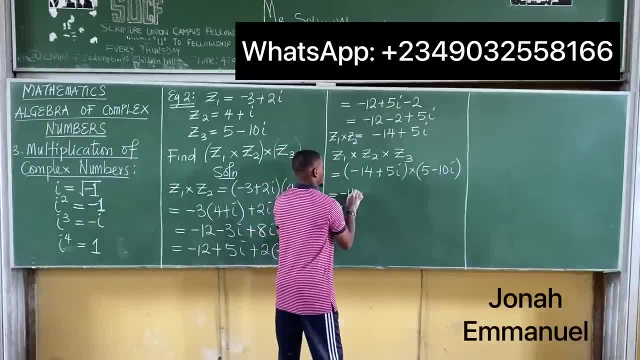 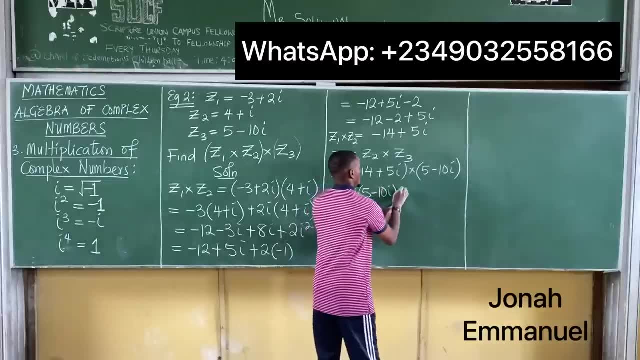 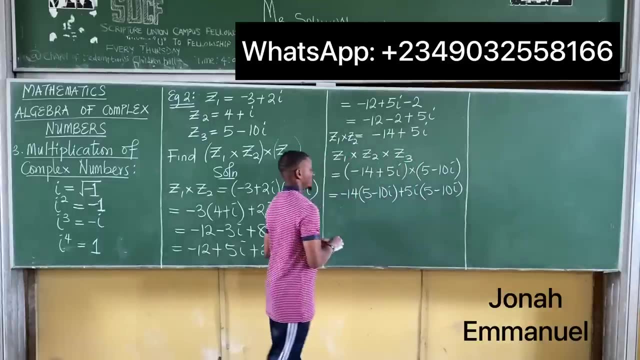 that's equal to: first, 10 here minus 14,. multiply everything here: 5 minus 10i. second, 10 here plus 5i. multiply everything here: 5 minus 10i. This is equal to, if I multiply this: 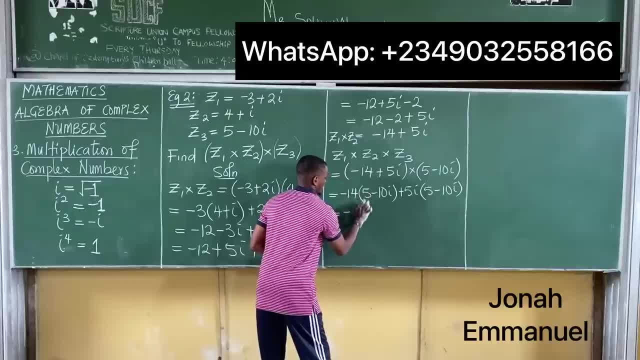 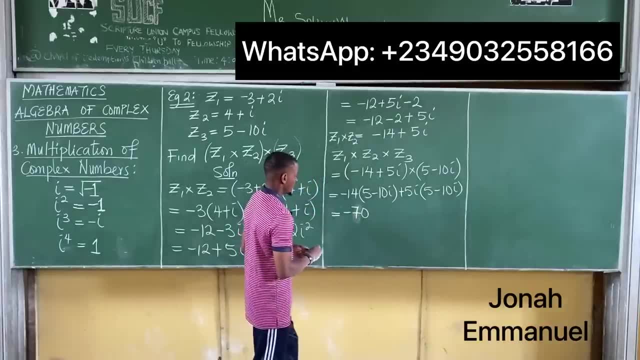 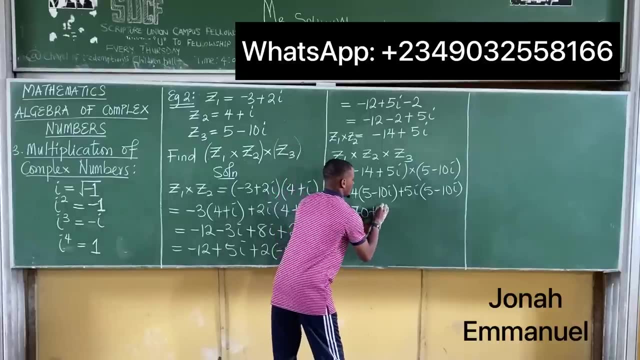 14 times 5, I'm having minus 70,. okay, so minus 14 times 5 is minus 70,. minus minus is plus minus 14, so minus minus is plus. 14 times 10 is 140i. 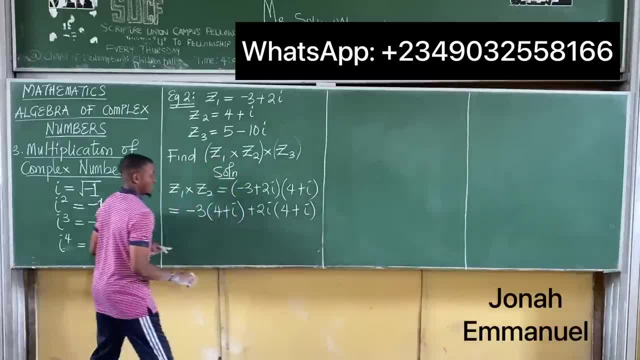 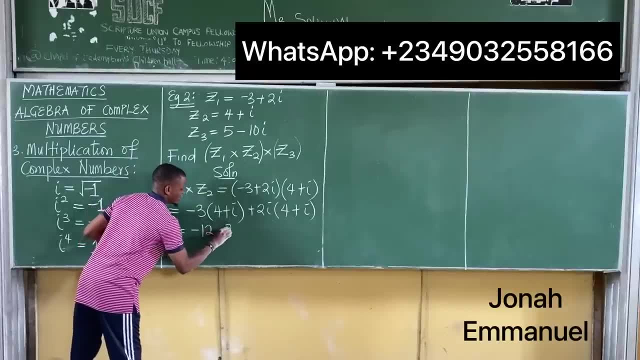 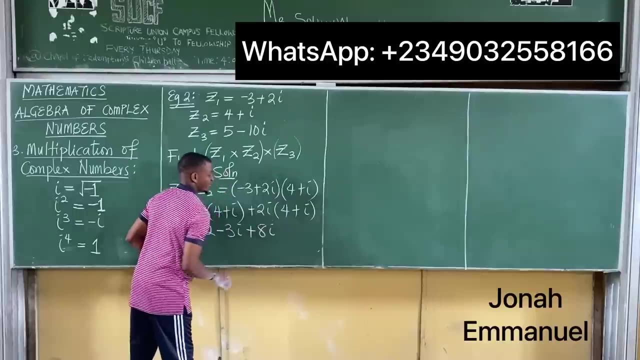 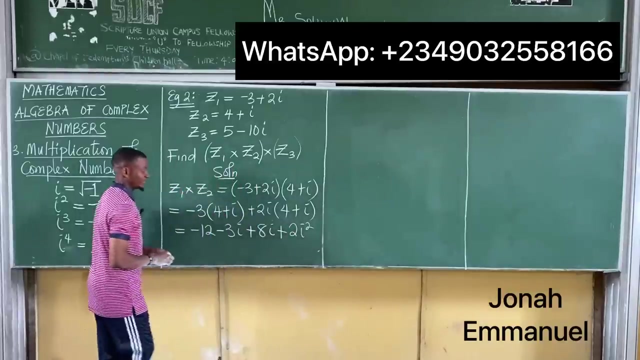 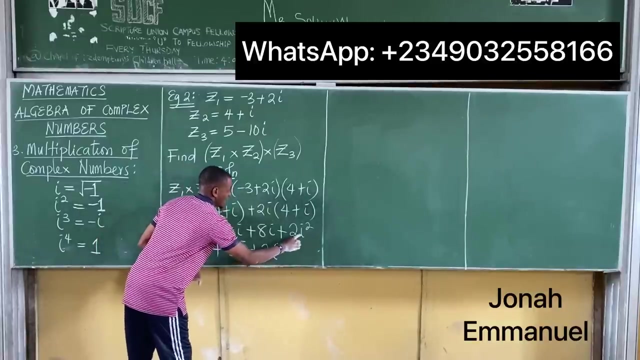 multiplies everything here: 4 plus i. so multiply this: minus 3 times 4 is minus 12, minus 3 times i is minus 3i. plus 2i times 4 is plus 2 times 4 is 8, bring down the i plus plus is plus 2i times i is 2i squared. this is i squared, please. all right, so that's equal to minus 12, minus 3 plus 8 is plus 5i, then plus 2, i squared, we said, is minus 1,. 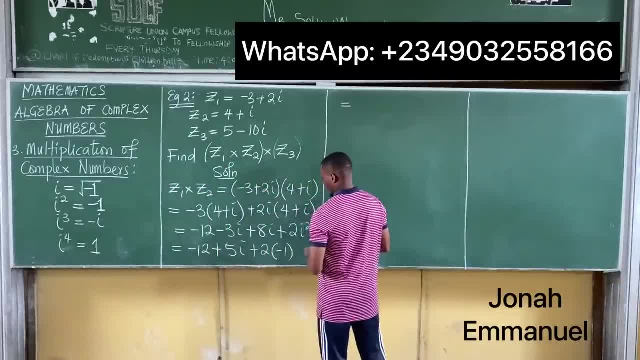 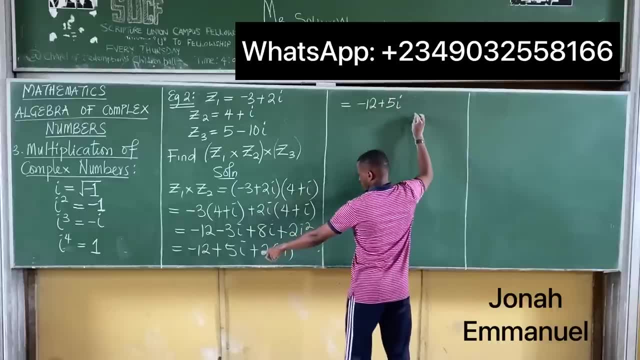 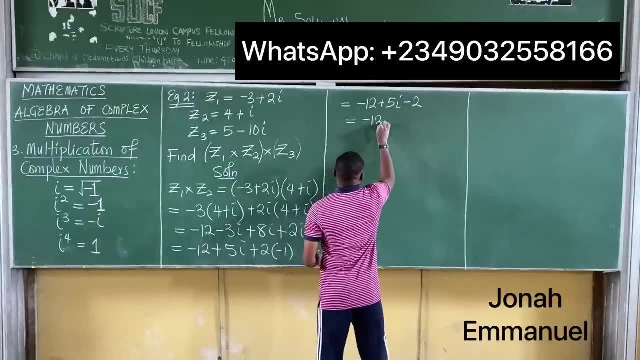 so that would be equal. to take the okay. simplify this first: minus 12, plus 5i plus 2 times minus 1 is minus 2, so if i take the real part minus 12 minus 2, the imaginary part, plus 5i minus 12 minus 2 is minus 14 plus 5i. 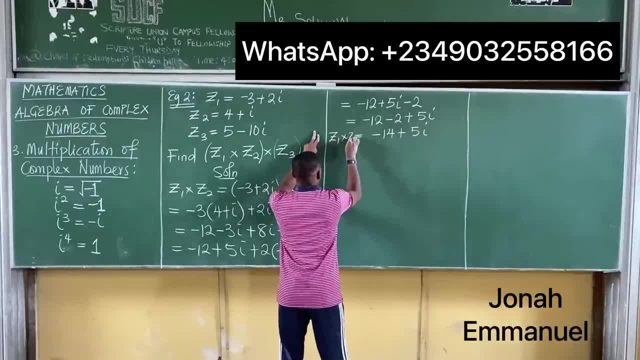 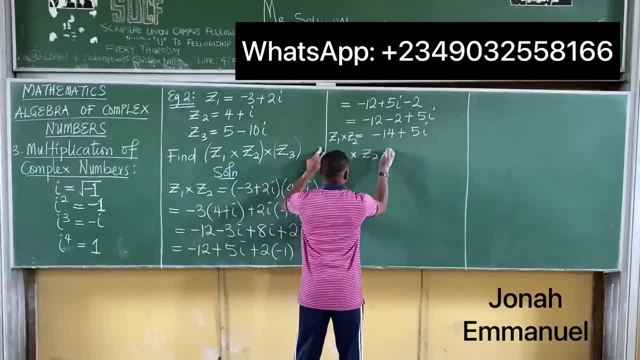 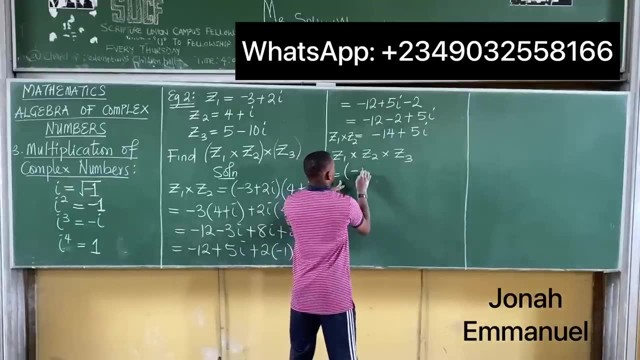 this is the value of z1 times z2,. finally, let's now add z1 times z2 times z3, so that would be equal to the result of z1 and z2, we have it as minus 14 plus 5i. 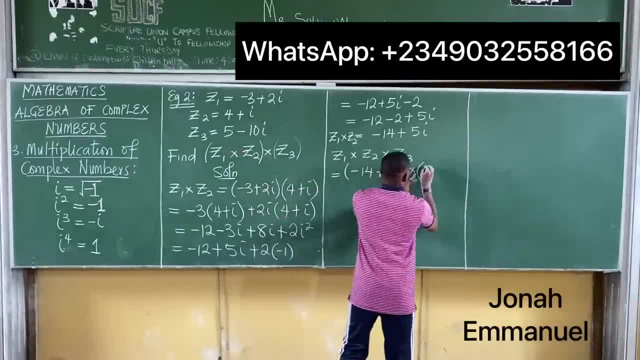 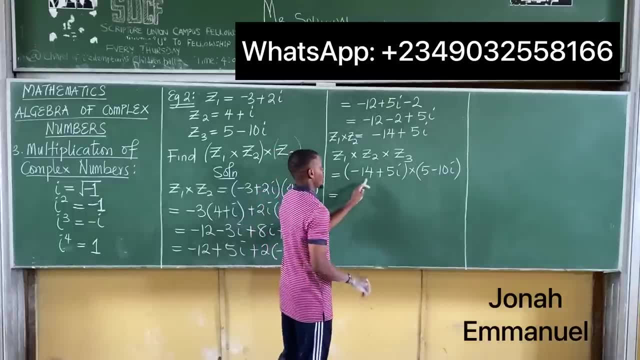 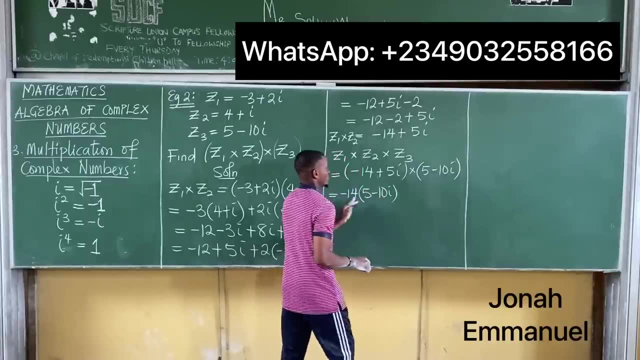 multiplied by the result of z3, that's 5 minus 10i. all right, so we go again. that's equal to first term here minus 14,. i everything here: 5 minus 10i. second, 10 here. 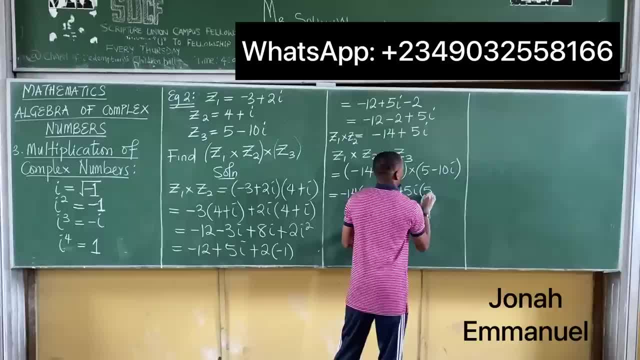 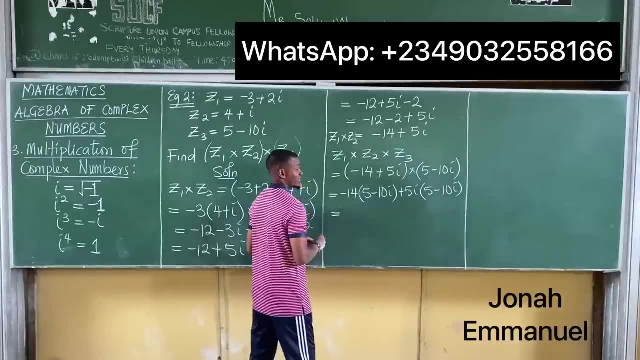 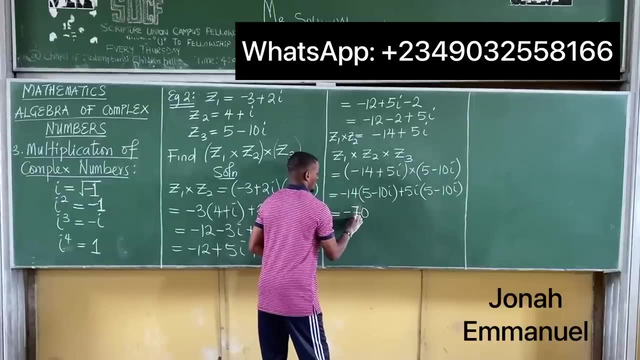 plus 5i. multiply everything here: 5 minus 10i. this is equal to: if i multiply this 14 times 5, i'm having minus 70,. okay, so minus 14 times 5, minus 70,. 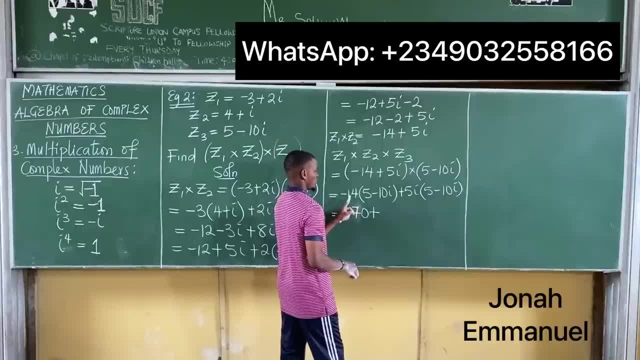 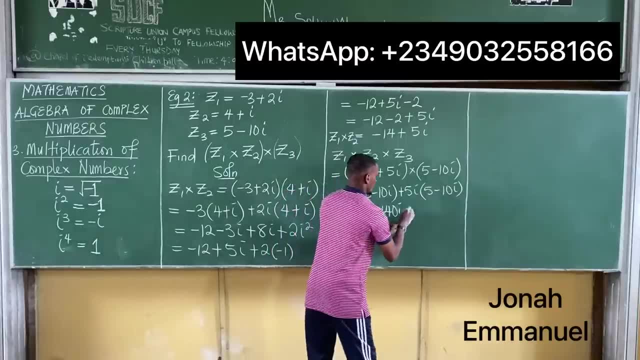 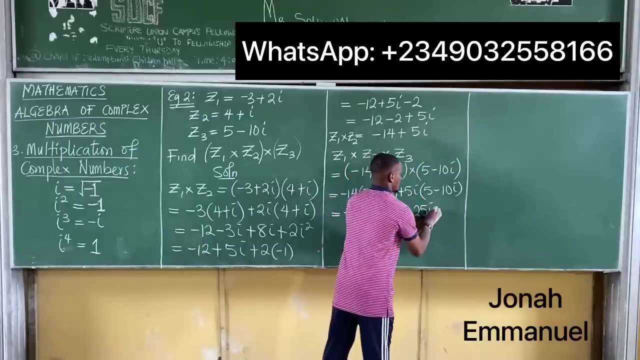 minus minus is plus minus 14, so minus minus is plus 14 times 10 is 140i. plus plus is plus 5 times 5,. 25i plus minus is minus 5 times 10 is 50,. i times i is i squared, so I have this: 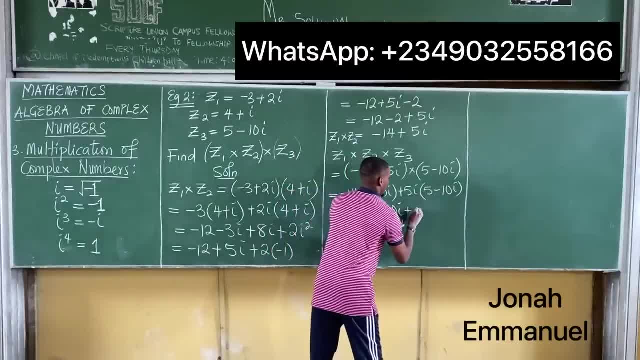 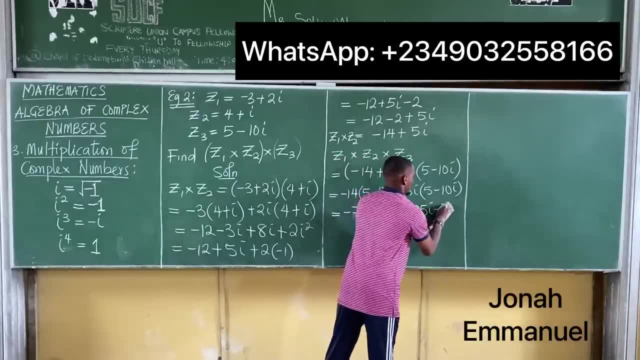 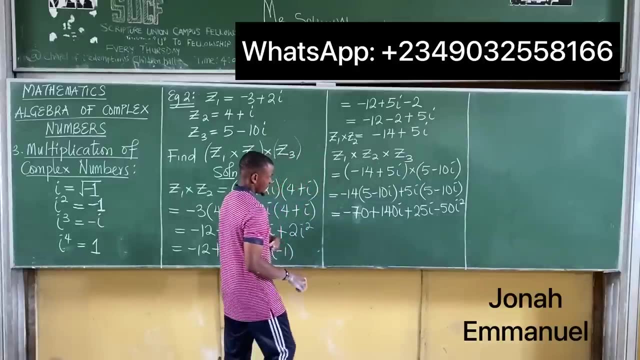 plus plus is plus 5 times 5,. 25i plus minus is minus 5 times 10 is 50,. i times i is i squared, so I have this Okay, so this is equal to minus 70,. 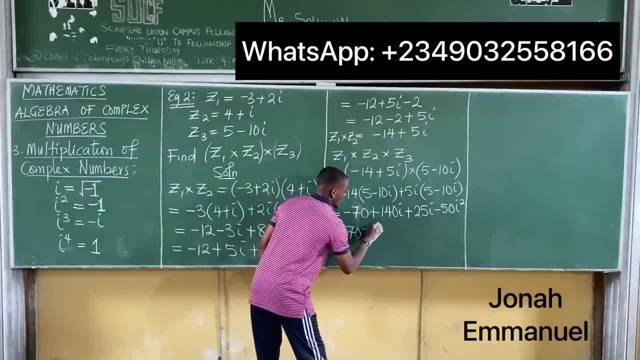 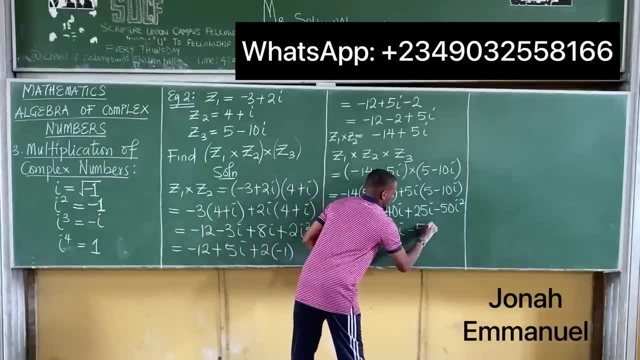 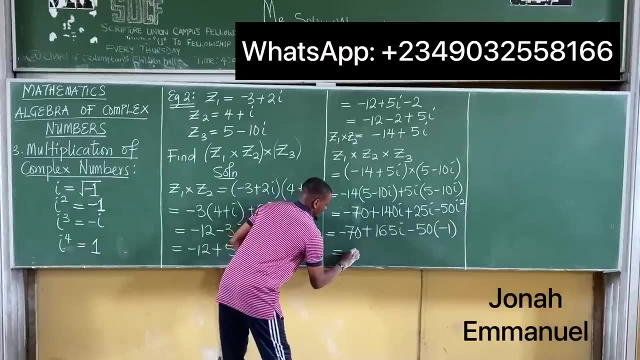 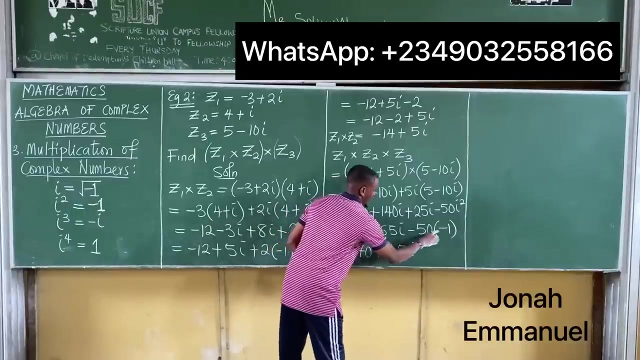 140 plus 25 is plus 165i, minus 50 into i squared, we said is minus 1, so this is equal to minus 70,, plus 165i, minus minus, plus I have 50.. 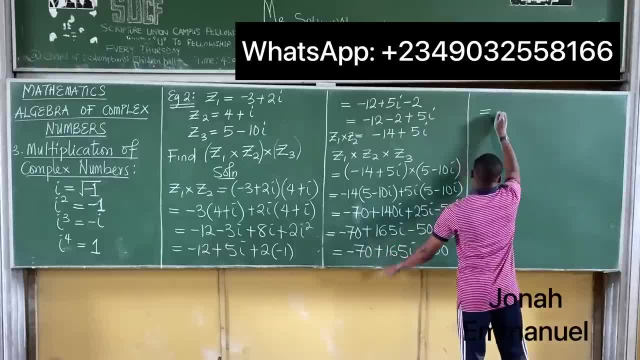 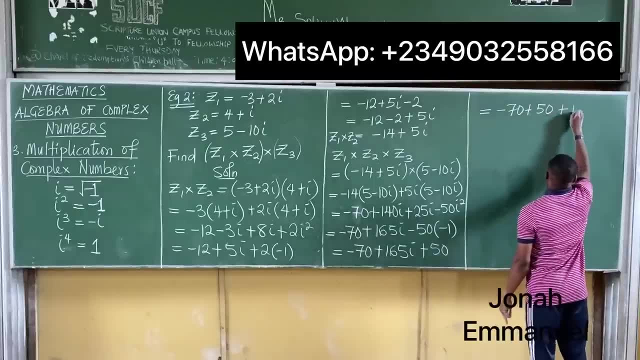 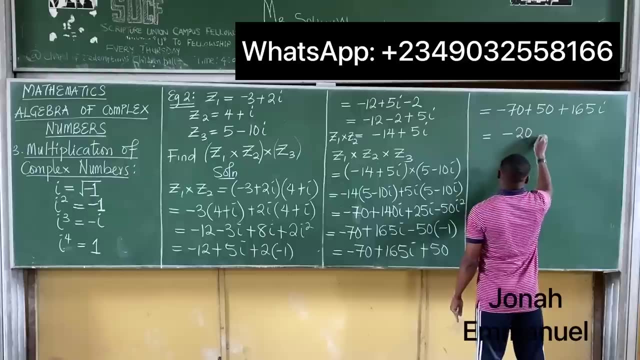 Separating the real part from the imaginary part. my real parts are minus 70, and plus 50,. imaginary part is plus plus 165i, and that's equal to minus 7 plus 50, is minus 20 plus. 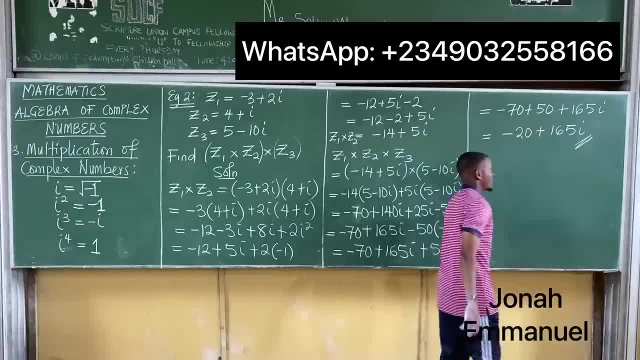 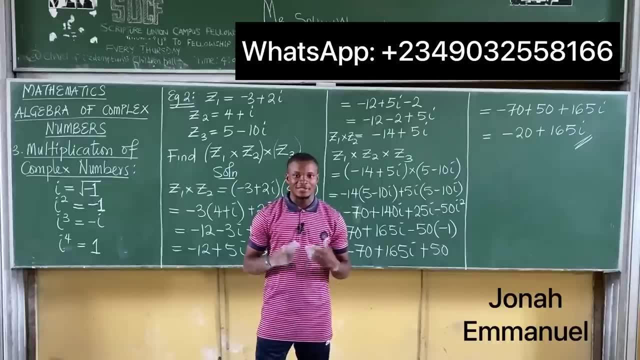 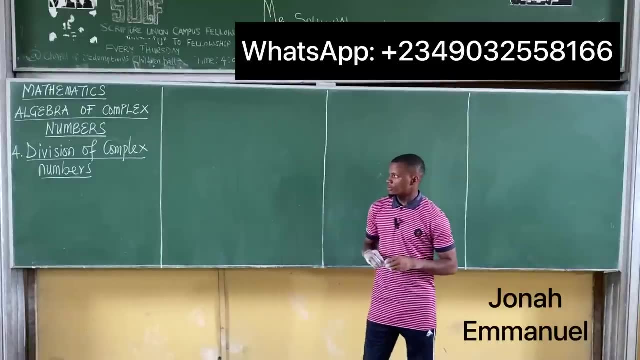 165i. That's my answer. So this is how you do multiplication of complex numbers. Finally, we now look at the division of complex numbers. Alright, so let's look at the fourth one, called division of complex numbers. Now, when it comes to dividing complex numbers, 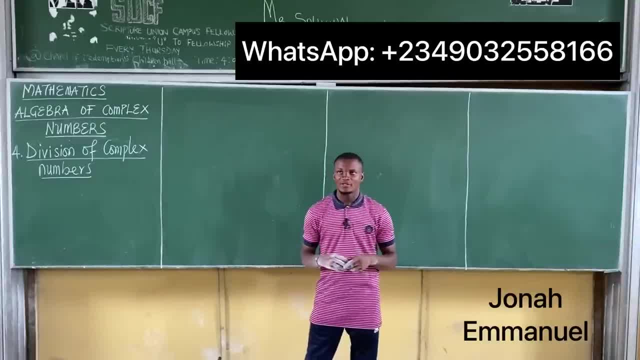 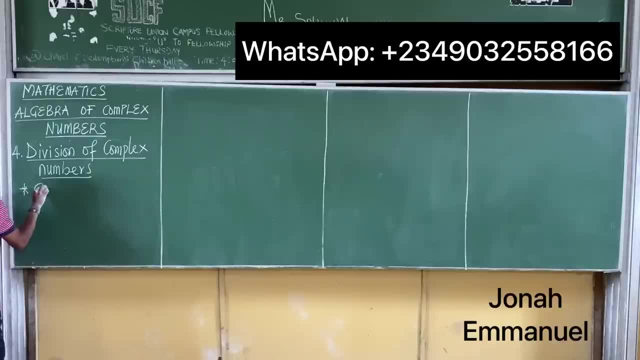 before you do a division of complex numbers, you have to have an idea of what is called the conjugate of a complex number. Let's look at, let's consider something called conjugate first, before we dive into the division of complex numbers. 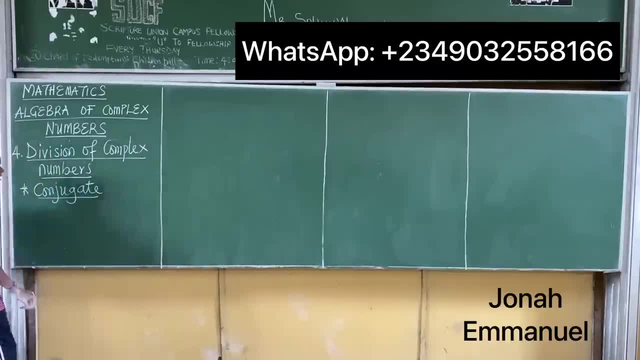 Let's look at the conjugate of a complex number. Now, given a complex number, z being equal to a plus ib, the conjugate of this complex number, z, is written as z bar, alright, so z with a bar on the head. 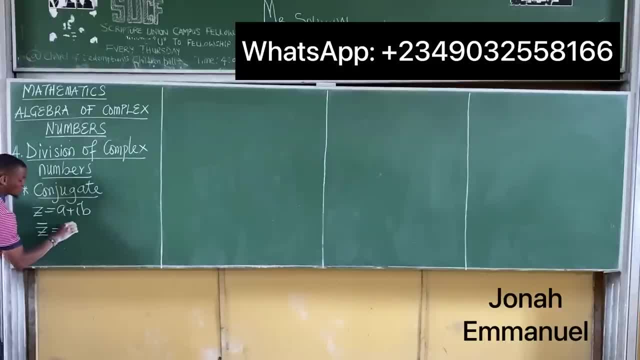 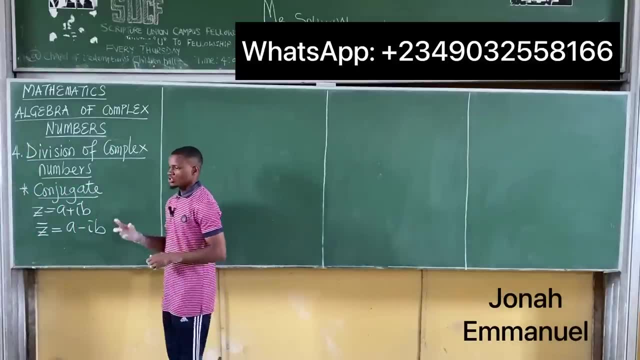 alright, z bar and z bar. the conjugate is equal to a minus ib. So when it comes to getting conjugate, the idea is simply: I'm going to change the sign of the imaginary part only to the opposite sign. 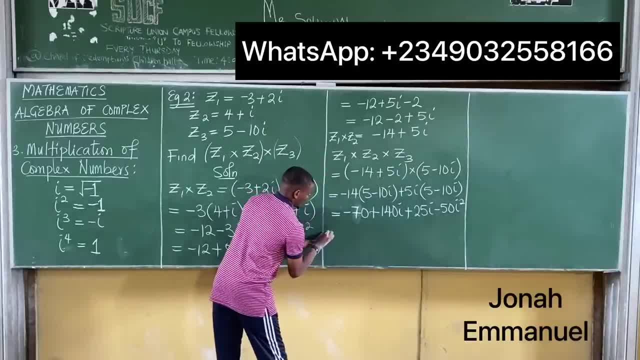 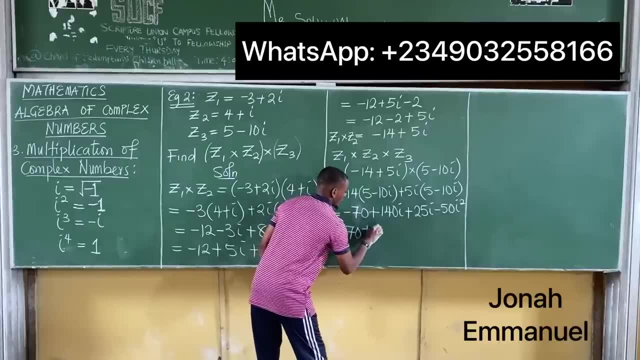 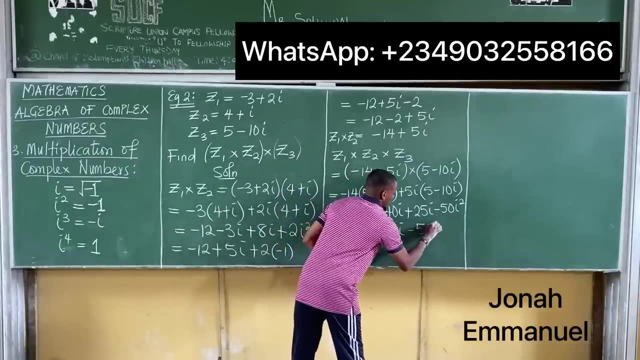 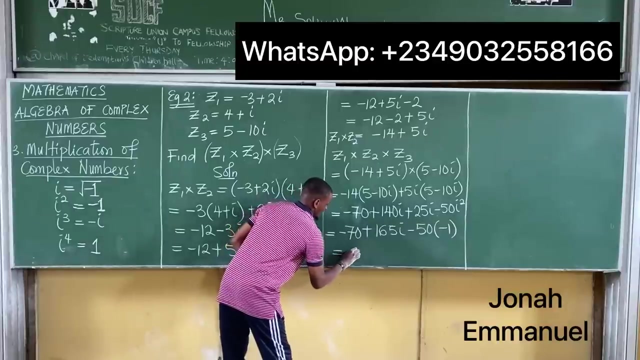 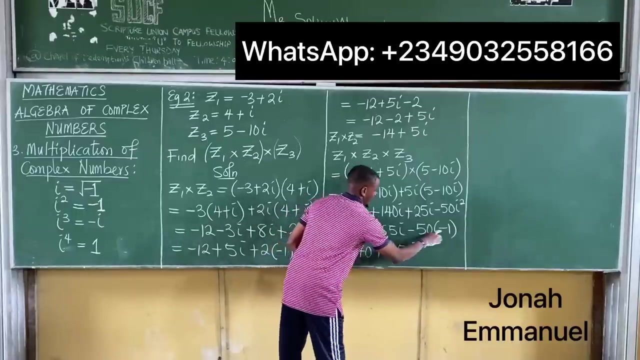 Okay, so this is equal to minus 70, 140 plus 25 is plus 165i minus 50 into i squared, we said is minus 1, so this is equal to minus 70 plus 165i. Minus minus plus, I have 50.. 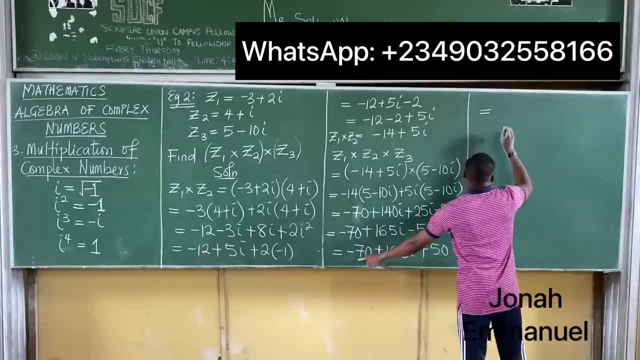 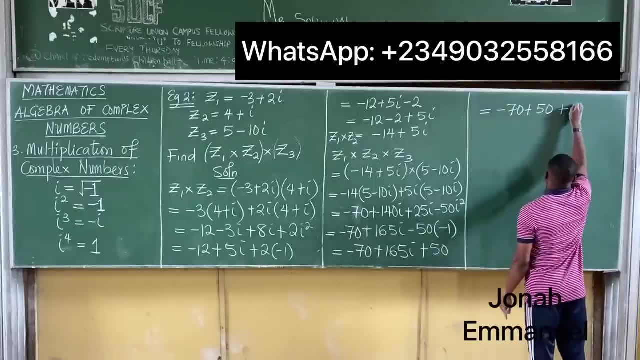 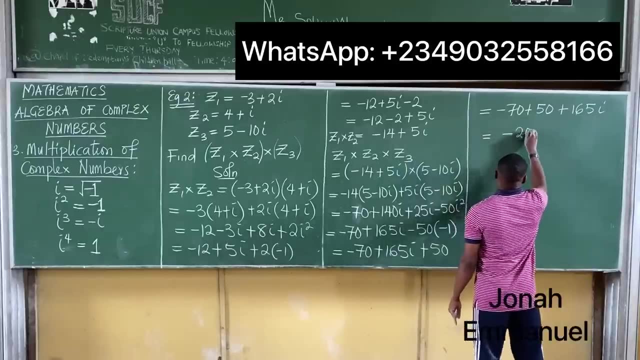 Separating the real part from the imaginary part. my real parts are minus 70 and plus 50, imaginary part is plus 165i and that's equal to minus 7 plus 50 is minus 20 plus 165i. That's my answer. 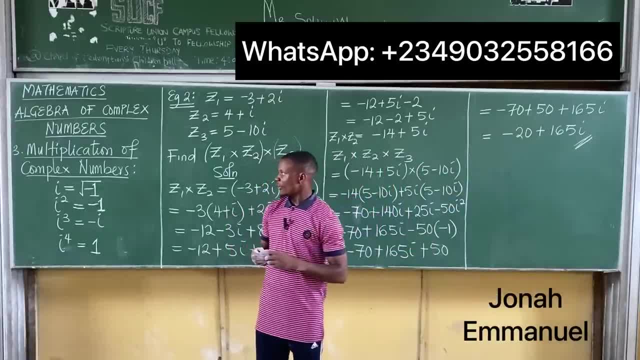 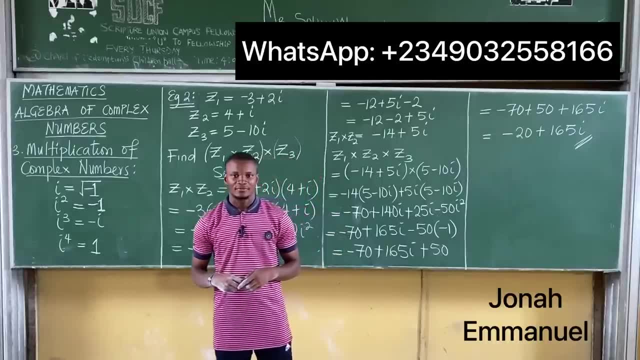 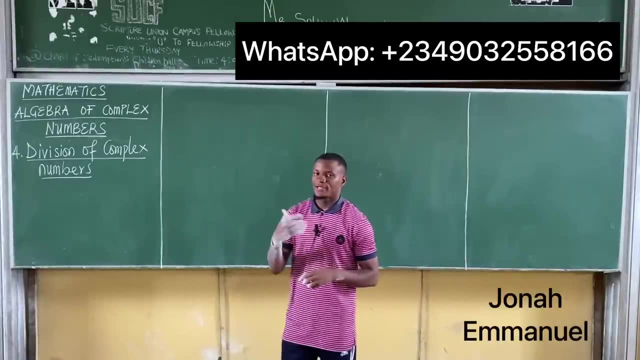 So this is how you do multiplication. Finally, we will now look at the division of complex numbers. Alright, so let's look at the fourth one, called division of complex numbers. Now, when it comes to dividing complex numbers, before you do a division of complex numbers, 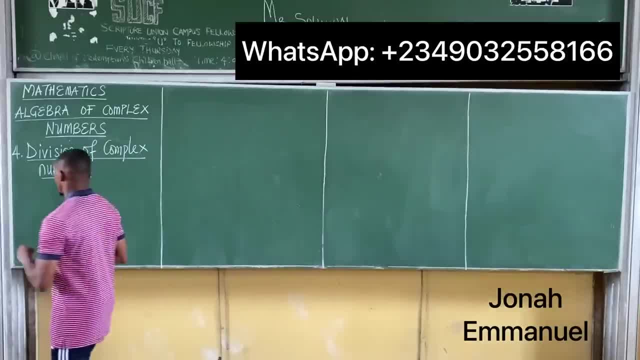 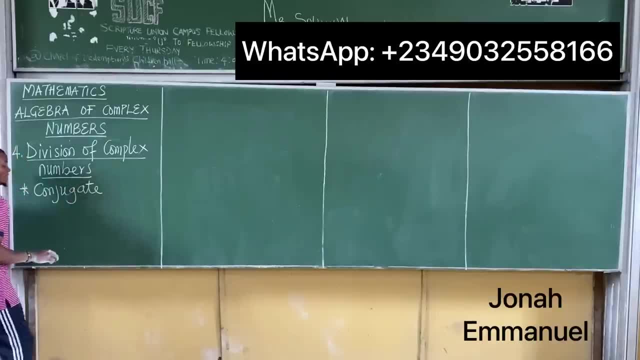 you have to have an idea of what is called the conjugate of a complex number. So let's look at, let's consider something called conjugate first, before we dive into division of complex numbers. Let's look at the division of complex numbers, what is called the conjugate of a complex 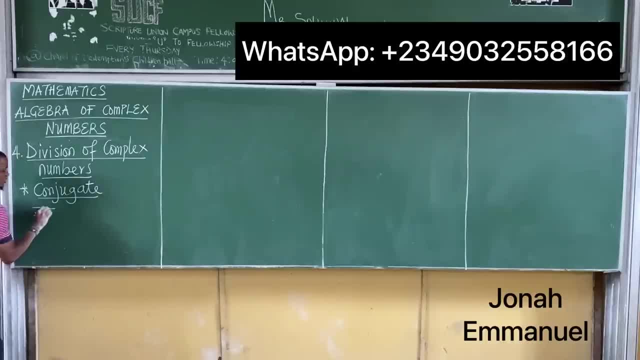 number. Now, given a complex number, z being equal to a plus ib, the conjugate of this complex number z is written as: z bar, alright so z with a bar on the head, alright z bar and z bar. the conjugate is equal to a minus ib. 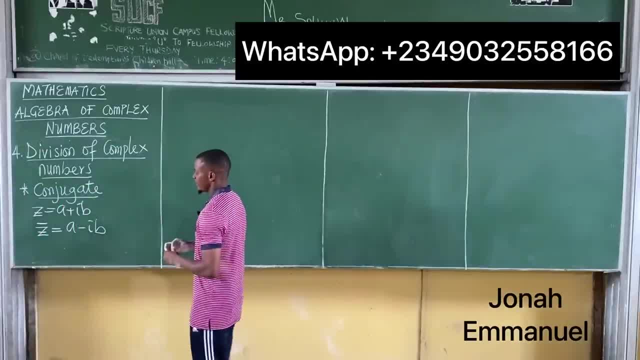 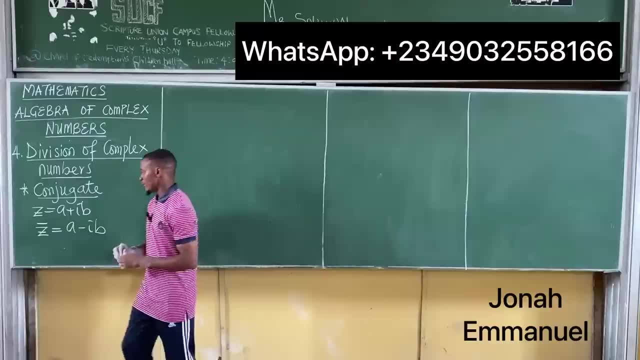 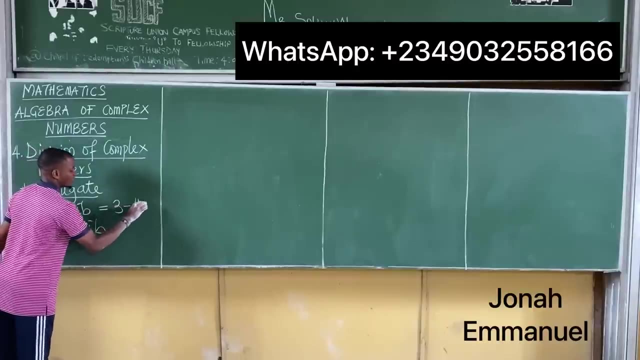 So, when it comes to getting conjugate, the idea is simply: I'm going to change the sign, the sign of the imaginary part, only to the opposite sign. So hence, let's say z, let's say z is equal to, let's say, 3 minus 4i. I will have that. 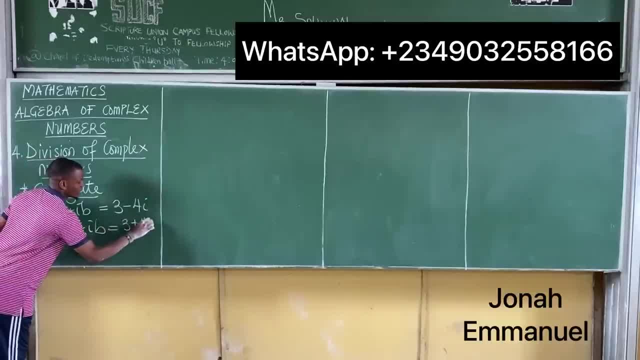 z bar is equal to 3 plus 4i. I am only changing the sign of the imaginary part. Finally, if z is equal to, let's say, minus 3 minus i, Alright, Having this in mind, let's see how we do division of complex numbers. 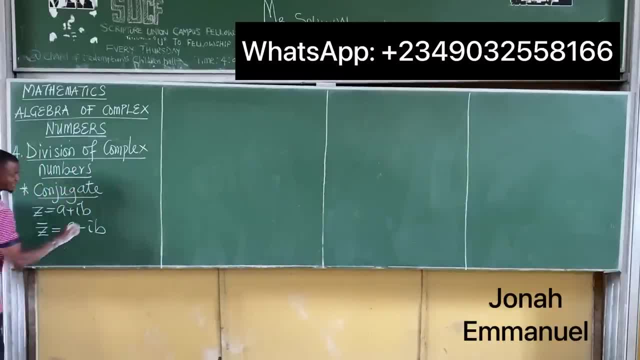 So hence, let's say z. let's say z is equal to, let's say, 3 minus 4i. I will have that z bar is equal to 3 plus 4i. I am only changing the sign. 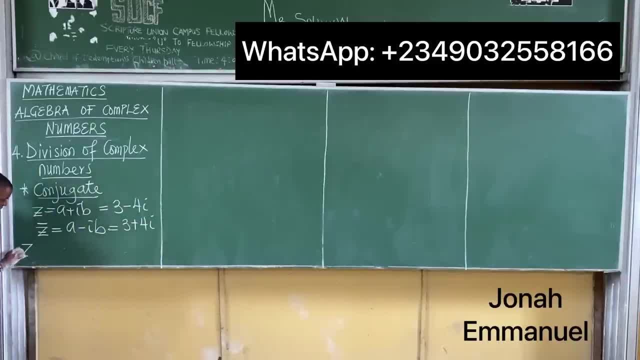 of the imaginary part. Finally, if z is equal to, let's say, minus 3, minus i, we'll have that z bar which is the conjugate of this. So let's call this z asterix. 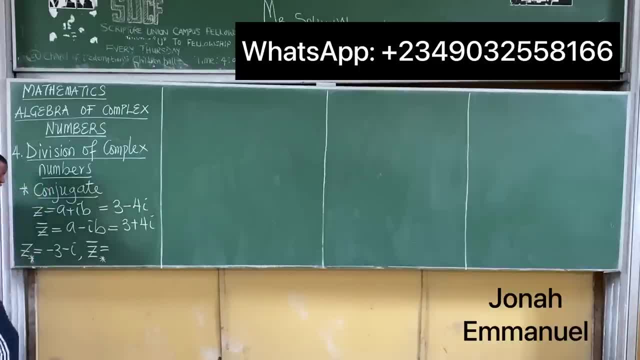 we'll separate this on here. So z asterix bar will be equal to minus 3, minus 3, plus i. So please take note that when it comes to changing, when it comes to conjugate, I am only changing the sign. 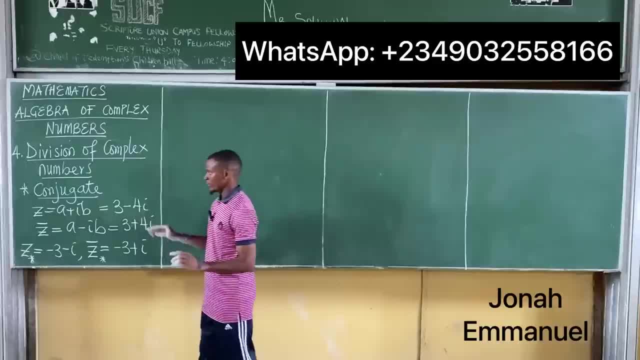 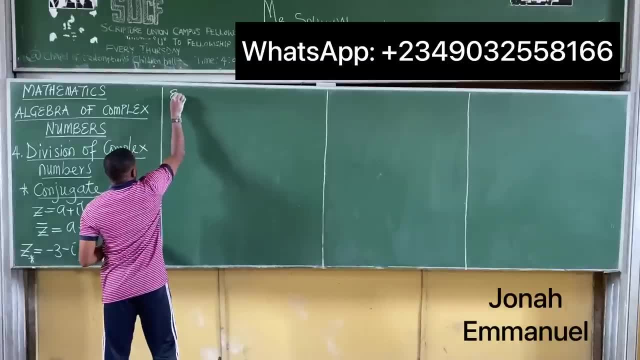 of the imaginary part, The ray part is left the same way. Alright, having this in mind, let's see how we do division of complex numbers. We'll take an example and explain this. Let's say I have 3 plus 2i. 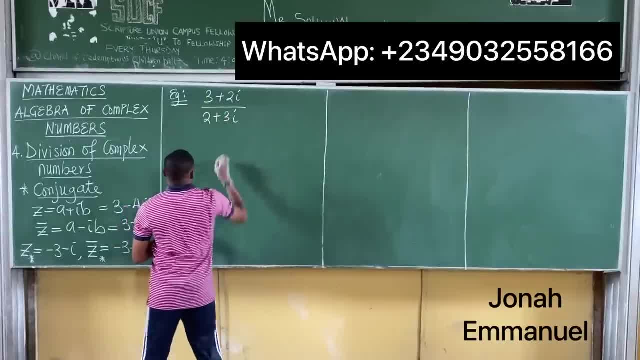 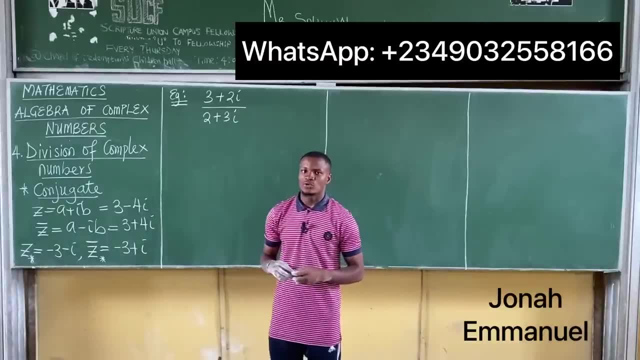 dividing 2 plus 3i. So this is um a division of complex numbers. The idea is this: it is improper to leave a denominator of a fraction as a complex number. It's not proper. So in cases like this, 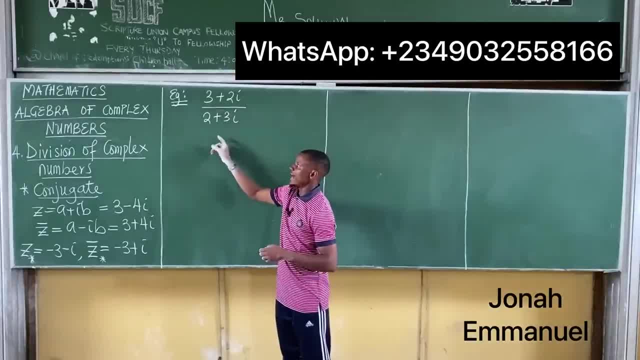 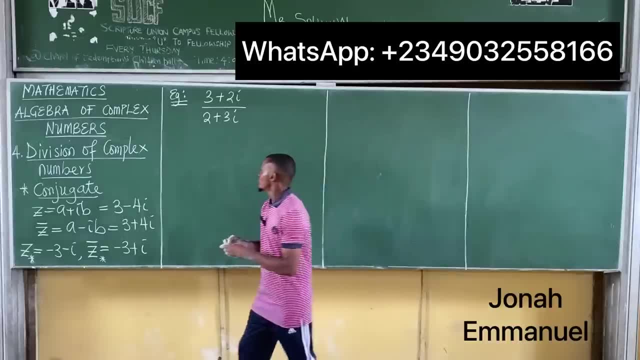 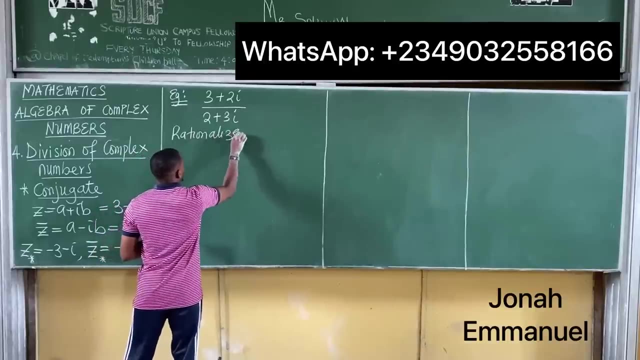 where I have the denominator of a fraction as a complex number. what do I do? I'll have to rationalize. Just like the same ideas with sorts, So I'll have to rationalize, um rationalize. What do I mean by rationalization? 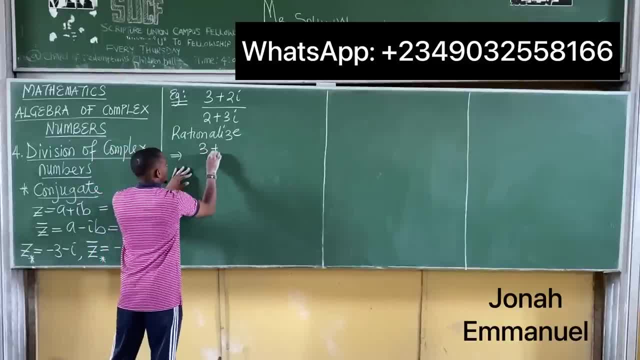 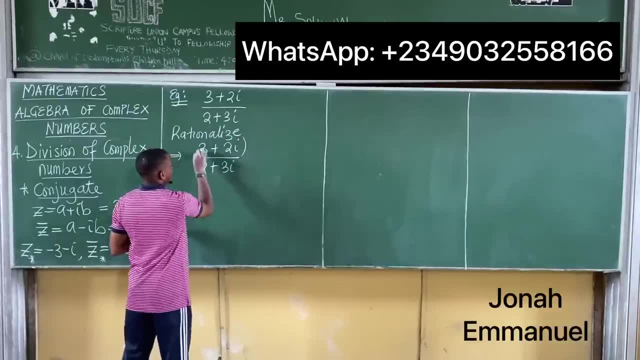 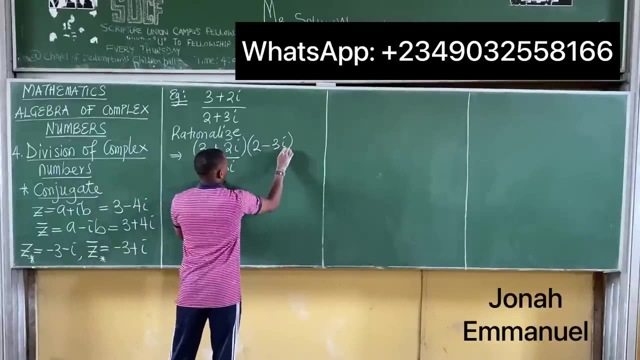 For rationalization, I'm multiplying numerator and denominator by the conjugate of the denominator, So it becomes numerator. that's this multiplied by the conjugate of denominator 2, this becomes minus 3i. 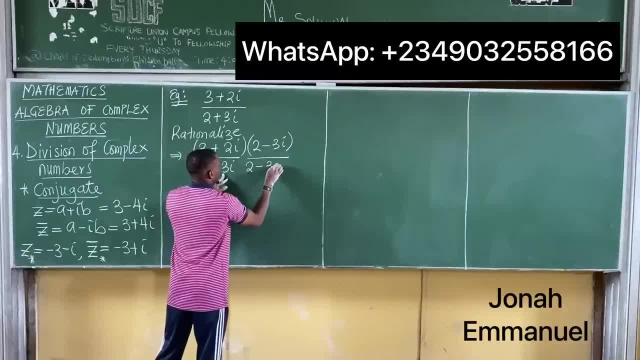 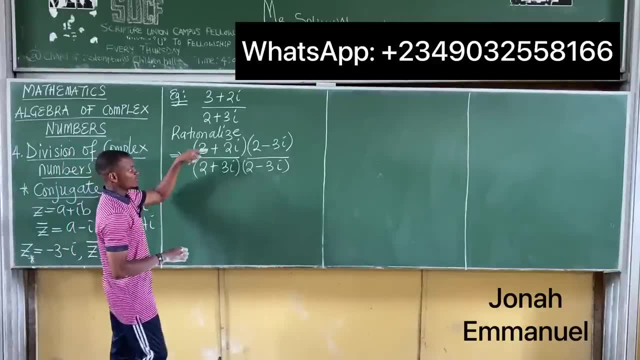 Do the same thing here, it becomes 2, minus 3i. So this is what is called rationalization of um complex numbers. Multiply numerator and denominator by the conjugate of denominator, So 2,. 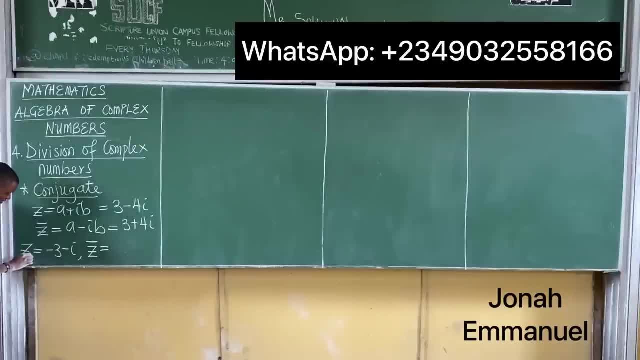 So when you have z bar, which is the conjugate of this, let's call this z asterix, so separate this on here. so z asterix bar will be equal to minus 3 plus i. So please take note that when it comes to conjugate, I am only changing the sign of. 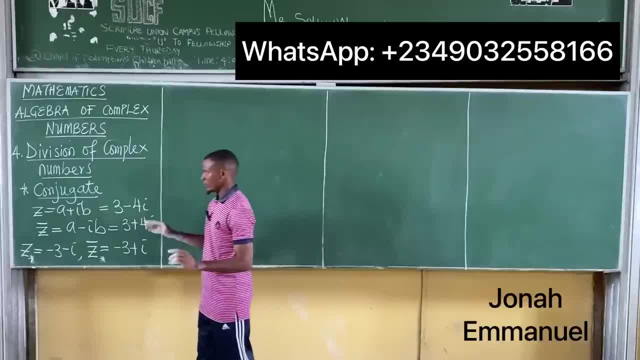 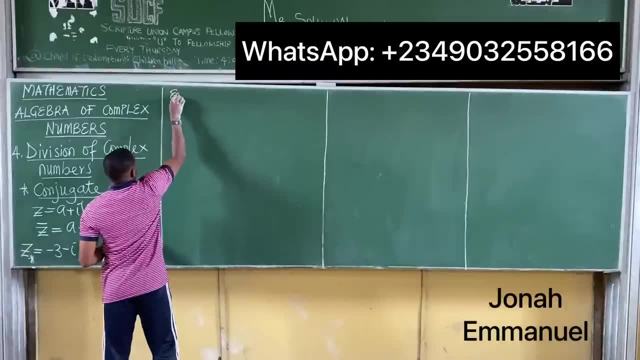 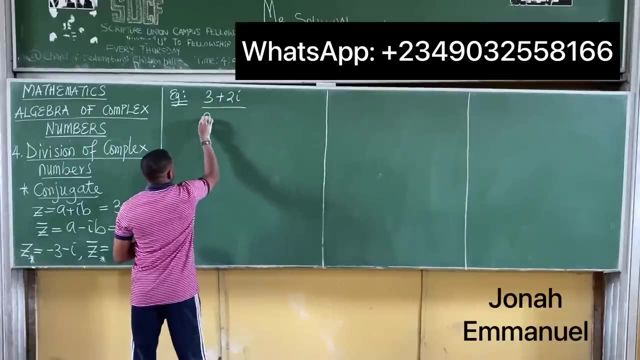 the imaginary part, The ray part, is left the same way. Alright, Having this in mind, let's see how to do division of complex numbers. Let's see how we do division of complex numbers. Alright, we'll take an example and explain this. Let's say I have 3 plus 2i, dividing 2 plus 3i. So 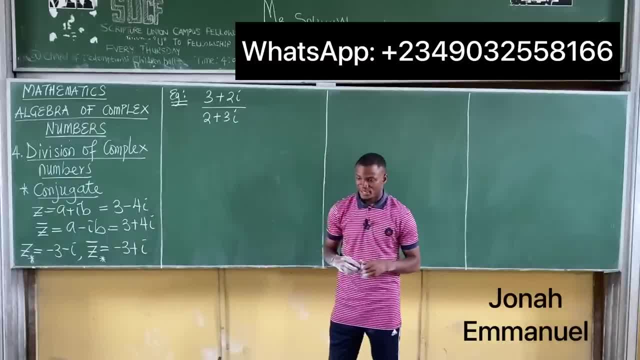 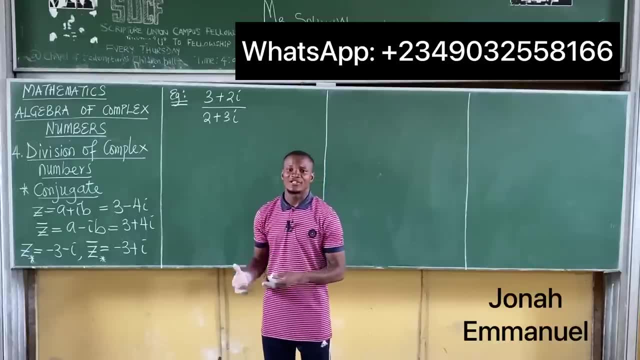 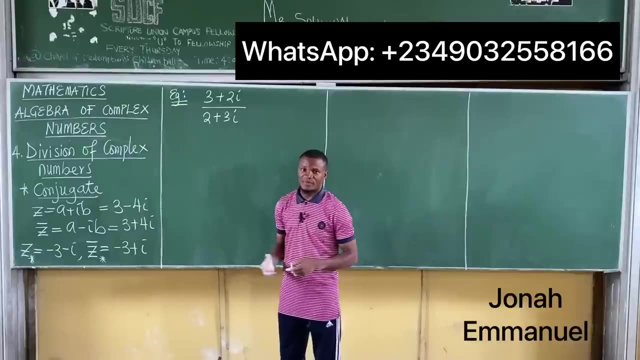 this is a division of complex numbers. The idea is this: It is improper to leave a denominator of a fraction as a complex number. It's not proper. So in cases like this, where I have the denominator of a fraction as a complex number, what do I do? I'll have to rationalize. 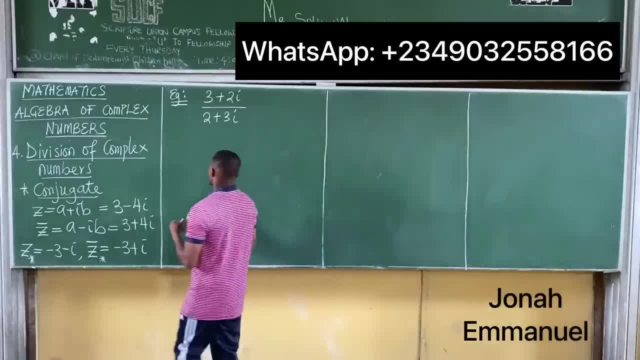 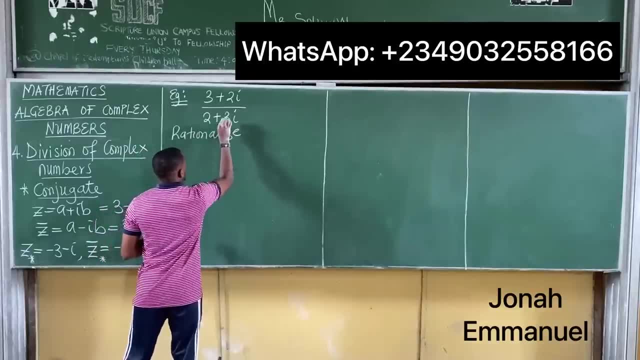 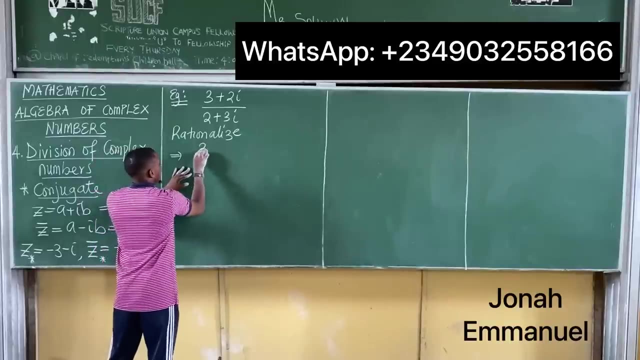 just like the same ideas with sorts. So I'll have to rationalize. What do I mean by rationalization? For rationalization, I'm multiplying numerator and denominator by the conjugate of the denominator. So I'm multiplying numerator and denominator by the conjugate of the denominator. So 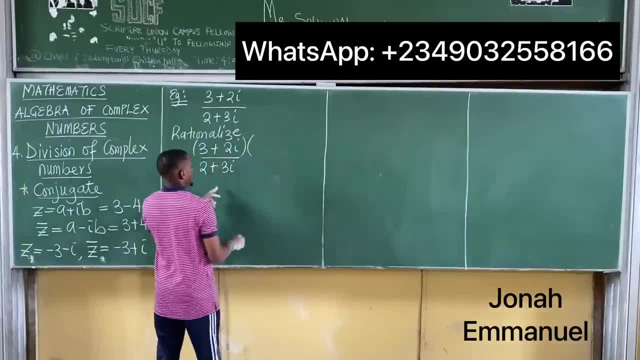 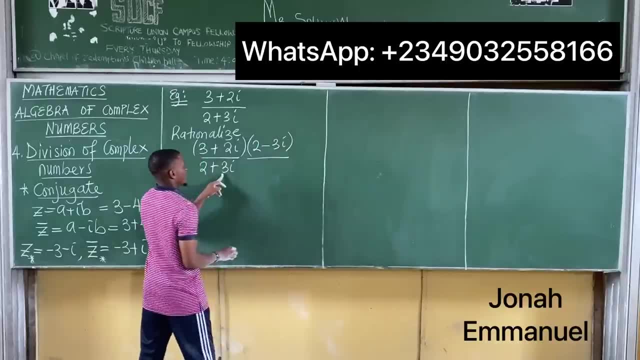 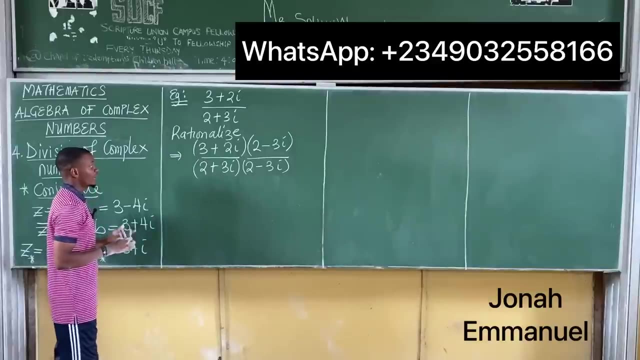 it becomes numerator. That's this multiplied by the conjugate of the denominator. So this becomes minus 3i. Do the same thing here: It becomes 2 minus 3i. So this is what is called rationalization of complex numbers. Multiply numerator and denominator by the. 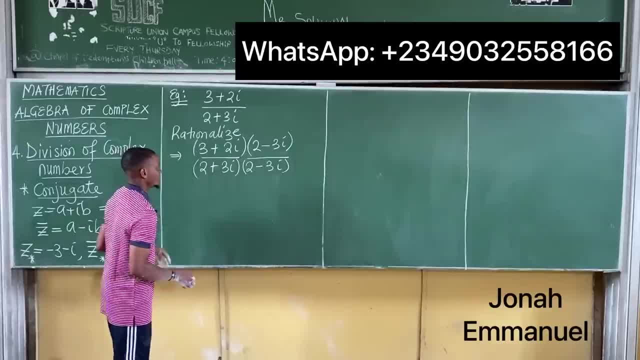 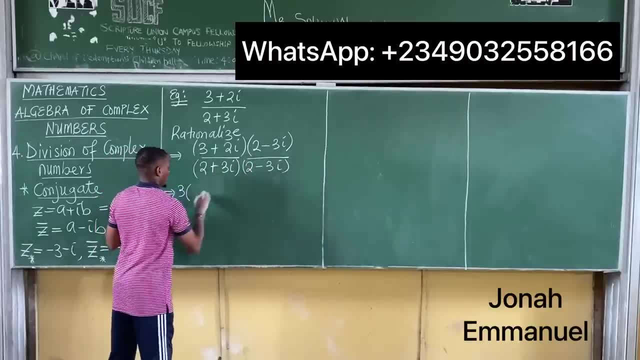 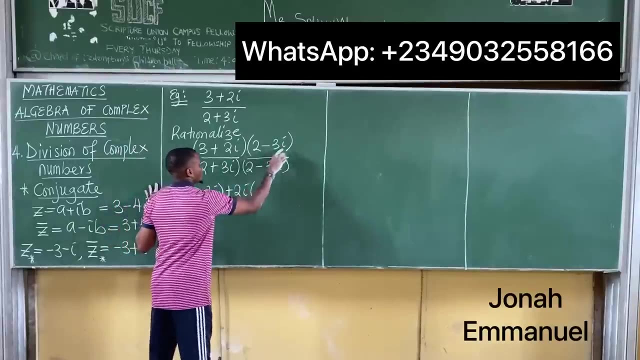 conjugate of the denominator So, 2 minus 3i. I have this. So multiply this. What do I do? Take this first time. So next term, this one. next term comes, Then top is, as usual, the 2-3 and 3, both side alsobij. therefore they are half so b and both are half o, and 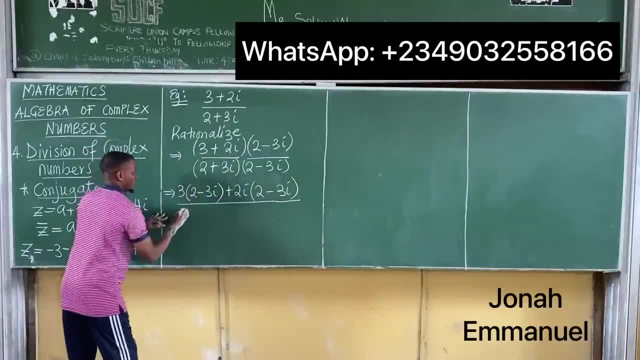 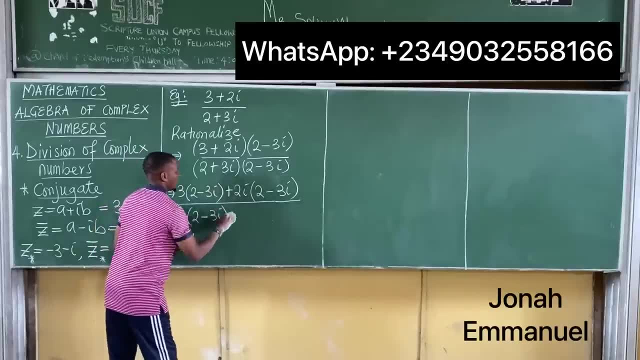 both are wonderful. b? y are not just the same thing. I'll have to rationalize them ultimately. So, just like this, after completing all the equations, we're starting to be정이 leg. Mortal Galactic law. The Un cama facultium. 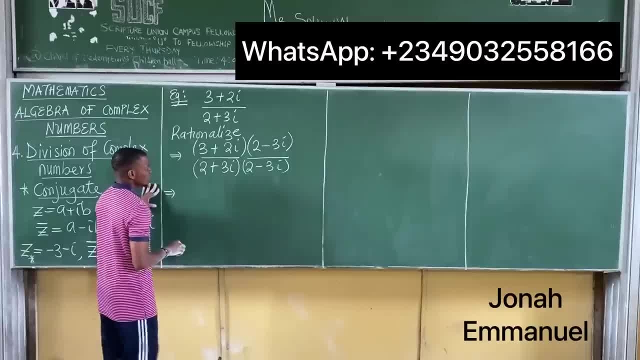 minus 3i. I have this, So multiply this, what do we have? This will give you first 10 here, 3,. multiply everything here: 2, minus 3i. Second, 10 here plus. 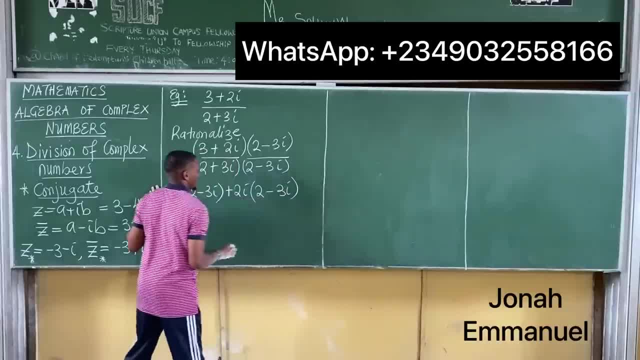 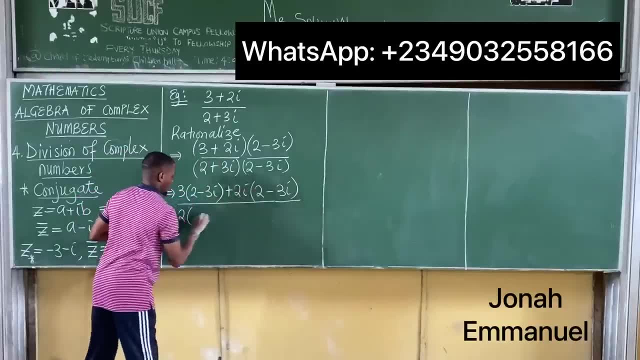 2i. Multiply everything here 2, minus 3i. All over: first, 10 here 2,. multiply everything here, 2, minus 3i. Second, 10 here plus 3i. 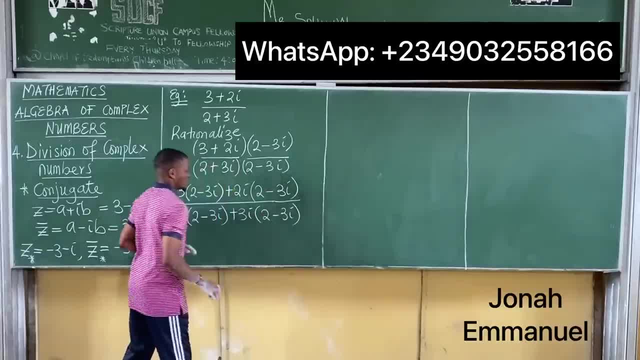 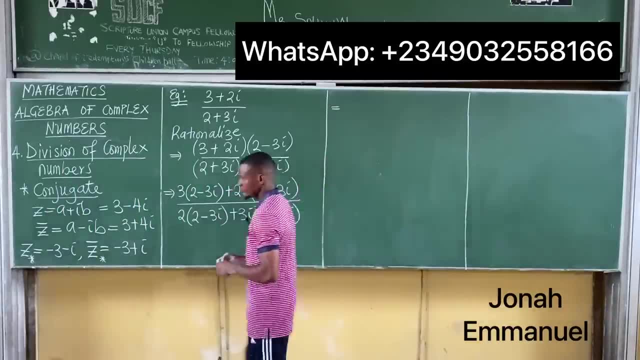 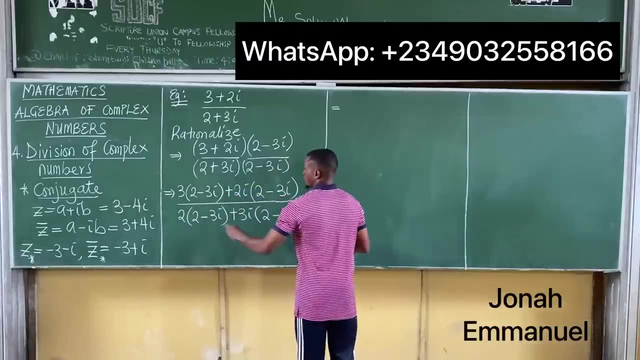 Multiply everything here: 2, minus 3i, So I have this. Alright, let's expand this and see what we have. This will be equal to: so that's equal to 3 times 2, is 6.. 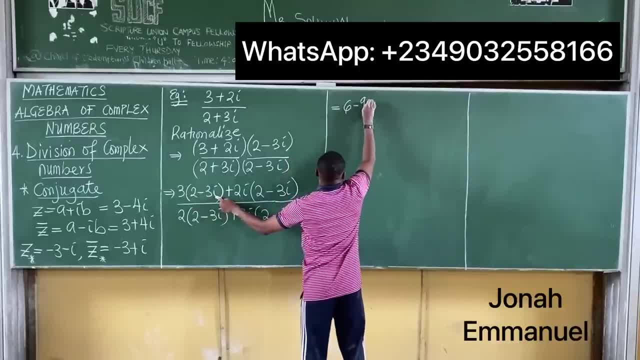 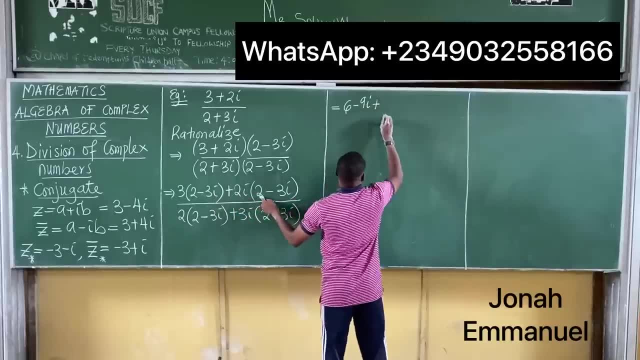 3 times minus 3i minus 9i. So 3 times minus 3 is minus 9.. Bring down the i Plus 2 times 2, is 4.. Bring down the i Plus times minus. 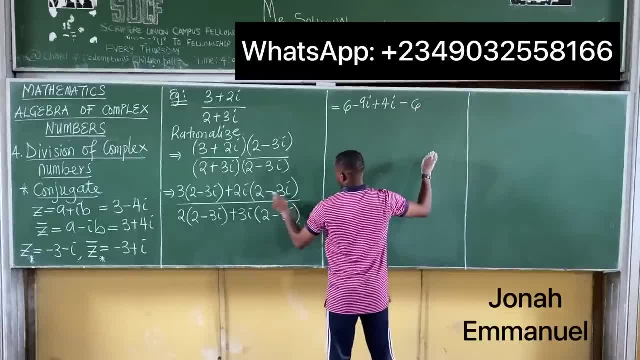 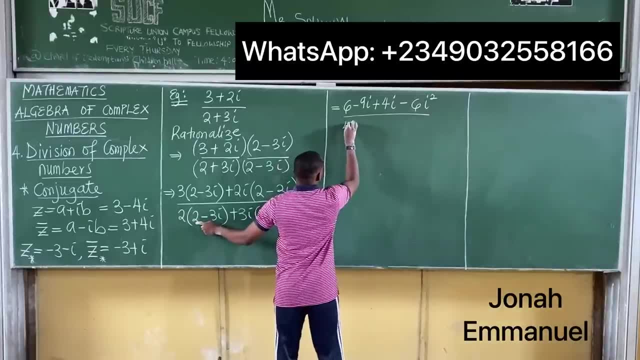 is minus 2 times 3, is 6.. i times i is i squared All over 2 times 2, is 4.. 2 times minus 3, is minus 6i. Okay, Plus 3 times 2,. 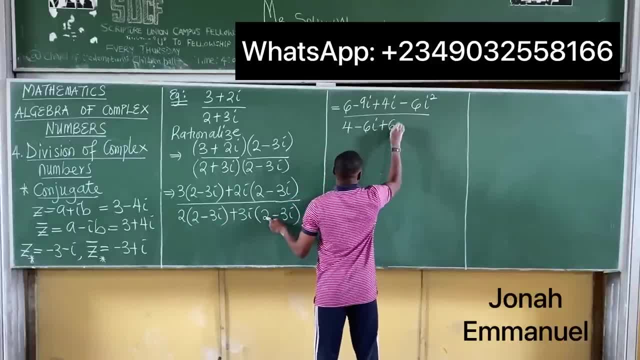 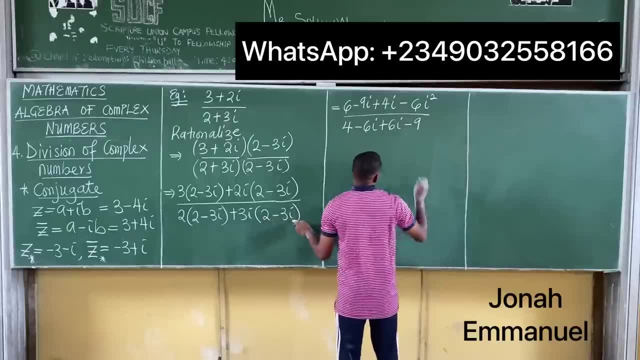 is plus 6i. Plus times minus is minus 3. times 3, is 9.. i times i is i squared, So work this out. This is equal to I'm having 6, minus minus 9i. 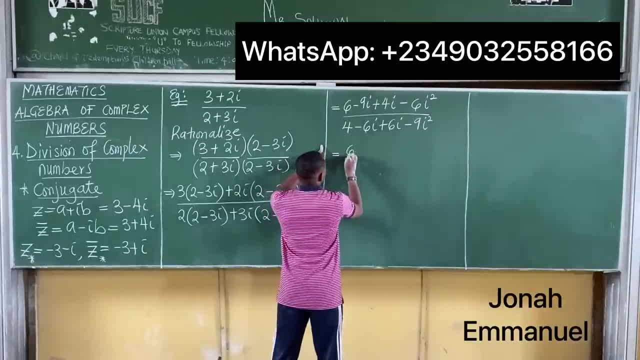 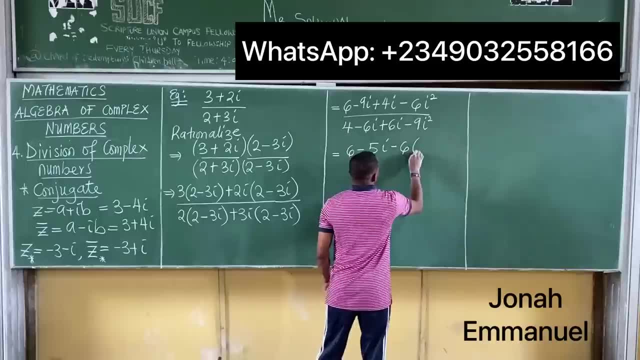 plus 4i gives you minus 5i minus 6, into i squared. We said is minus 1.. So 3 times 2, is plus 6i Plus is minus 1.. 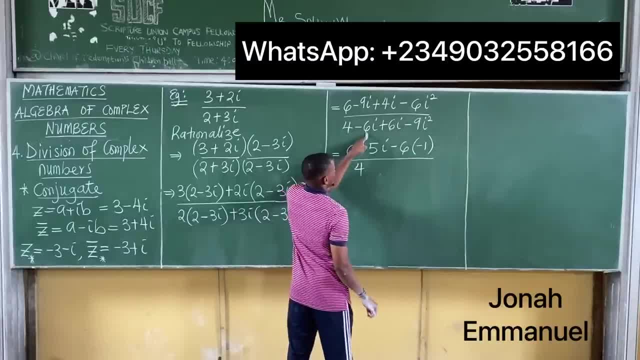 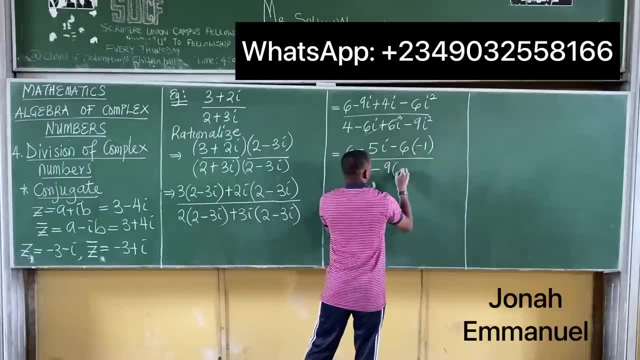 All over. I'm having here is 4, minus 6i plus 6i will cancel out. That will give you 0.. I'm left with minus 9i. squared is minus 1.. So this will be equal to. 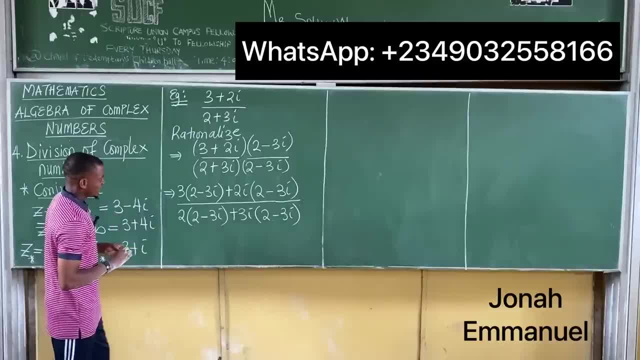 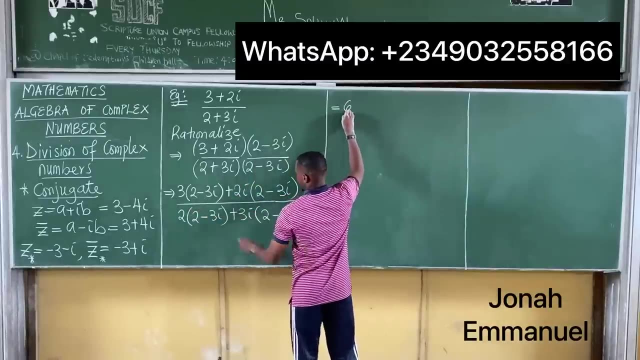 minus 3i. So I have this. Alright, let's expand this and see what we have. This will be equal to: so that's equal to: 3 times 2 is 6.. 3 times minus 3i minus 9i. so 3 times minus 3 is minus 9,. 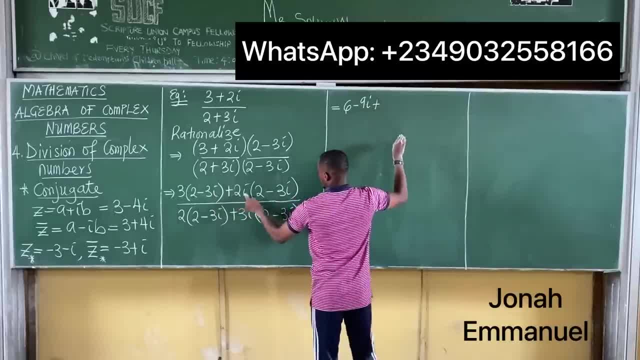 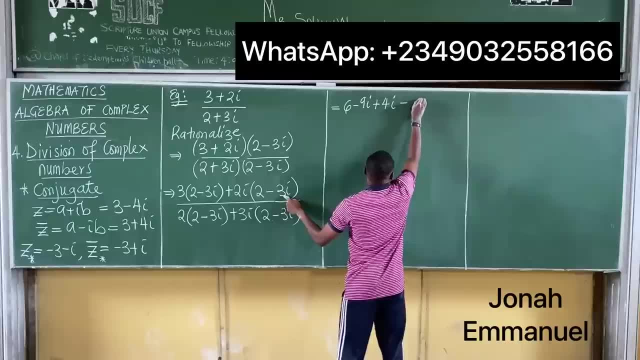 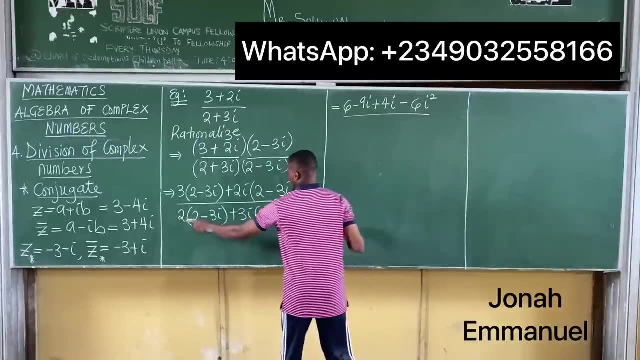 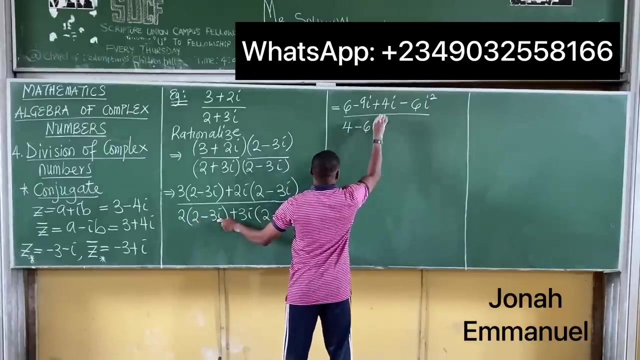 bring down the i plus 2 times 2 is 4,. bring down the i plus times minus is minus 2 times 3 is 6,. i times i is i squared all over. 2 times 2 is 4,. 2 times minus 3 is minus 6i okay. 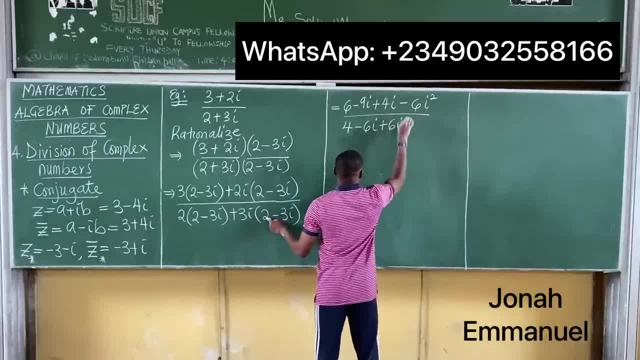 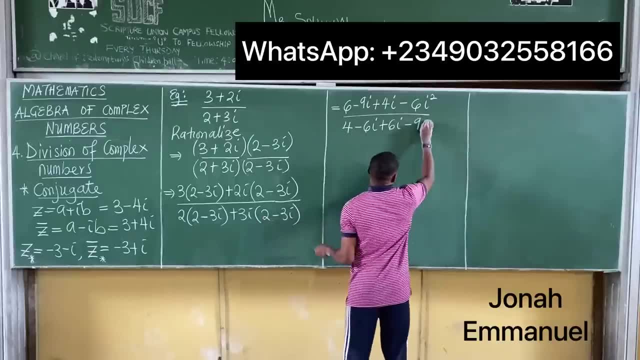 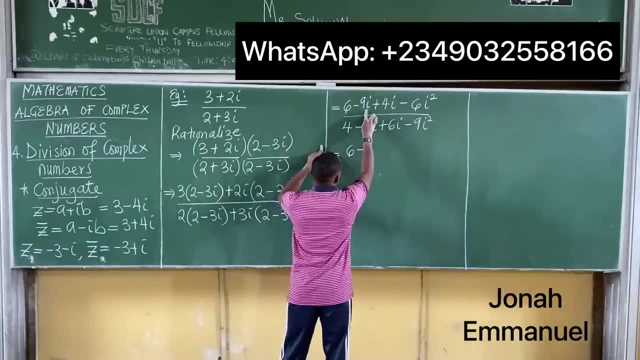 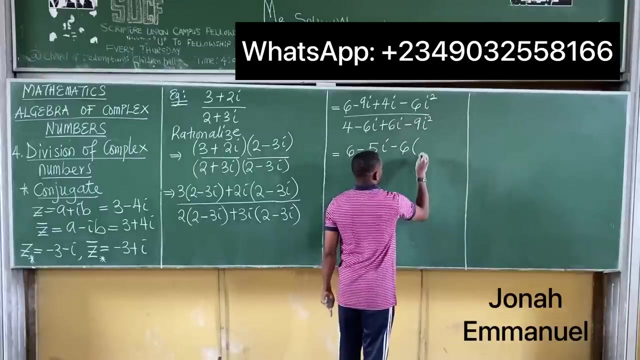 plus 3 times 2 is plus 6i. plus times minus is minus 3. times 3 is 9, i times i is i squared, So work this out. this is equal to I'm having 6 minus minus 9i plus 4i gives you minus 5i minus 6 into i squared. 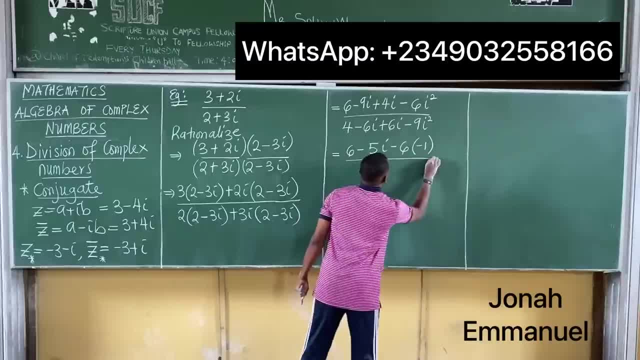 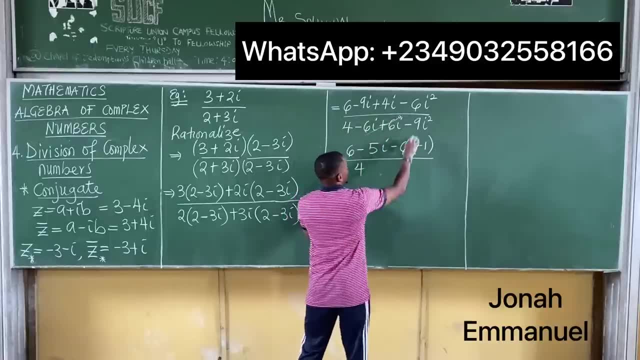 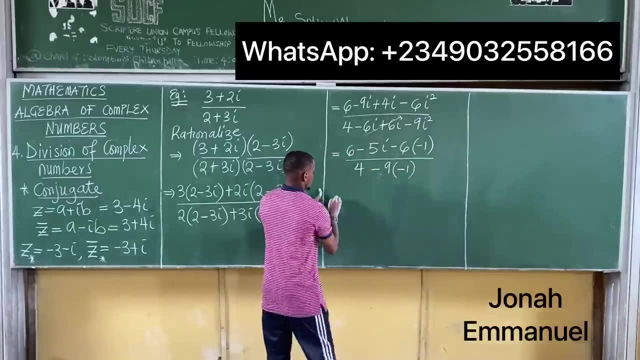 we said is minus 1,. all over I'm having here is 4, minus 6i. plus 6i. we cancel out that will give you 0.. I'm left with minus 9i. squared is minus 1.. So this will be equal to 6 minus 5i. minus minus plus 6,. 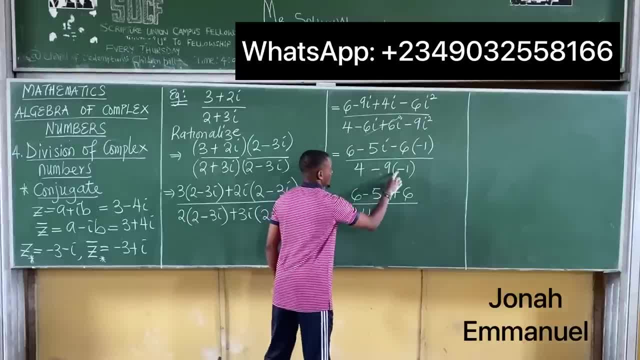 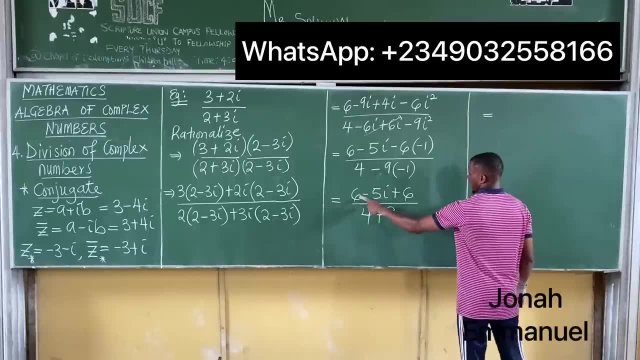 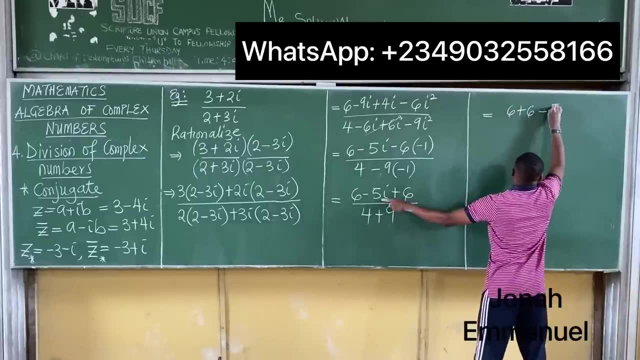 all over. I'm having 4 minus minus, plus 9 times 1, 9.. So this will be equal to: I'm having um: take this and this, that becomes 6 plus 6, and then that's the real part, imaginary part- minus 5i all over 4 plus 9, that's 13.. 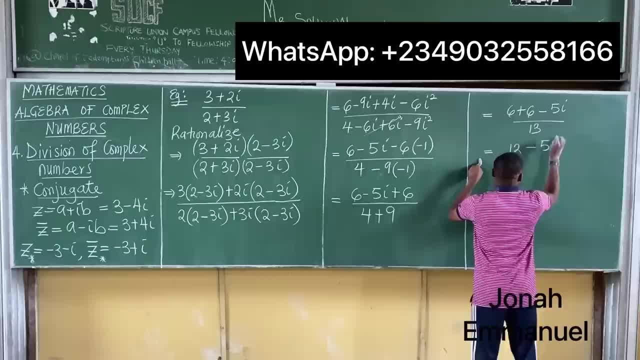 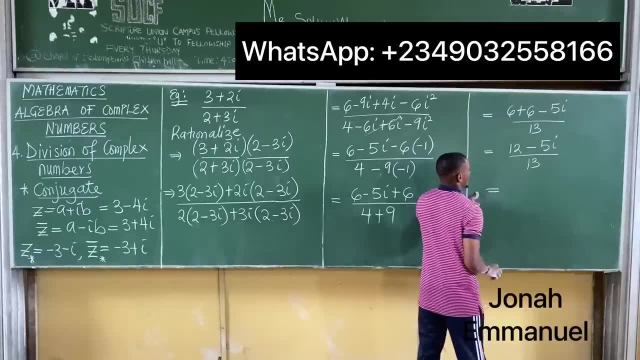 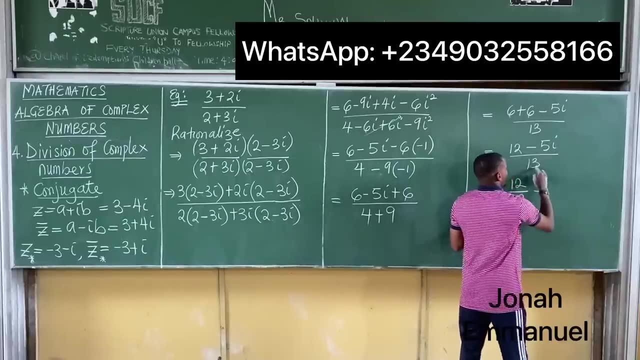 This is equal to 12 minus 5i, all over 13.. So this is my answer. So that means um for this. I will separate them becomes 12 over 13,. so I'm having 12 over 13, minus I'm having 5 over 13,. 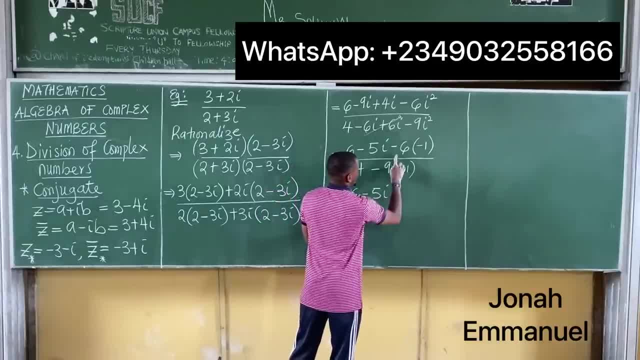 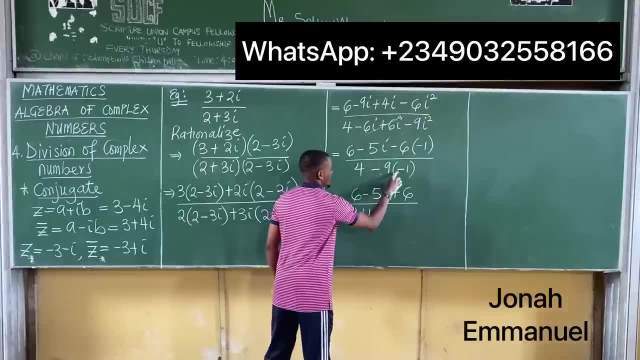 6, minus 5i minus minus plus 6.. All over, I'm having 4, minus minus 9, times 1, 9. So this will be equal to I'm having 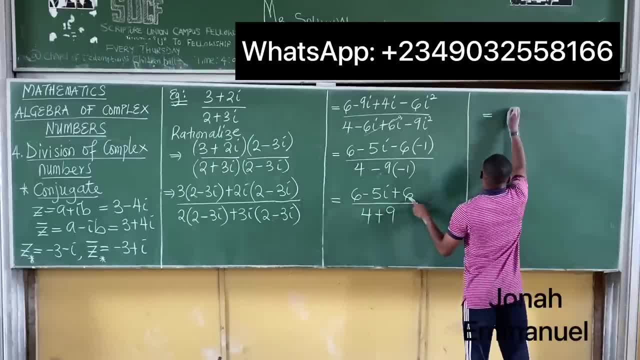 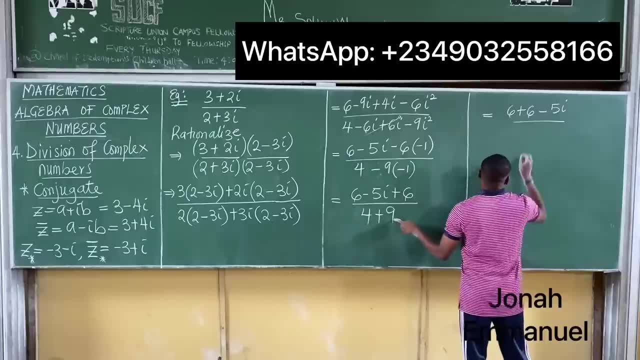 take this and this, that becomes 6, plus 6.. And then that's the real part, imaginary part, minus 5i. all over 4, plus 9, that's 13. This is equal to. 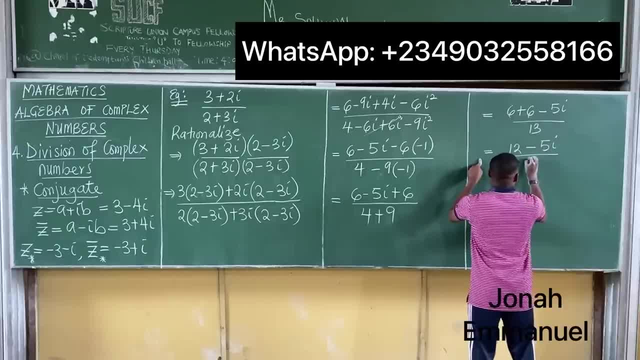 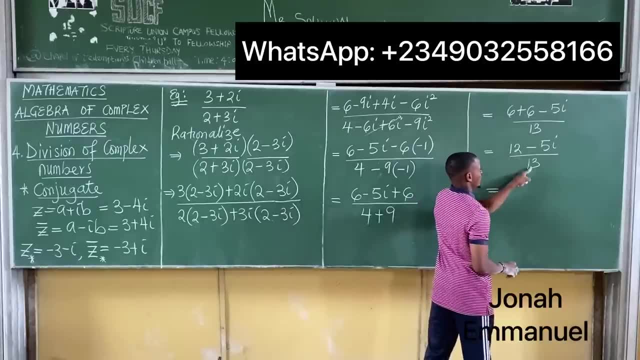 12, minus 5i all over 13.. So this is my answer. So that means for this I will separate them becomes 12, over 13. So I'm having 12, over 13,. 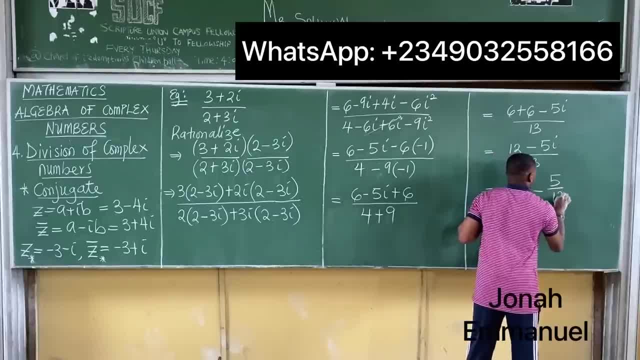 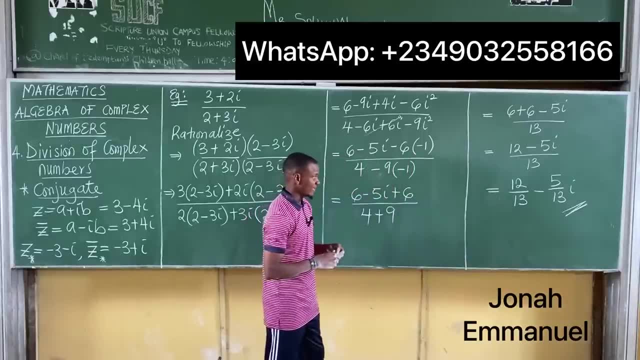 minus, I'm having 5,, over 13,, and then I have i. All right. so this is how we do um um division of complex numbers. So observe that the denominator now is no longer a complex number. 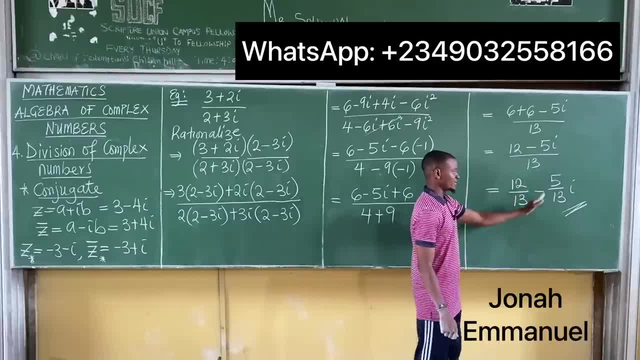 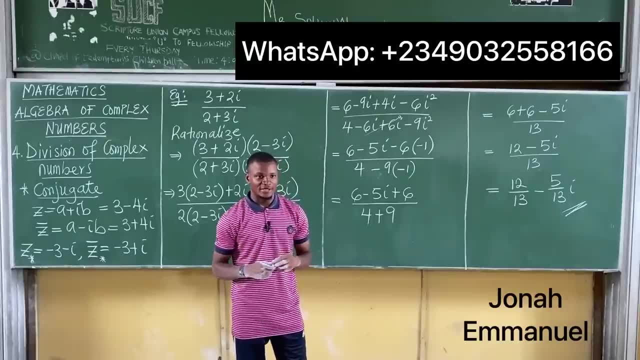 It's just um a real number. So I have this. You can now separate this. So this is how we solve problems on division of complex numbers. Take some other examples and then move on to something else. 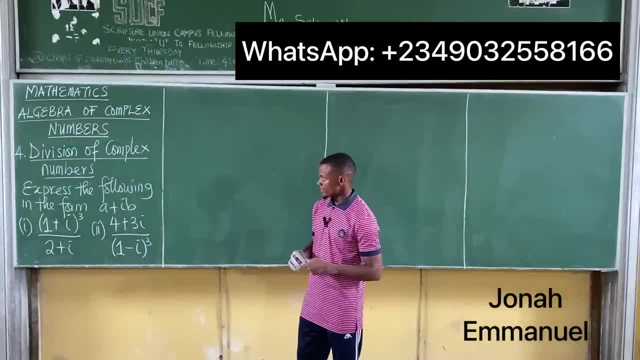 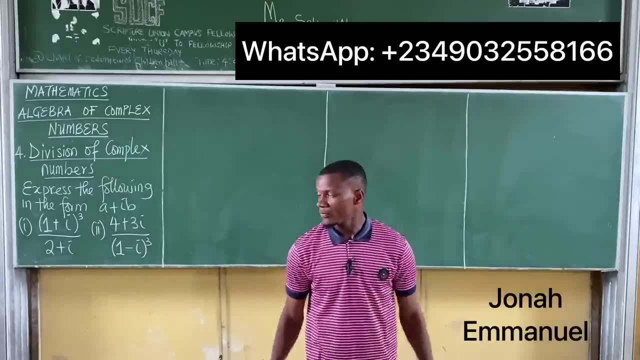 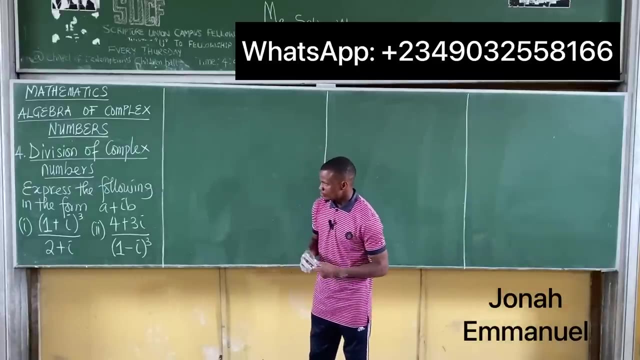 All right, so we'll end the division of complex numbers doing this example. All right, so we'll end the division of complex numbers doing this example. I'll do question one and you do question two. All right. 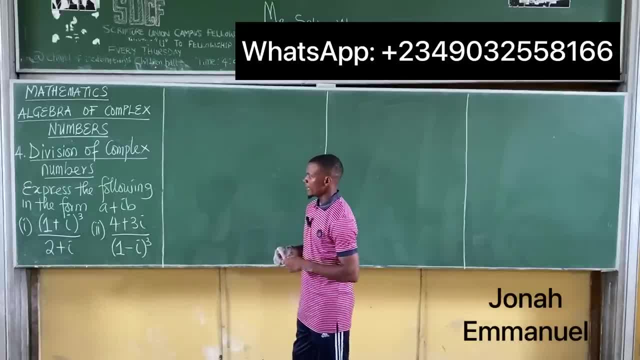 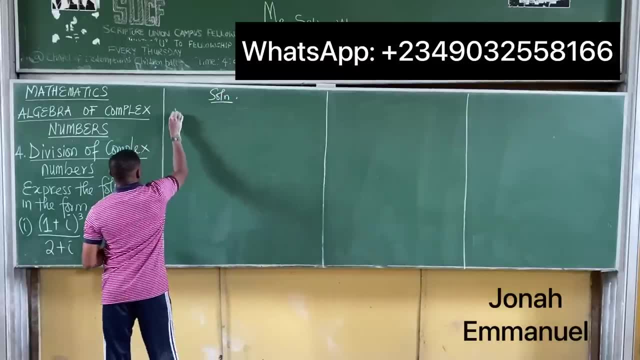 so I express the following in the form: one plus i all cubed all over two plus i. So solution um number one: I'm giving one plus i, all cubed, all over two plus i. 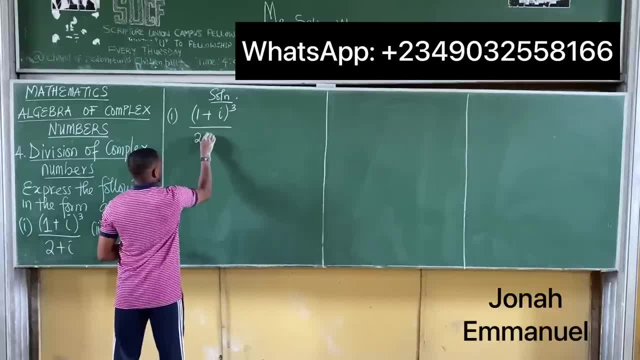 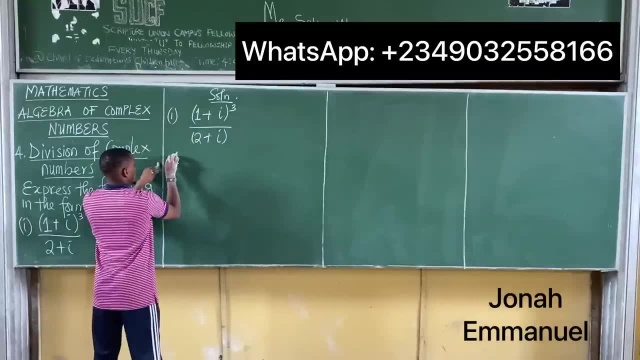 I have this. My first task would be to simplify this. This would be one plus. i cubed Um. I want to use the binomial expansion formula to to, to, to, to, to. 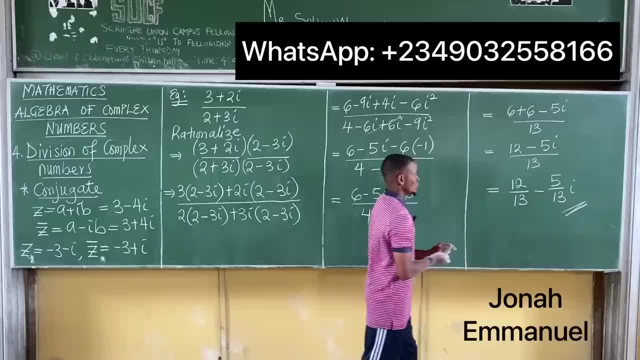 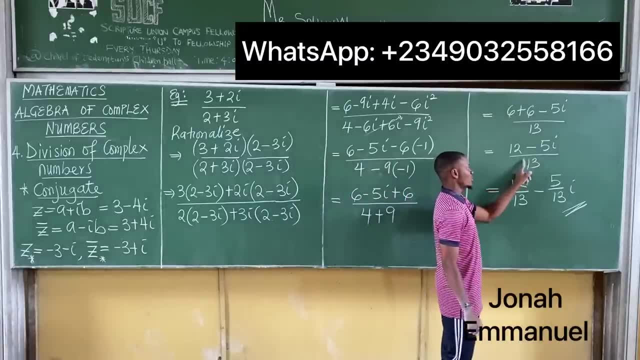 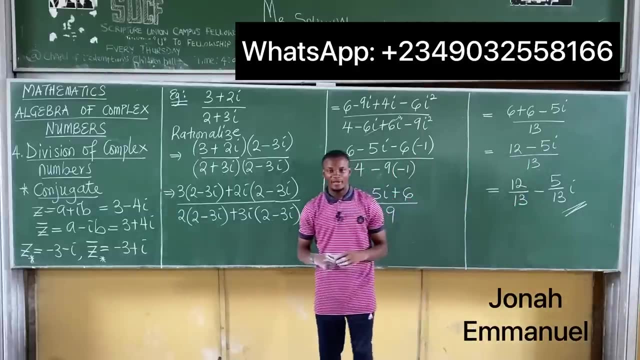 and then I have: i All right. so this is how we do um um division of complex numbers. So observe that the denominator now is no longer a complex number, it's just um a real number. So I have this. You can now separate this. So this is how we solve problems on division of complex numbers. 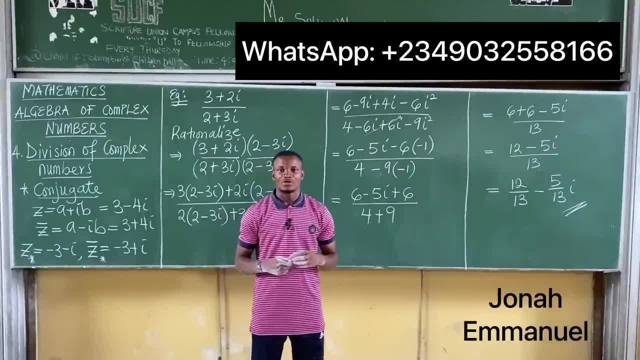 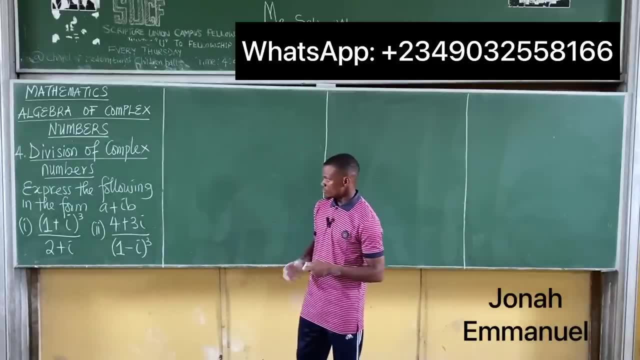 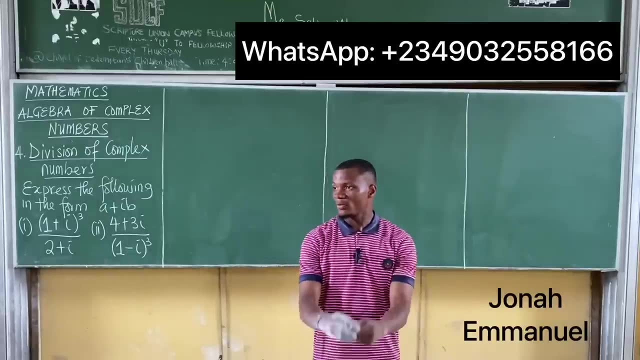 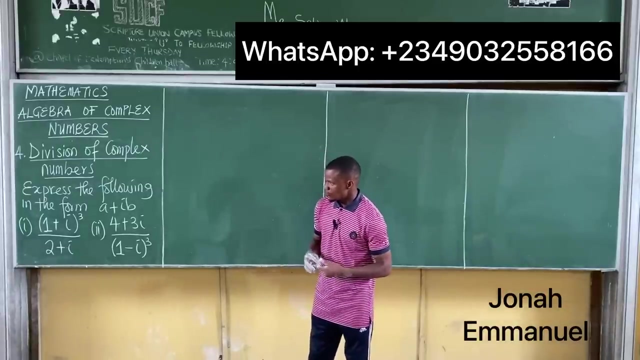 We'll take some other examples and then move on to something else. All right, so we'll end the division of complex numbers doing this example. All right, so we'll end the division of complex numbers doing this example. I'll do question 1, and you do question 2.. 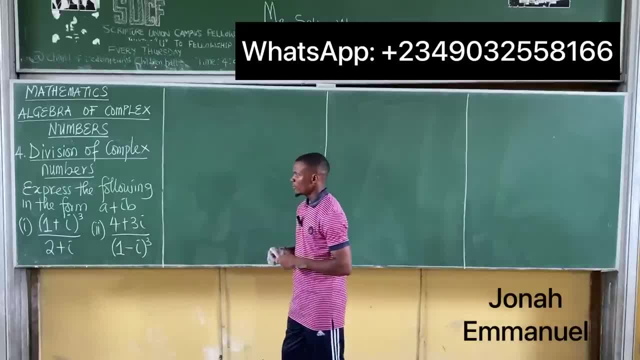 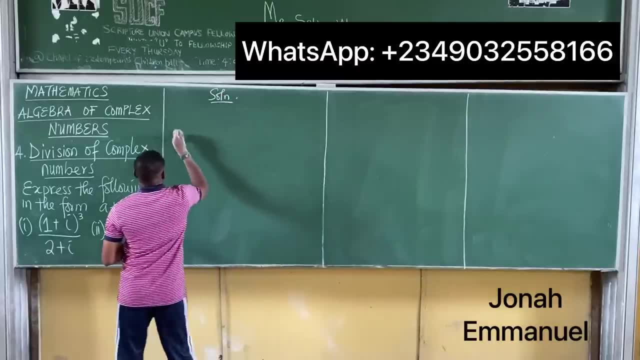 All right. so the question says: express the following in the form: 1 plus i, all cubed all over 2 plus i. So solution um number 1.. Given 1 plus i, all cubed all over 2 plus i, I have this. 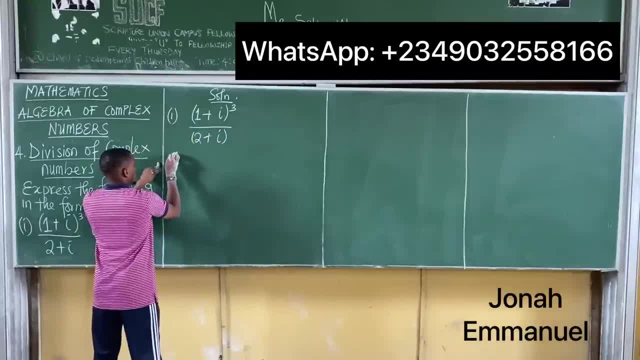 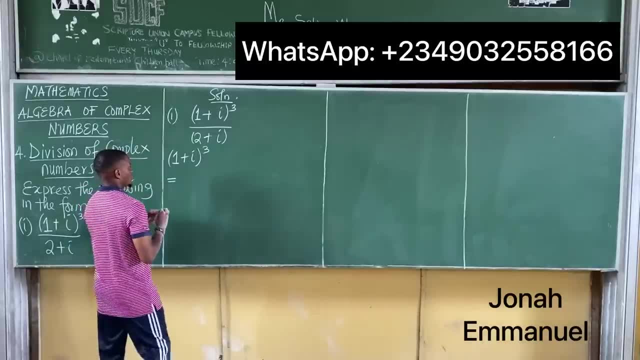 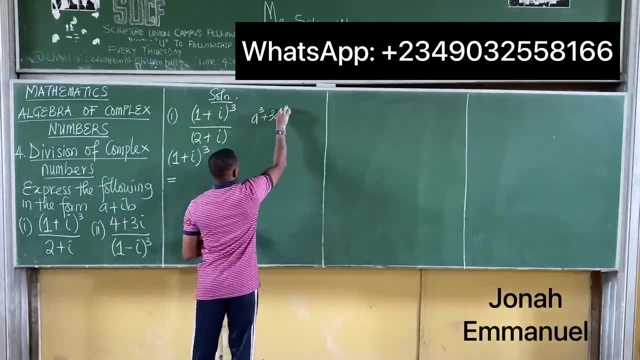 My first task would be to simplify this. This would be 1 plus i cubed, Um. I want to use the binomial expansion formula in which, if I use binomial expansion formula, it's um a cubed plus 3ab, squared plus 3ab. 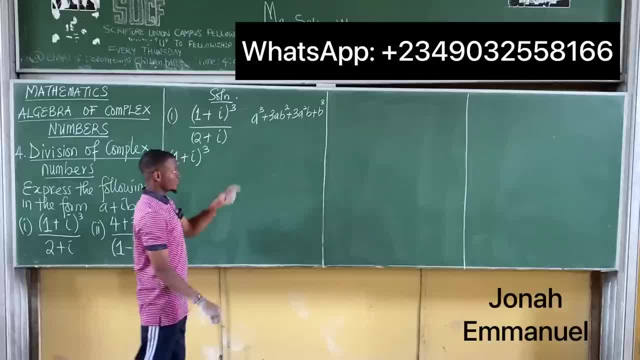 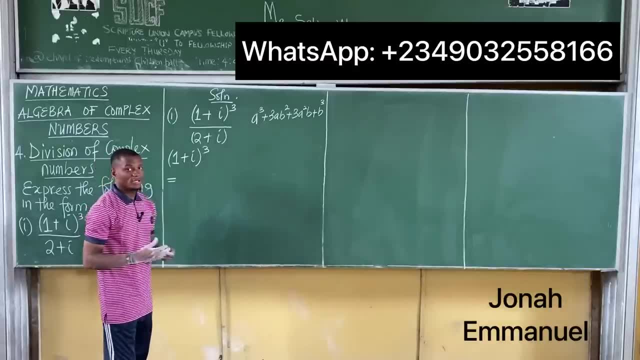 a squared b plus b cubed. We've discussed this in our previous class. binomial expansion: I'll leave a link to this um binomial expansion in the comment section. Just take sorry- in the description of this video. I'll leave um a link to binomial expansion. 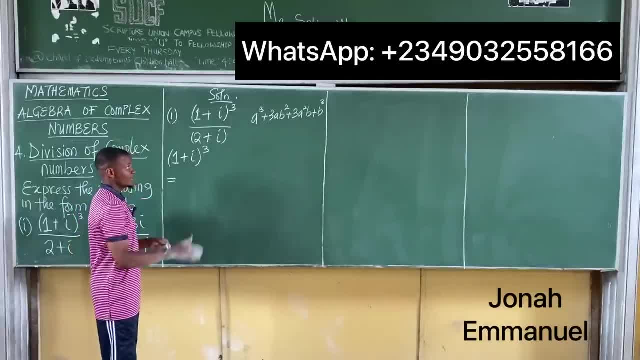 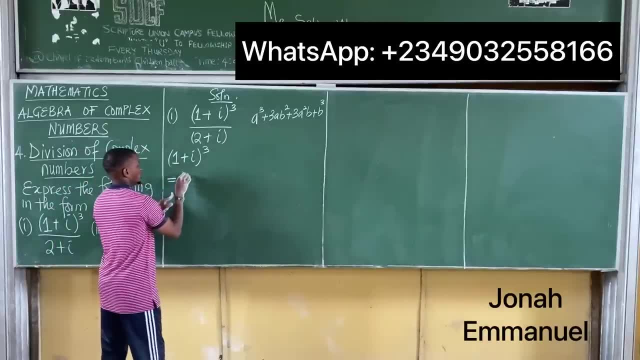 Or perhaps you could just go through our playlist for mathematics and you'll see the video on binomial expansion. So if I use this concept here, a is 1, so it becomes 1 cubed. 1 cubed Plus 3 into a is 1, into b: squared. 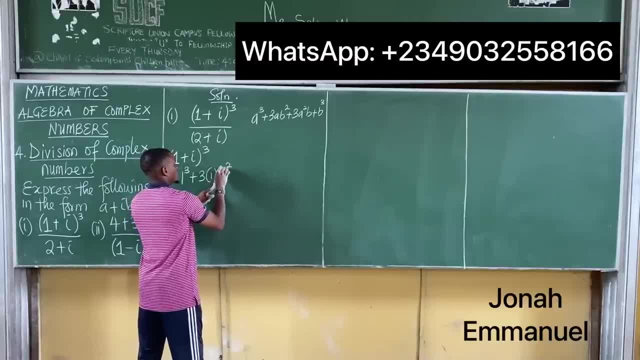 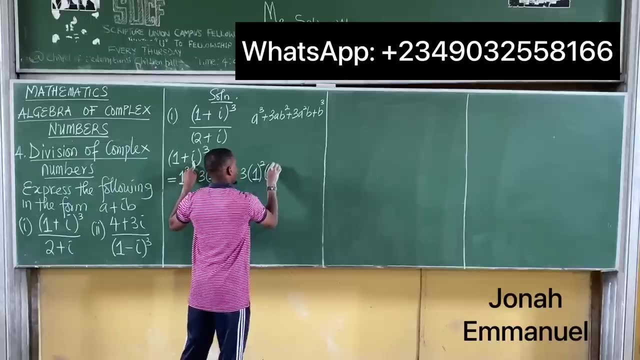 b is now i, so it becomes i squared. This is i squared. Okay, so here's 1.. Here's 1.. Plus 3 into a squared, a is 1, so it becomes 1 squared times b. b is i plus b cubed. 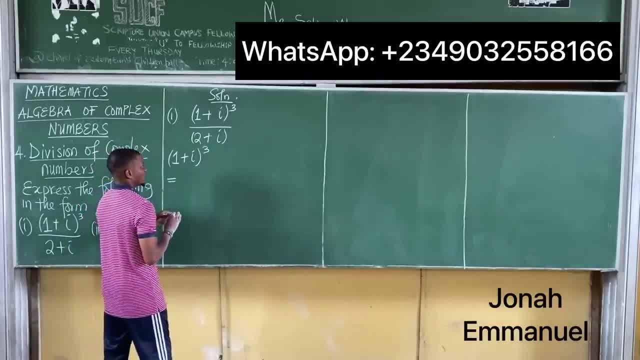 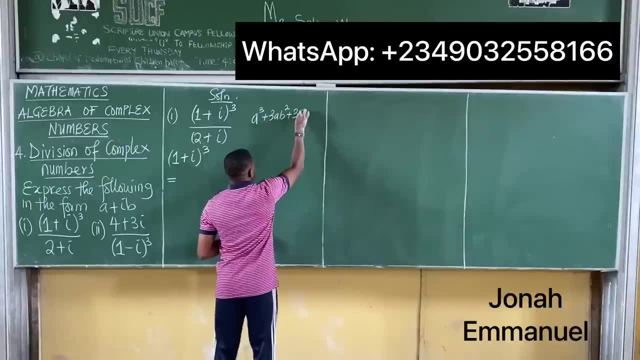 in which, if I use binomial expansion formula, it's: uh i-cubed plus three, a b-squared plus three a-squared, b plus b-cubed. We've discussed this. 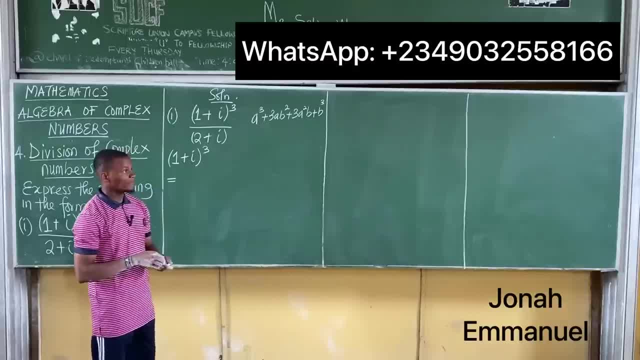 in our previous class, binomial expansion. I'll leave a link to this um, binomial expansion in the comment session. So just sorry. in the description of this video I'll leave um, perhaps you could just go through our playlist for mathematics and you see the video on binomial. 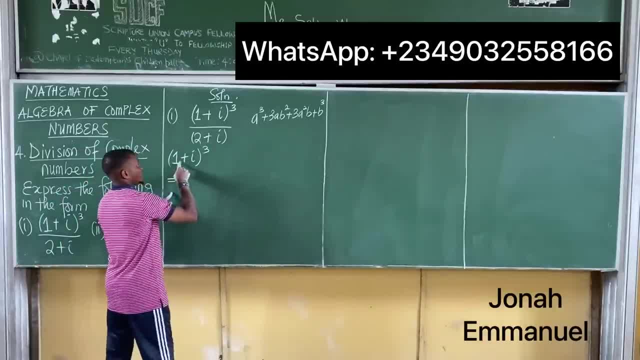 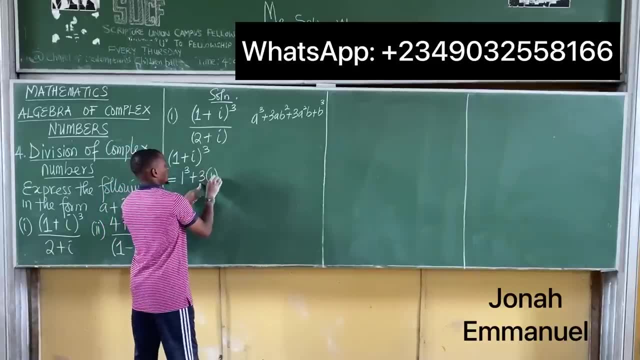 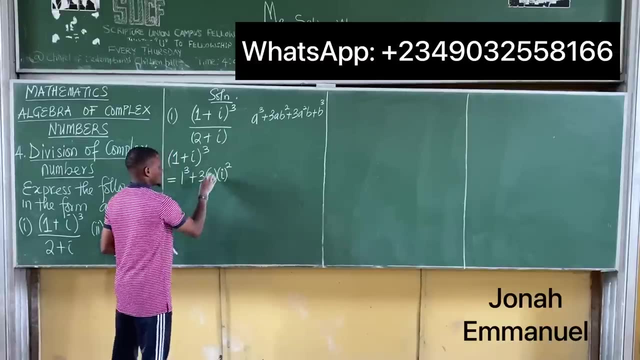 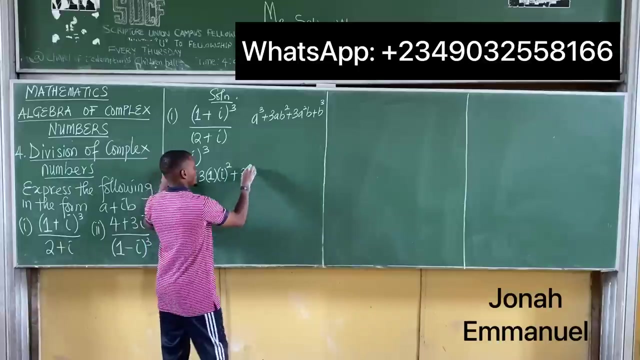 expansion. so if i use this concept here, a is one, so it becomes one. cube plus three into a is one. into b. squared b is now i, so it becomes: i squared this, i squared okay. so here's one, here's one plus three into a squared a is one, so it becomes one. squared times b, b is i. 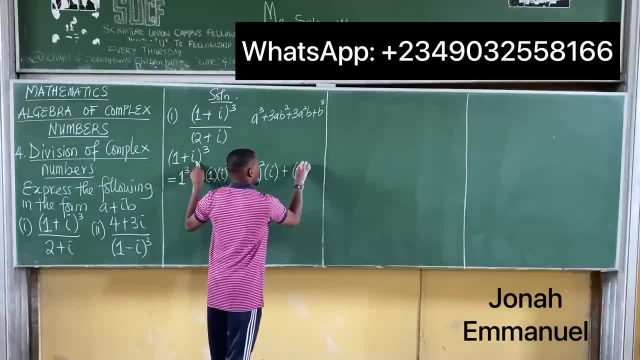 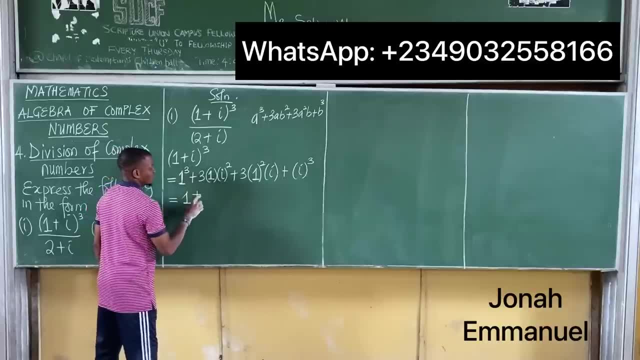 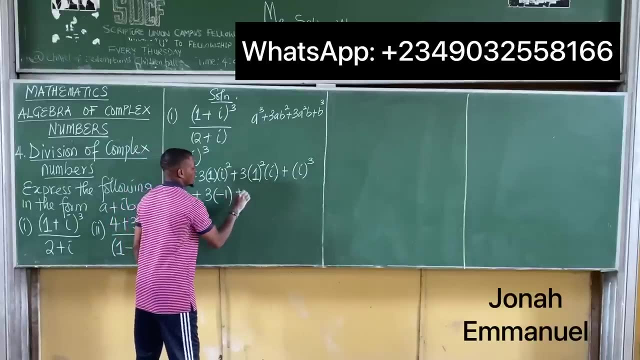 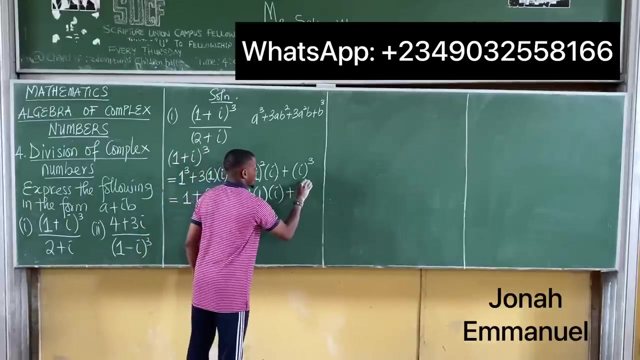 plus b cube, that becomes i cube. if i work on this, this is equal to one cube is one plus three times one is three times i squared. we said i squared is minus one plus three times one squared is equal to one times i plus i cube. so i have this all right, so this is equal to one. 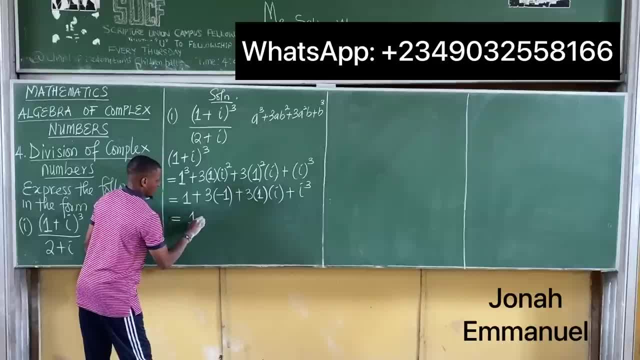 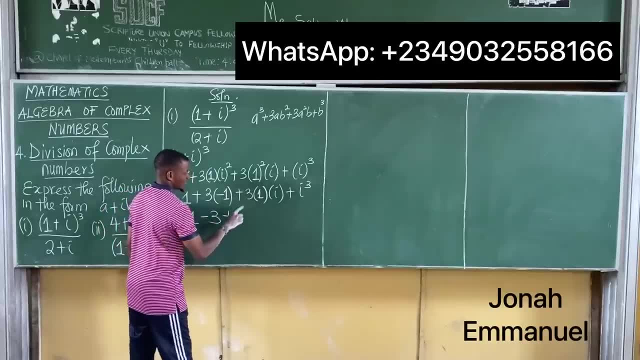 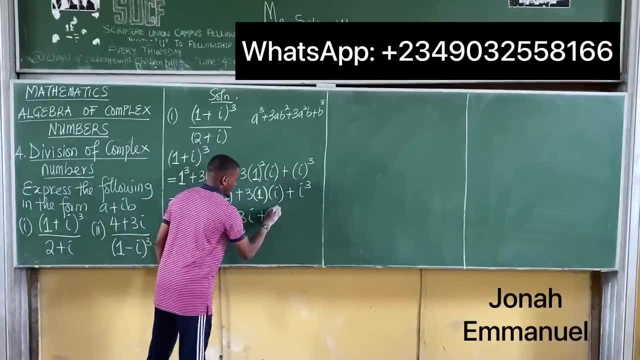 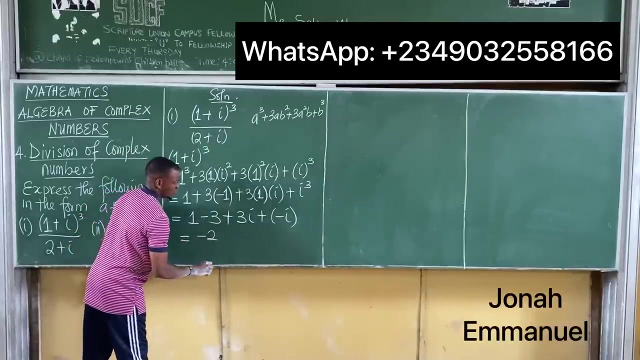 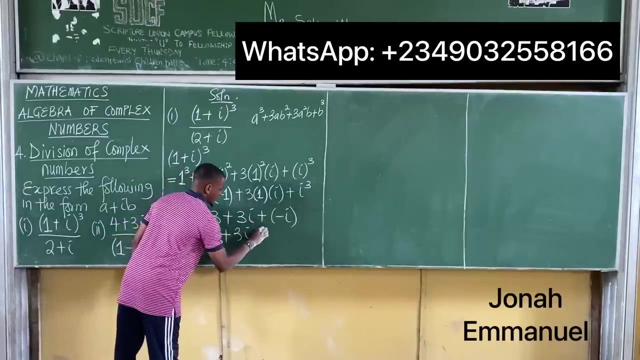 three. three plus times minus is minus three times one is three plus three times one is three times i is three. i plus i cube is that is equal to minus i. So this is equal to 1 minus 3 is minus 2, 3i. so plus 3i plus minus is minus i. 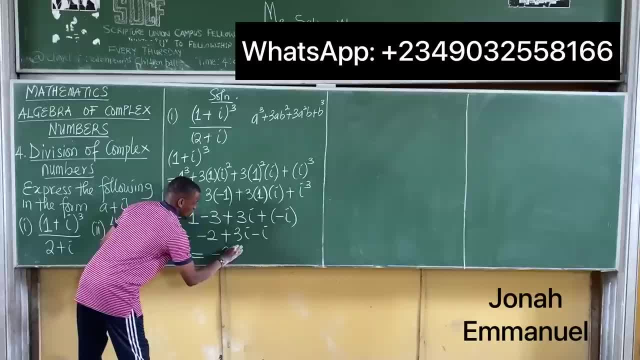 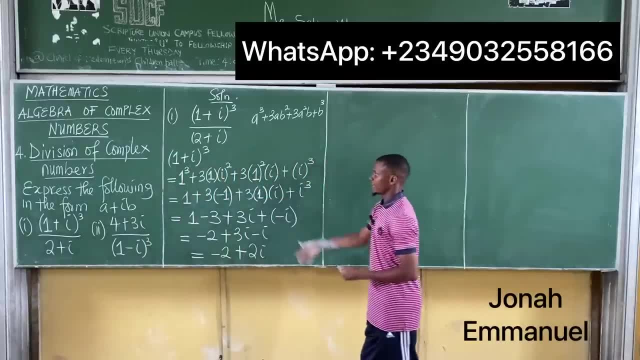 If you simplify this, that's equal to minus 2 plus 3. minus 1 is 2i, So I've gotten my answer. So this is like a faster approach on how to expand this. So it's better you learn how to use binomial expansion. 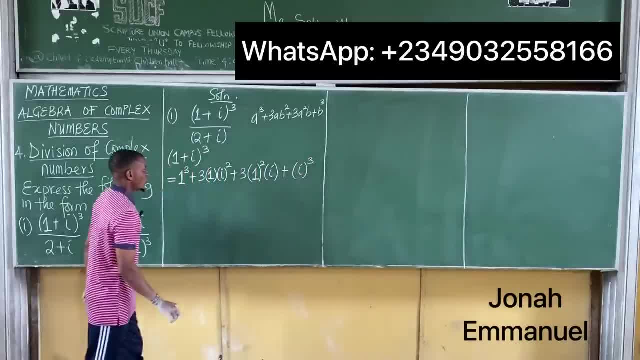 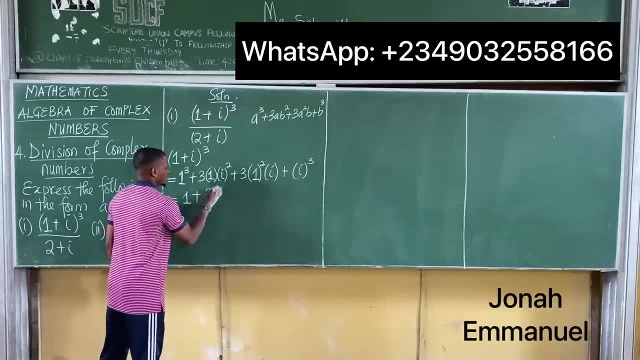 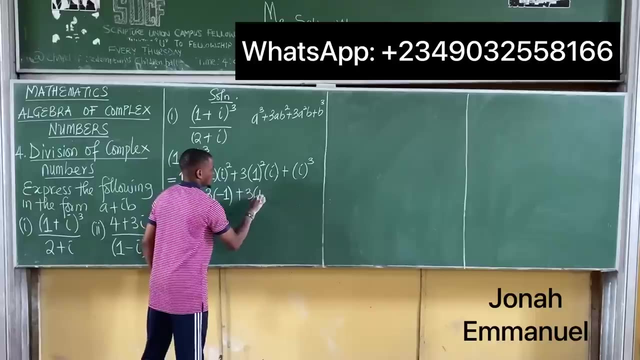 That becomes i cubed. If I work on this, this is equal to 1. cubed Is 1 plus 3 times 1 is 3 times i squared. We said i squared is minus 1, plus 3 times 1 squared is equal to 1 times i plus i cubed. 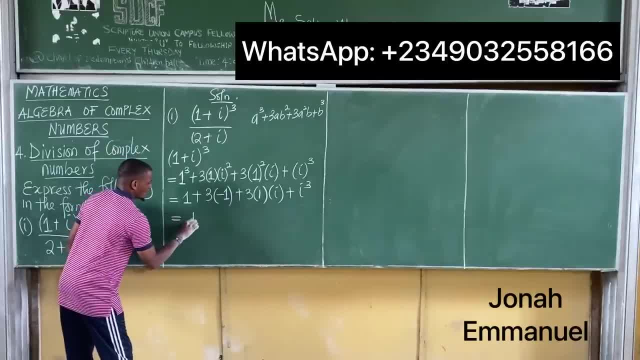 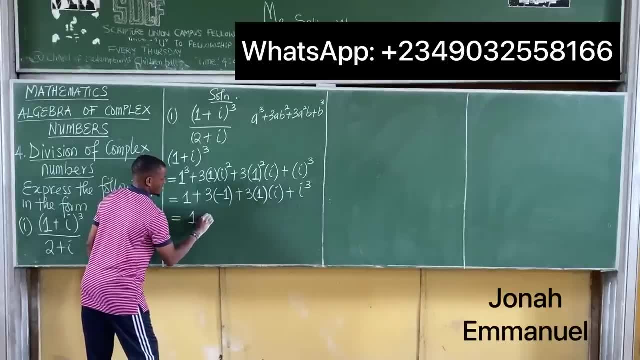 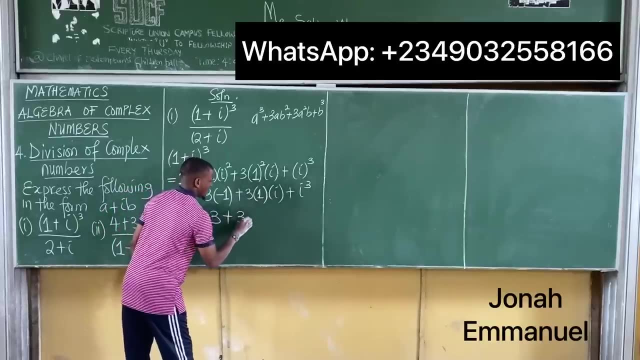 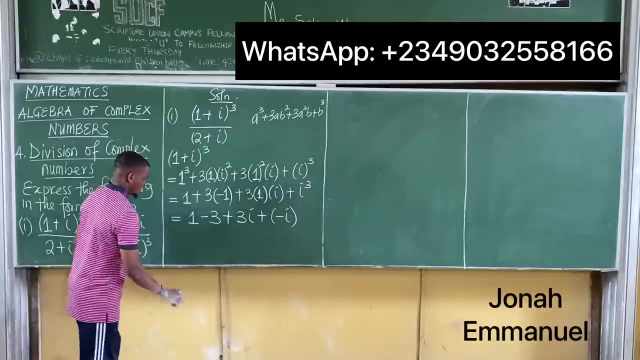 So I have this Alright. so this is equal to 1.. 3, 3, plus times minus is minus 3 times 1 is 1.. is 3 plus 3 times 1 is 3 times i is 3i plus i cubed, so that is equal to minus i. so this is. 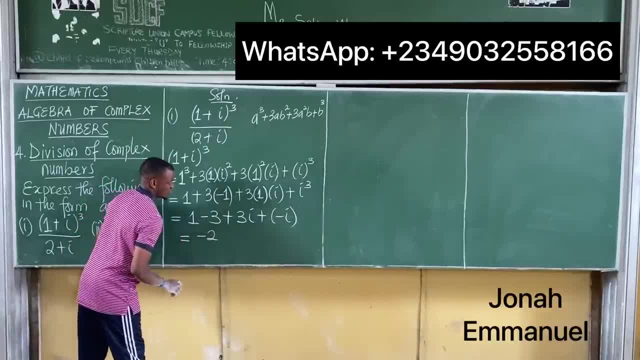 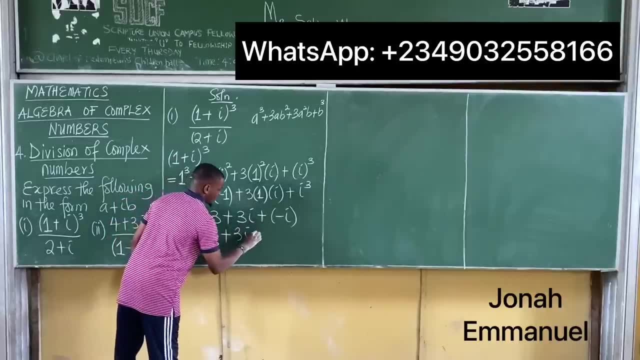 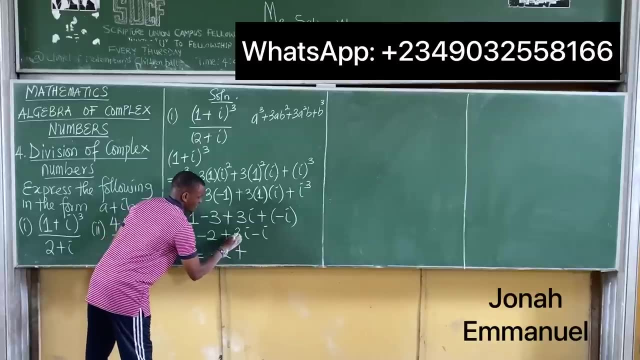 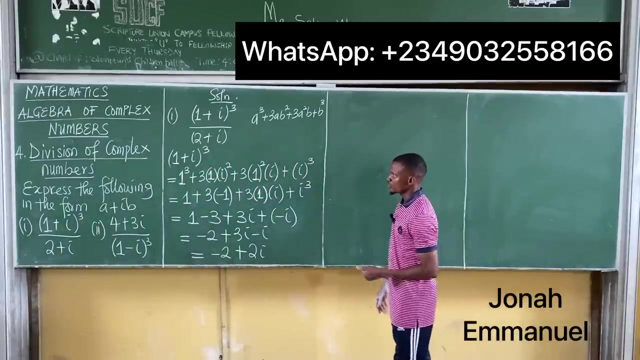 equal to 1 minus 3 is minus 2, 3i. so plus 3i plus minus is minus i. if you simplify this, that's equal to minus 2 plus 3 minus 1 is 2i. so i've got my answer. so this is like a faster approach on how. 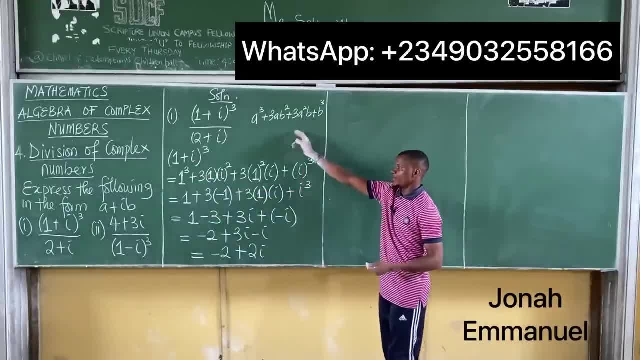 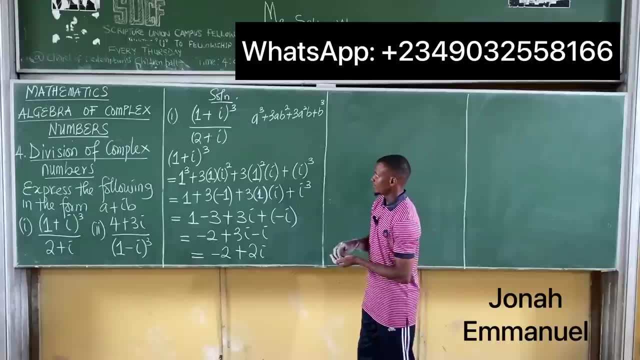 to expand this. so it's better you learn how to use binomial expansion instead of going, instead of having to multiply this one itself twice. that's way longer, so it's better you learn how this is done. i'll leave a link to the video lesson on binomial expansion. 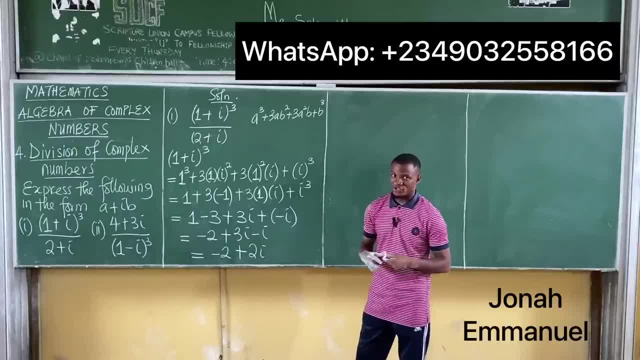 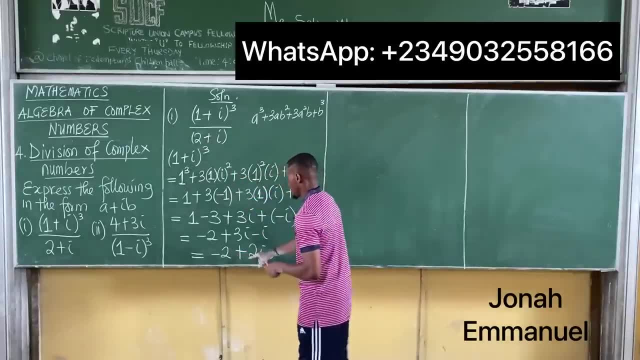 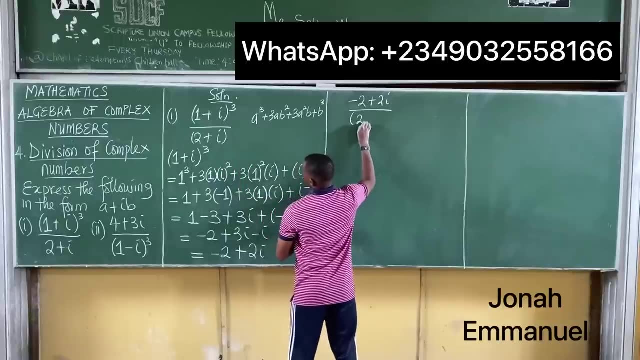 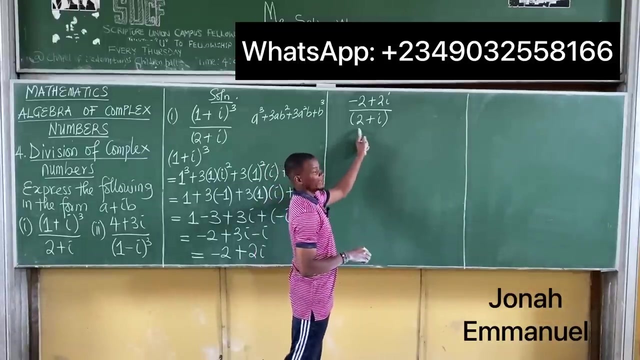 in the description of this video so you can check the description of this video for the lesson on binomial expansion. let's proceed. so it means that all of these numerators, nowadays that's minus two plus two, i, all over denominator 2 plus i. so we have this one here. what's wrong here is that my denominator is a complex number. 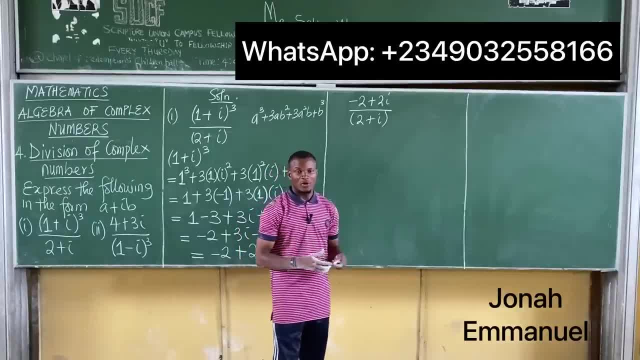 and we said it is improper to leave the denominator of a fraction as a denominator of equivalent dual types of no Aqua, 2 times i minus 2 times 2i in my polynomial. So we just need to make some a complex number. so in this case, what do I do? I'll have to multiply both. 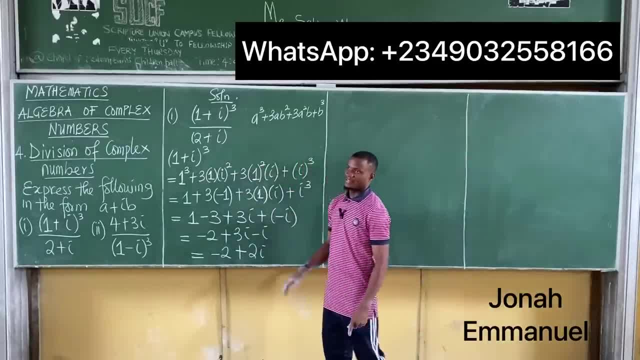 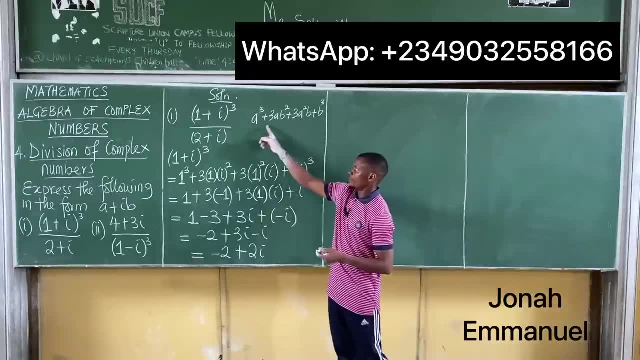 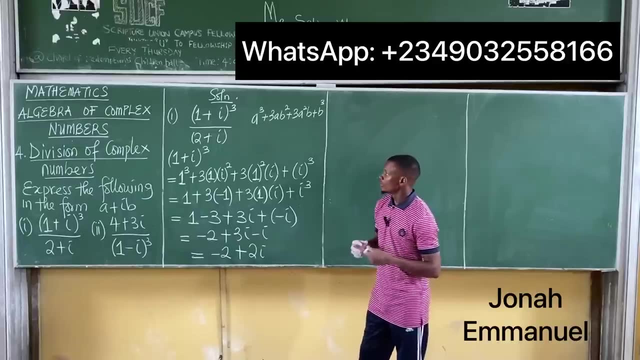 Instead of having to multiply this one itself thrice. that's way longer, So it's better you learn how this is done. I'll leave a link to the video lesson on binomial expansion in the description of this video, So you can check the description of this video for the lesson on binomial expansion. 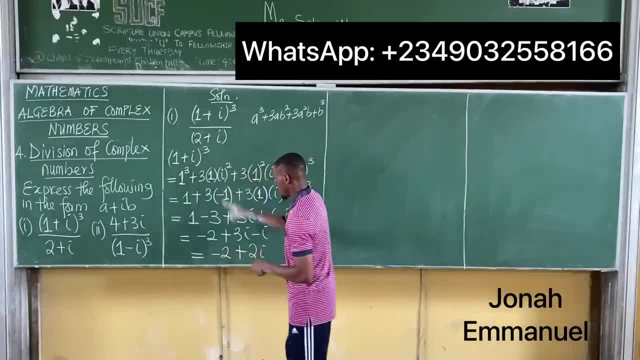 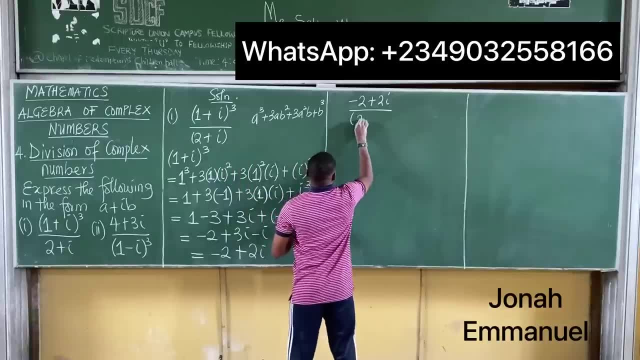 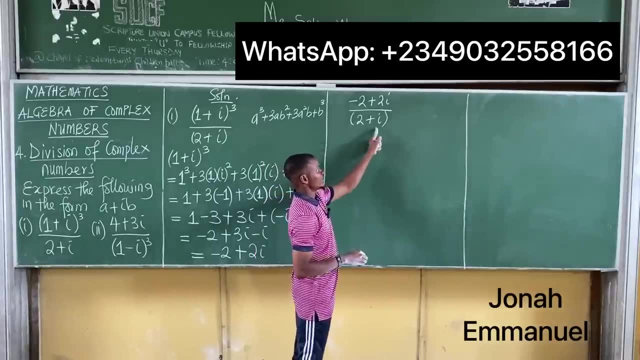 Let's proceed. So it means that all of this numerator is now this: That's minus 2.. Plus 2i all over denominator 2 plus i. So we have this one here. What's wrong here is that my denominator is a complex number. 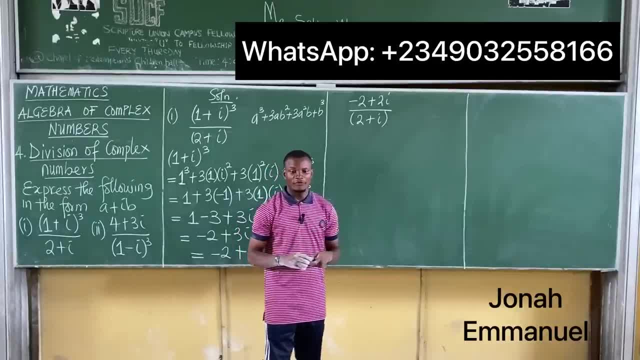 And we said it is improper to leave the denominator of a fraction as a complex number. So in this case, what do I do? I'll have to multiply both numerator and denominator by the conjugate of denominator. So multiply this, This one, here. 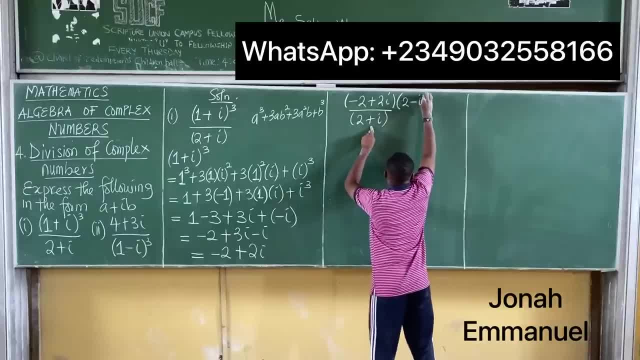 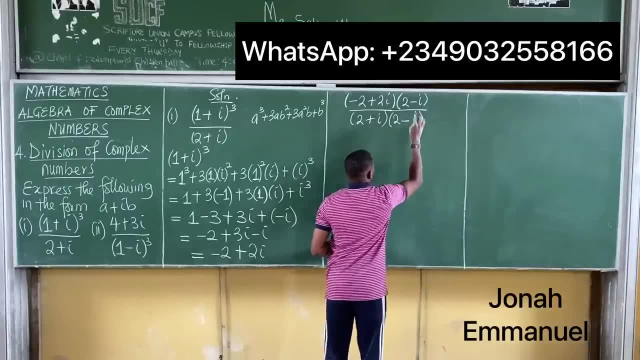 Multiply This by the conjugate of this. That becomes 2 minus i. all over. Multiply this by its conjugate 2 minus i. So I have this. So this is now equal to Use the first term, Minus 2.. 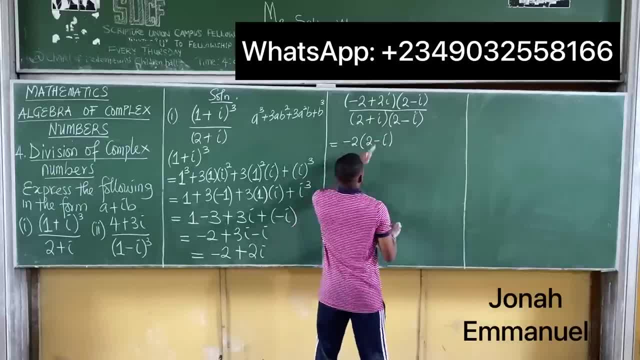 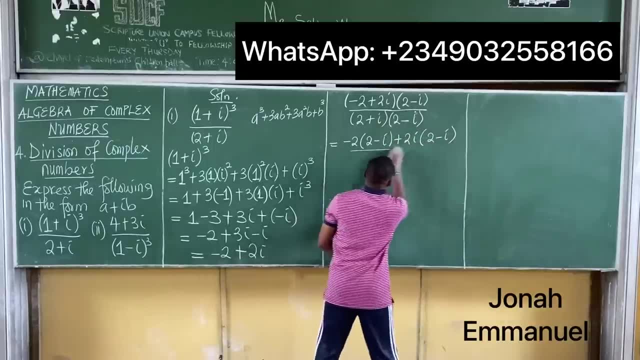 Multiply everything here: 2 minus- i Use the second term- Plus 2i. Multiply everything here: 2 minus i All over. Use the first term here: 2.. Multiply everything here: 2i, 2 minus i. 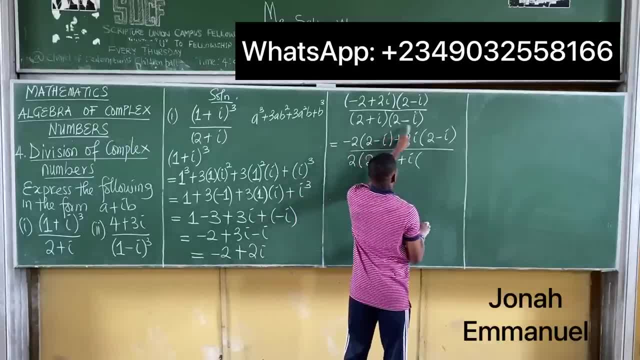 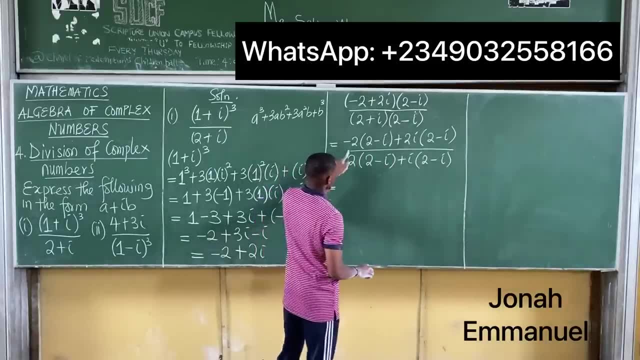 Use the first term here: Plus. i Multiply everything here: 2 minus i, So I have this All right. So this is now equal to Minus 2 times 2 is minus 4.. Minus times minus is plus. 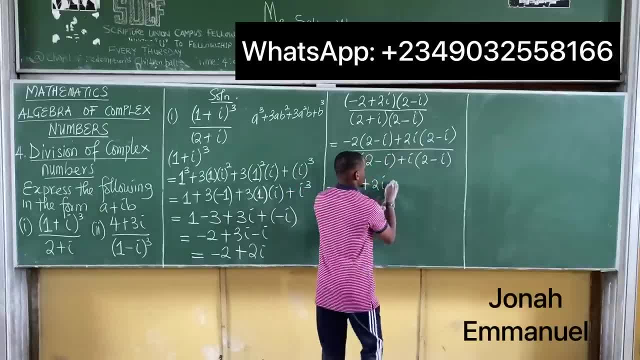 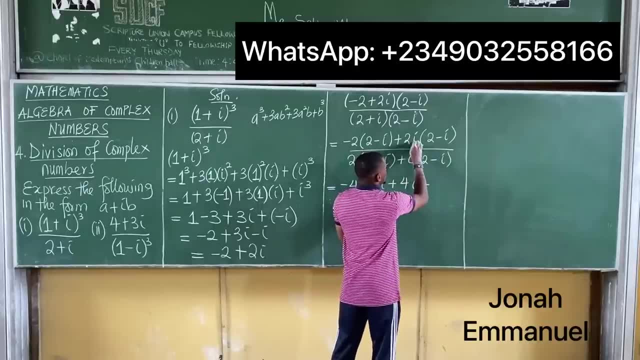 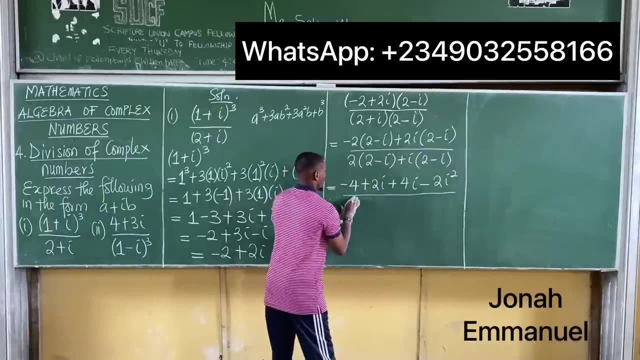 I have the 2i Plus times. plus is plus 2 times 2 is 4.. Bring the i down: Plus times minus is minus 2i times i Is 2i. squared All over 2 times 2 is 4.. 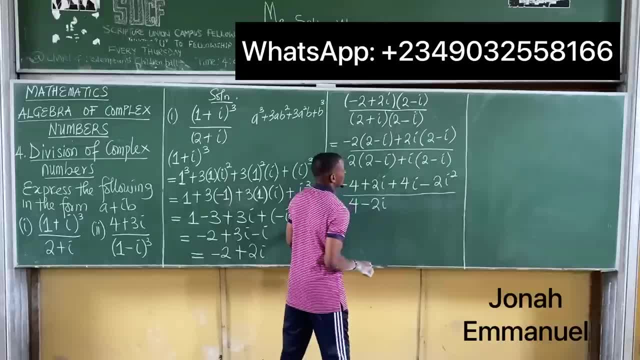 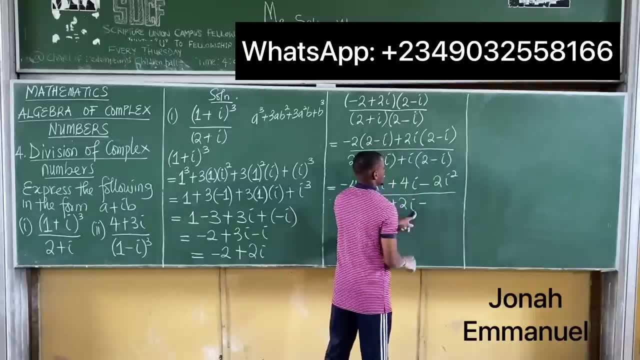 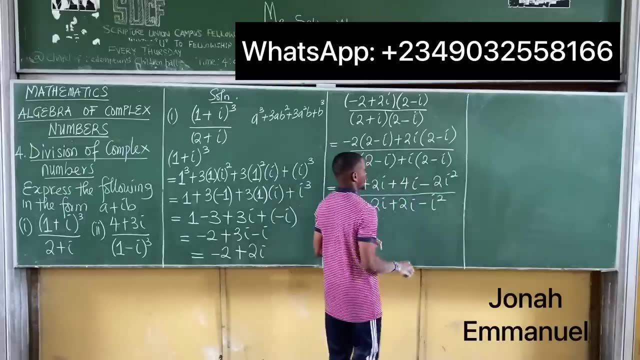 2 times minus i Is minus 2i, Plus i times 2.. Is plus 2i Plus times minus is minus i times i Is i squared. So we have this All right, So work this out. 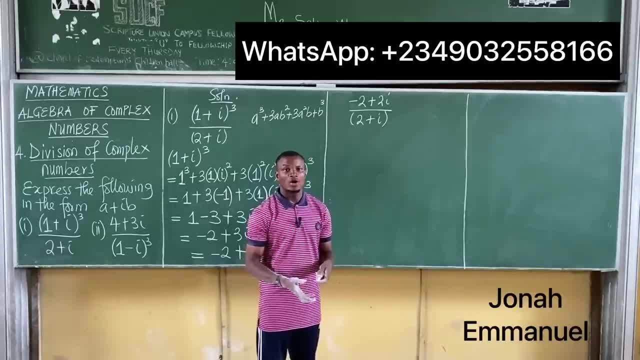 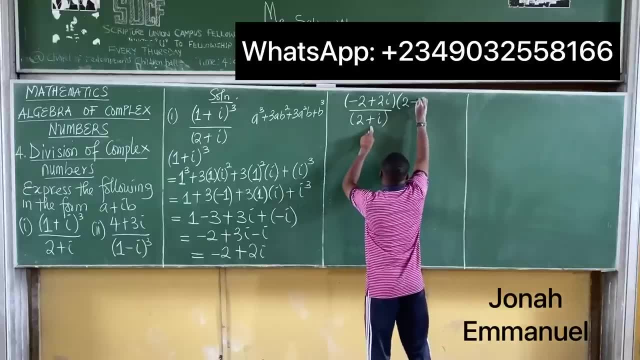 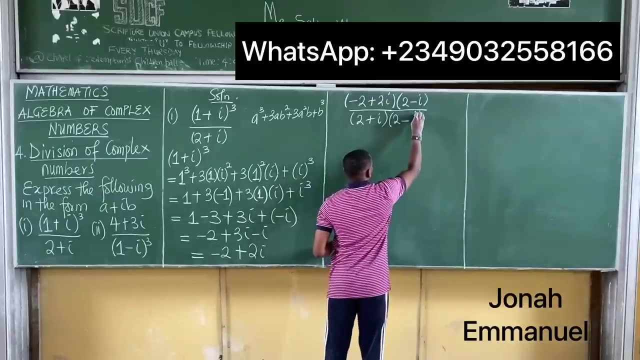 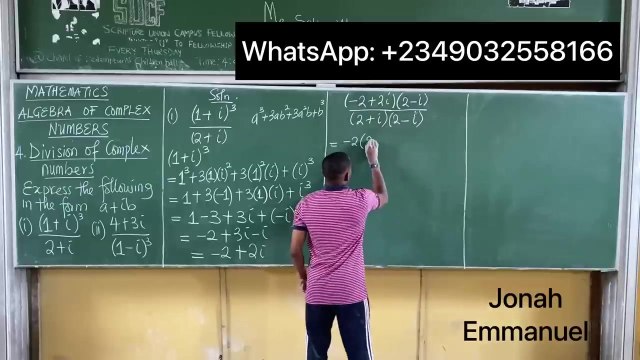 numerator and denominator by the conjugate of denominator. so multiply this, this one here. multiply this by the conjugate of this. that becomes 2 minus i, all over. multiply this by its conjugate: 2 minus i. so I have this. so this is now equal to use the first time minus 2. multiply everything here: 2 minus my use. 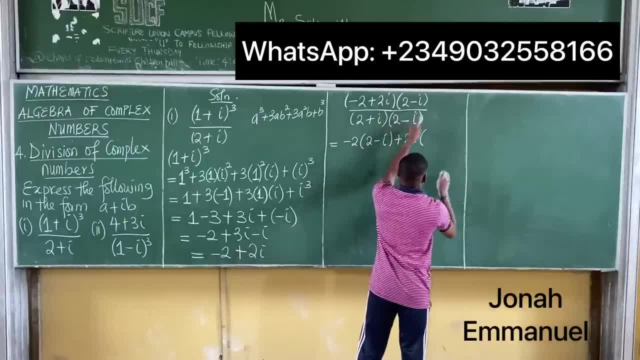 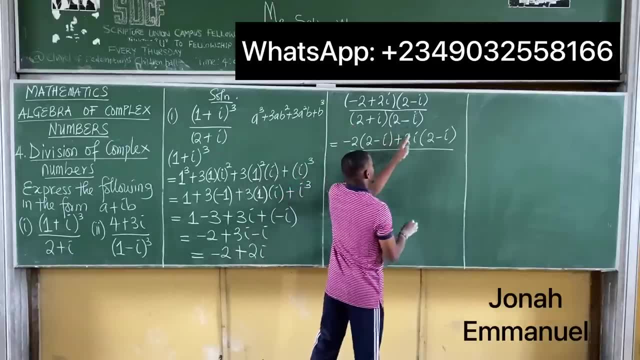 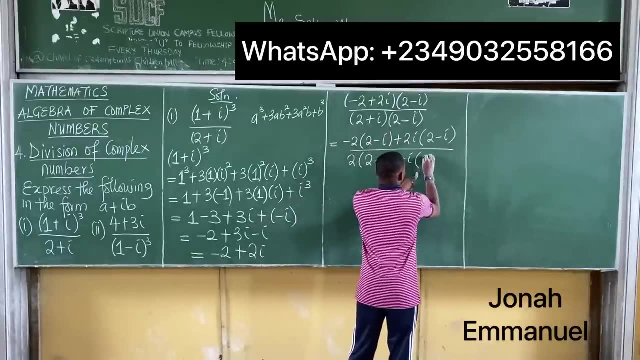 the second term plus 2i. multiply everything here 2 minus. i all over use the first time here to multiply everything here 2 minus. i use the first time here plus. i multiply everything here to minus i. so I have this alright, so this is now equal to. 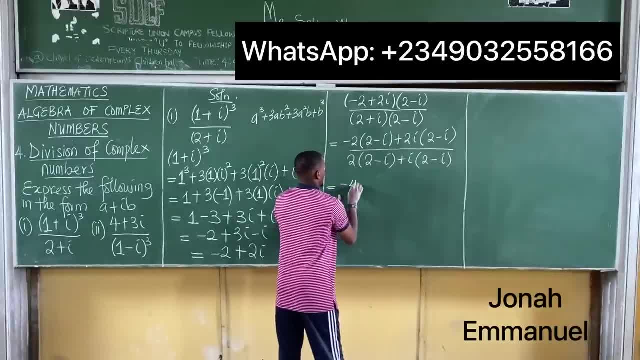 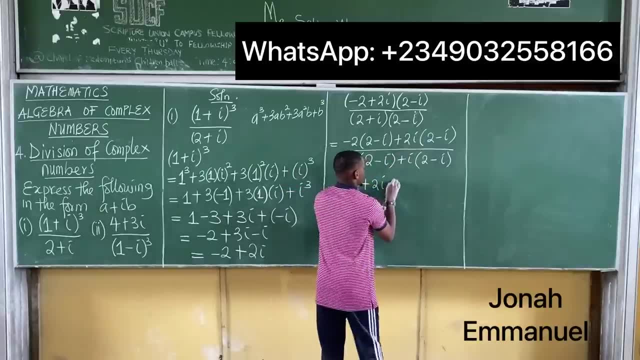 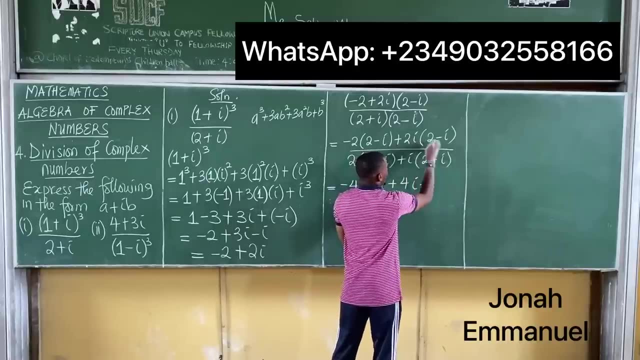 minus 2 times 2 is minus 4. minus times minus is plus. I have the 2i. plus times plus is plus 2 times 2 is 4. bring the i down. plus times minus is minus 2i times i is 2i squared. 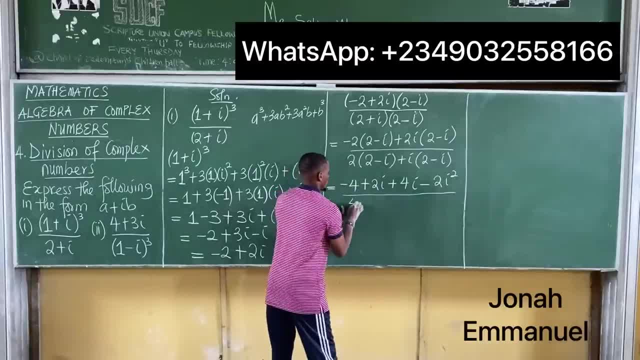 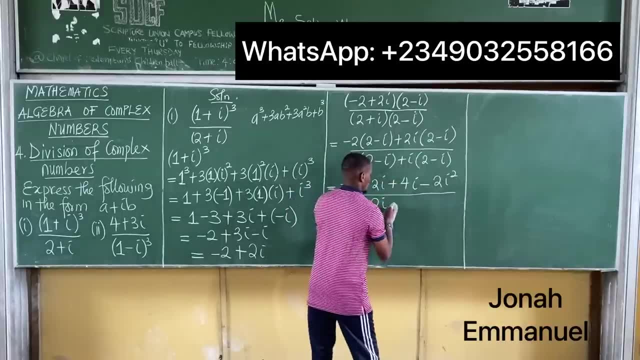 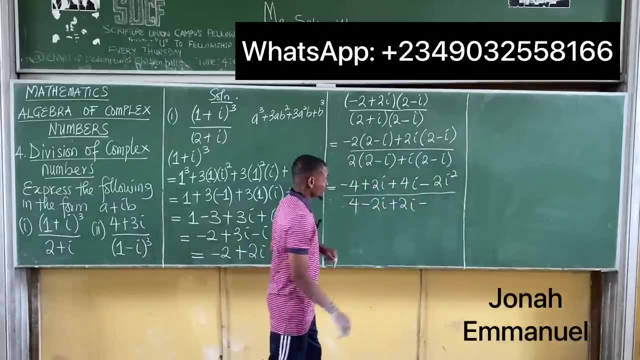 all over. 2 times 2 is 4. 2 times minus i is minus 2i. plus i times 2 is plus 2i. plus times minus is minus i times i is i squared. so we have this all right, so work this out. 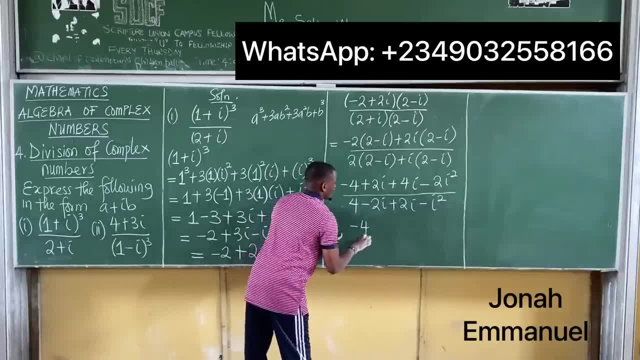 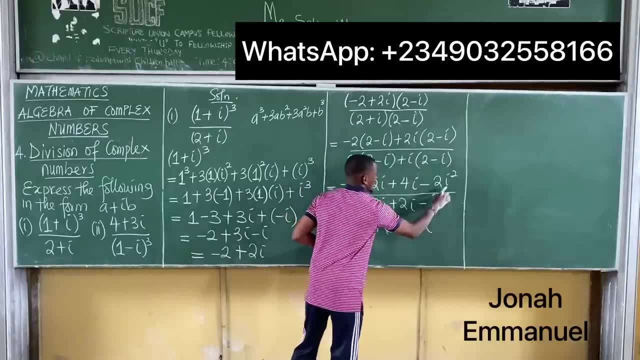 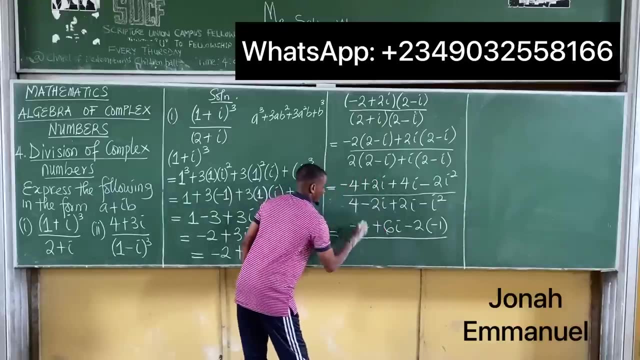 this is equal to I'm having here is minus 4 plus 2 plus 4 is plus 6i minus 2 into i squared. we said i squared is minus 1, all over. this is 4 minus 2 plus 2. we'll cancel out. 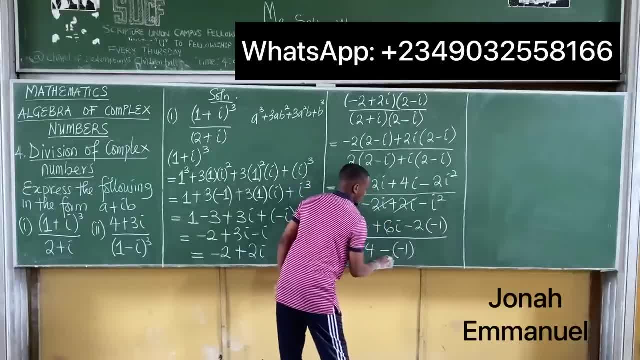 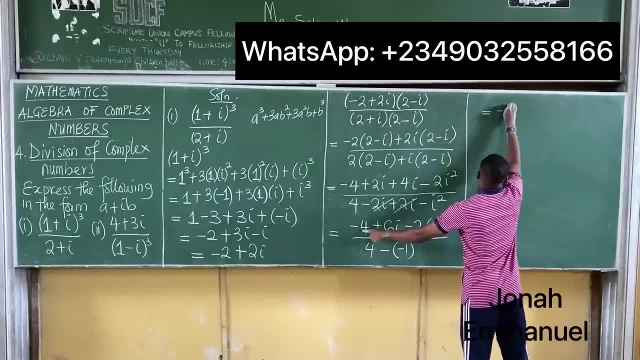 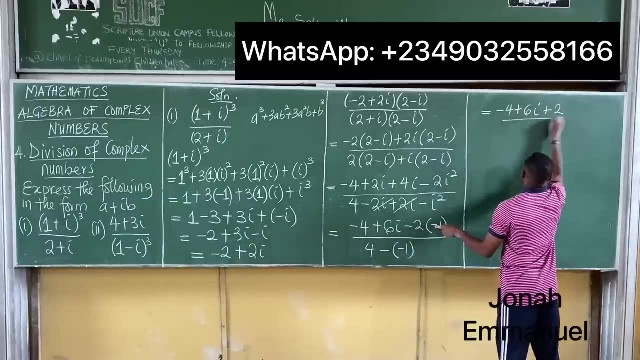 minus i squared is minus 1, so minus i squared is minus 1. we have this, so this is equal to I'm having. here is minus 4 plus 6i, minus minus plus 2. all over this is 4 minus minus plus 1.